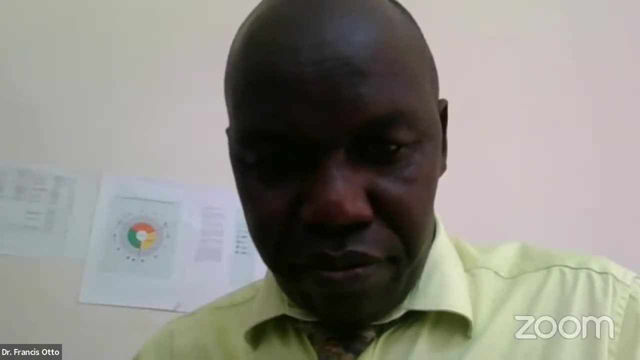 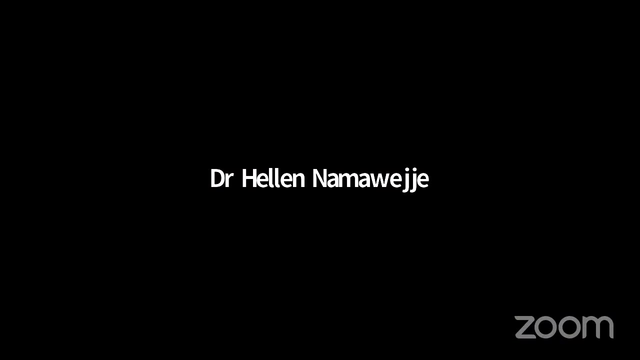 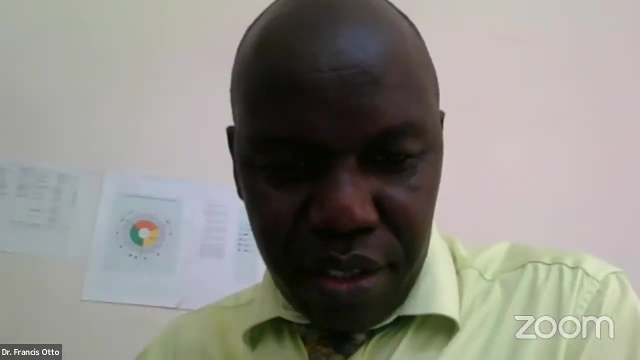 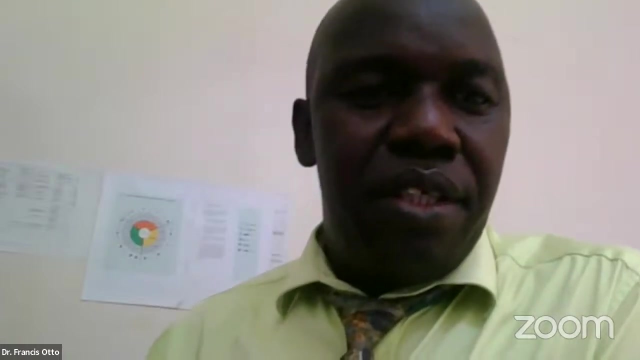 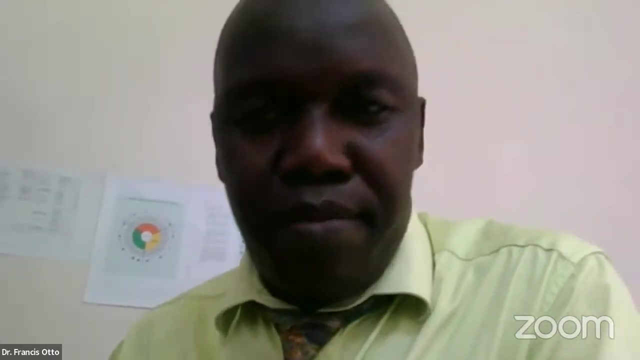 Yes, Francis, we can. Good morning, good morning. Good morning. I think one of you should mute the lowered volume. Okay, I take this opportunity to greet you and send you warm greetings from Roo Forum Secretariat here in Kampala. I do understand. 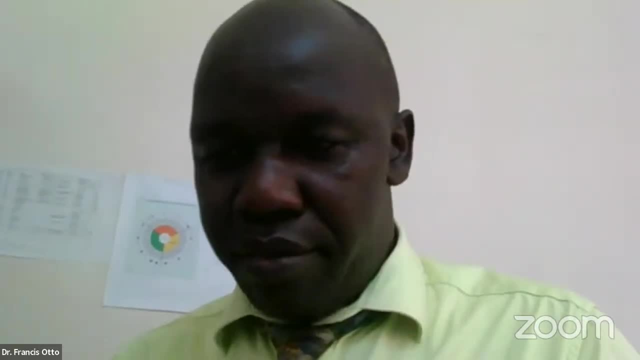 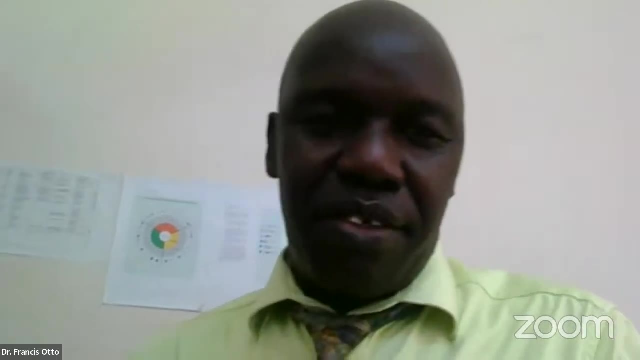 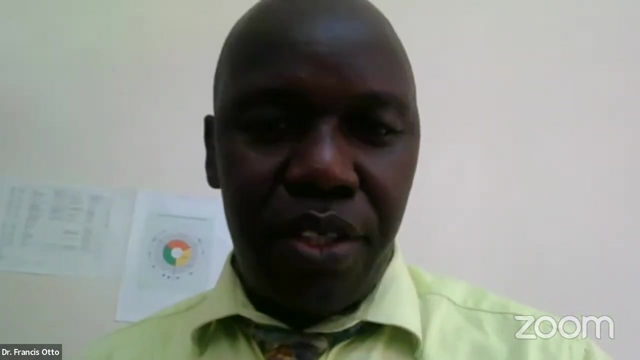 we have now about 150 people already logged in from different places. I can see people from Cameroon, Nigeria, Ghana, several African countries. This training was designed targeting staff and postgraduate students of Makerere University. However, because of the importance of this training, we do welcome. 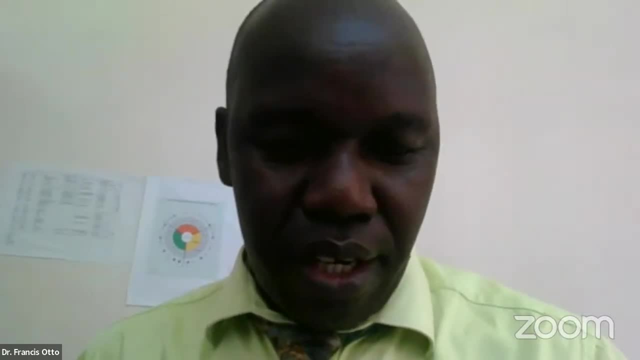 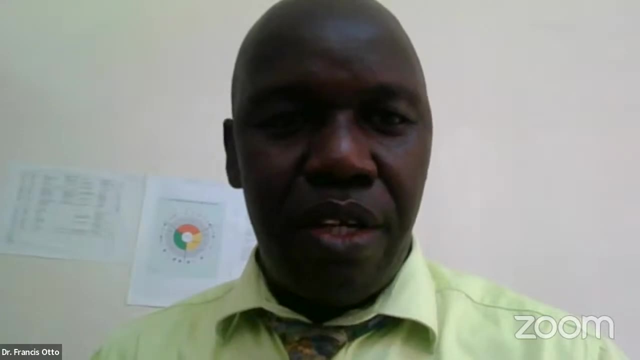 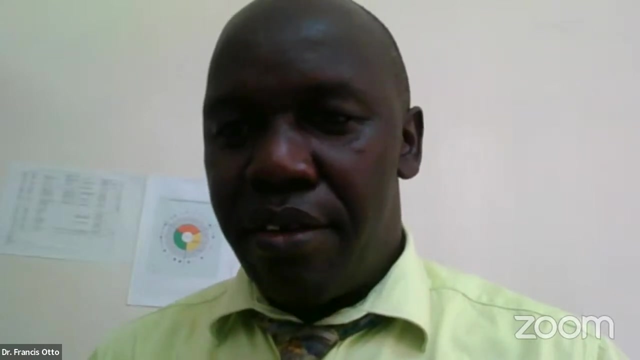 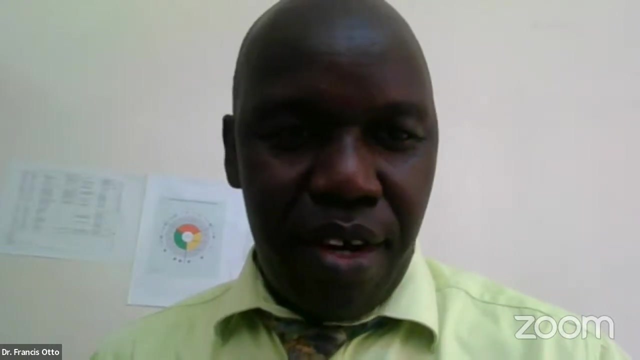 other participants from across the Roo Forum network, And I would like first of all to introduce the trainers and then say a few words to welcome you. This morning we shall have three excellent trainers who will be taking you through the six days. We have Associate Professor. 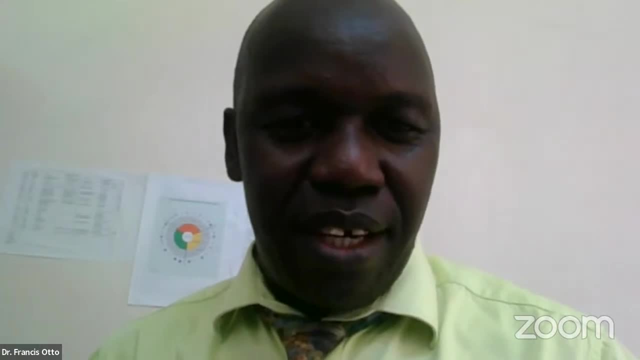 Susan Balaba, who is a staff at Makerere University and has been helping us at Roo Forum in building capacity in this particular aspect of research training. And then we have Dr Helen Namawetje, who is also one of the staff members at Makerere University. They will give you details. 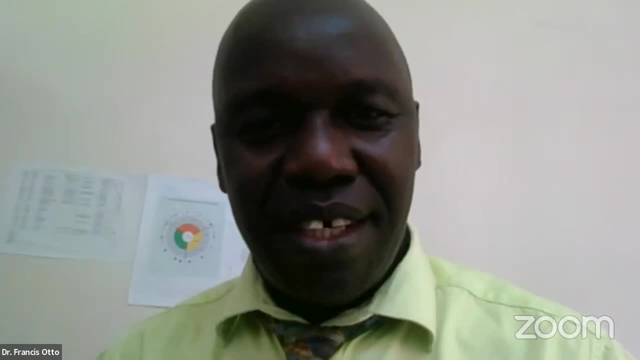 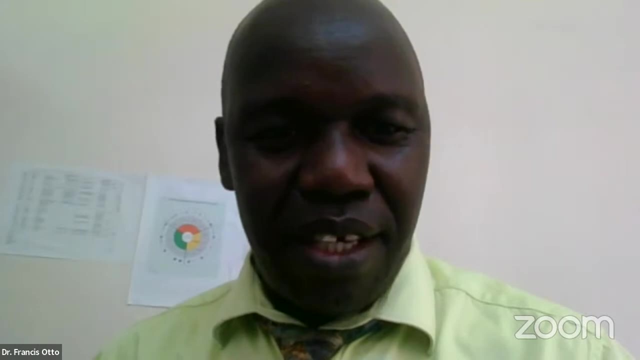 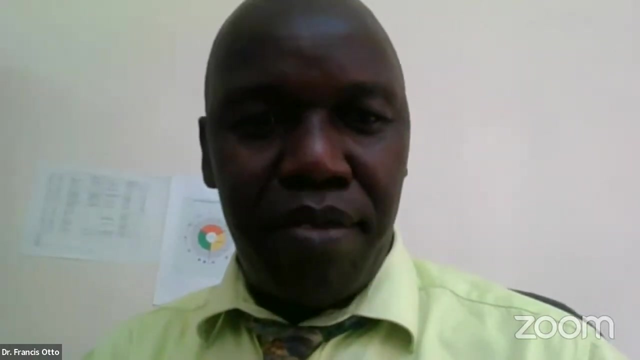 of themselves when the training time begins. Then we have Dr Thomas Odom, who is also a staff at Makerere University. What is interesting is that the three of the trainers come from Makerere University, but from different departments. but they are all. 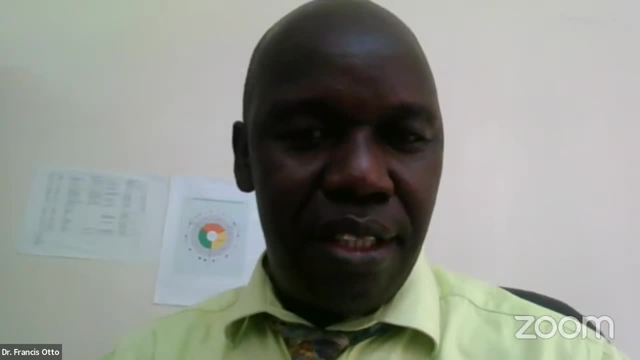 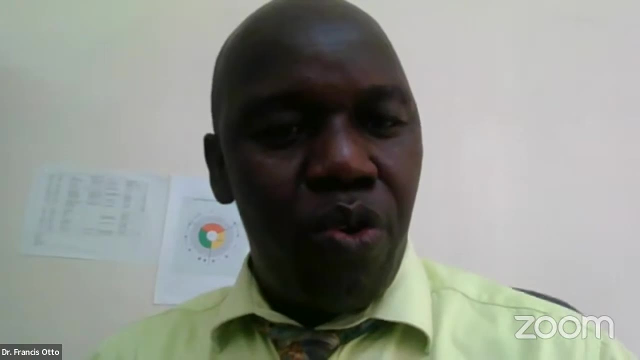 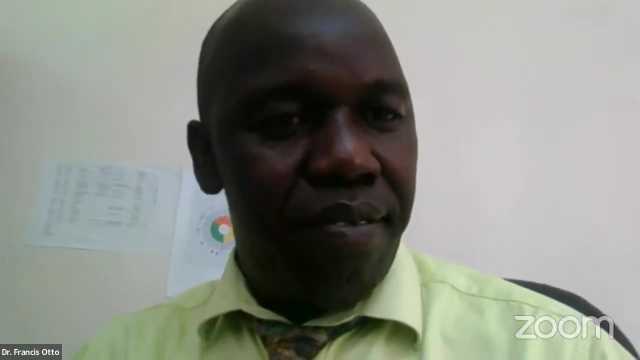 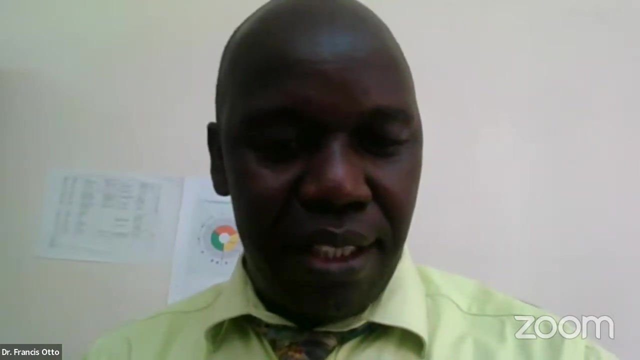 experts within this statistical data analysis. Then we have another colleague of mine. This is David Martin-Amito, who will be providing technical support to the platform to ensure that there is effective interaction between the trainers and you, the participants. So what I would like to say, 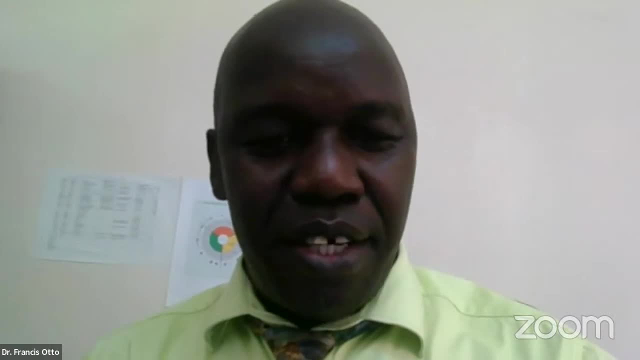 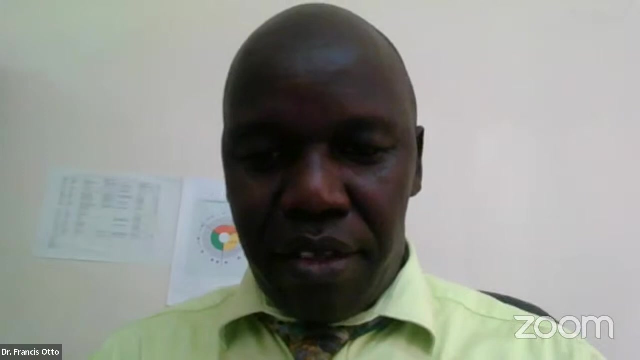 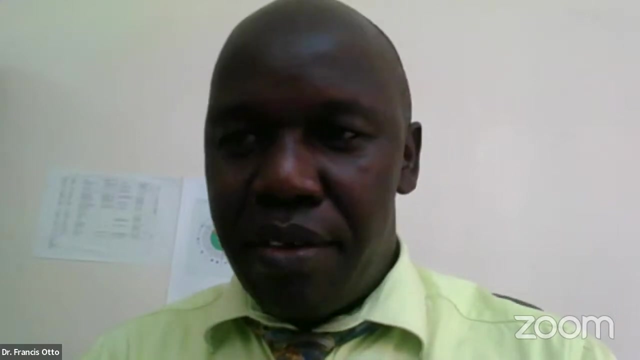 in the form of welcome is that this is a very important training, which is aimed at building your capacity as our upcoming scientists and particularly for you to be able to understand the biomedical components of research, particularly when it comes to the design and implementation of research. 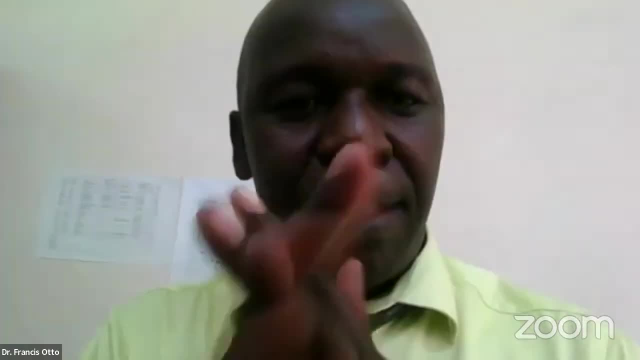 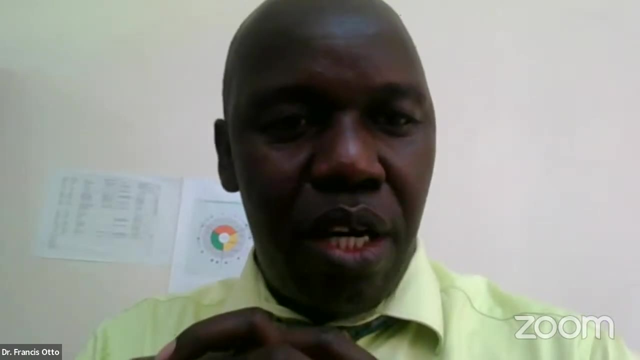 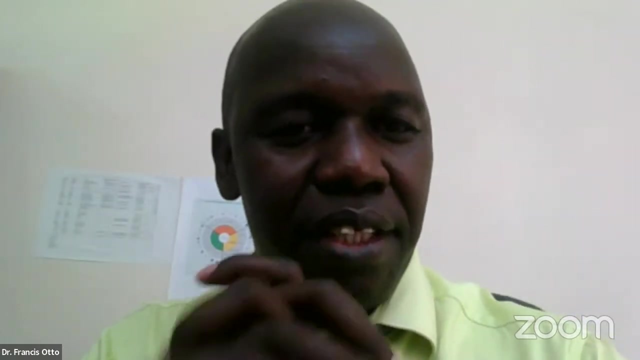 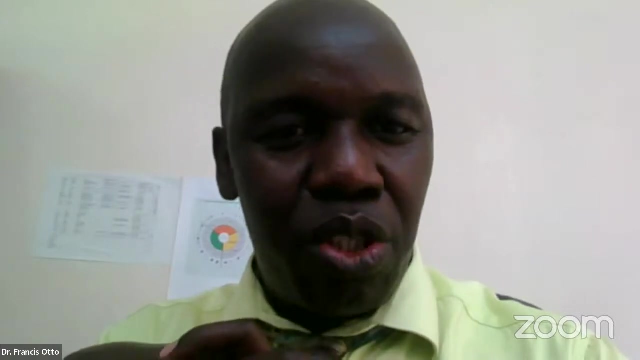 particularly also for those who are interested in quantitative methods. So you do understand that in your study you cannot graduate before you deliver a thesis and a thesis will be nothing if you cannot show evidence and finding, And what source you are finding is significant. 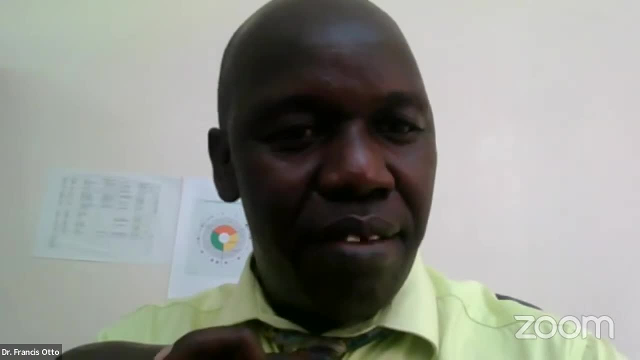 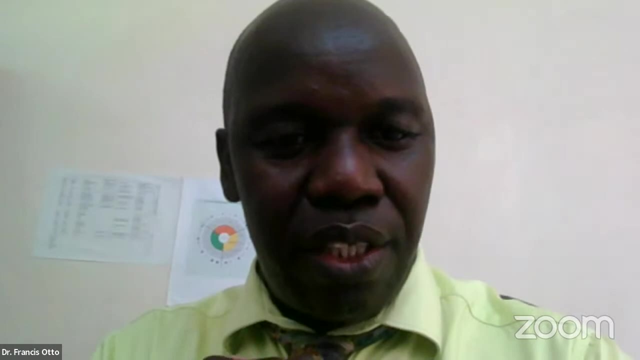 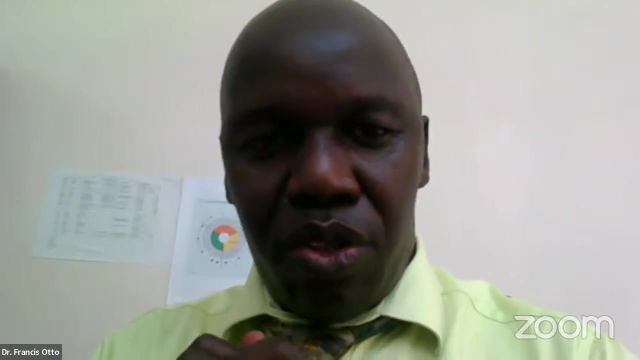 is when you produce a right information, and that right information is got after analyzing the data. So this is a good skill for you: to be able to get your data, manipulate them and be able to produce research. So Roo Forum as a network. 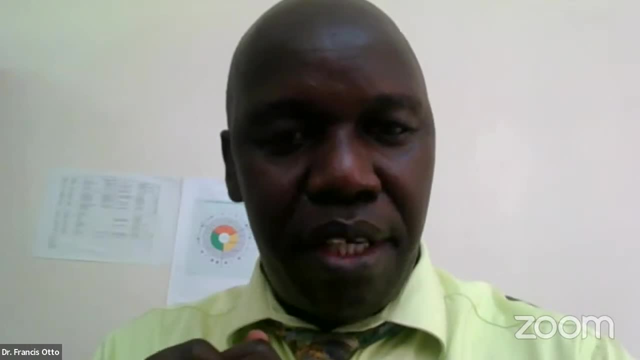 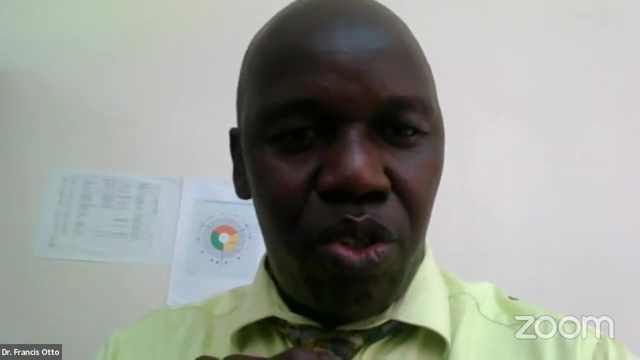 is interested in building capacity of staff, students and those who are involved in capacity and development, especially in the area of agriculture and related sciences, to be able to produce good and usable research to propel the development of the continent. So we always support our universities to be able. 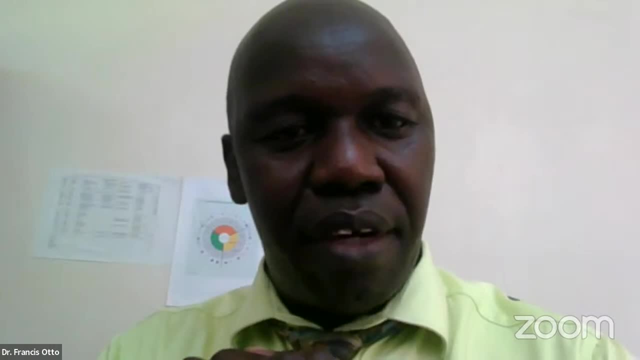 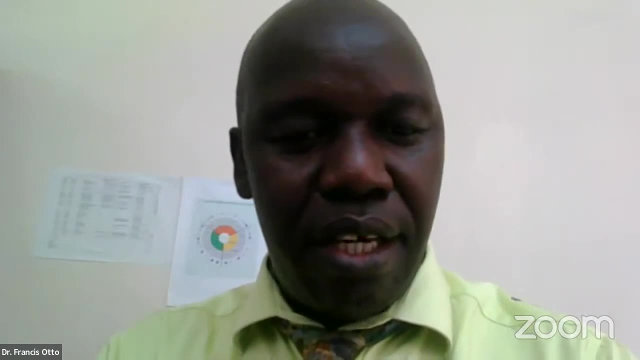 to do research and connect to the community, for us to make a contribution towards agricultural transformation in Africa. So we have been running this sort of skill training and a number of trainings have already taken place and some of you may be attending this training. 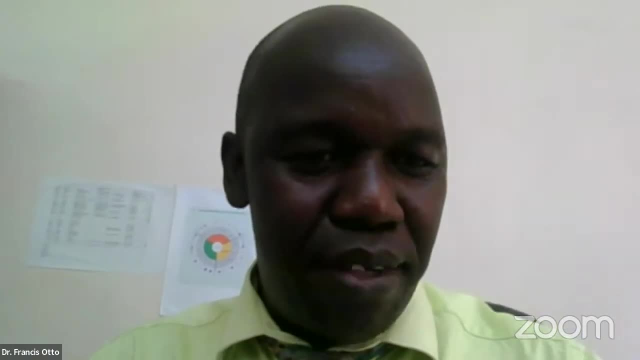 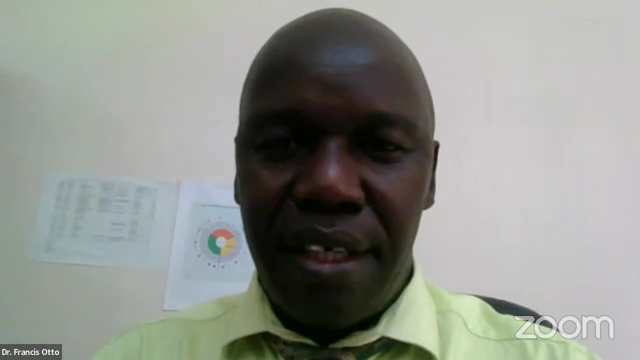 not for the first time, But if this is your first time, please do know that we do occasionally- I mean regularly- provide trainings like this, and not only in research methods, but also in other areas, including project planning and integration, and 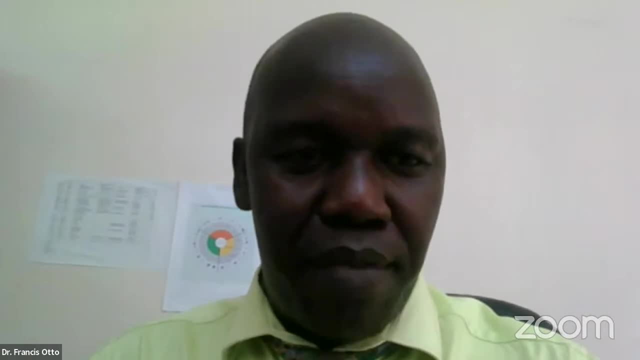 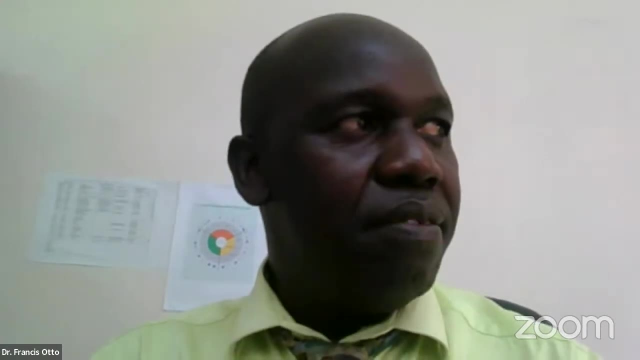 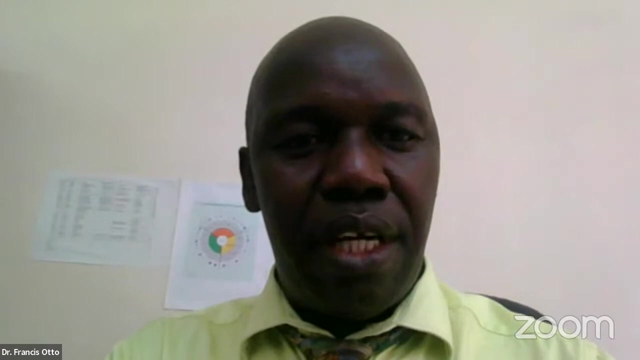 others, So you will always check our website to see what is coming up Without wasting a lot of time. I say on behalf of Professor Dipala Ekpomo, who is the Executive Secretary, that you are most welcome to the training and that you should take this opportunity to ensure that. 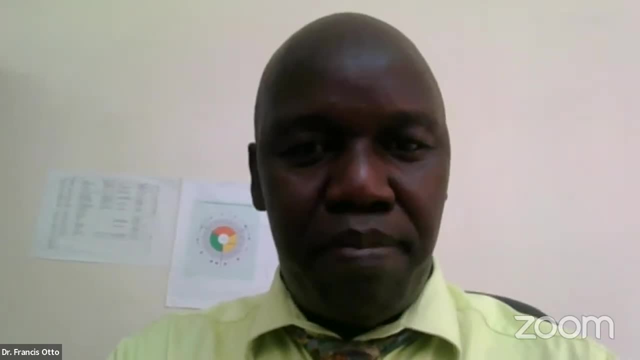 your skill gap is well covered- and participate. This is online training, but your participation is very important. They will tell you what to do in order to be able to make a contribution or to engage. So my name is Francis Soto and I work here at the 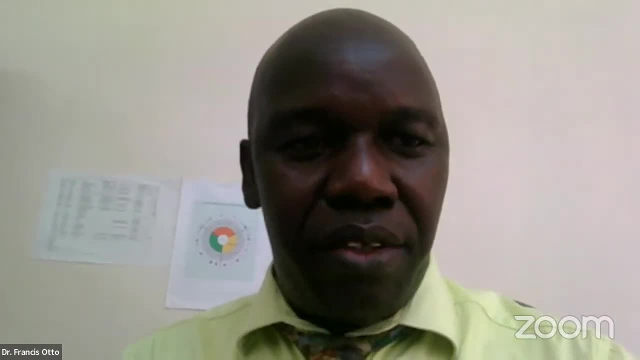 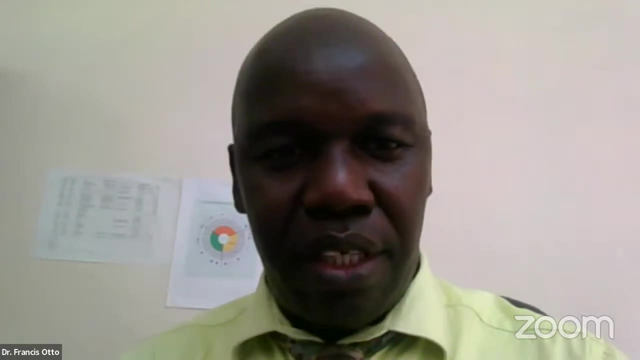 Forum Secretariat, as Manager of Knowledge Hub, Together with my colleague David Martin-Amito. we will be supporting you in terms of technical issues that may arise. So, before I call upon the trainers, may I invite my colleague David Martin-Amito to give you a few? 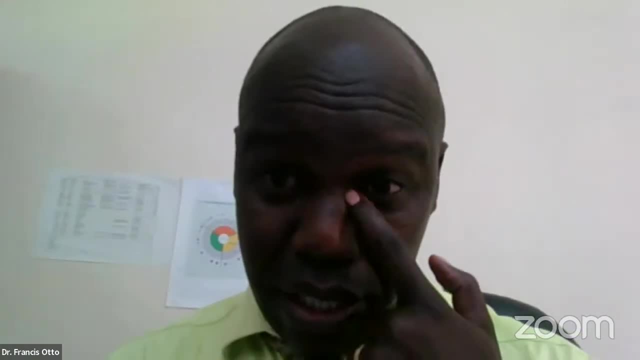 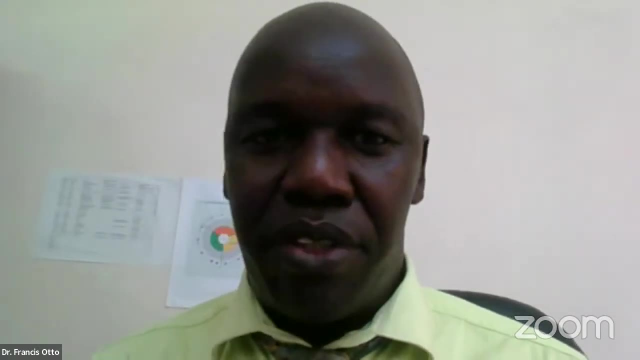 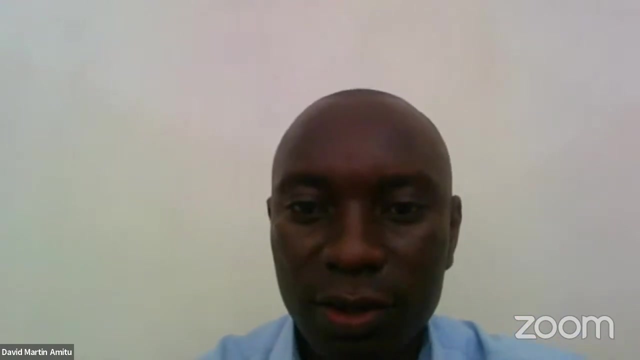 points to consider in terms of technical issues regarding the platform that we are using. David Martin-Amito. Thank you very much, Francis. So, basically, most of you have actually used the platform before, So this is just a reminder, maybe for the new people who have not used the platform before. 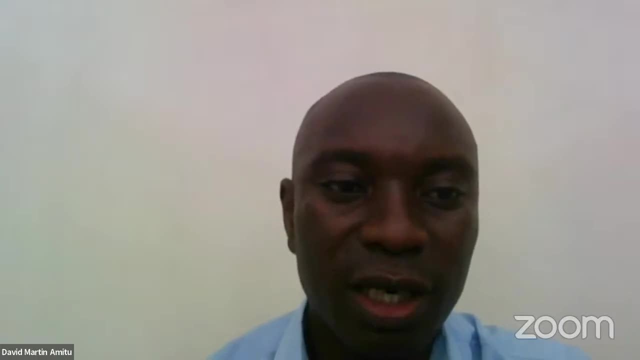 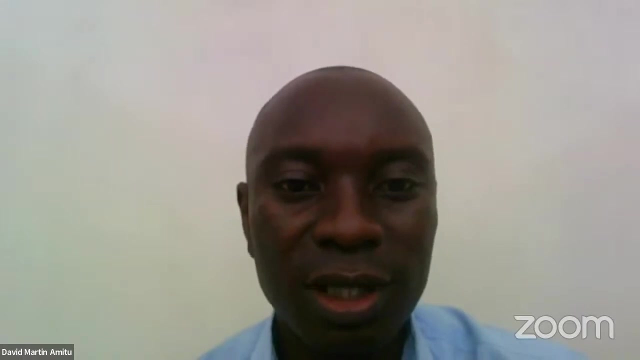 As usual, when you have an issue or a question to raise, you should be able to see the Q&A section in your screen right now. So we encourage you to raise questions through that Q&A section And then, if you have a comment. 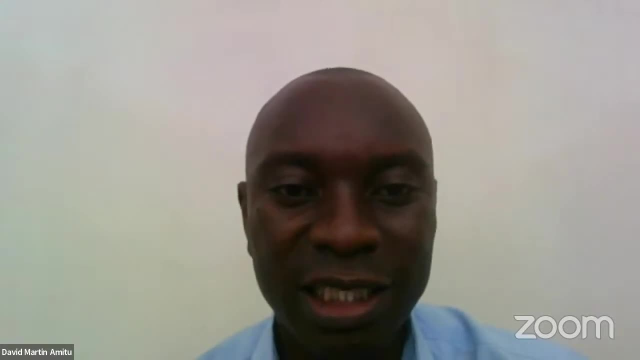 you just put the comment under the chat so that it's easy to ask questions clearly, because usually the chat section is overwhelmed and it will be difficult to trace your question if you put it in the chat section. So we encourage you to use the Q&A And then also 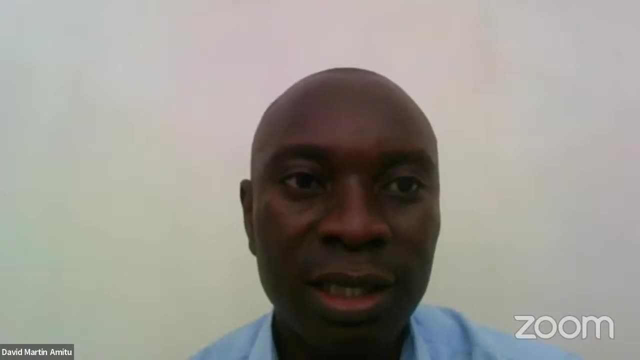 there are cases whereby the analysts or the instructors want you to participate, maybe at the start of the session. Usually, what we do is that the instructor will ask you to raise your hand. After you have raised your hand, then we allow you to talk, to respond to the question And 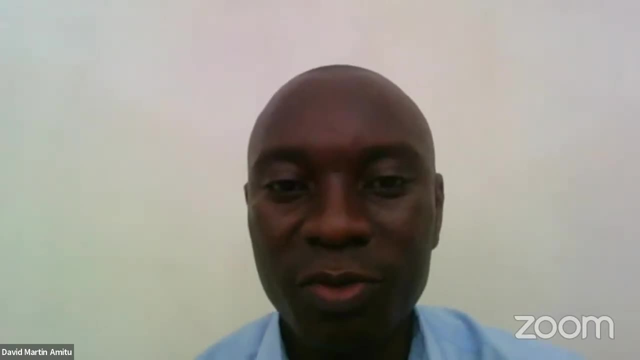 this happens usually at the start of the session. Maybe, like today's session, the instructors can give you an assignment to do And then tomorrow, when the next session starts, you might be required to present. In that case, we shall enable you to present, And then also. 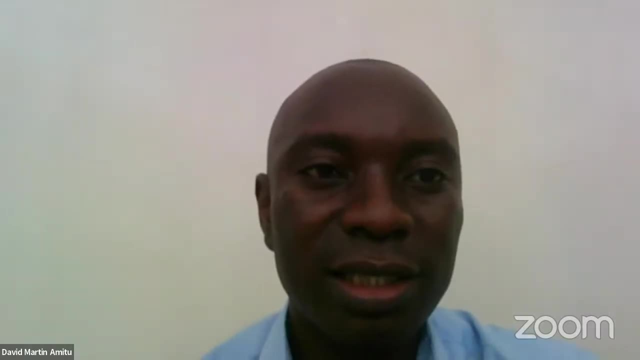 another thing you should note is that this is being live streamed on YouTube, So some of you- maybe you might encounter network problems and then you are cut off. So usually our instructors share with you also the YouTube link at the end of the day or tomorrow morning. 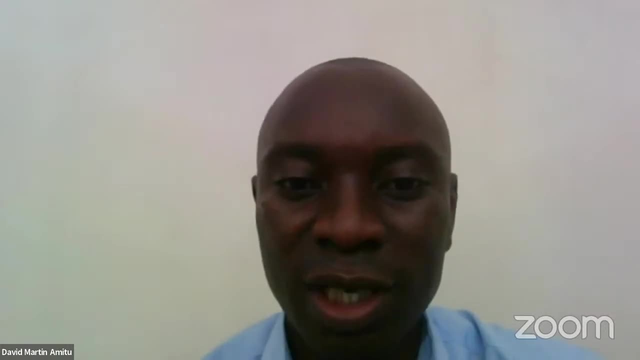 for day one, Because already we have captured this training and we shall share with you in case you miss any section. And then another thing is that, in case you are allowed to talk, make sure that after you have finished, you have to keep your mic. 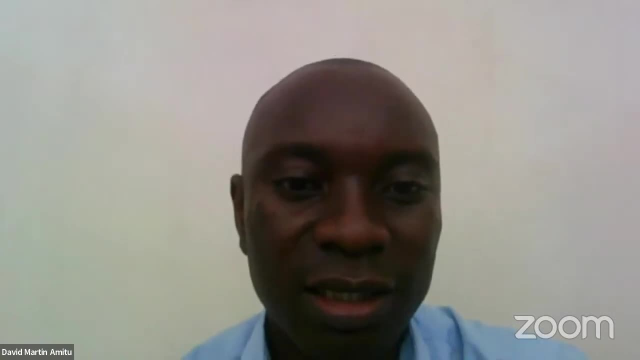 muted such that it doesn't interrupt, Because sometimes we allow some of you and then maybe when you finish you forget to mute the microphone. So usually what we do, we shall also put you back to the attendee status in order to automatically remove your mic, But there are some cases. 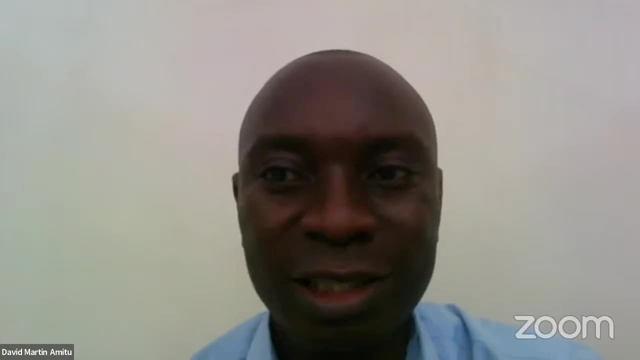 whereby we can maintain you such that maybe you can respond to the questions. So once you have finished talking, make sure that you are muted. So I think that is for now the basic information I can provide, But you shall also be following any comments in the chat section and questions. 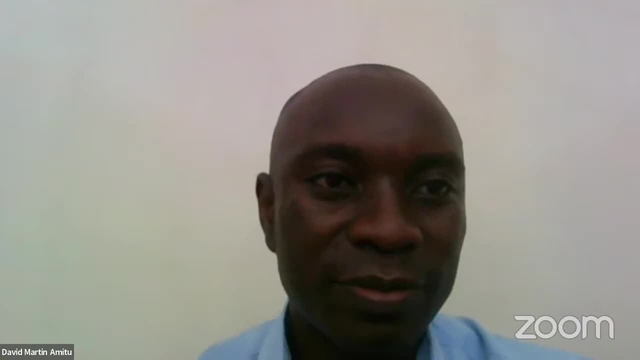 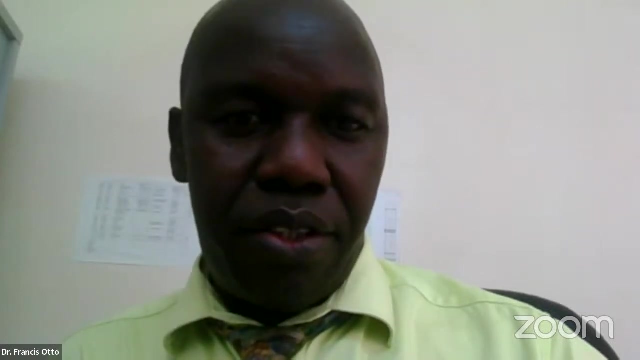 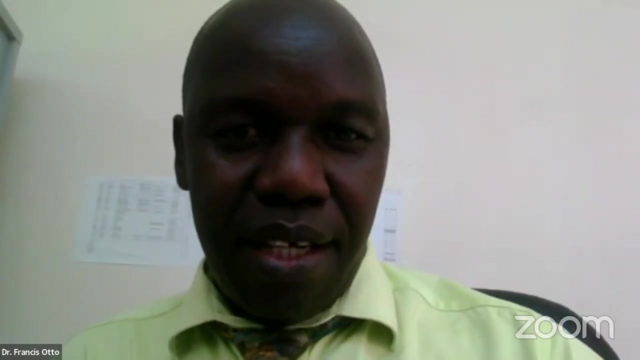 in the Q&A. Thank you very much. Thank you, David, So can I therefore hand you over to the trainers so they will take charge for this training starting now until Saturday. So you're welcome, Professor Susan Balaba, you may want to take the lead. 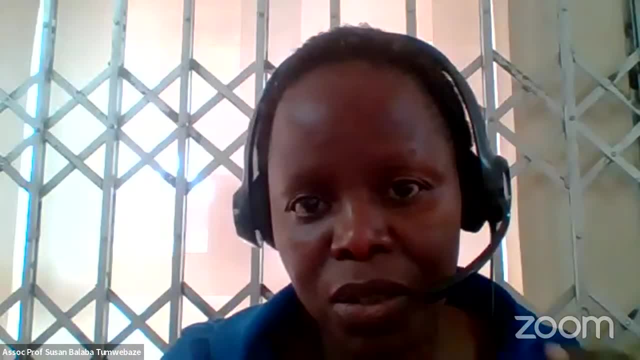 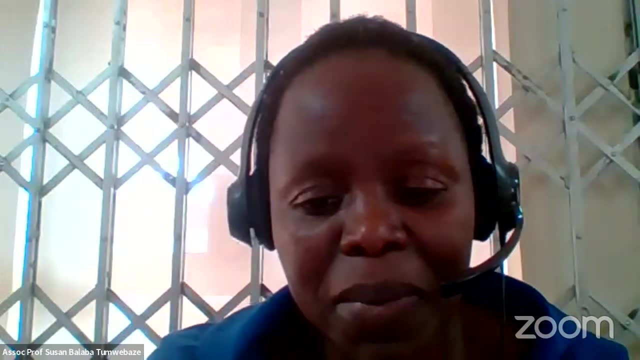 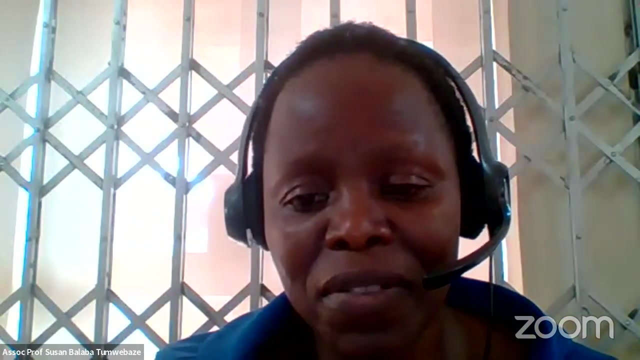 Thank you very much, Dr Francis. Good morning participants. I'm Susan Balaba Tumwebazi from Forestry School of Forestry, And I'm going to take you through the five days. I take this opportunity to thank you for. 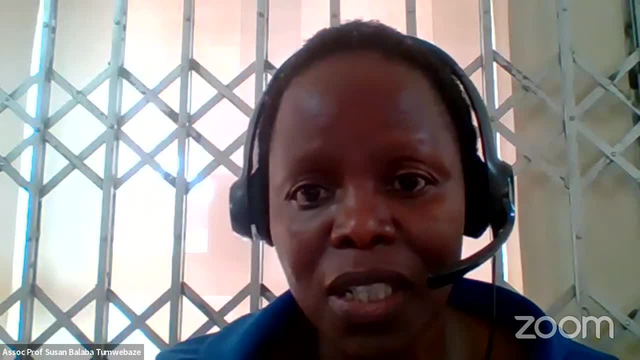 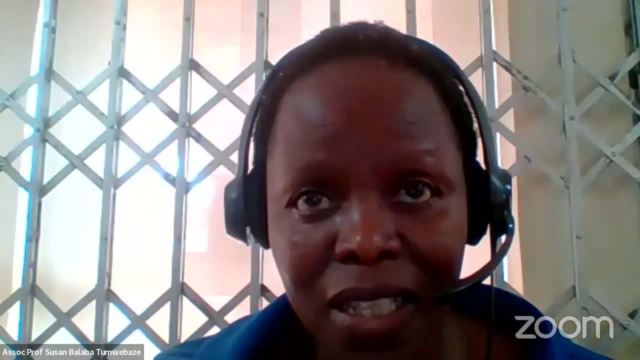 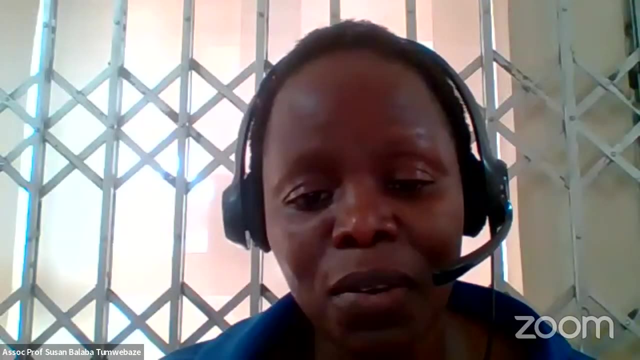 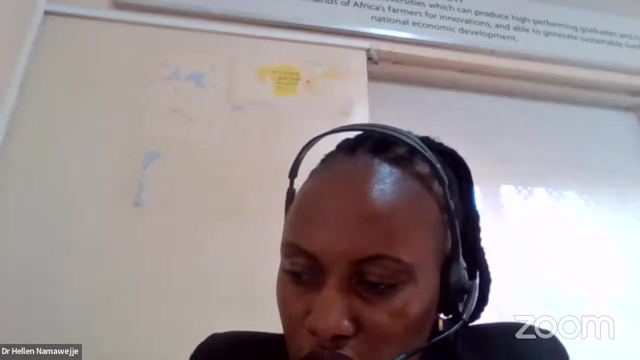 registering for the course. I also take this opportunity to thank the forum for funding and organizing the training. I also take the opportunity to thank all the universities for allowing you to be in this training. The training is important because if you don't know statistics, you can't write your thesis. 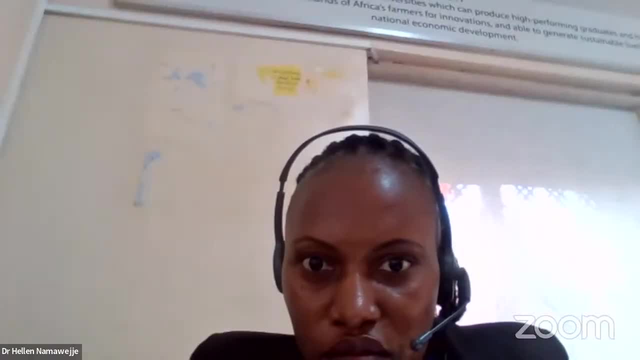 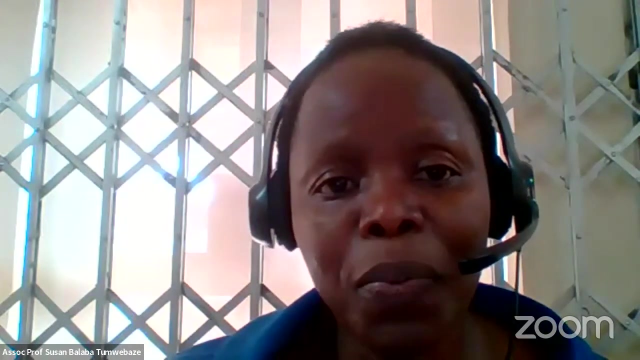 So the more you know how to analyze your data, the shorter the time you take to complete your thesis. So this is a great opportunity which you need to take into account. I also take the opportunity to thank my co-facilitators for joining us. 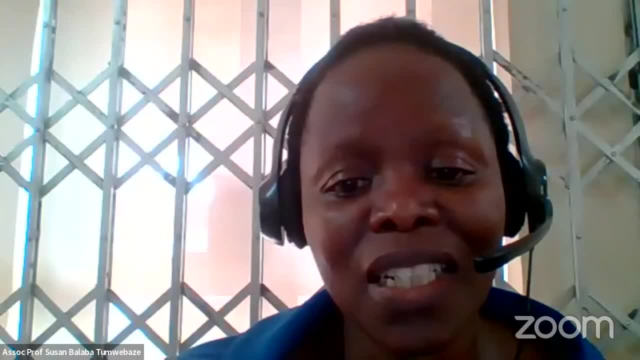 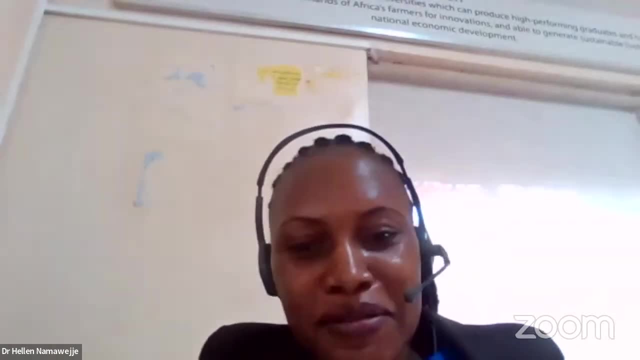 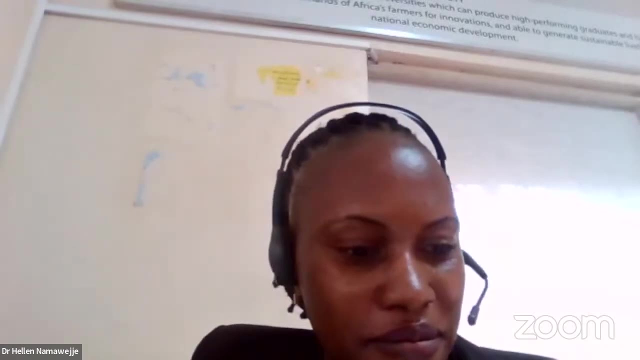 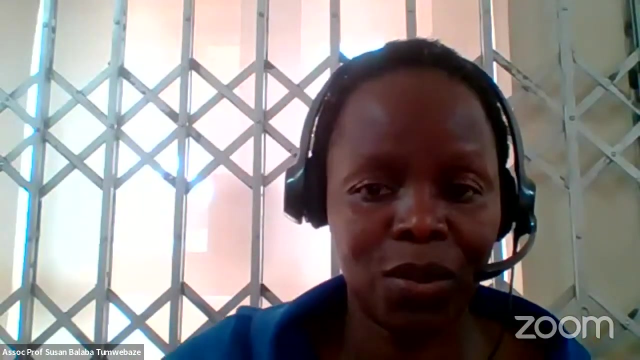 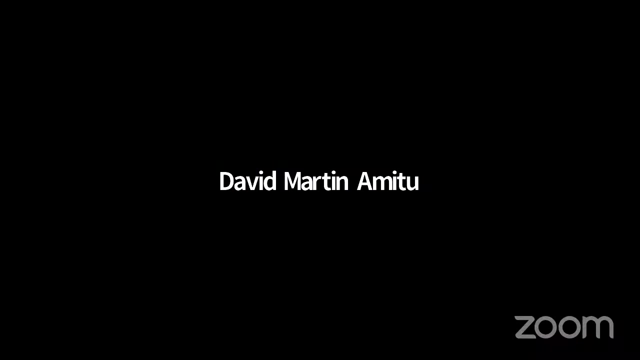 And I hand over to Dr Helen to introduce herself. Okay, Good morning everyone. Can you hear me? There is an echo. Yes, we are hearing you clearly. Can you hear me now? Okay, Yes, They're saying yes. 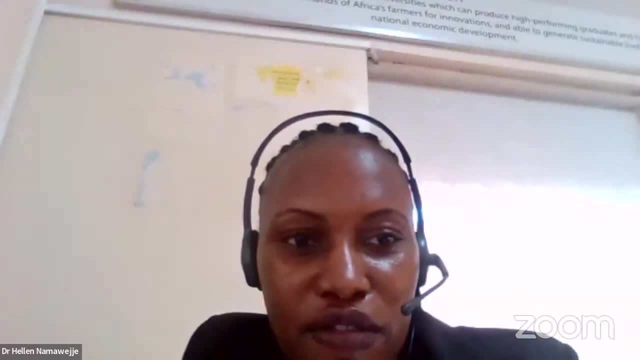 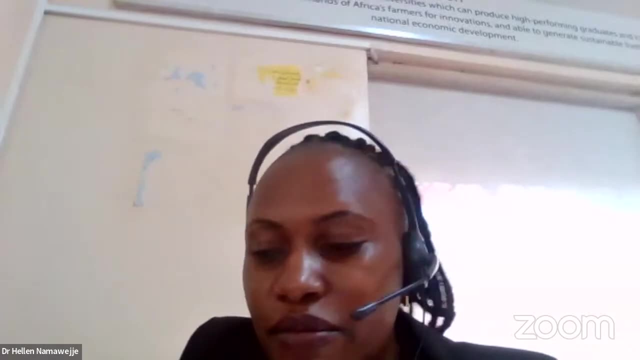 Okay, A very good morning. I'm Dr Helen. I'm a lecturer at Macquarie University in the Department of Statistical Methods and Actuarial Science, in the School of Statistics and Planning. I'm so glad that I'm going to be among the facilitators. 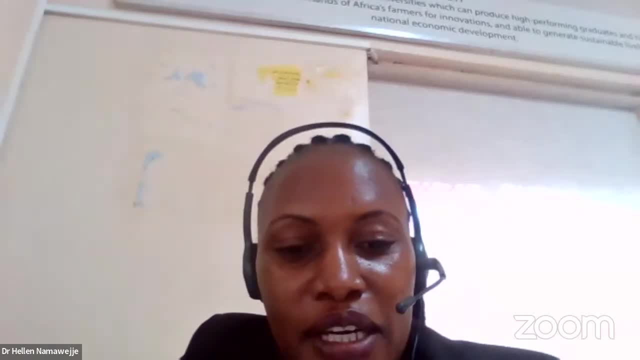 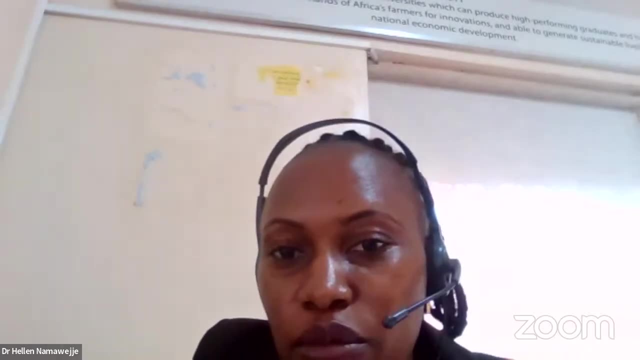 in the week's training. I welcome you all. I pray that by the time the week ends you have achieved the expectations. I hope that you will find some time to log in and see how you can really get supported as you're building your career. 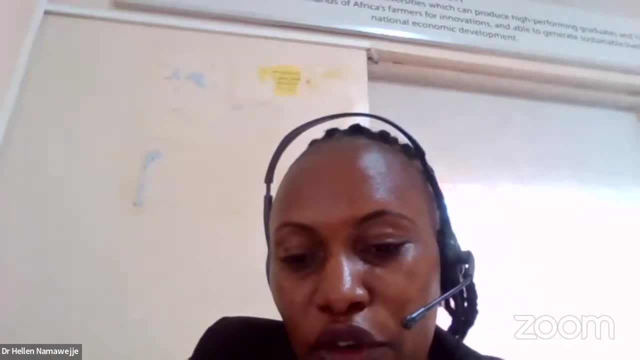 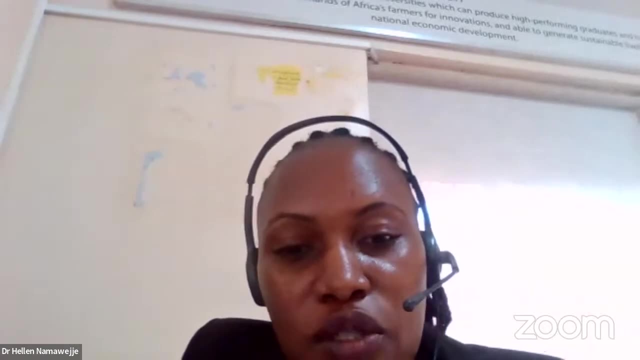 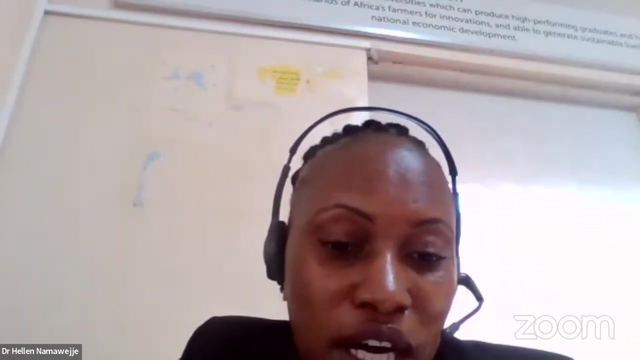 Like my senior said, I also thank Roo Forum for giving us this opportunity to train again, And also my other colleagues who are on the same panel. Best wishes. I encourage you to participate and, where you can, please ask many questions. Ask as many questions as you can. 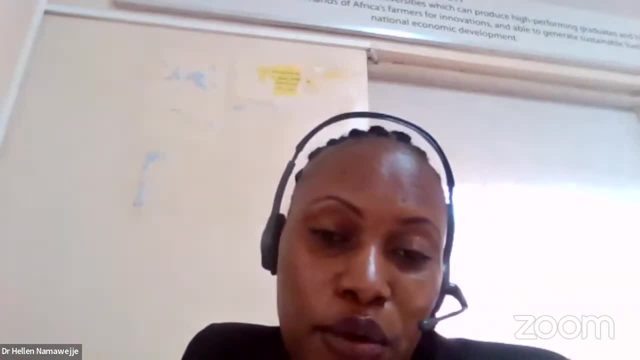 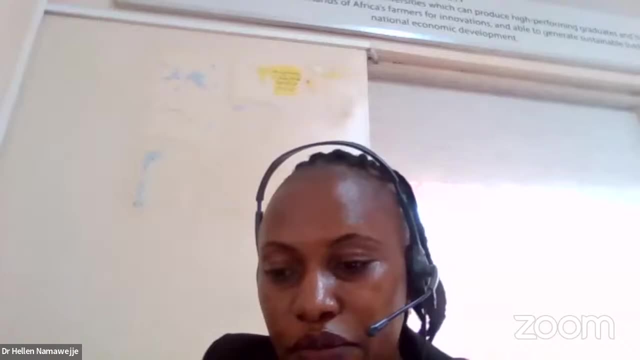 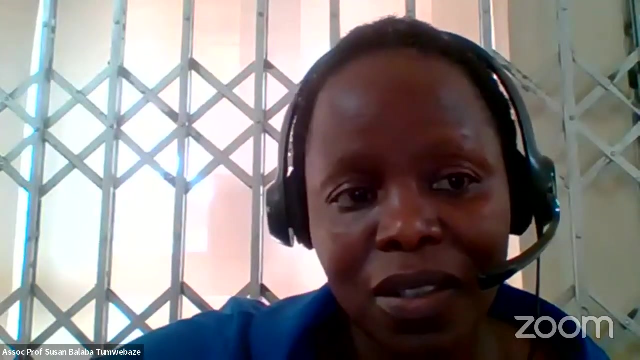 So that by the time you finish the training, you have a right roadmap for how you're going to do your analysis. Thank you so much, and you're very much welcome, Dr Thomas. Dr Thomas, can you introduce yourself? Thank you. 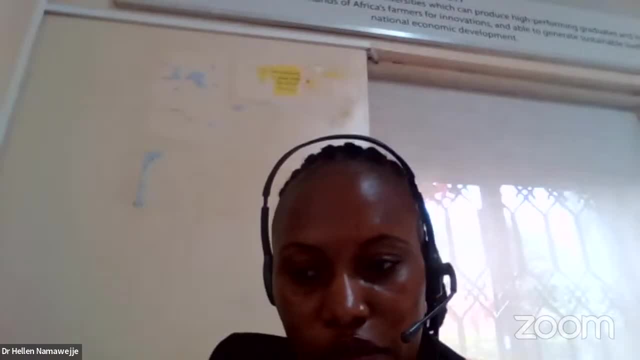 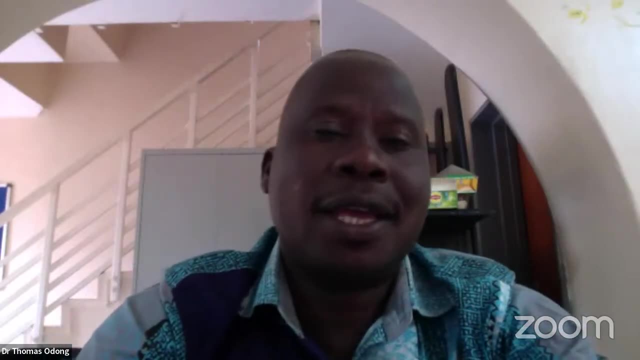 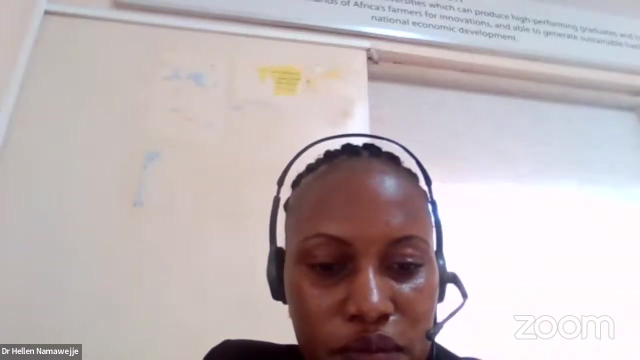 Hello, good morning everyone. I'm called Thomas Odom. I also work at Macquarie University in the College of Cultural and Environmental Sciences. I'd like to welcome you to this training and expect to have a profound discussion and interaction with you. 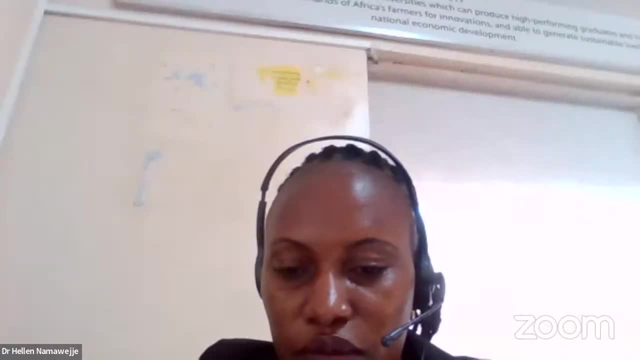 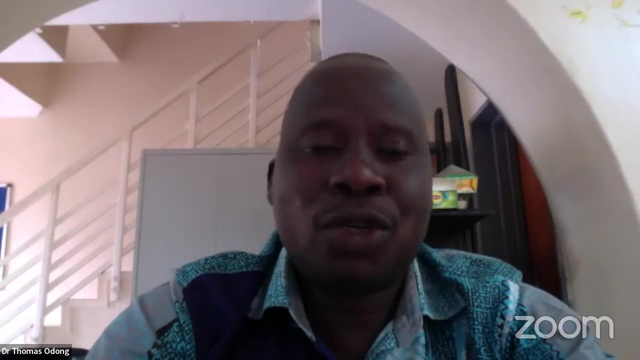 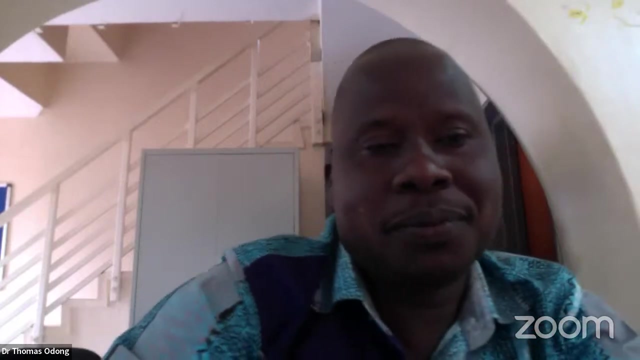 throughout the week. I'd also like to thank Roo Forum for giving us this opportunity to share the little knowledge we have and also to learn from you. I wish you all the best and please pay attention and try to benefit as much as possible. Thank you. 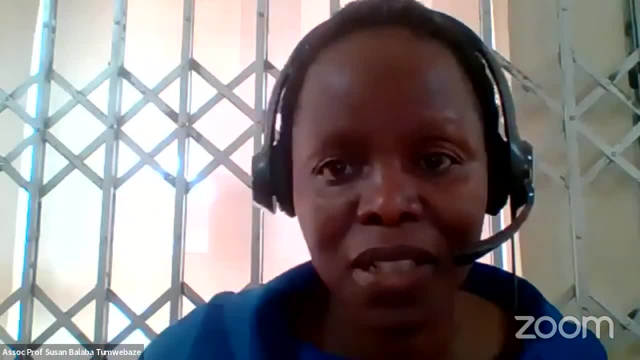 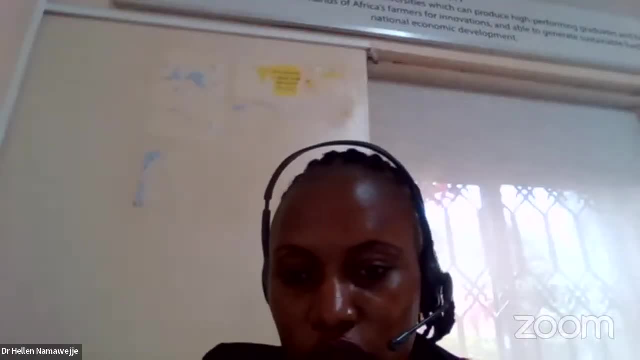 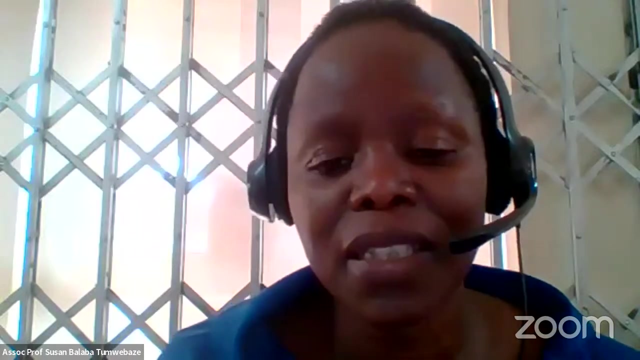 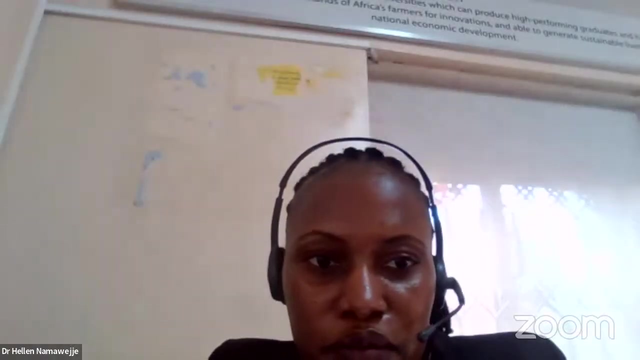 Okay, Thank you very much, facilitators. We are now going to start with an overview of the training. We are going to start with an overview of the training. We will also present results from the training needs assessment tool and afterwards I will hand over. 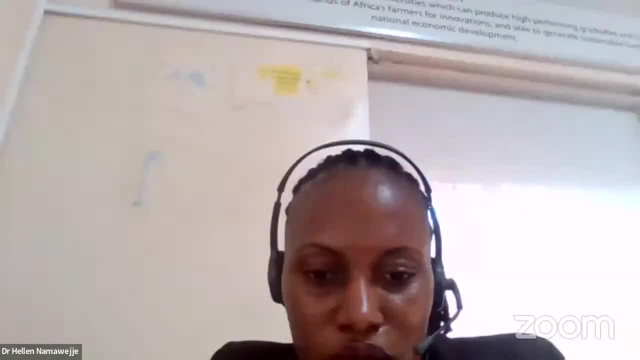 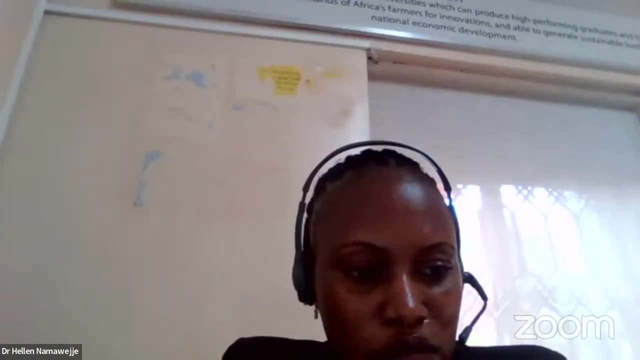 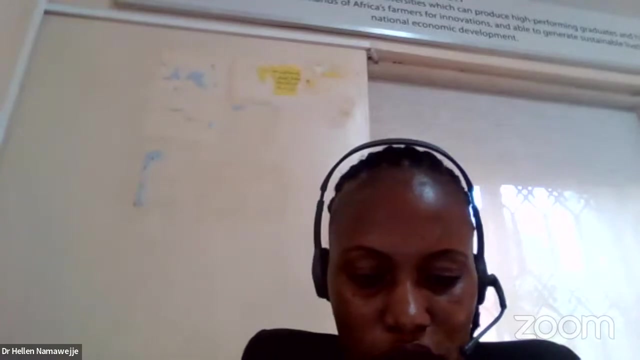 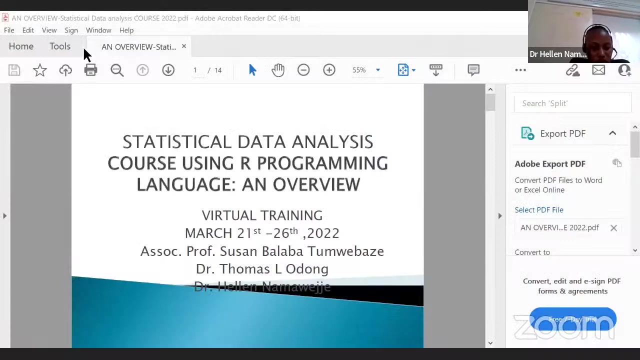 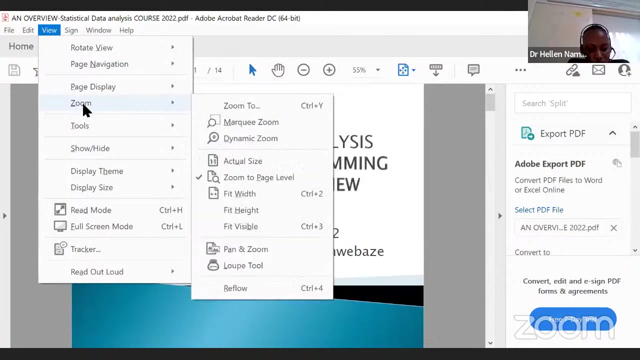 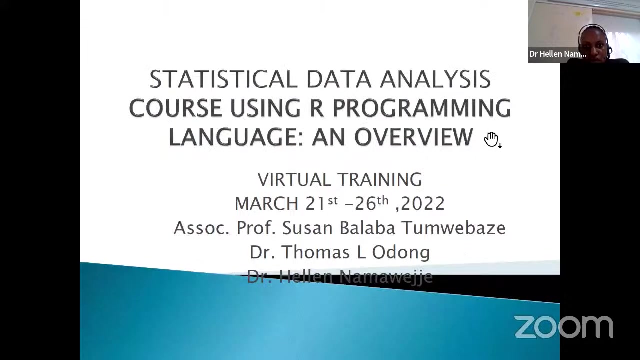 to Dr Helen to start with our overview of the training. So let me share the overview of the training. Okay, So the training is called statistical data analysis. Can you hear me? Yes, Yes, Okay, Thank you. The training is called statistical data analysis. 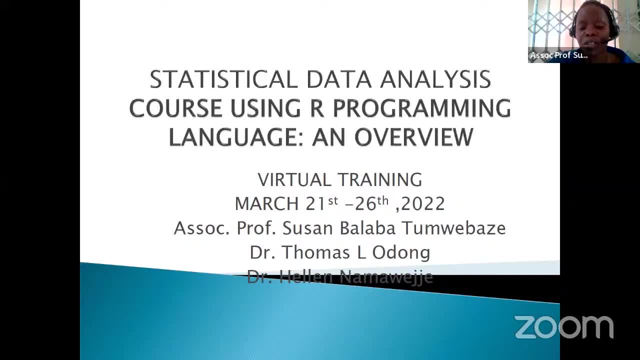 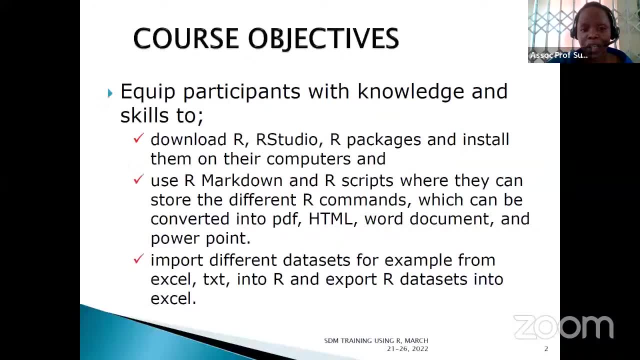 and before we train normally we send out training needs assessment That helps us to modify the training. The course objectives for this training are to equip participants with the knowledge and skills to download R R, studio R packages and install them on their computers and use R markdown. 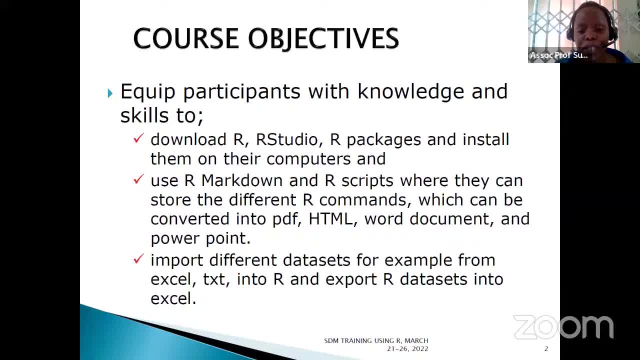 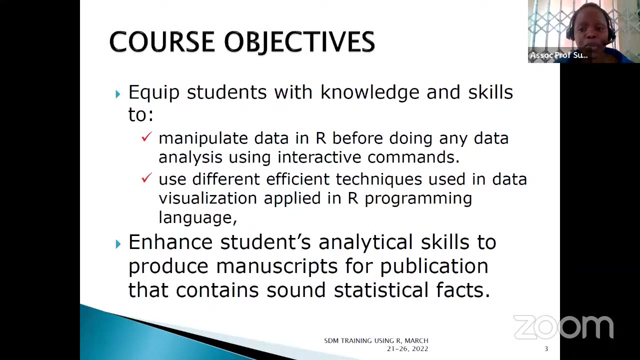 and R script where they can store the different R commands, which can be converted into PDF Word document, which can be imported into Excel and then export different data sets, for example from Excel text into R and export R data sets into Excel or other software. 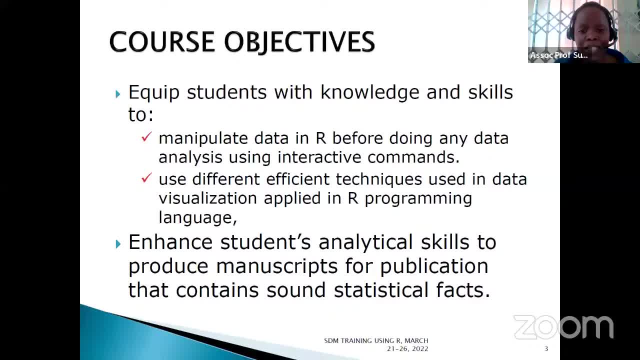 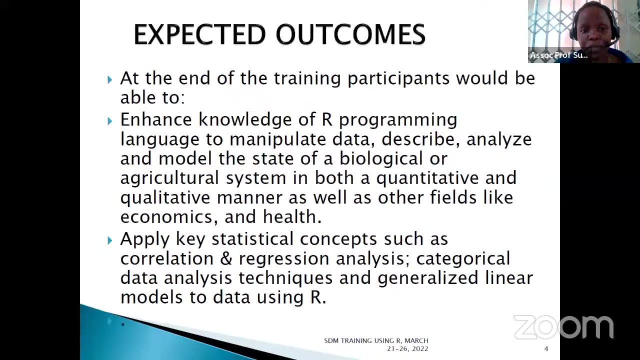 To keep the participants with skills and knowledge to manipulate data in R before doing any other data analysis using interactive commands programming enhance the students and lecturers analytical skills to produce manuscripts for publication that contain sound statistical facts. And then we also have expectations for this. 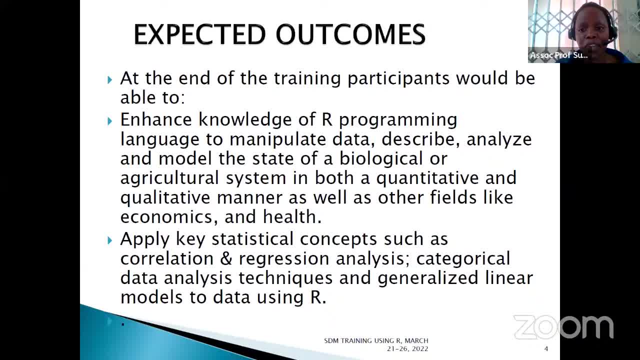 course. We assume that at the end of the training, participants will be able to enhance knowledge of R programming to manipulate data, describe, analyze and model the state of a biological or agricultural system in both quantitative and qualitative manner, as well as other fields like economics and 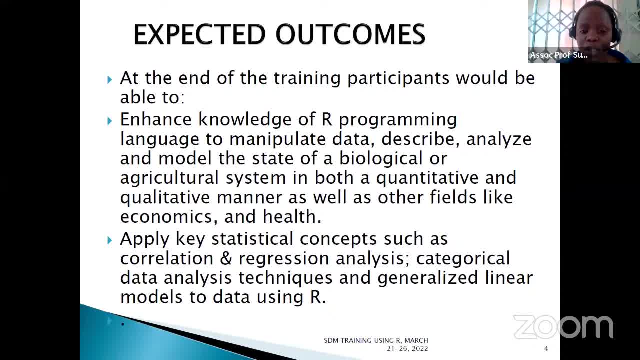 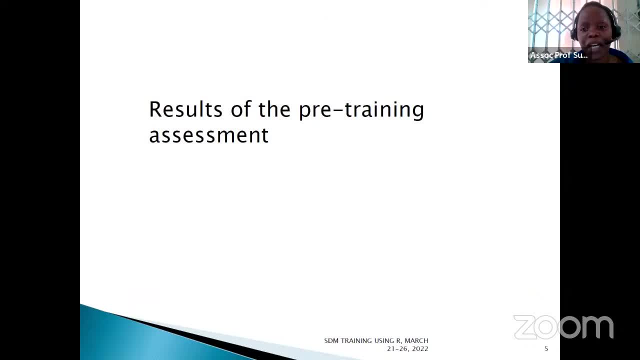 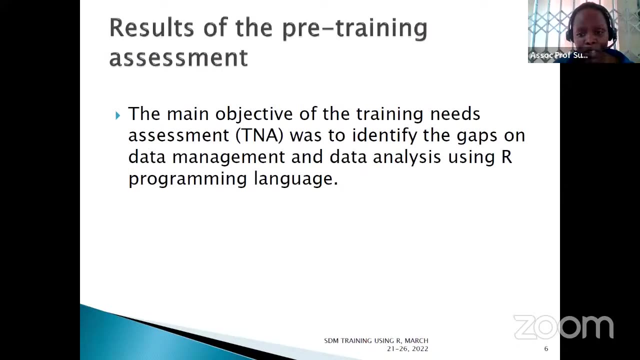 health. apply key statistical concepts such as correlation, regression analysis, categorical data analysis, generalize linear models using R. Then the results for the pre-training assessment include the main objective of the three needs assessment was to identify the gaps on data management and data analysis using R. 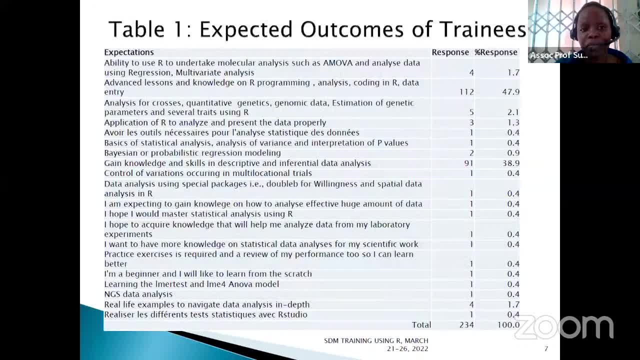 programming language. We captured the expectation. this is an open-ended question and I have summarized output from around 158 comments, So I have over-summarized them. So in case I don't present them the way you presented them, they are within the results that. 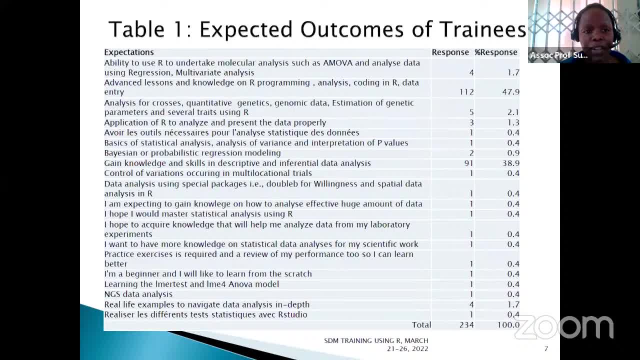 you see in the output. So the first expectation was ability to use R to undertake molecular analysis such as AMOVA, and analysis analyze data using regression multivariate. Then the next one is advanced lessons and knowledge on R programming, analysis, coding in R and data entry. 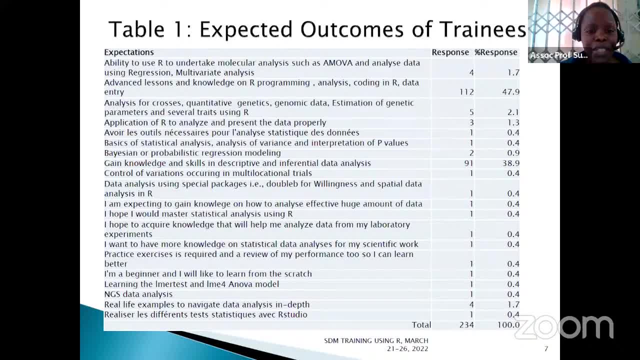 Analysis for crosses, quantitative genetics, genome, estimation of genetic parameters and several traits using R: Application of R to analyze and present data properly. This other expectation is in French, so maybe one of the French speaking will help me. The next one is basics of statistical 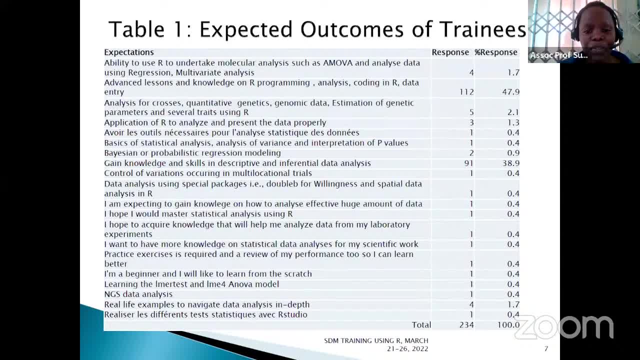 analysis: analysis of variance and interpretation of p values. The next one is Bayesian or probabilistic regression modeling. The next one is to gain knowledge and skills in descriptive and inferential data analysis. The next one is control of variation occurring in mouse location trials. 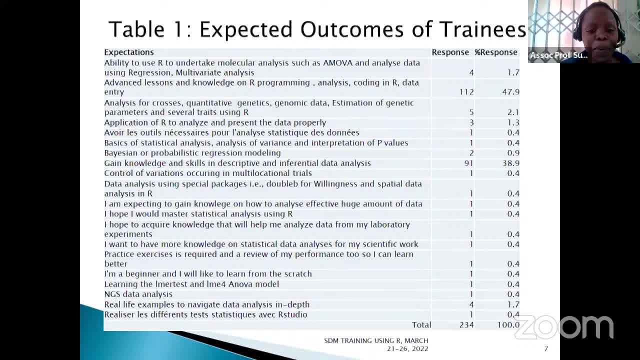 The next one is data analysis using spatial packages for willingness and spatial data analysis in R. The next one is to gain knowledge on how to analyze effective huge amount of data. The next one is that they hope that they will master statistical skills using R. 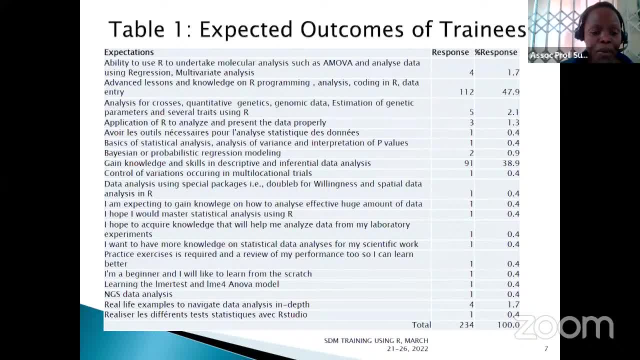 The next one is that they will acquire knowledge that will help them analyze data from laboratory experiments. The other expectation is they want to know more on statistical data analysis for scientific work. The other expectation is practice. They need more practical exercises, or practice exercise is required. 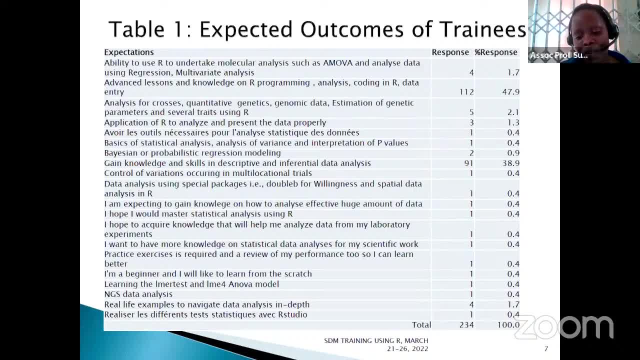 under review of their performance analysis. Then this one in particular, I didn't merge. it says I am a beginner and I would like to learn more from scratch. Then this expectation wants to learn about IMA test and IMA ANOVA model. This expectation, which seems 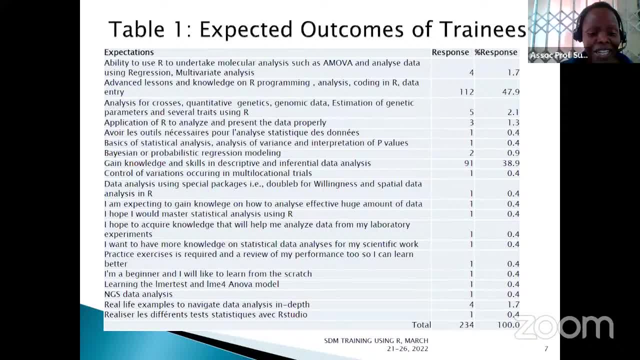 to be outside. R is NGS data analysis. I think this should be national geographical data analysis, Next generation sequencing. that is interesting. I've been told that it's next generation sequencing data analysis. I had misinterpreted it. The next expectation is real life. 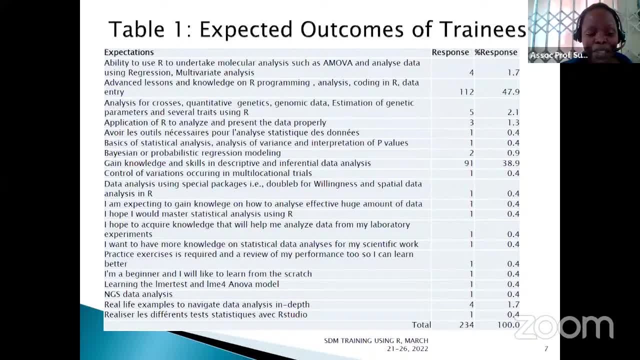 examples to navigate data analysis in depth. The last one is also in French. I don't know whether my colleagues Thomas and Helen know French. If they don't know, so we'll have one of the forum staff to interpret this French part of it. 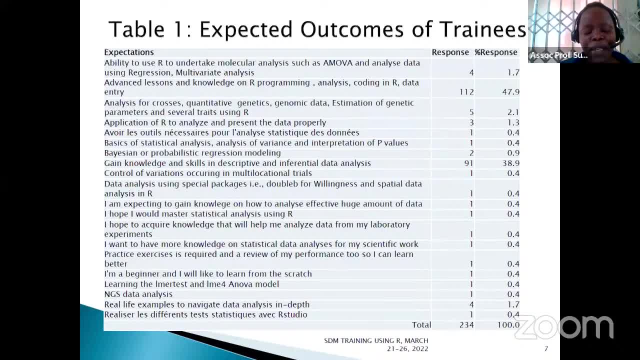 Otherwise, most of these expectations have been captured in what we are going to cover. Just like he said, he's a beginner and would like to learn from scratch and from also other expectation: we see that people would like actually to learn about how to use R to manipulate their data. 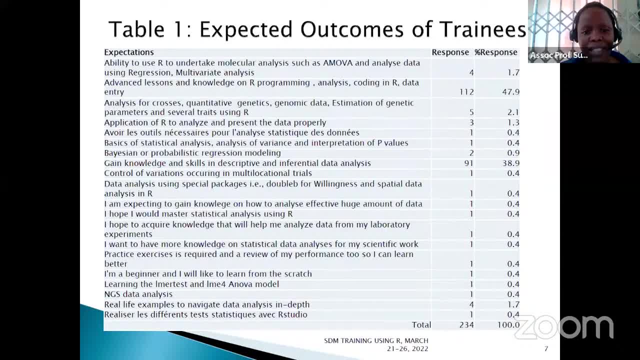 enter data and also do advanced statistical analysis. So all these expectations depend on time and also depend on how much participants will absorb at a time. So if the participants absorb the information we are passing on very fast, then we cover more. But if the participants are a bit, 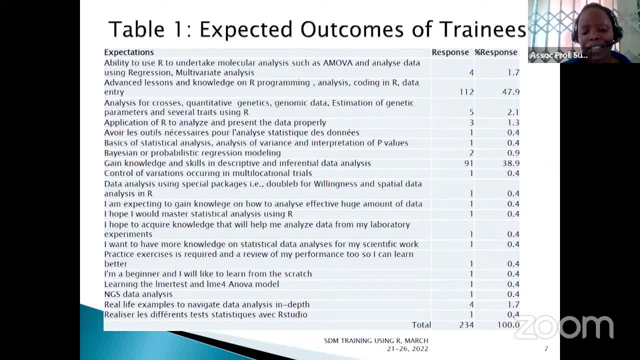 slow. we cannot really cover a lot of things just because we want to finish, So we will go slow by slow, making sure we don't leave anybody behind, but also making sure others are gaining from the R training. Okay, And to note the commonest, 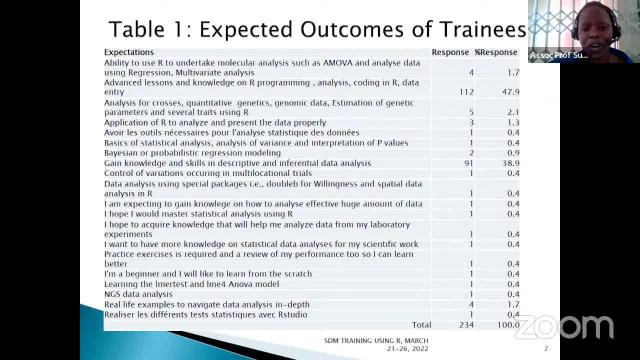 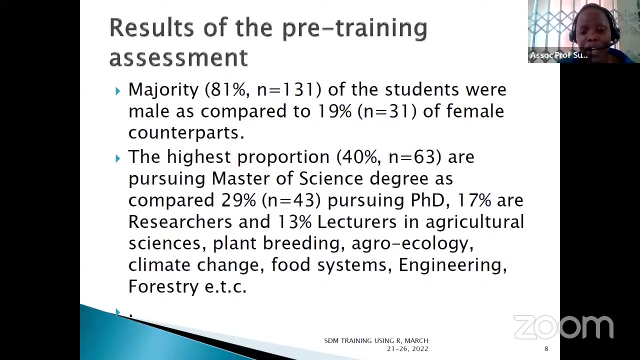 expectation was advanced lessons and knowledge on R analysis in R and data entry, and also there is gain knowledge and skills in descriptive and inferential statistics. So those were the common expectations among the participants. Now, overall we had around 162 responses out of the 1000 that 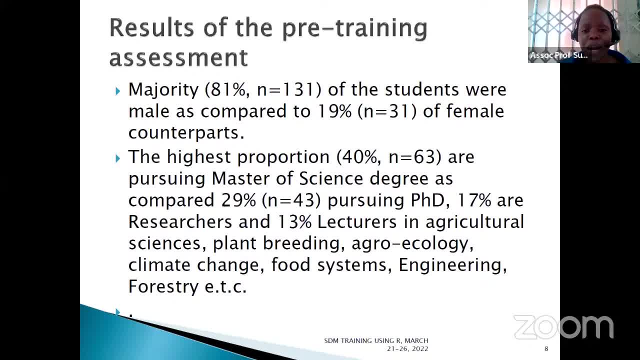 registered and majority were male, with 81 percent, and the female were 19 percent. The highest proportion- 40 percent- are pursuing MSC lesson masters and then 29 percent are pursuing PhD, 17 percent are researchers, while 13 percent are lecturers in various fields. 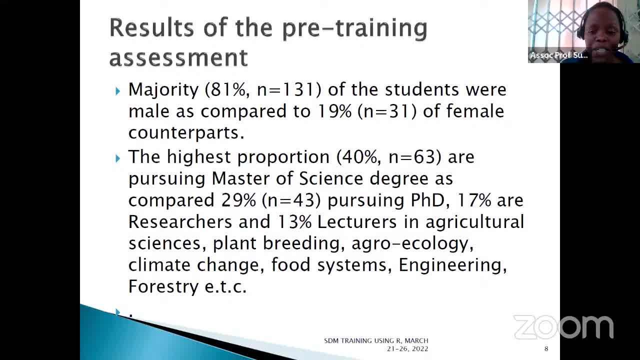 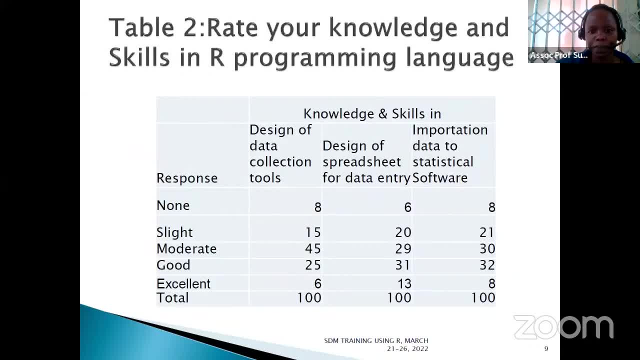 which include agriculture, plant breeding, agroecology, climate, food science, engineering, forestry, etc. We also had a question to find out the knowledge and skills in various components of statistics. One of these components are design of data collection tools, then design of 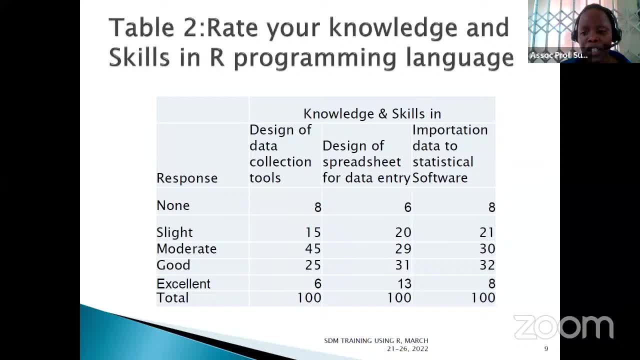 spreadsheets for data entry, importation of data to statistical software. So overall, we find that most of the participants had moderate knowledge in design of data collection, design of spreadsheets for data entry and also importation of data for statistical software according to the percentages. 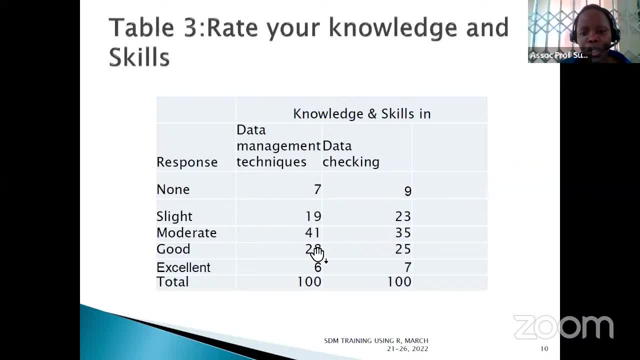 Then we also wanted to know knowledge and skills in data management and data checking. That is, after you've designed the spreadsheet, you've entered your data, are you able to export your data to other packages? Are you able to save and clean your data? Also check. 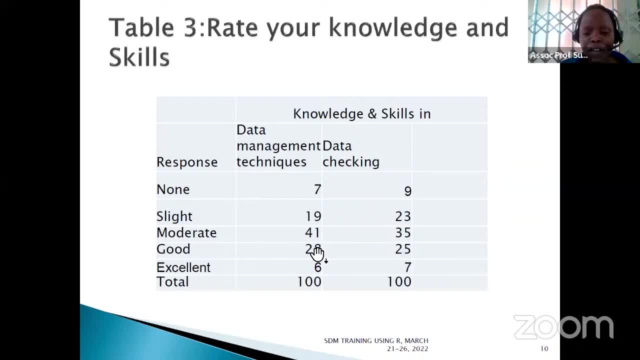 for outliers, We found that participants overall had moderate knowledge. You can see that under data management techniques we have 41 percent of the participants saying that they have moderate knowledge and also under data checking it is 35 percent. Those are the highest percentages. 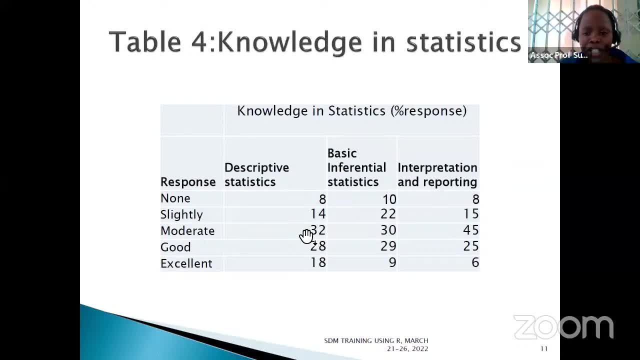 Then we needed to know knowledge in statistics, Basically descriptive statistics and basic inferential statistics, as well as interpretation and reporting. So when we look for the highest frequency or percentage response, we find that participants had moderate knowledge in descriptive statistics, in inferential statistics and as well as 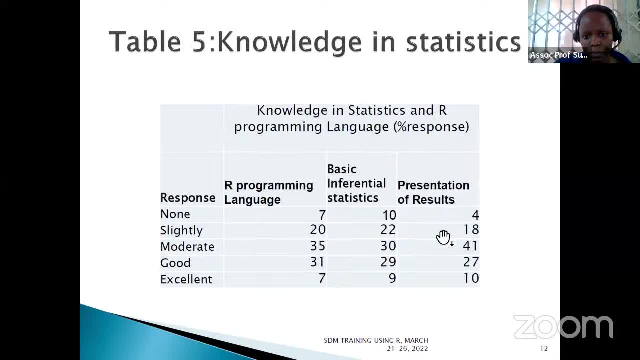 interpretation and reporting. We also wanted to know knowledge in statistics and R programming language and we found that participants had- there were few who had no knowledge in R- 70 percent, then 20 percent have a slight knowledge, while most of them had moderate and good. 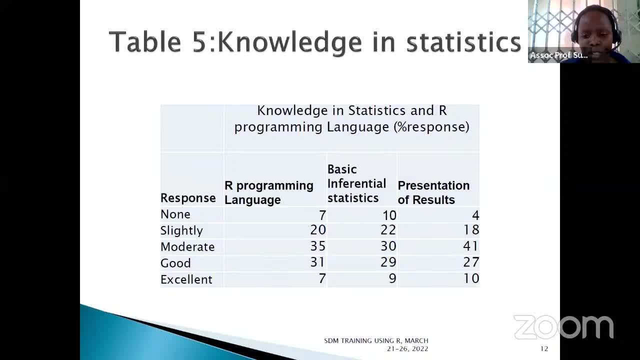 knowledge and a few are excellent, which is really good. That tells us that this time, after this training, those who have good knowledge will move into excellent, Those who have moderate will move into good knowledge. in R, Then basic inferential statistics, we find this is: 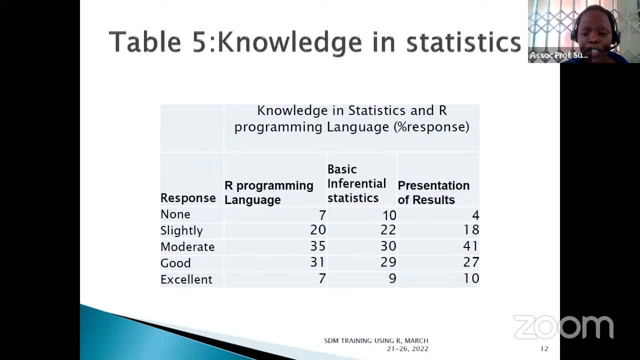 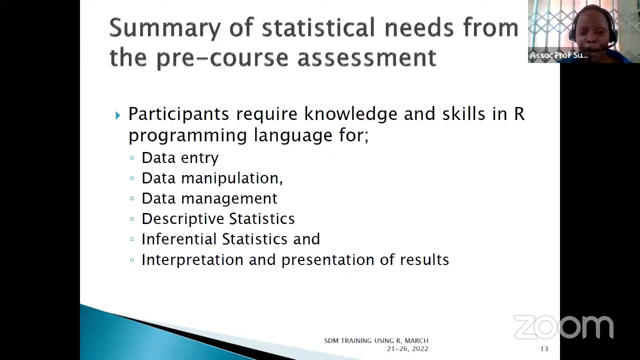 a repetition, we find that they had mostly moderate knowledge and then presentation of results after analysis. most of them have moderate knowledge in presentation of results after analysis and a few of them have none. 10 percent have excellent. Then, overall, to summarize the results: participants require knowledge. 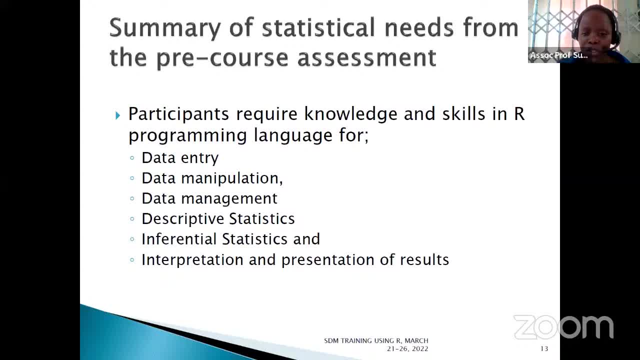 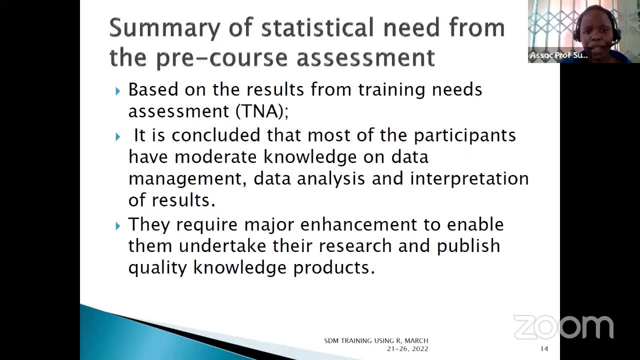 and skills in R programming language for data entry, data manipulation, data management, descriptive statistics, inferential statistics and interpretation and presentation of results. Based on the pre-course assessment, we conclude that most of the participants have moderate knowledge on data management, data analysis and interpretation of results, and they require 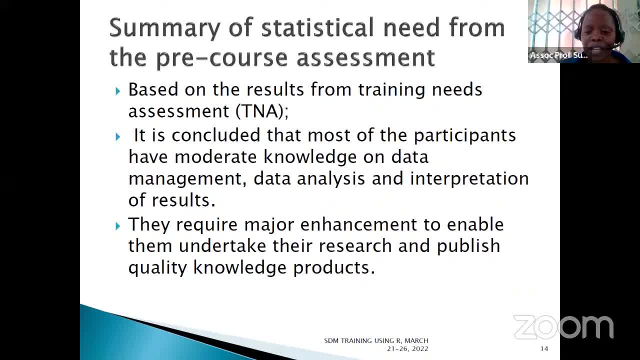 major enhancement to enable them undertake their research and publish quality knowledge products and also complete on time. So that's what we found in the training needs assessment and throughout the training we will be checking the expectation of the participants and, if time allows, make sure that we. 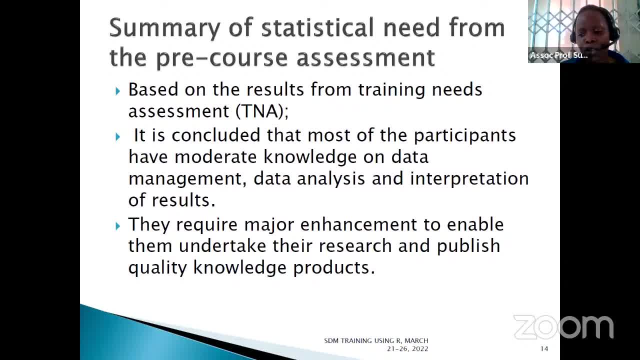 are able to meet the expectation of this course and also the participants. Thank you very much for your attention and I'm going to hand over to Dr Helen Namaweje, who is going to take you through R programming language, and if you have a question. 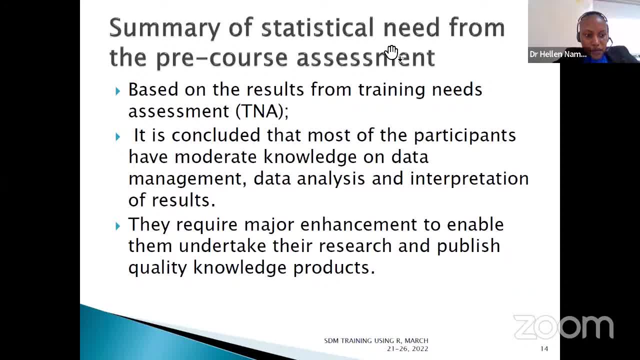 please use the Q&A and if you have a comment, use the chat. so when you use the Q&A, the questions stay longer so we are able to attend to the questions and the chat. the questions move very fast because very many people are commenting, so please utilize the Q&A. 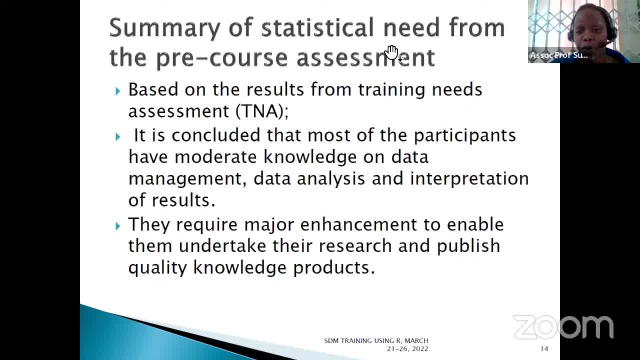 as has been mentioned before. Thank you very much for your attention. I hand over to Dr Helen. Thank you so much, Professor Susan. a very good morning once again. I just want to confirm. if you can hear me very well, then I proceed. please type in the chat. 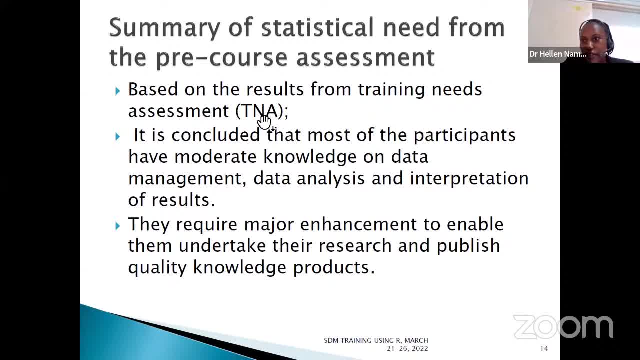 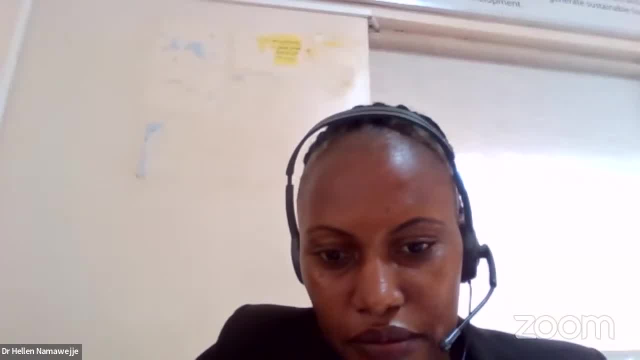 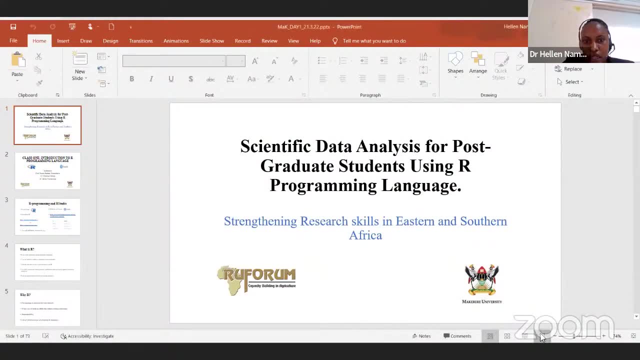 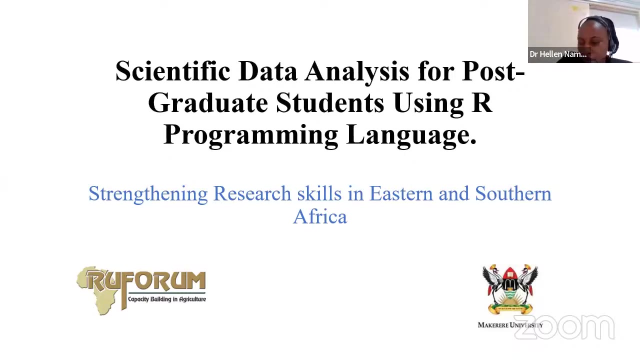 if you can hear me, okay, great, thank you, thank you, please stop sharing, okay, okay, um, as we've heard from Professor Susan, especially when she was presenting the expectations of the participants, and some, some of you are saying that you're just beginners, we've got good, And I still guess maybe we have a certain category of participants as well that have attended before. 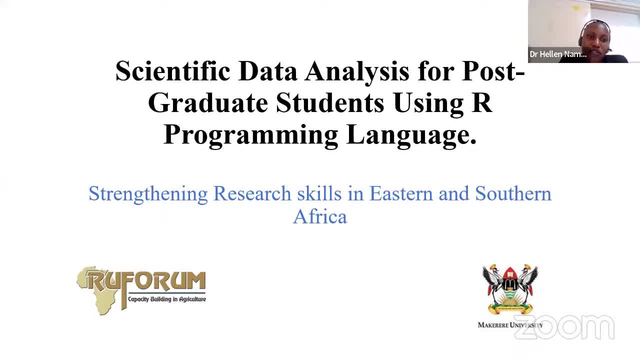 But the point is that what we are going to do again within these five days, we are going to start from the scratch. We need to understand what is involved in R. Maybe just to clarify. I've been posting the Google link which has the materials for today. 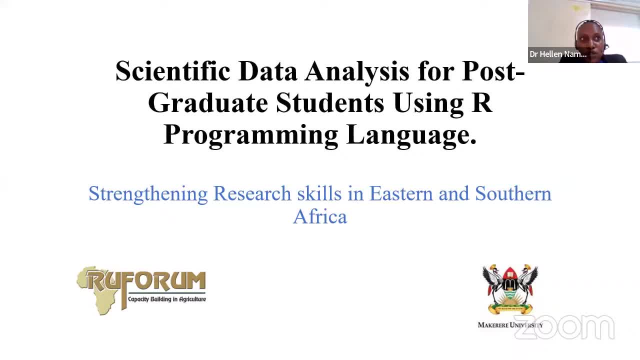 Kindly pick the materials that we are going to use. OK, Like I was saying that I've posted the materials in the chart, I'm posting the Google link. Kindly pick it and then paste it in a URL site that you're able to get the materials that we are going to use for today. 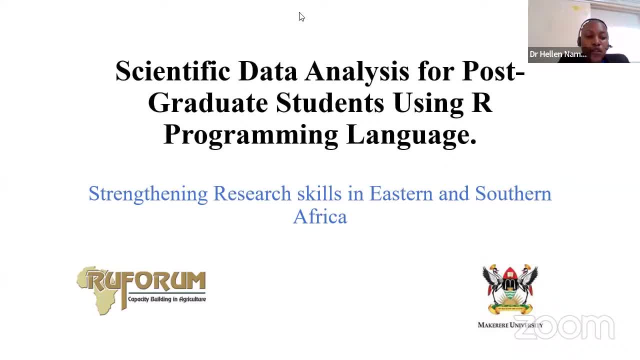 I've pasted it again. Pick it and then it will take you direct to the folder that has got materials for day one, And then it is this link that we are going to be using Every day, what we shall be doing to add more materials for the next day. 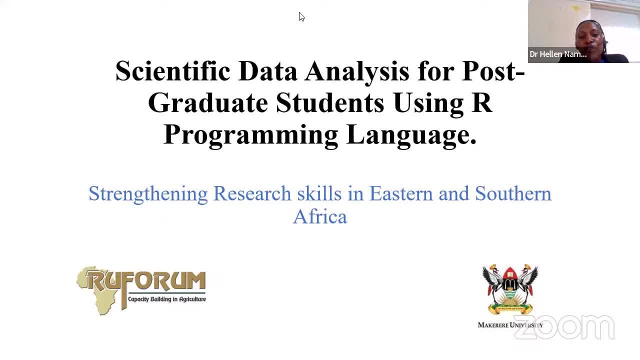 So all you need to do is to keep checking and see if there is new material. But whatever we're going to use today, the material is already there. I've seen some people in emails that complain they have not yet received the materials for the training. 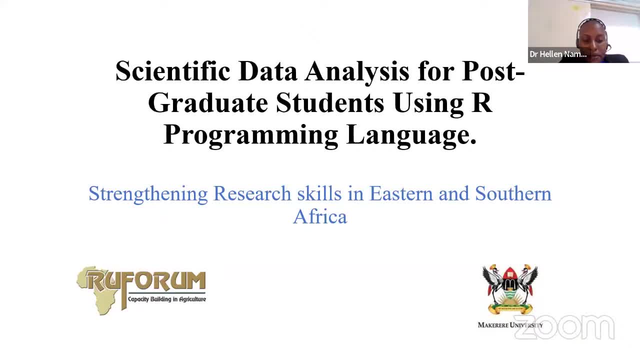 But this is the link we shall be using. So I'm giving you two minutes to ensure that you go to the, you get the Google link, Download and get all the materials for day one And then we get started And like some, like other, how, like other participants have suggested, we'll be giving some, we'll be giving exercise every day at the end of, at the end of the training session. 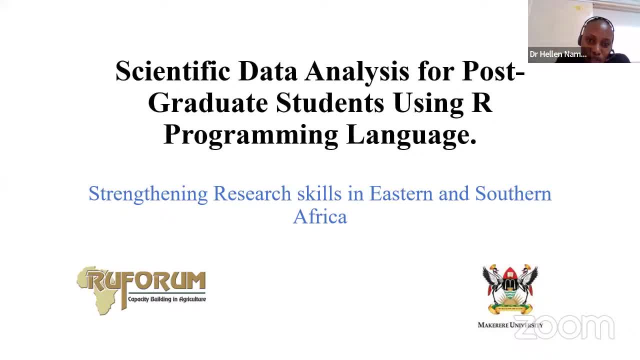 Those still will encourage you, in case you've got your personal data somewhere, as we are, as we are teaching, It is always good that now you transfer the materials, Now you transfer the knowledge that we've taught onto personal data there to make more sense than however much we are giving you field data sets or the kind of data set that you expect to encounter. 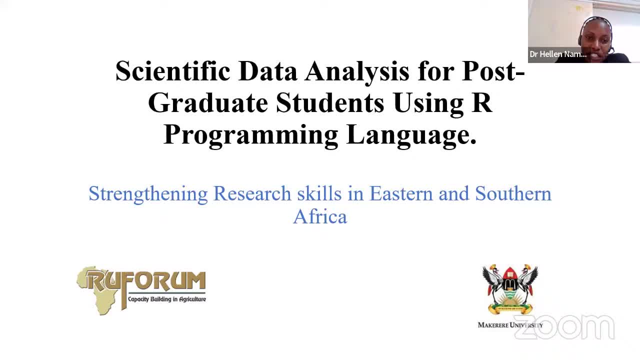 Maybe as you go to the field and so on. But in case you already have a data set that you have on your own after the training, maybe given an exercise, you can. you can try to use the skills that you've learned on your personal data set. 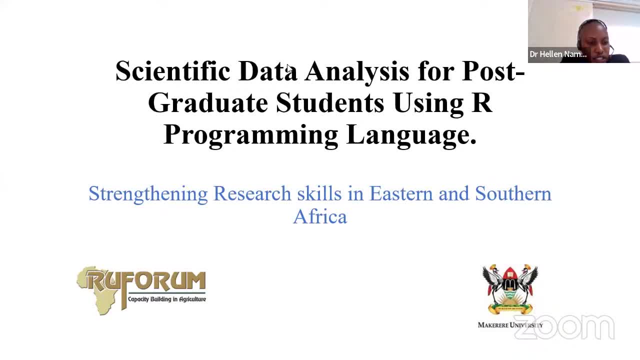 Okay. So let me ask in the chat: Would you share us the training material? Okay, Okay, saying that downloaded already. Please get the training materials from the Google Drive. Otherwise, in case we say that we're going to be sending to everyone, then we'll still have many complaints. so it's what you want to reduce. the training materials are within the Google Drive that have. 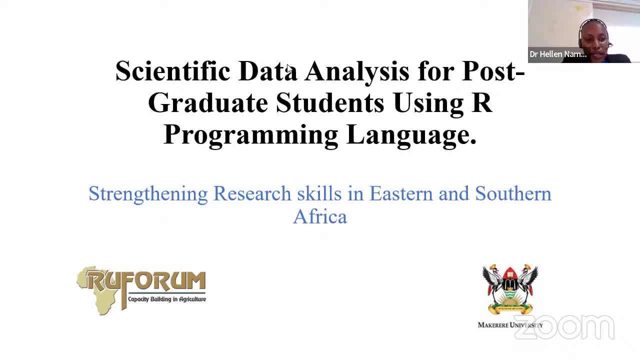 posted in the chat, So pick one And then I will start. Jim says also posted about downloading- are using the link that he has given us. That is also very good. since we're going to use our, We need to have our, our studio on our computers. unless you have those two, unless you have those two downloaded and installed on your computer, then you can do anything. 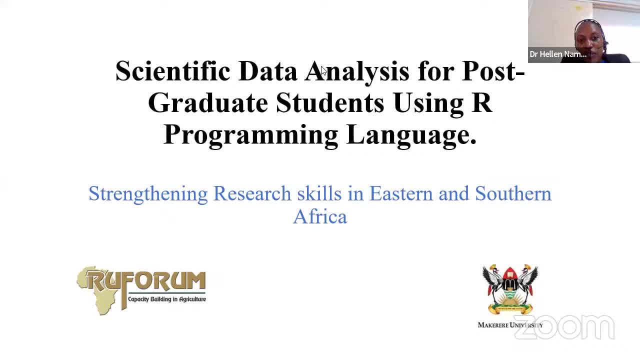 Okay, Okay. somebody is asking that kindly show us how to install our packages. Well, we are going to see that, but let's ensure that everyone has been able to get the materials. So let me ask: in the chat, kindly type: Have you received the materials, the folder for the one? type in the chat with the type for me. yes, that I get to know if I should begin. 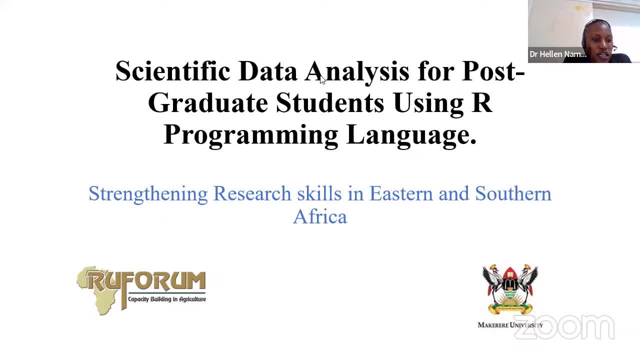 Okay, Okay. I'm seeing great numbers saying that, yes, that they have received. All you need to do is the link. If you've got internet, then you'll be able to come up with that folder. We are downloading them. Okay, I'm going to give you only one minute now, so that those who have not yet done so. 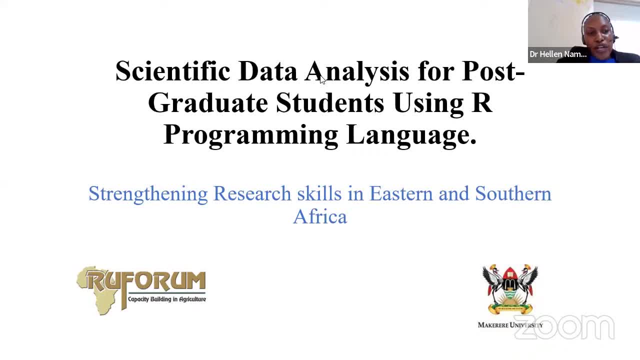 We are still getting materials from there, We are still getting materials from the, from the Google Drive, and then, at the moment you doubt you'll get the folder. kindly save it on your computer somewhere where you want to, where you want your training materials to be. 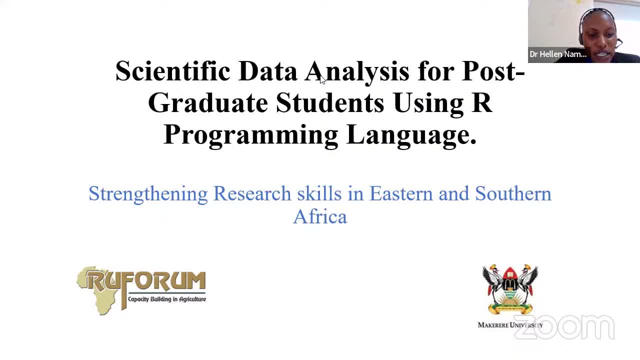 It has been posted again, So please get it. download the material. there's only one folder, but as we end the training, will be updating this assembling, so you need to keep it open, our document, and keep it somewhere or save it within your training materials. 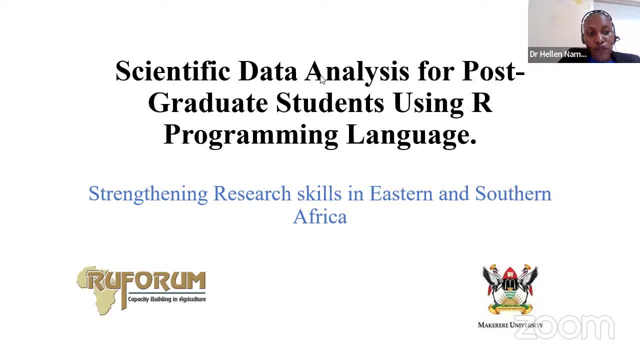 It's what we want. It's what will be keep updating for, for example, we'll put the materials for day two, day three, up to day six. So if you pick it now, then it will be. it will make both your work and my work easy. 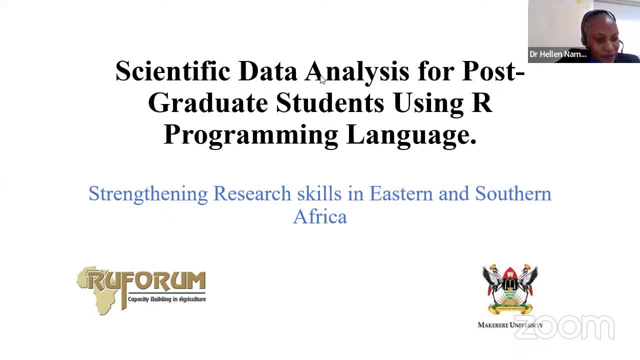 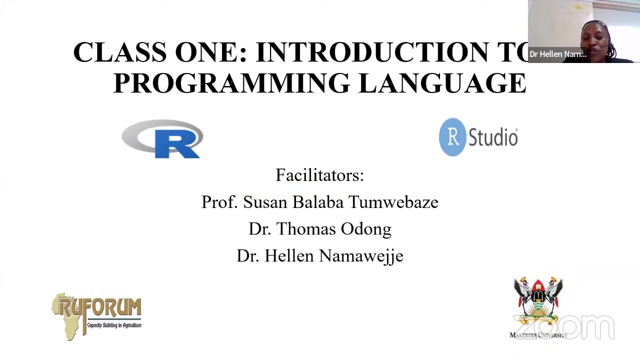 All right. so can I get started? Just type continue. if we are safe, Type continue in the charts and I and I start Okay, great, All right. Okay, Now we are starting again. we're going to use our programming language in in our training, So we need to first understand clearly what is what is involved in our, and then we're going to integrate it with our studio, this to work together. we're going to see the 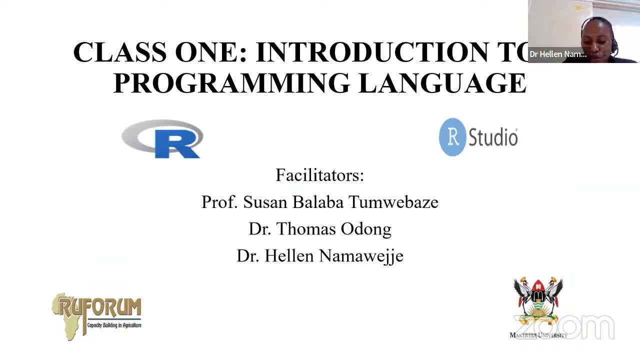 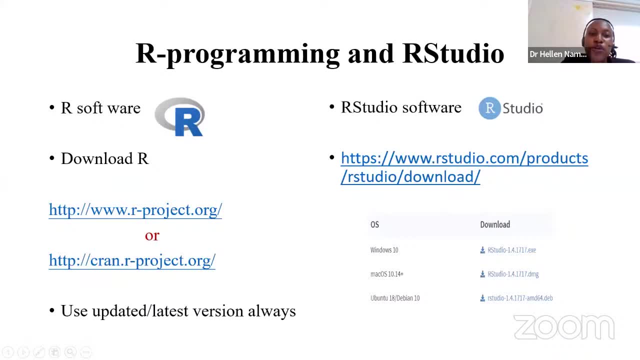 differences and see how our is really interesting in case you're going to do, in case you want to do, analysis, And then we're going to use the software, like the ones that you've used before or you've had about. you need to first install them on your computer. 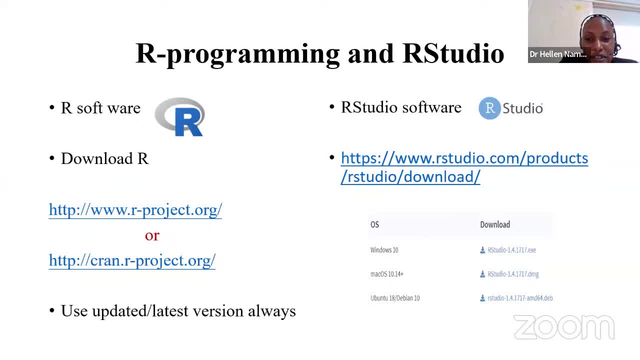 Right. So what we are going to first do right now is to download our. after downloading our, we're going to install it on our computer. Then later we are going to download our studio. After downloading it, we install it on our computer. 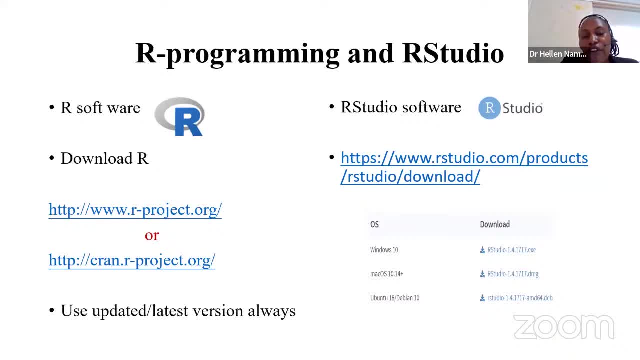 I have at the back of my mind that maybe there's some participants already have This. People already have our and our studio. But the point is, is that package updated? So in case we have some colleagues, in case we have participants that up? 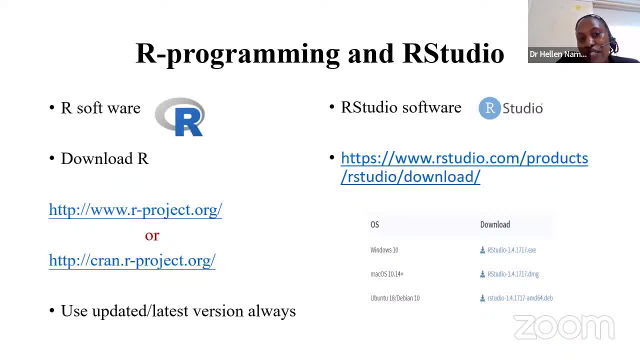 However much I shared the material, but I still think maybe there's some other people have not yet downloaded our. In case we have such people, let's try to go through. how do we download our then our studio, the moment everything is on our computer, then will be more than good to go. 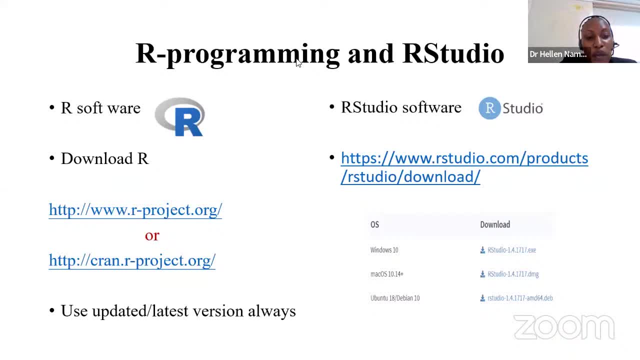 So, in case you've got the our package already, All you're going to do is to update, because- remember what we talked about our- All you need to do is see that you use the latest package, use the latest version of our, because it's an open source and every now and then, a lot of information is being done to see that our is being developed to a better version. 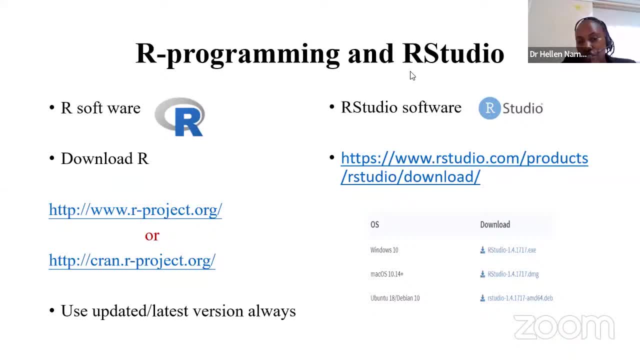 Okay, so I'm going to stop sharing this. Okay, so I'm going to stop sharing this and I share the video. Okay, so I'm going to stop sharing this and I share the video. And for now, And how we can download our in this. you have it already. 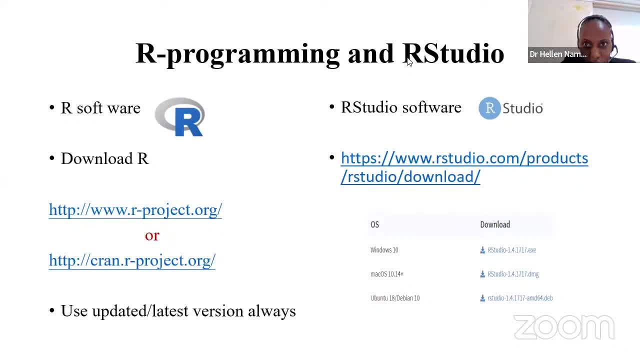 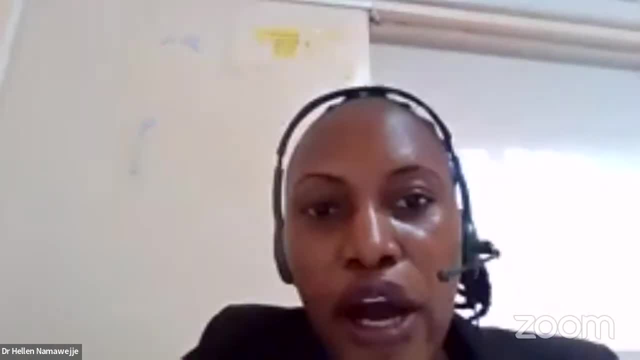 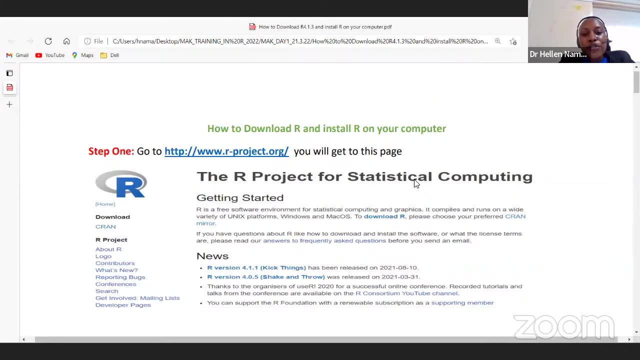 you need to update it, the latest version, Okay, So what I'm sharing now is how to download our and install it on your computer. Okay, Remember, I'm still in the in the in the training materials for today. Okay, 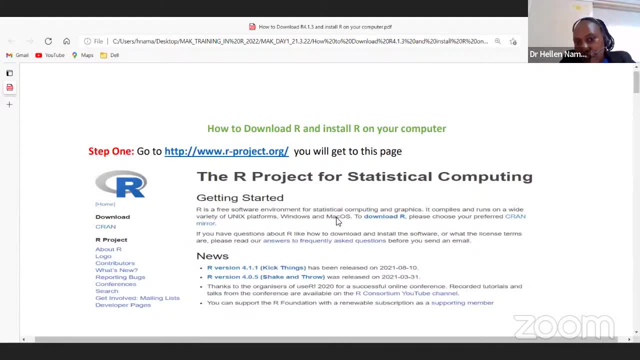 all the things that I'm sharing with you. they are all there. If you have the folder already on your computer, you can as well open the PDF that is served as how to download R and install it on your computer. So within that folder there's this particular PDF. 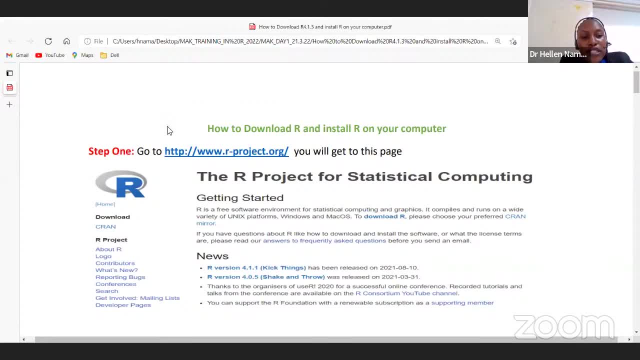 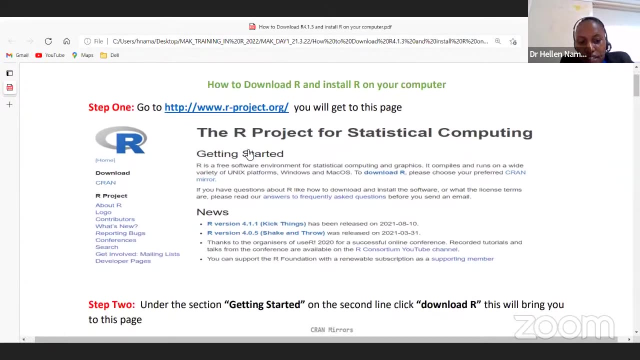 Let's go step by step and we see. Step number one says that go to the URL here, which is http, then wwwr-projectorg. okay, So in case you click on that, step number two is going to be under the section get started. you click on download R. 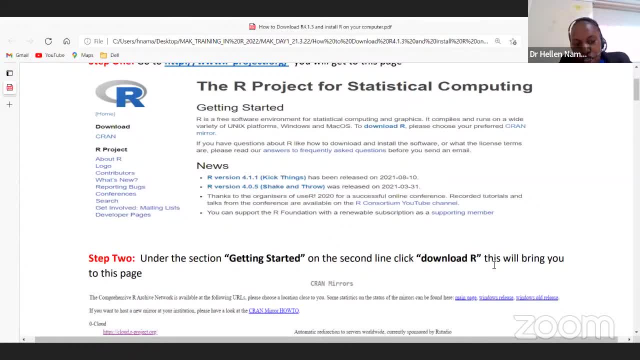 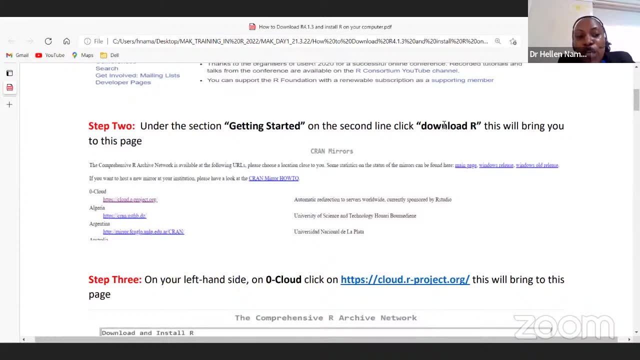 But let's first go through the steps, then I'm going to do it with you. Then after that, in the next step that you click on download, on download R, The moment you click on download R, you're going to come up with this particular page. 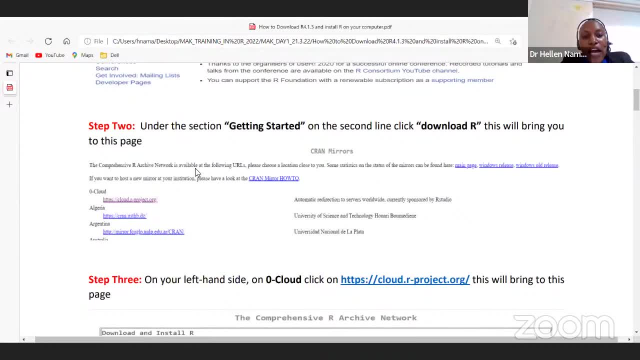 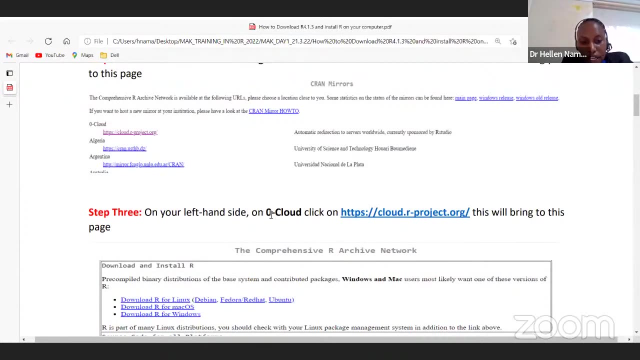 There are only two screenshots that you're able to see, And then on your left-hand side, you're going to see this where I'm putting the cursor: https, then cloudr-projectorg. So what you do on your left-hand side on O cloud, where you see this: 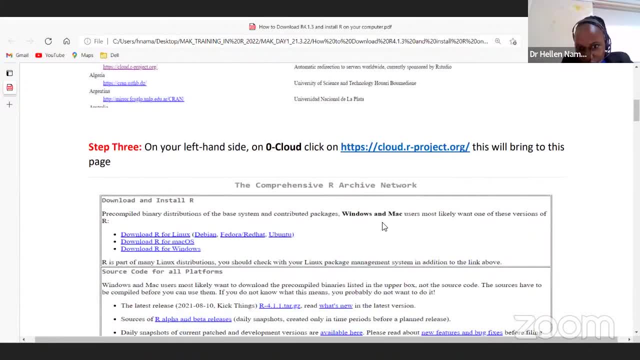 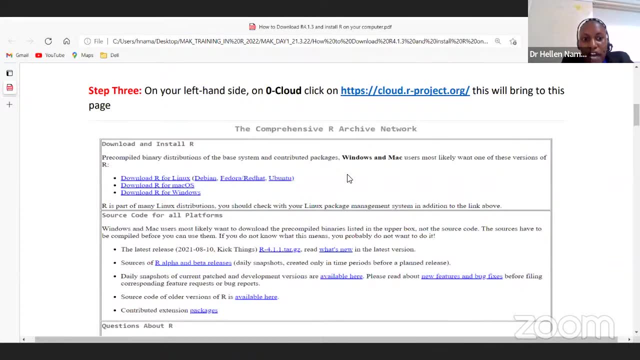 then you click on it, it will bring this particular page. The moment you see this, all you need to do is to get to know what kind of computer are you using. Are you using the version? are you using a Mac? are you using Windows? 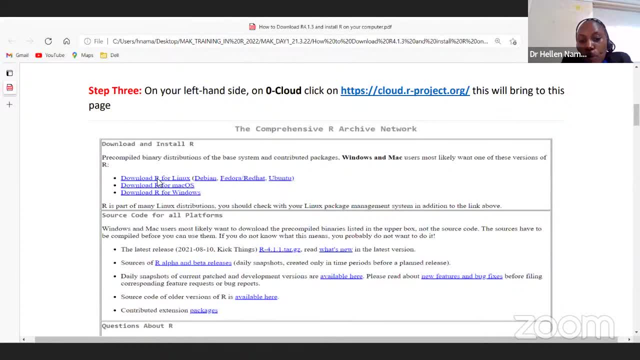 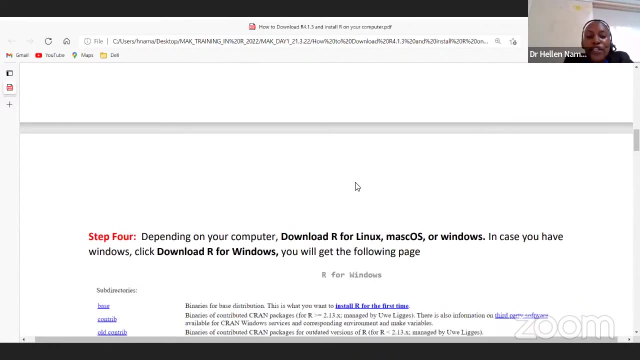 are you using Linux? So you come here and then you click on what, on the type of version that you have. So for my case, I'm using Windows. So the moment I reach this stage, I'll click on Windows And then I come down after that, depending after that, after clicking on downloading R. 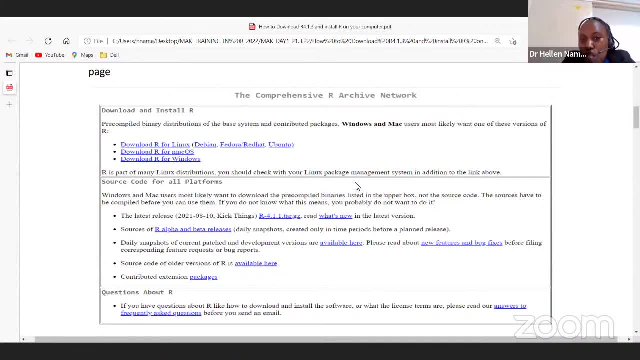 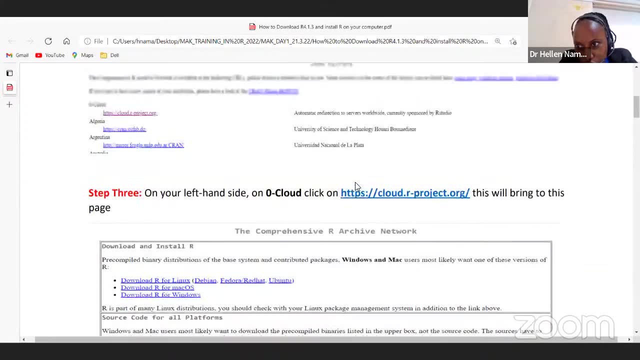 the application is going to start downloading, So all you need to do- All you need to do- is to give it a minute to install on your computer, And we are going to do the same for R studio. So now let's go back together. 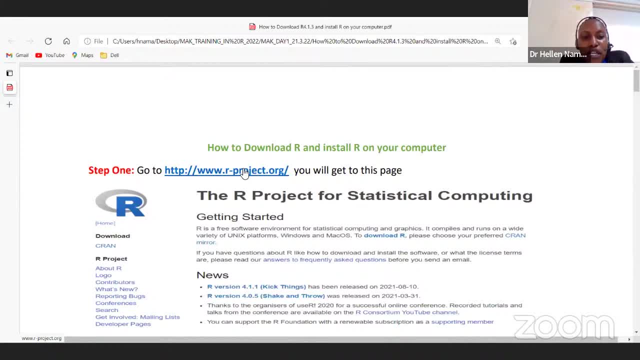 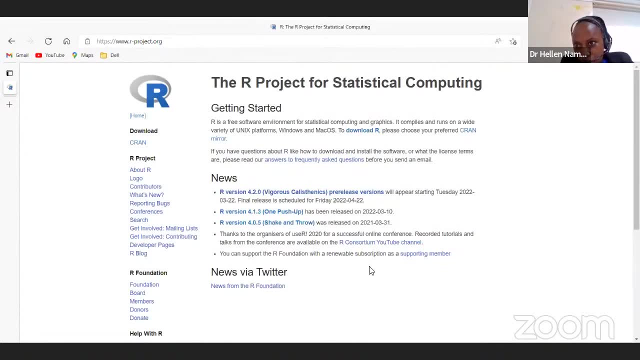 Let's walk through the steps and we'll see So on your computer. just click on this URL. The moment you click on it, it brings this page, like how I shared before. Okay, So, after clicking, our next step is you come and click download R. 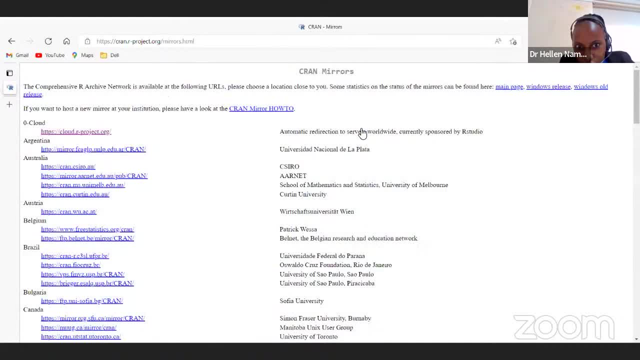 Okay, You come and click here. That's step number two. The moment you click download R, this is the page that you're going to get The next step. step number three: you come and click on your left-hand side where there is all dash cloud. 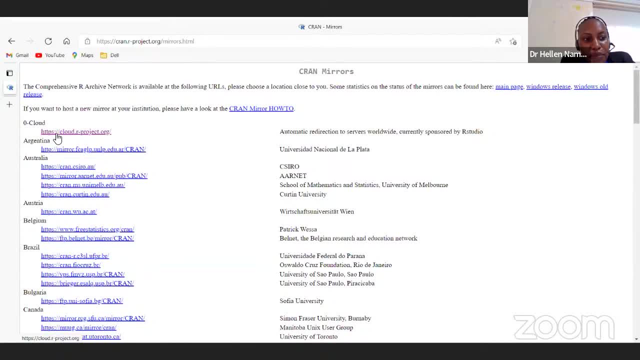 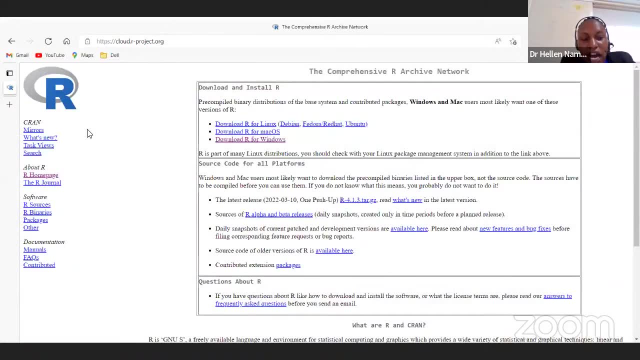 You click here, You click on HTTPS, then cloudrprojectorg, You click on it. After clicking the fourth step, This is the page that you're going to see To download and install R. So it depends on like the version you're using of the computer. 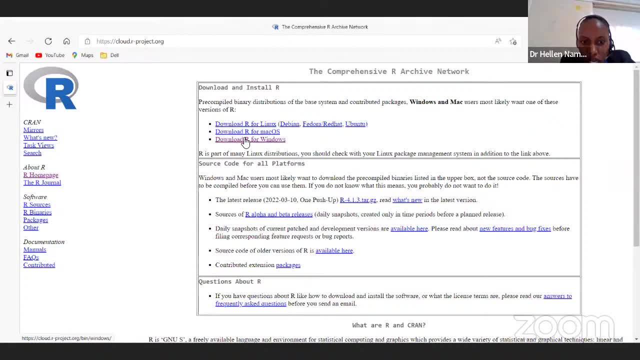 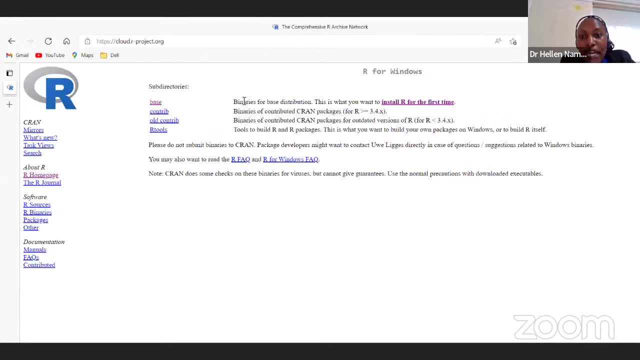 So right now, for my case, like I mentioned, I've got R, I've got Windows, So I'll click download R for Windows. I click there. The moment I click that, this is the page it brings me. Then I go on the fifth step. 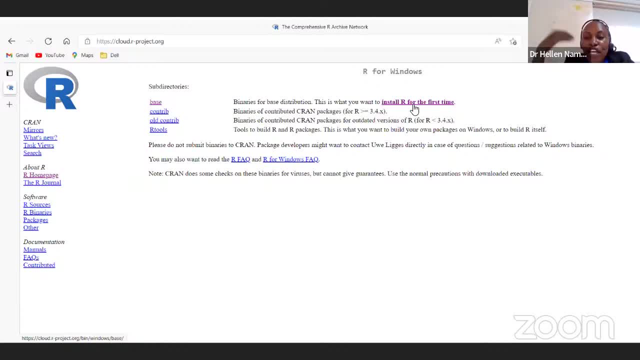 Install R for the first time. By the way, in case you've got an updated version, you can also install again and get the latest version. If you don't have R on your computer, you still go through this, the same steps. 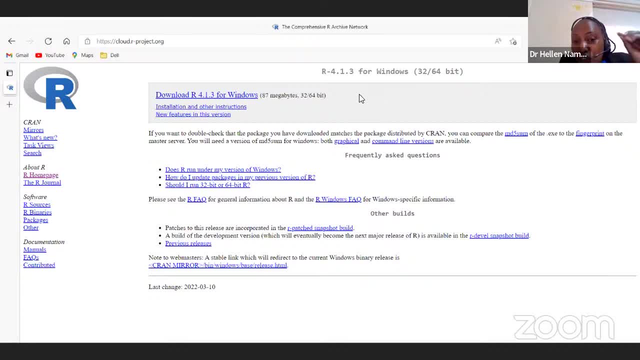 So you click there Right now. the current version of R is R-4.1.3 for Windows, So it is the current version that we need to use, In case the version of R you're having is R-4.1.3 for Windows. 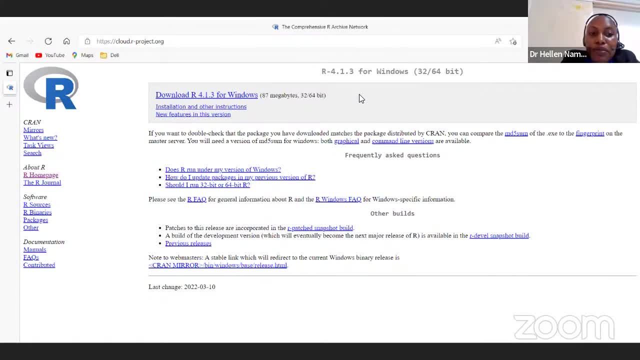 is below 4.1.3,, then it implies that you need to update to the latest version. So the moment you reach this particular page, you come and click here. download R4.134 Windows or as the R project. their website will give you the latest version of R As more packages. 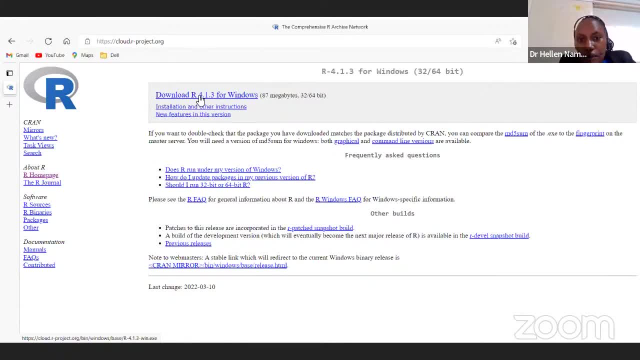 or more updates come in. there is update the R software. So if you click on download R, the moment you click there, what is going to happen? if you're seeing on my right-hand side, there is a download that is taking place- R-4.1.3-windowexe- The moment after this. 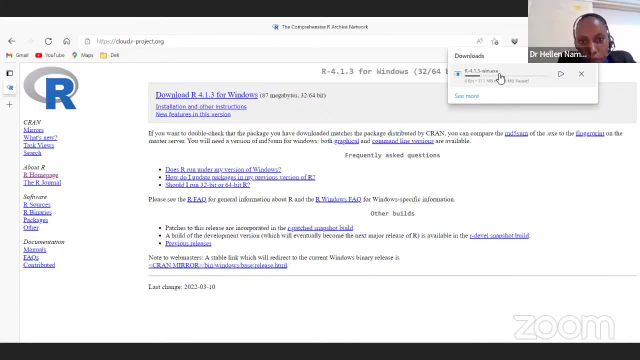 installation is complete. all you need to do is to follow the prompts. They will tell you: do you allow to install on your project? Do you allow to install on your project? You click yes and you follow the way you install other softwares. I don't want to install R again. 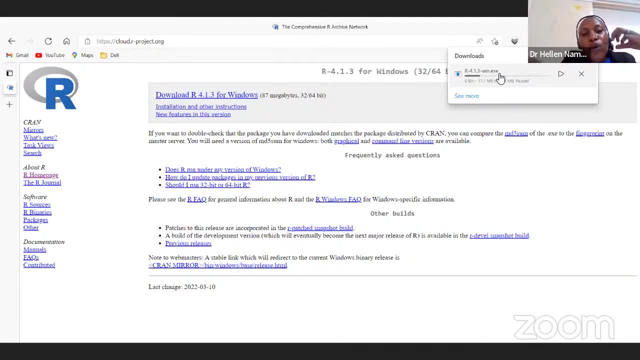 because I already have it on my computer. but I was just showing you how you can do it, how you get the last step of installing R on your computer. So let me ask in the chat: have you managed to go through those particular steps? Faith is saying I'm not hearing anything. 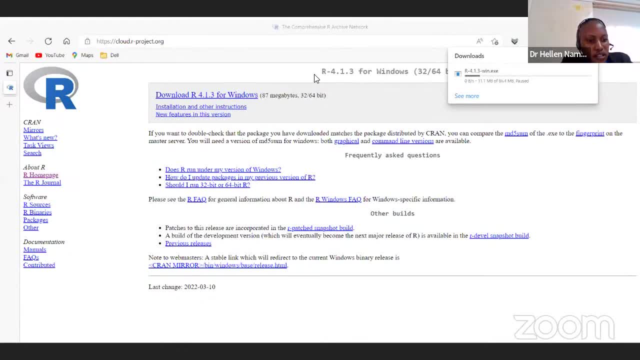 really Okay, Okay, Great. I'm seeing majority are saying that, yes, they have managed. Downloaded, Yes, I already downloaded. That is great. Okay, That's wonderful, All right, Downloaded and running. Downloaded, Yes, but it is downloading slowly. I've not been able to. 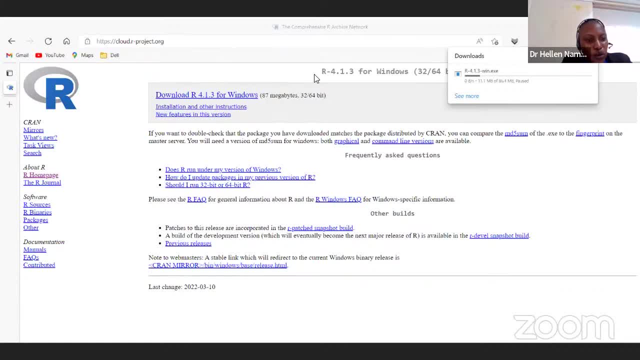 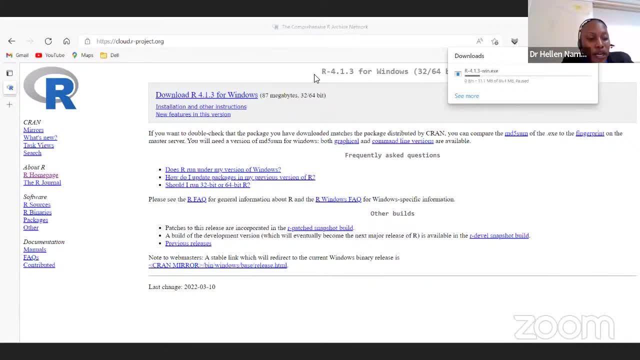 who had utilized the material and downloaded R on your computer. Thanks for the great work done, But me I don't have the link Downloaded and installing. Kindly help me paste the links for the Google Drive Downloading progress. Okay, That is great. So these are the procedures I was talking about on how you download. 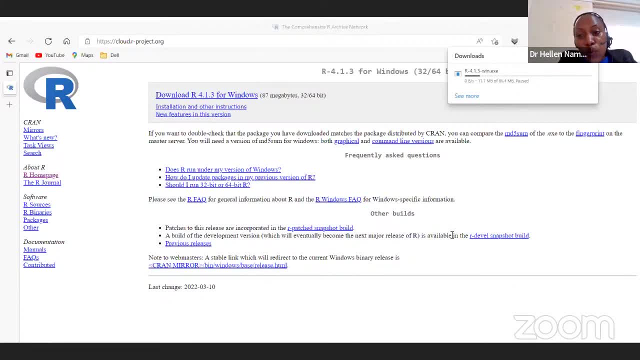 R, In case you have a version that is less than 4.1.3,. we are going to see how do you update the latest version So that you what are the various commands that you need for you to always update what you have version, And as you update the latest version, you are going to see that you have. 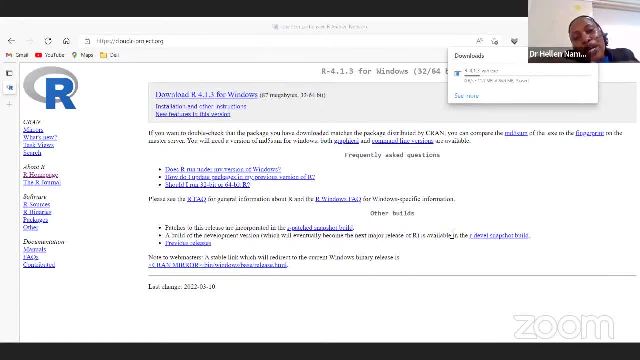 the latest version So that you what are the various commands that you need for you to always update. still, R will tell you. as you use R, it will be able to tell you that you know what. there is a current version. Would you like to update? Would you like to now to upgrade to the newest version? All you. 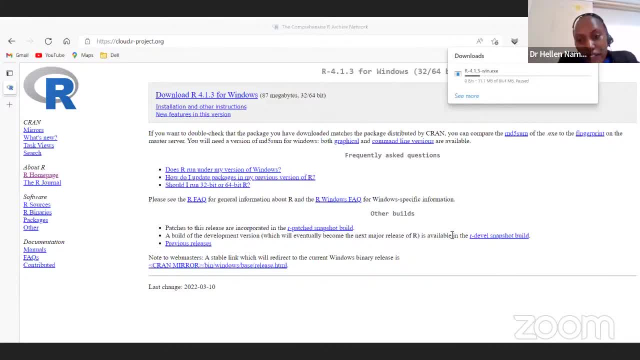 need to do is. I mean all you need to do is to type yes And then it will. I mean, as you click the prompts, it will be able to direct you how to go ahead. Okay, I'm going to stop sharing this. 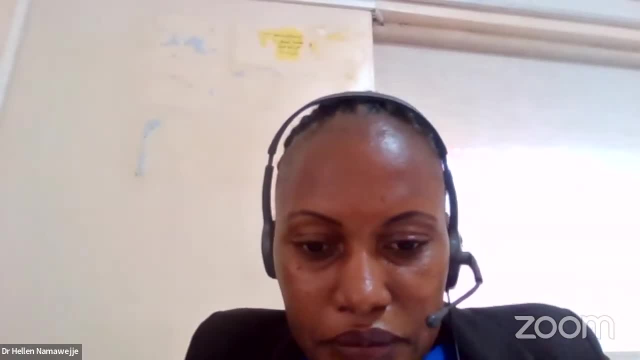 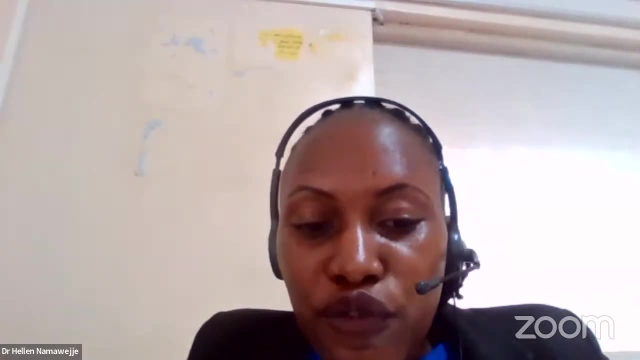 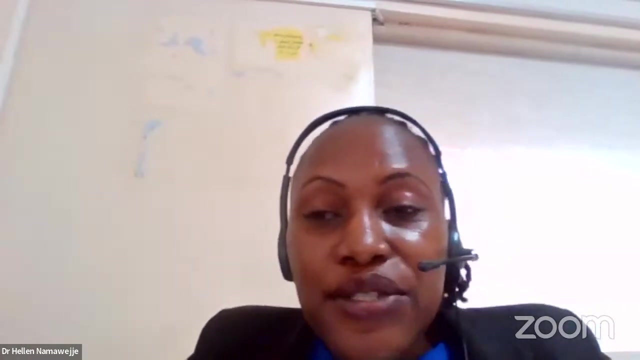 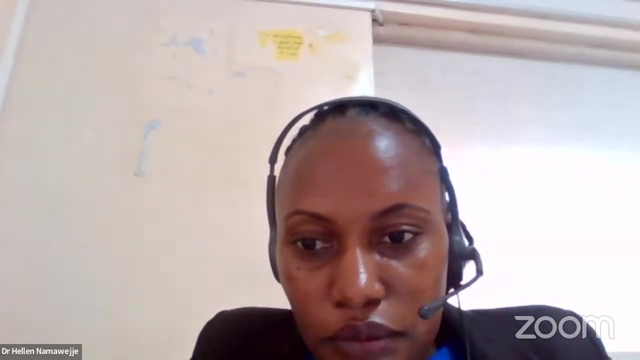 and I share my PowerPoints again, Sorry. Okay, The new version of R is 4.1.3.. In case you have maybe 4.1.2, it implies that you need to update. you need to upgrade to the newer version. All right, Okay, So I'm going back to 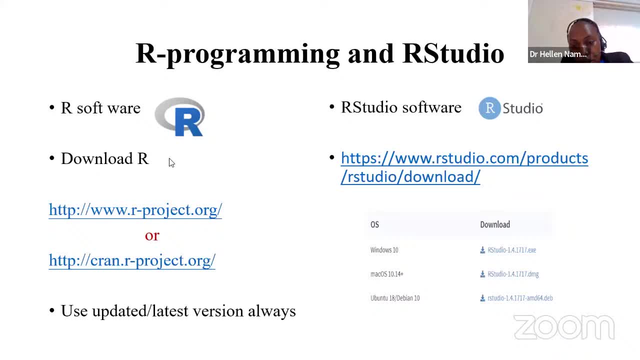 the slides. Our first step was to download R. Those are the steps and they're easy to follow, like I've showed you, And always ensure that you use the updated or the latest version. Now, after having R on your computers, it is also important. 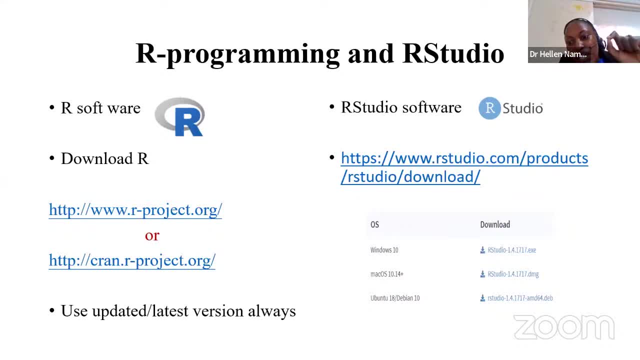 that we download R studio. Okay, We need R studio as well, such that we have the. we are able to use both of them. But as we move on, we are going to understand the difference between R and then R, How R studio. I mean, could I use one and leave the other, or what is going to happen So? 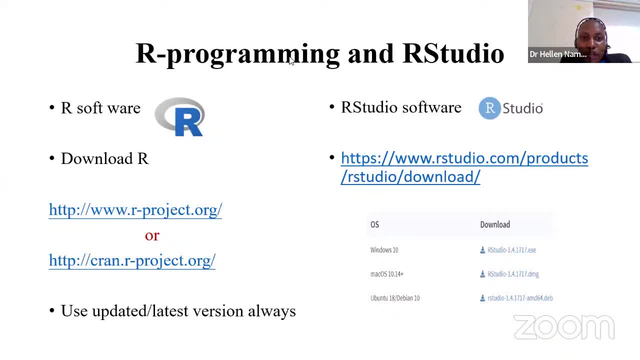 okay, some people are asking for the scripts in the chat. Send us the different R code. Kindly check in the in the google drive. all the materials are there. we didn't get the pdf um send us the, please. let's move step by step. our first step, where i sent the: the google link it. 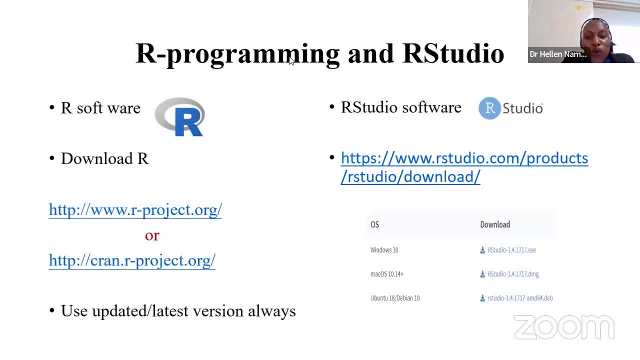 has still has been posted again by professor susan. within that google link, please check. there is a folder. hamilton is saying that folder has material and we need to move step by step. wonderful, yes, some. how come that's uh, in the same folder, some people having the materials. 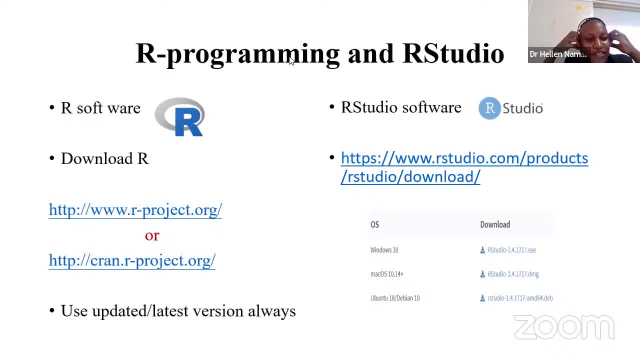 and that's um, don't you know it's. it's interesting, it's the same google drive. uh-huh. jambi is saying that all the materials are there. please follow the link. download the the folder. it has day one material. okay, whatever that, i'm showing you all the things are there so that we are able to move. 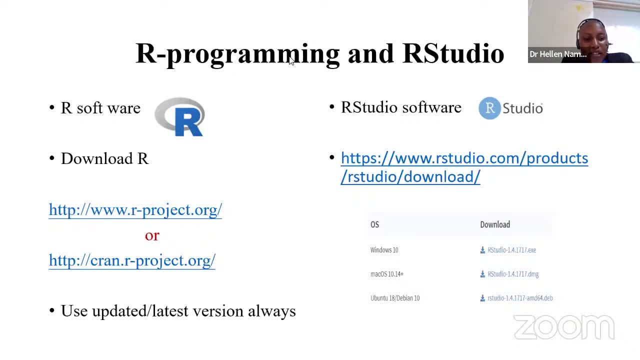 great, james, thank you. he's also confirming that all the materials are in the folder. all you need is to paste the google link on the url and then download that particular folder. you'll be able to see the material and then put the folder on your pdf. uh-huh or chase saying that step by step. please, no rushing. keep out of this space. 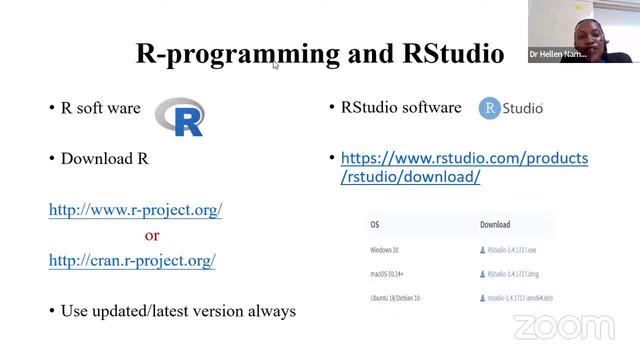 okay, i was reading people's comments, so let me ask in the chat: have you been able to download r, can we? can i say that we are done with downloading r and we move on to our studio? muhammad is saying 98. uh-huh. okay, r is downloaded. great, both have downloaded. i'm glad that some people are faster than me. 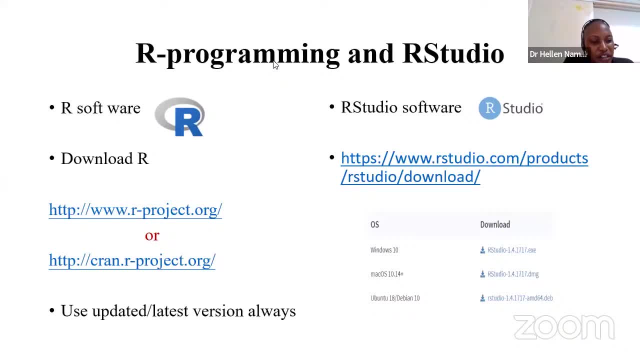 um, help with updating. we are going to get there. in case you already have r, we are going to update. if you're um. if you don't have the latest version, great for all. i've seen your comment that waiting for you to shout: update, downloaded and installed, not updated. we are going to do that. okay, let's. 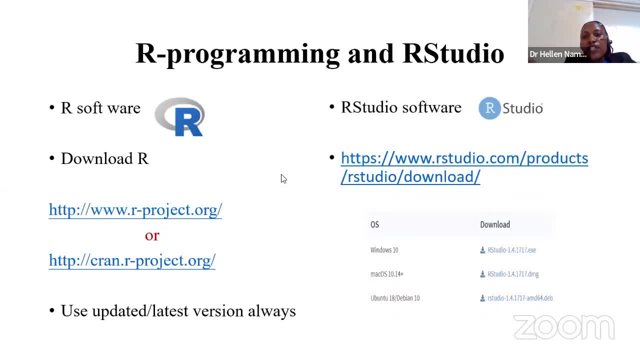 continue. now let's move on. we need also the r studio. still, if you don't have an updated r studio, we are going to see how to update it. but remember, in case you, the moment you install a newer version, it automatically overwrites what you, what you have earlier. okay, and that is one option on how you can. 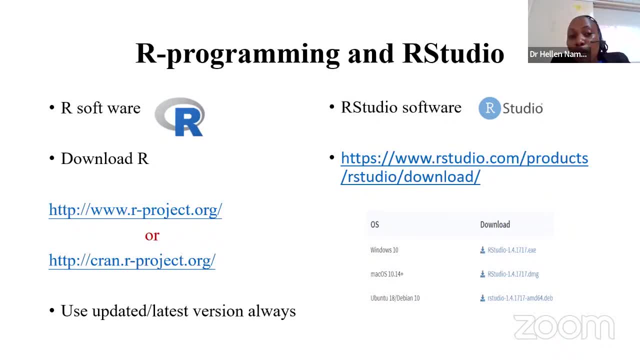 update r. however, we are still going to see certain commands that you can use within the old version, such that automatically the older version is updated to the newest one. okay, now, the moment you come to, we are going to go to our studio. now let's move on to our studio with our studio. 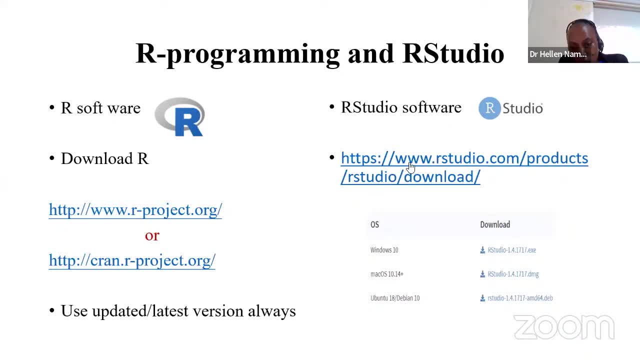 software, because we need both of them. you go to wwwourstudiocom, just get this, this url, and paste it in google, because they already have the powerpoints. the moment you um, the moment you paste it in google, all what we are going to do is to um, to scroll down until when we see the windows and 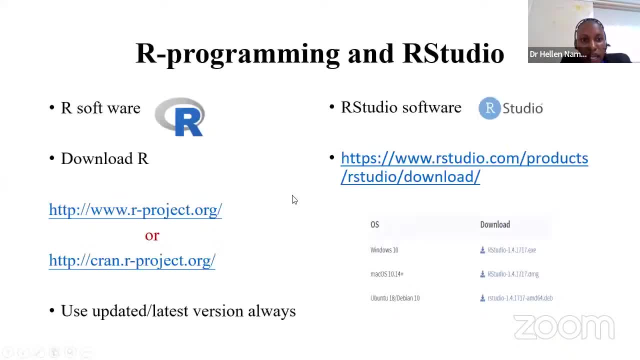 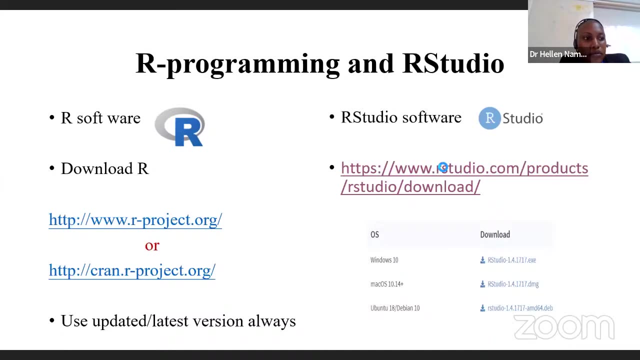 we click on it and then we we download. okay, maybe, what i can do, we can still um do step by step. i'm clicking on, hopefully to um okay, it's a little taking long, um, let me try to. all right, um, what i'm going to do, i'm going to. 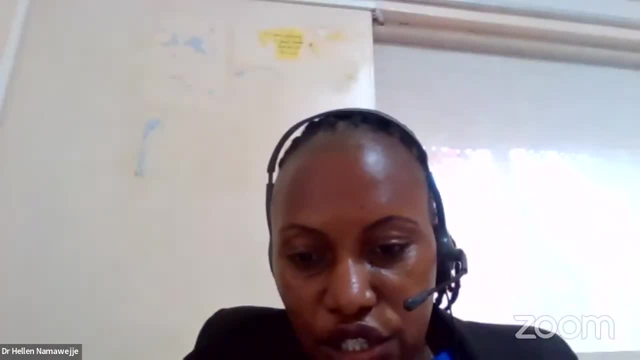 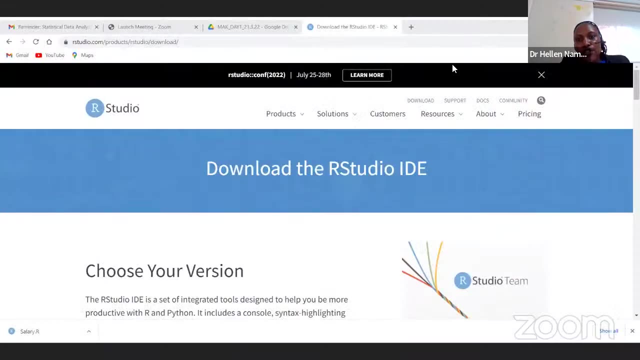 i'm going to stop sharing this and then i share my um. yes, let me share the url direct. so, in case you, in case you um, you type in, you go to your url. if you see, very clearly, i've pasted it, my url up here: our studiocom slash products slash. our studio slash download. that is the, the link that. 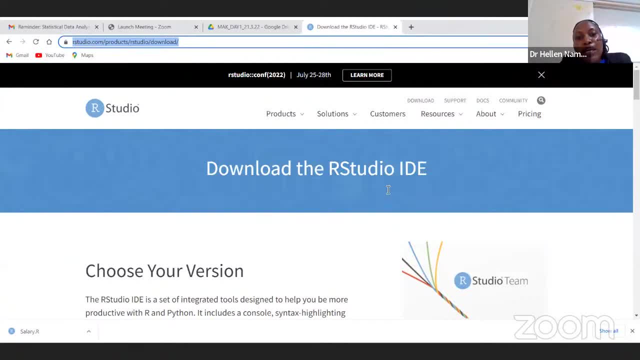 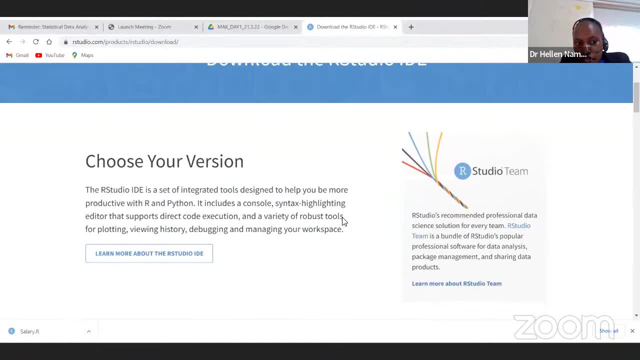 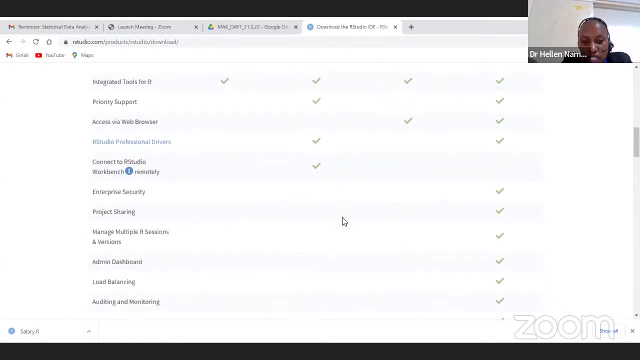 i sent you in the url. you need just paste it there. so the moment you paste that link in google, this is what you're going to see: the download our studio ide. so, um, it will always tell you that, to choose the version, there is a free one. you download for that. you can read into those particular details. but as you scroll, 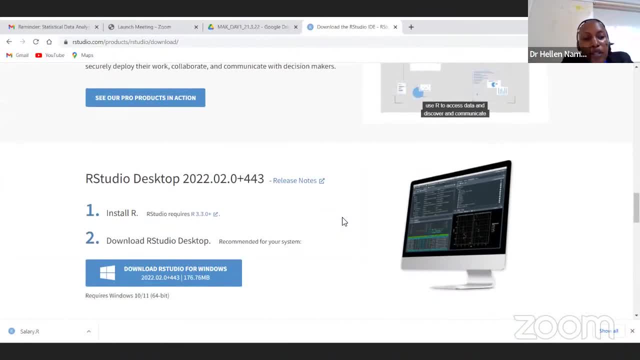 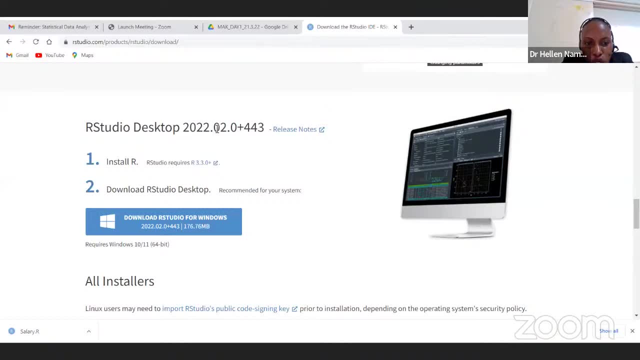 down as you continue. i want you to scroll down and come to this particular page here where it is showing you our studio desk 2022.org, plus 443 still. this is the latest version of our studio, so there is a new version in in in this. 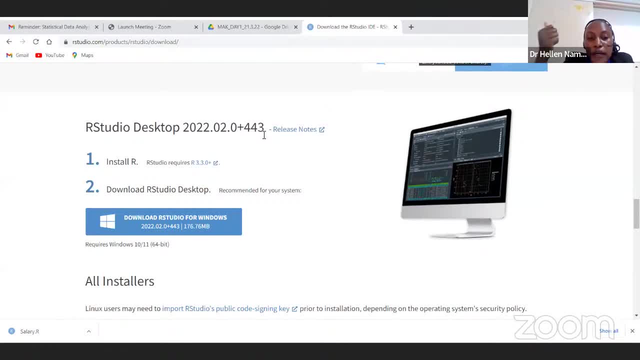 current year, the one we had earlier. it had um, it had a 2021 of september, but now we've got a current one. so, as you see here, because when you look at the first step, still they are telling you that install r okay, you need uh, and they're telling you that our studio requires r 3.3 or plus. 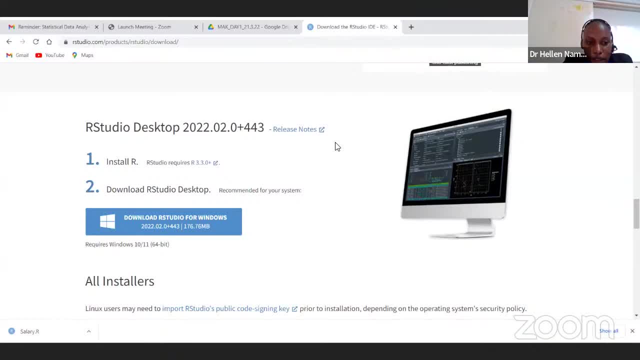 and above. but we've done that first step of installing r. now i want to download our studio for the desktop, and this one also works for windows, so in case you don't have it installed, all you need to do click here. i already have our studio on my computer, so i don't want to install. 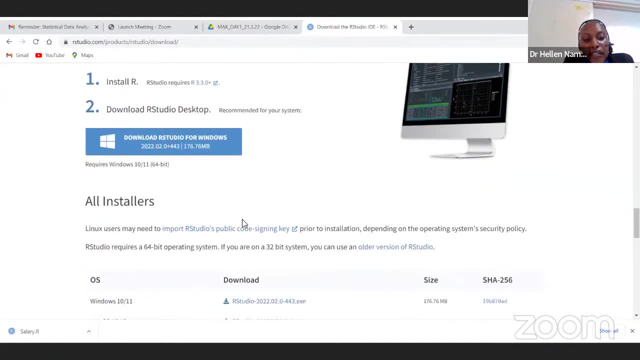 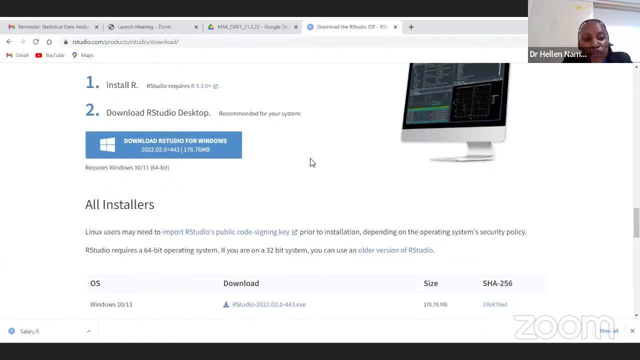 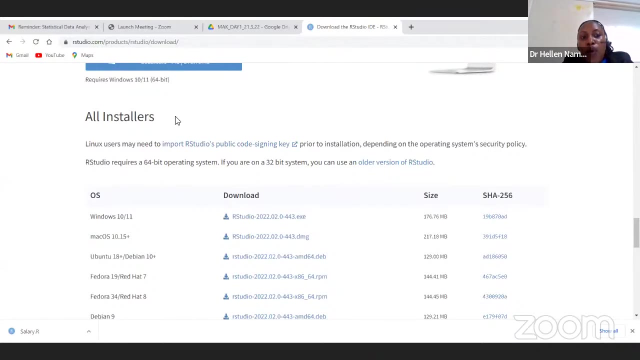 it again: the moment you click on uh, the moment you you come and click, uh, download our studio for windows- what is going to show you when you move down on the other steps it is going to bring you. you're going to see this particular, this particular page, which has all installers. 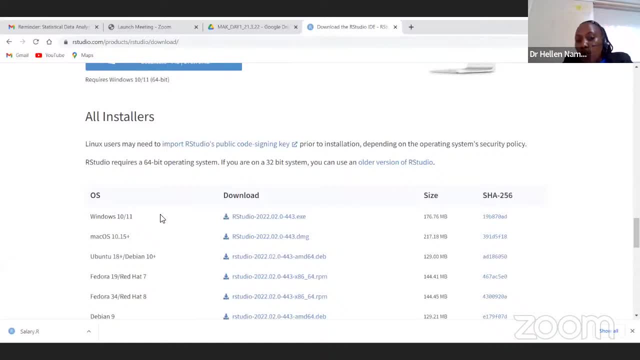 and all you need to do is to come and check windows, depending on the os you're using. so, like i mentioned for my case, if it's windows, then i'll come and click on this. uh, on r studio 2022, then .02.0-443.exe, and this is the installation file, like we did for our studio. 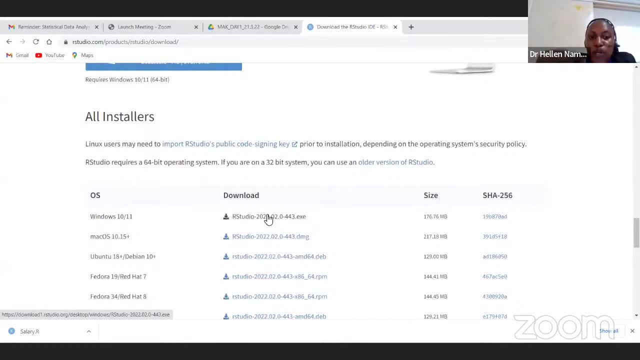 then all you need to do is to follow the prompts, as we continue to, and as, as it downloads on your computer, you keep following the the process and then, after that, you'll be able to have our studio. so I'm giving you a minute, and then you go through them such that you have our studio with you. 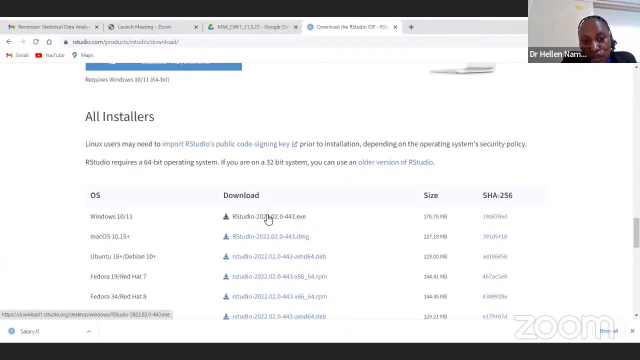 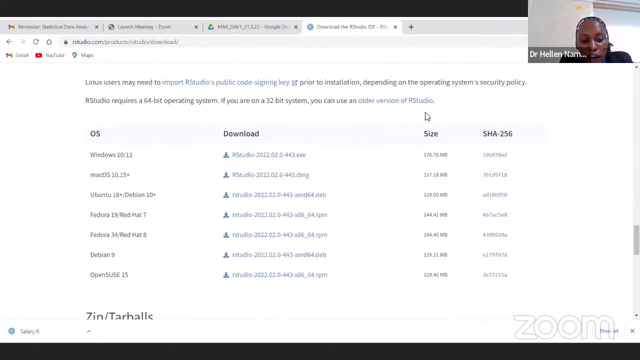 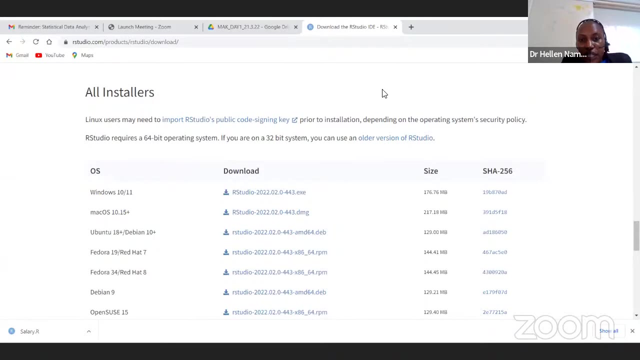 because we need both. we need our and then our studio as you're downloading. I don't think it will take a lot of time. it will take you around to two to two to four minutes to have our studio and that is all that that you need. okay, let me stop sharing this and I share my slides again. 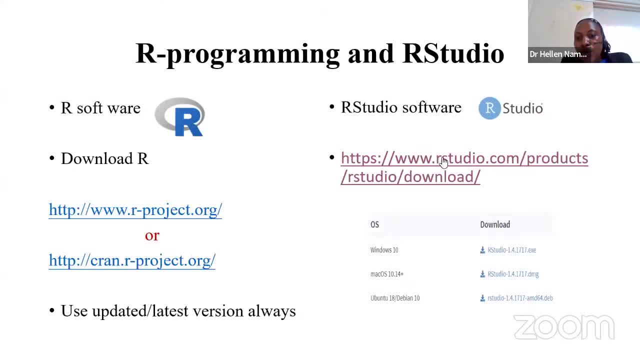 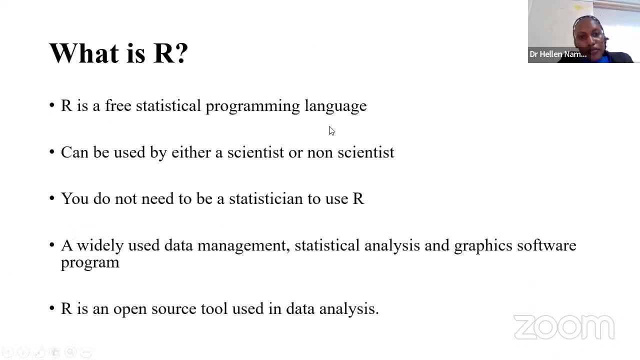 all right, in case you got this and pasted it, we should be able now to have our studio. okay, let me ask in the chat: um, have you been able to download our studio? just click on the link. it will automatically open. yes, um. alice saying yes. pascal saying still downloading a recent downloading. 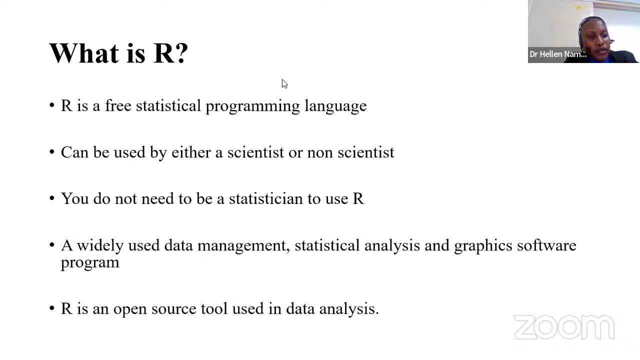 yes, okay, great. yes, ours, our studio downloaded, downloading. kindly share the link for downloading the our studio, please. that's a good one. okay, all right, okay, updating downloaded had then already, of course, great. in case you have a specific question where you need more clarification, please paste it in the q and a? um. other facilitators will be happy to answer your. 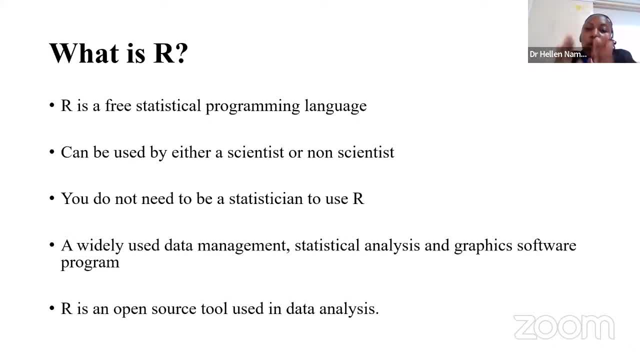 questions as the training is going on. so if you have any questions, please feel free to ask them. so if you have a question that that really needs attention because, uh, when you paste it in the comments in the in the chat it really moves on very fast. but in case you post it in the key and 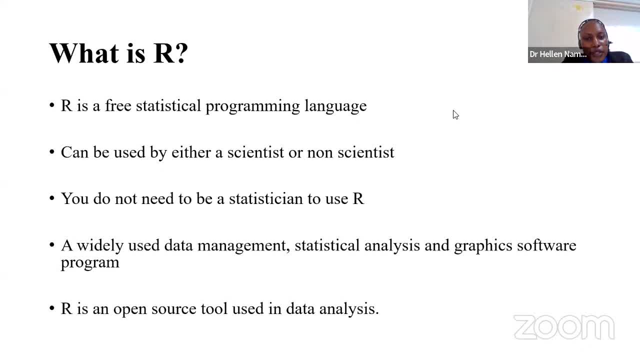 they will be able to get an answer in a um in a very short time. so let's move on. what is r? you know? we need to understand what is this program all about, and it's like that we are able to say that you know what. r is really a good program which I can use over other um statistical. 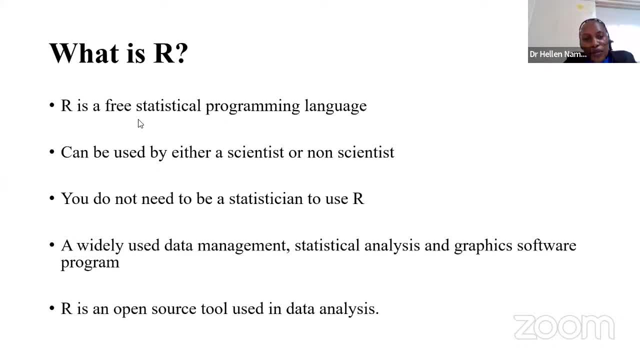 programming languages. so, like I said, with this, with with r, it is a free statistical programming language. all you need to do have internet, go and download it in case you know the procedures of download, do the download. you don't need to pay for this software because it's an open software. 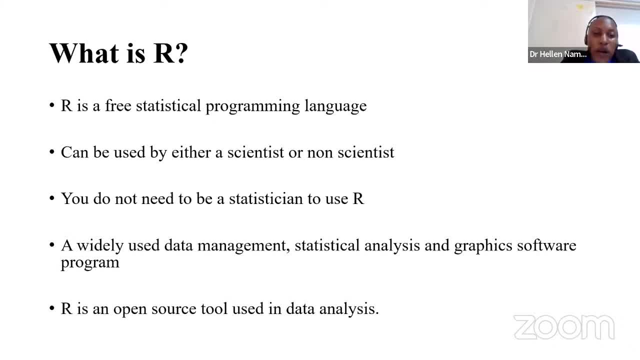 and anyone can use it, depending on the analysis that you want to do. it's open. you don't need to be a scientist, or, or, or anyone- a scientist or a non-scientist can be able to use r, and you don't need to be a statistician to use our programming language. 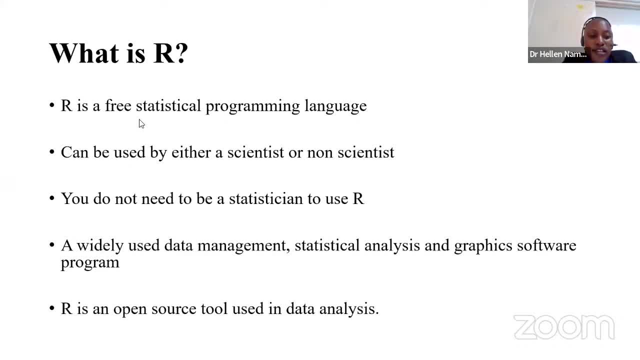 it's quite interesting, but r is widely used as a, as a data management tool, and it can be able to to to to support in good graphics of uh, depending on the program that uh or the kind of data visualization that you can see. I was like I mentioned earlier that r is an open source. 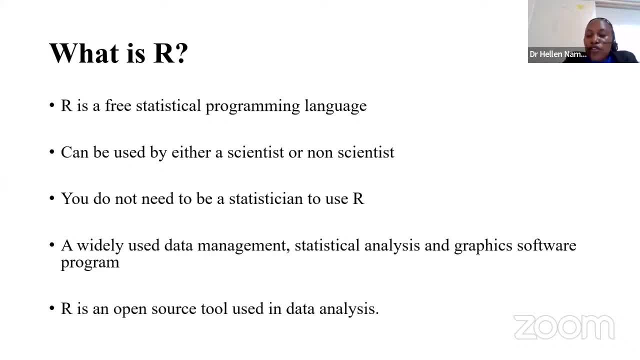 tool used in uh that analysis. the moment you have r and r studio installed on your computer, like we are going to learn, you can even go to your village, wherever that you want to go, and do your analysis from wherever you want, the moment you have uh, the, the, the, the software. 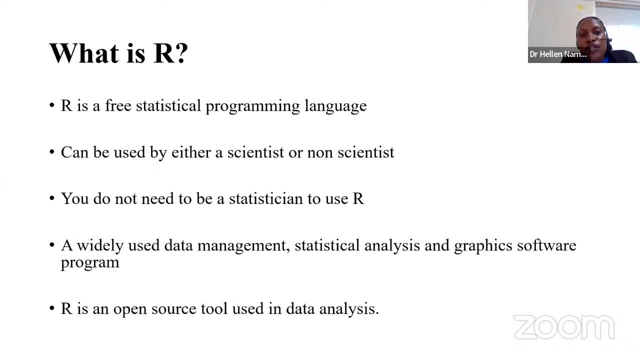 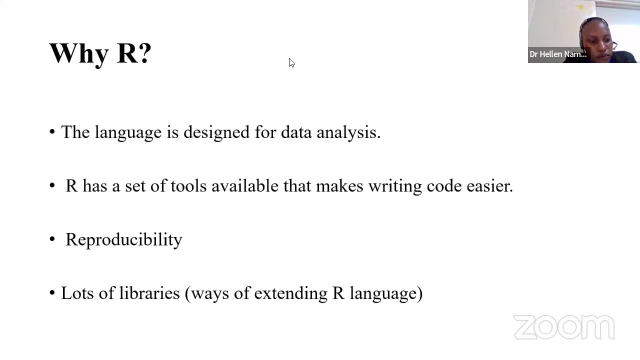 on your computer. you don't need to be on internet all the time because you read, you have already um, downloaded and installed it and all that is all that you want. so, um which one? I have a challenge, um and kindly post your questions in the q and a. a lot of questions are coming in, but 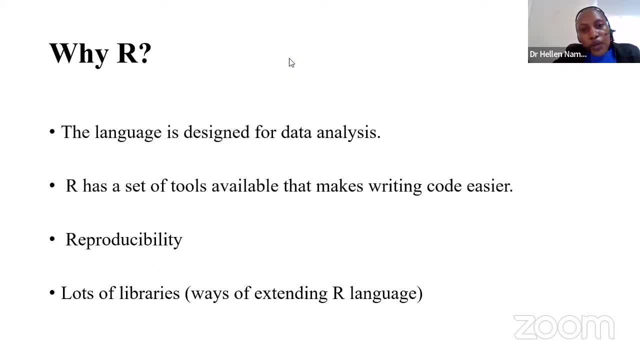 put them in the queue and it's like that, um, we are able to guide you quickly as we move on. uh, git is asking: what's the difference between r and r studio? okay, we are get. we are going to get there. please. which one is for windows? um, like I explained, or when you 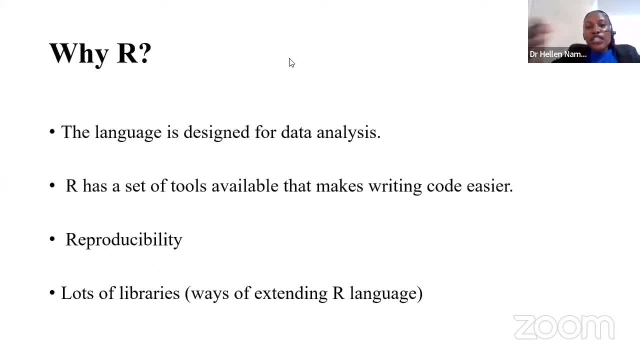 check. in the pdf that I sent, everything is clear that, in case you've got windows, in case you've got linux, in case you've got a mac, what do you do? okay, and fiona is saying that three minutes remaining to complete download. okay, so maybe, um, let me just take another one minute to try to to share now. 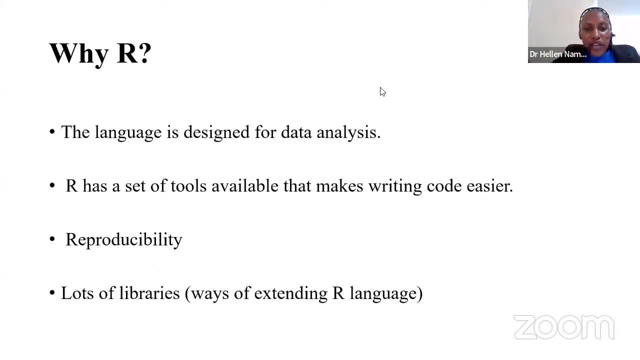 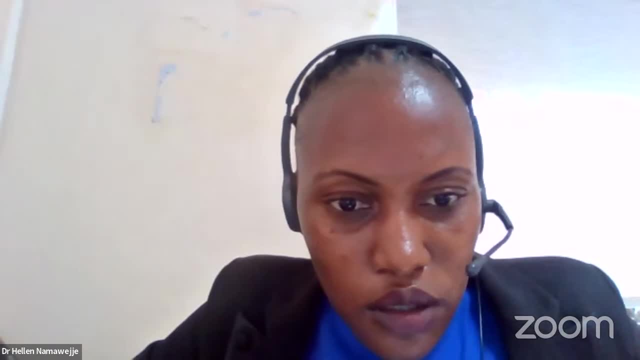 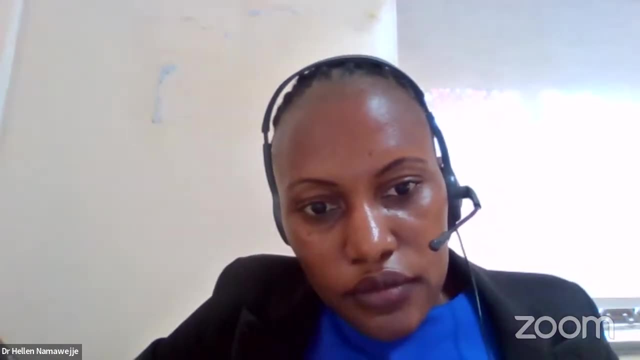 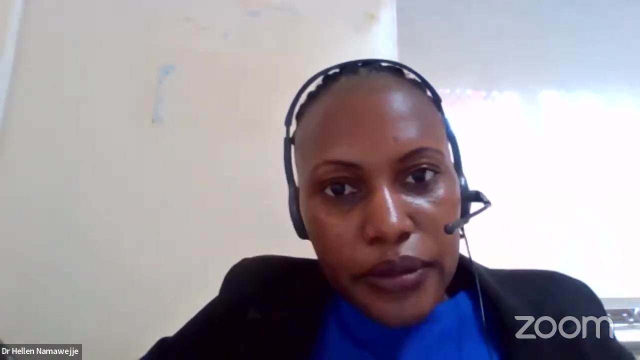 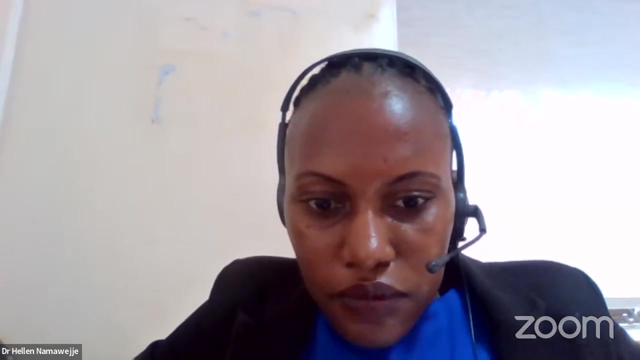 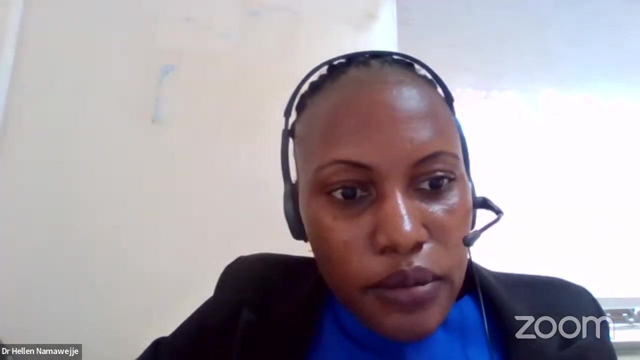 the pin to share the the pdf again and then I'll get back to the powerpoints. okay, um Así que déjame un segundo. I open it again and I share. yes, I'm going to answer that. okay, I'm using just um one minute to go through the things again. very, 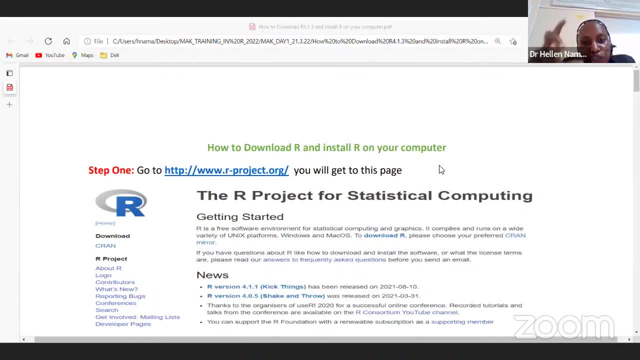 um, I'm going to answer that. okay, I'm using just um one minute to go through the things again very, very fast because I've already explained in details. It is important that, in case you're going to use R programming language, you have R installed on your computer, plus R studio. 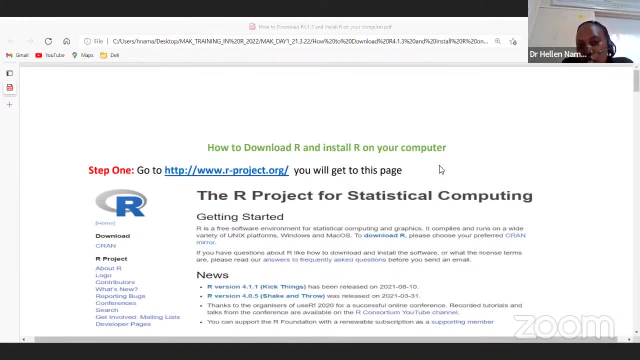 You need both. At one point we are going to see what is the difference between the two. So let's first get things fast. I say that there are some people with a challenge on how to download R When you check in the materials that we sent yesterday. okay, there is a PDF. 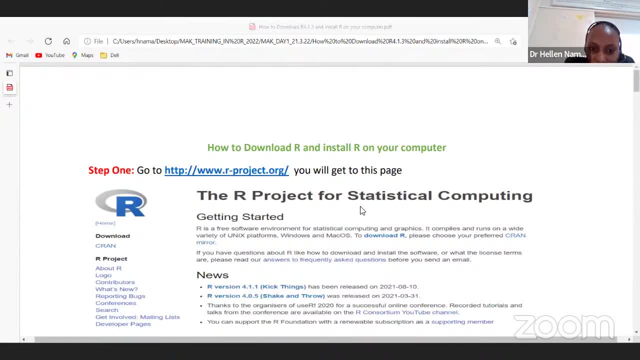 which I sent. that has got how to download R and install R on your computer. Like with the steps I took, all you need to do is to go to wwwr-projectorg. That page will open for you this, the R project for statistical computing. 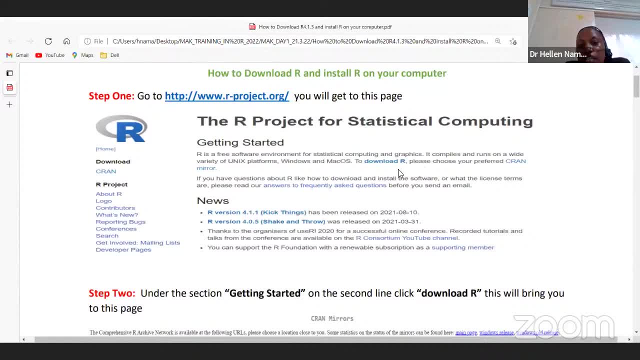 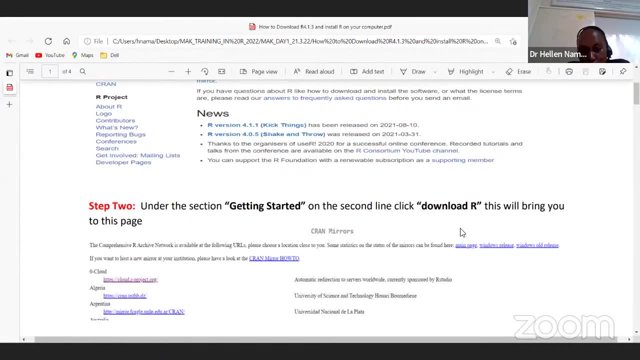 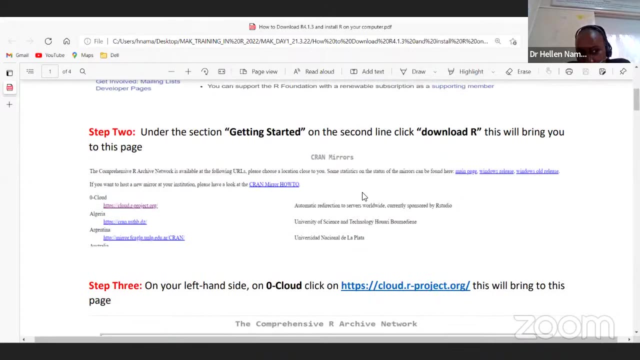 So, getting started, all you need to do is to click on download R. That is step number two. Okay, you need to click on download R. The moment you click on download R, you're going to see this particular page which has got the crane mirrors, And then you check on your right hand side. 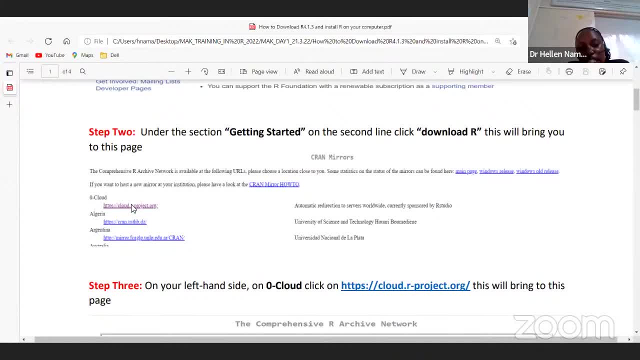 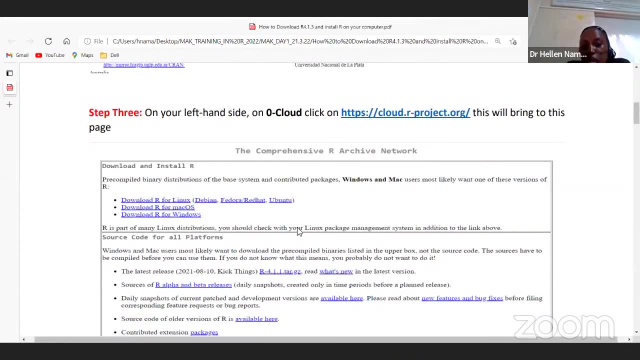 which has got zero cloud, And then you click on the HTTPS. If you click on it, what is going to happen? It is going to bring you this particular page: the comprehensive archive network. Okay, When you look at these three bullets up here, as you're following on internet, you're going to have 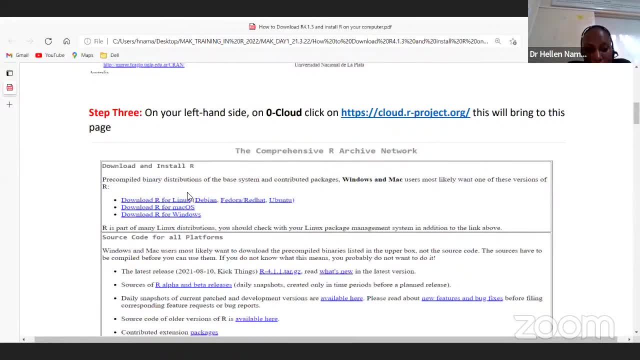 download R for Linux. download R for Mac, download R for Windows. So, depending on the version that you're using- I mentioned that personally, mine is Windows, So I click download R for Windows. The moment you click download R for Windows, what is going to happen? It is going to take. 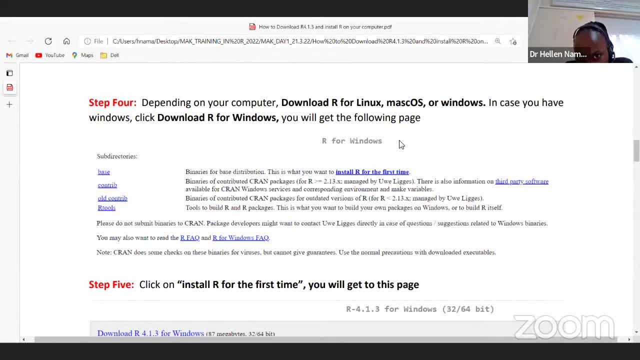 it is going to bring this particular page which has R for Windows. I guess if, in case, you click for Linux or for Mac, it will take you, it will tell you R for Mac. Here the page is bringing, that is, R for Windows. So what you do? you click on install R for the first time. And I say that 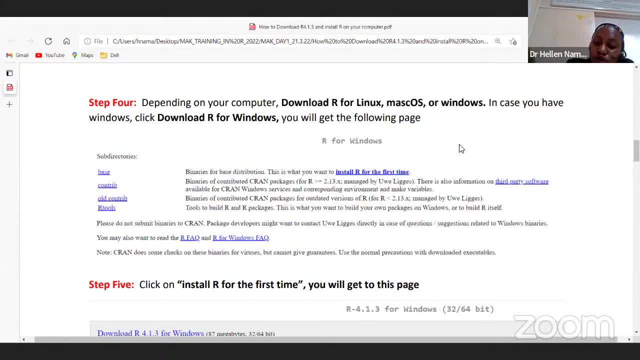 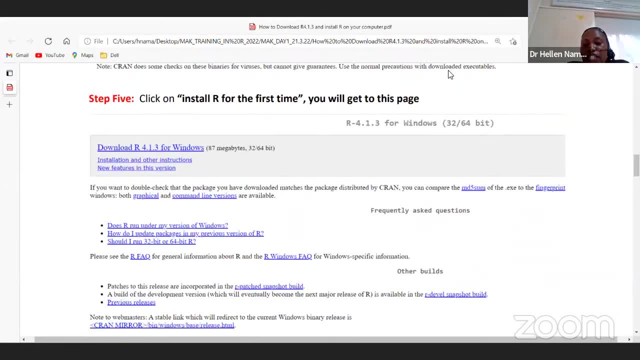 another option on how to update the package that you have is to click. it's to reinstall again to the newest package. So currently the newest package is R4.1.34 Windows. So all you need to do is to come and click download R4.1.34 Windows. If you click that, 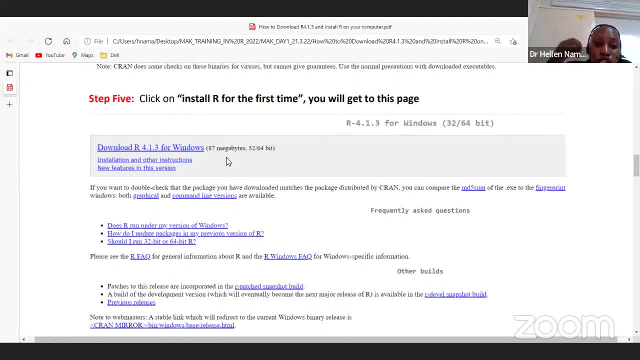 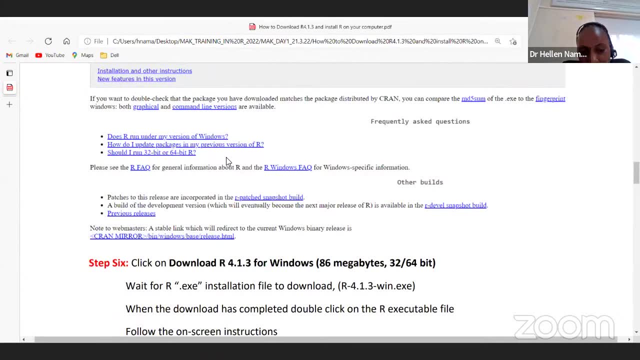 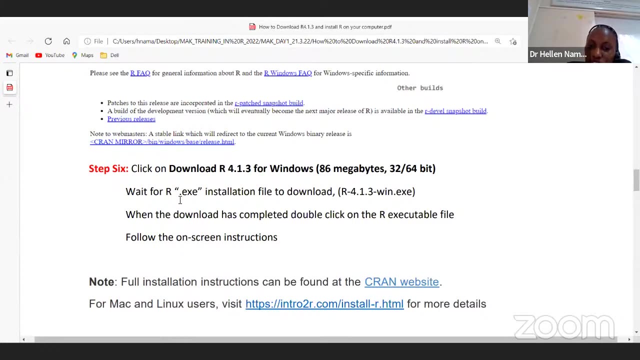 it is going to bring you an installation file And all you need to do is to follow the prompts and see that R is installed on your computer. Okay, So that is the last step. So the moment you get the EX installation file, which is when it's 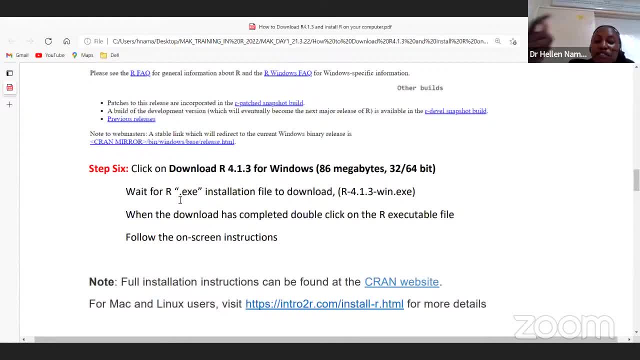 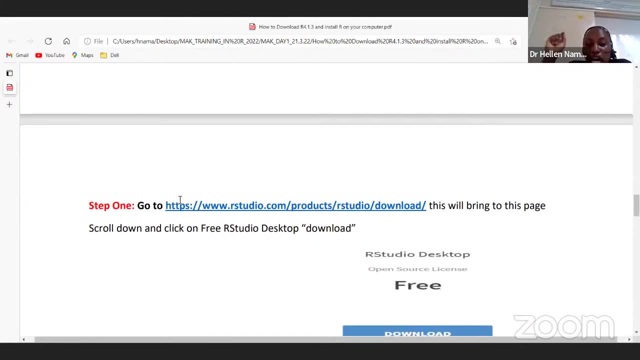 downloading on your computer. follow the prompts and see that all the steps that are being given to afford very well. How do we download and install RStudio? Like I mentioned earlier, this is the URL that you go to The moment you click on it. scroll down on that same page. 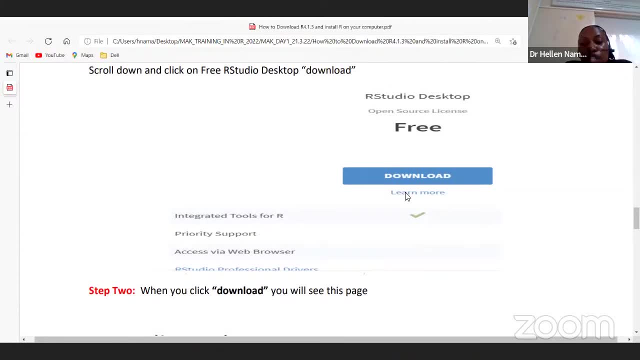 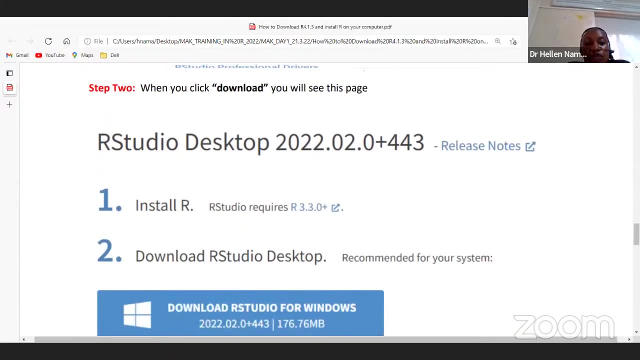 and then you will see something like this. And then you say: you click on downloading RStudio for free. If you click on download, this is what is going to bring you. You're going to see RStudio, the latest one. It is telling you there are two steps. First, 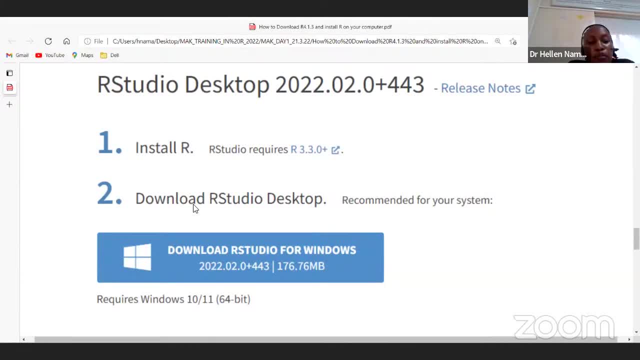 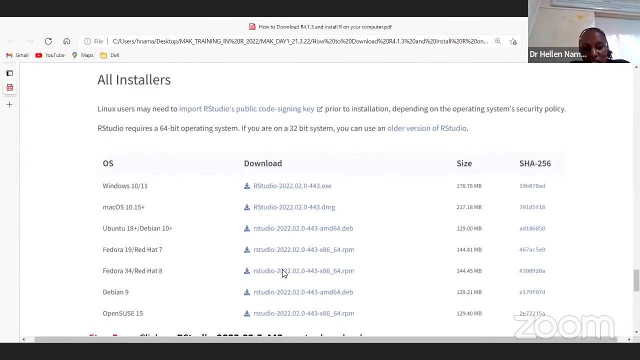 install R with a mentality that we've already installed, Then move on to download RStudio desktop. So if you click on download RStudio for Windows, what it's going to do- step number three- it is going to bring this particular page And all you need to do what is your OS? Is it Windows? 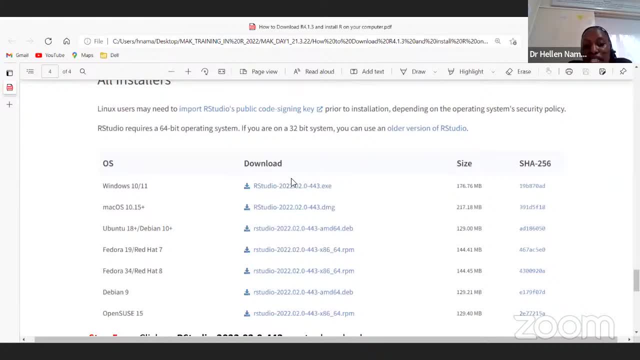 Is it Ubuntu, Is it a Mac? And then automatically you follow depending on the version of the computer that you have. If it is Windows, then you'll click on this extension: the RStudio- RStudio- 2022.02.2-443.443.EX. 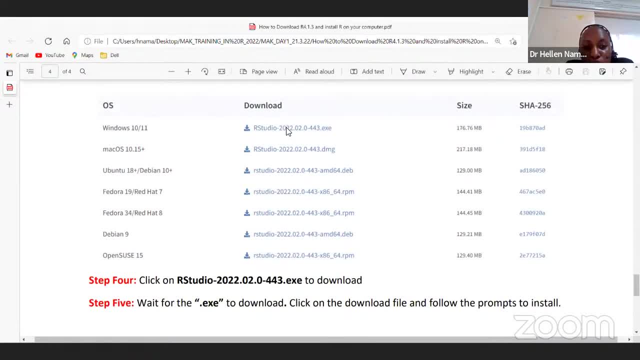 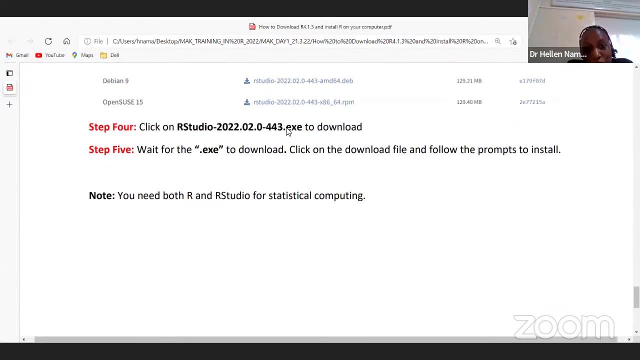 Okay, The moment you click on this, then let it download and click on the prompts as they come. After downloading, you click on the downloaded file and then follow the prompts to install. Basically, those are the steps, And you need both R and RStudio for statistical computing. 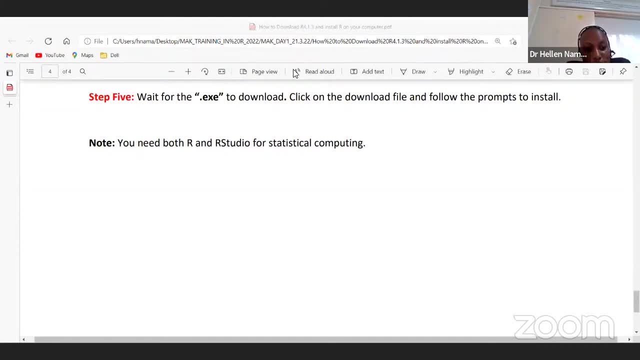 Okay, Let me check in the charts. So are we all in? Yes, we are. Okay. Let me check in the charts. So are we all in? Yes, we are. Are we all set? Okay? Pauline is saying that I've been able to download it both. 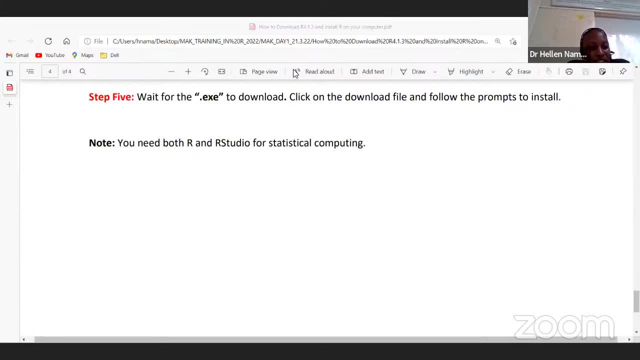 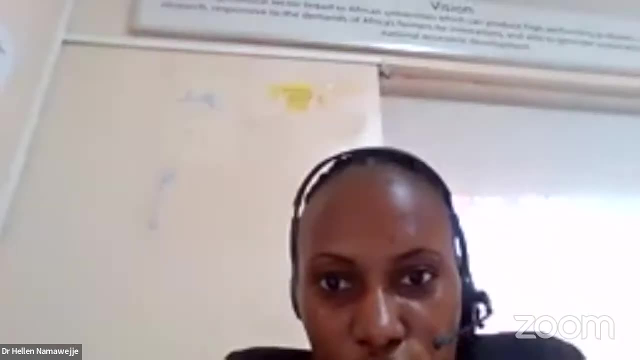 though I also don't have received the PDF yesterday. Okay, Okay, I think now we are set. We both have R and then RStudio. Great, Let's move on. I'm stopping to share that. Now I'm going to go to the next slide. 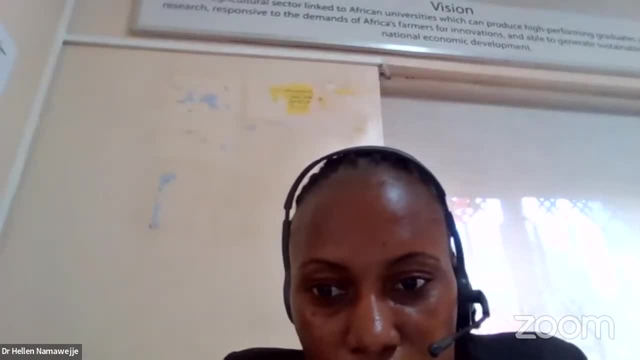 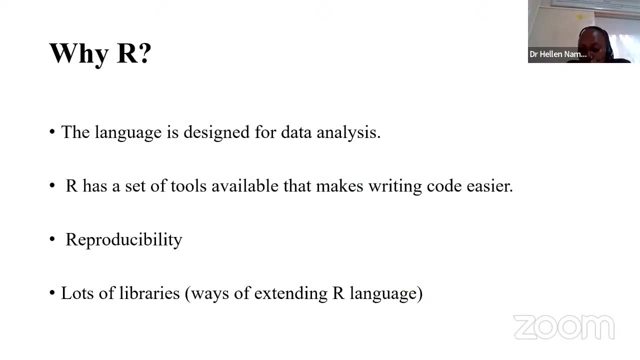 Now I'm going back to share my slides. Okay, So we're still continuing- YR. we've just seen on the previous slide, we just saw what is R And now we are saying that YR, And what is most important is that R is reproducible. 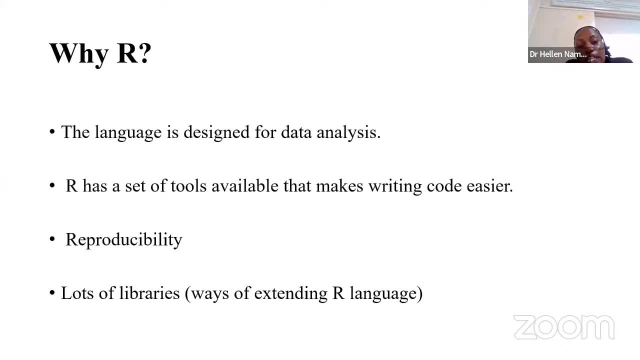 implying that the codes that you use in one project you can be able to reuse them in the next project. What is important here is that the moment you understand what exactly you want to do, because most of the things that we're doing in analysis you have to import data. 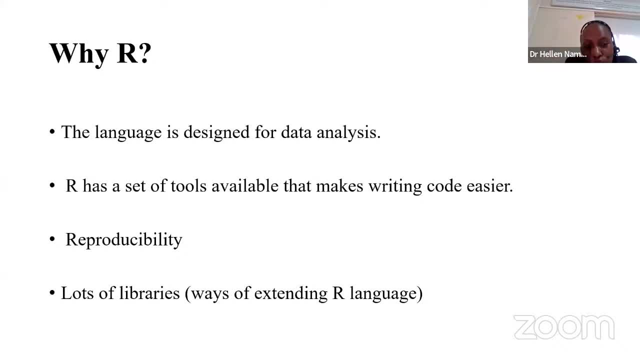 the moment data is involved. after that, what do you do? So within R, it is easy for you to set the tools available that make the coding easier. In that particular sense, I'm saying that the codes that can be used in one project can be reapplied in the other. 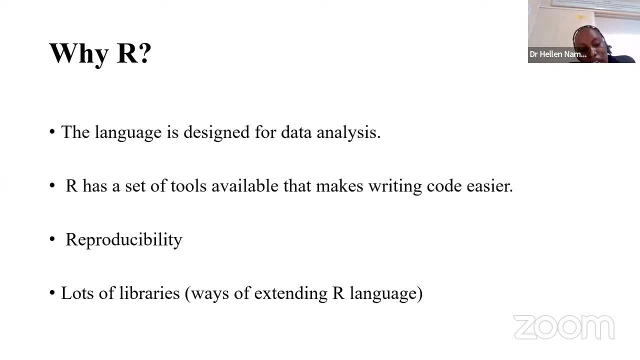 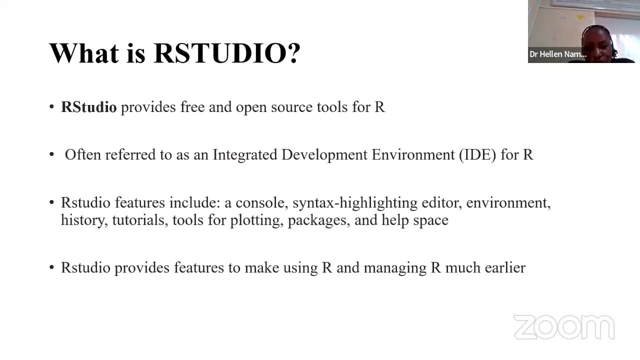 That is the point of reproducibility, And it has got a lot of libraries that can support you during your analysis. There's a question that was: what is the difference between R and RStudio? And we are getting there. So what about RStudio? 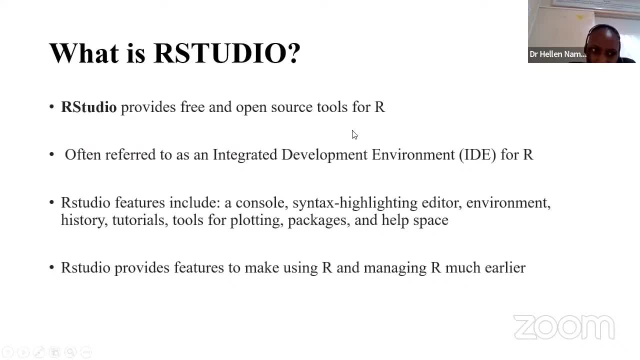 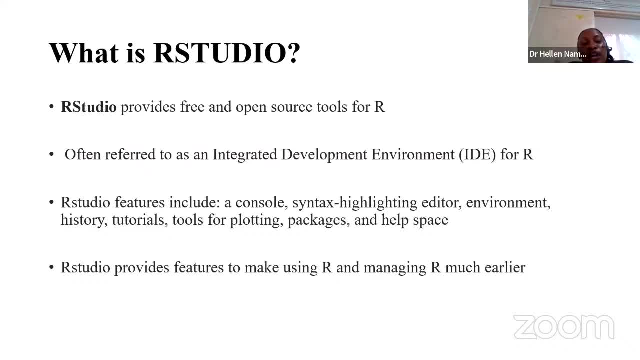 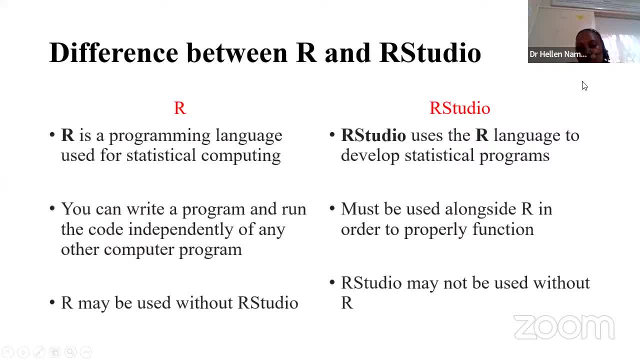 So what is the difference? We need to understand the difference between the two such that we are able to appreciate why we need to use R and RStudio. we need to install both of them. So, number one, I'm saying that R is a programming language used. 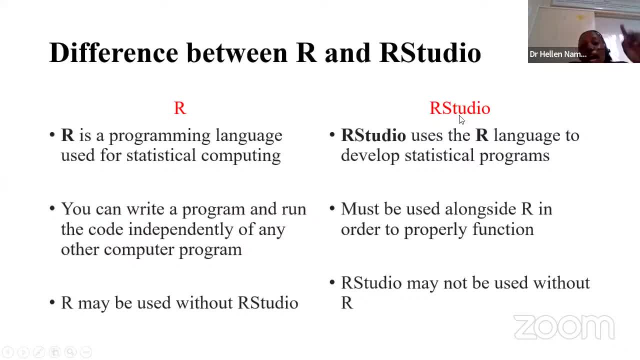 for statistical computing, But R studio uses the R language to develop statistical program And then the other one is within R. you are able to write programs and run codes independently of any other computer program, But you need R alongside to use R studio. In other words, 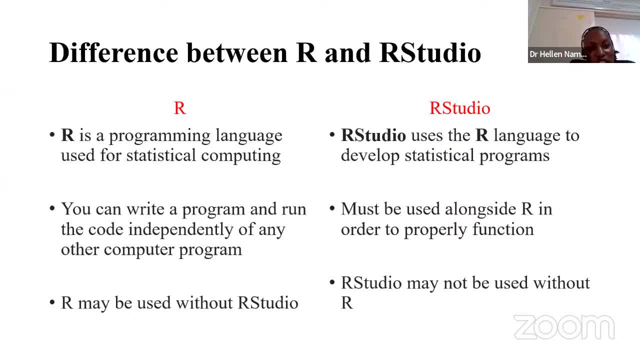 R studio cannot be used without R. yet R can be used independently without R studio, But we're going to see what is the relevancy of having R studio and R at a go, And then R may be used without R studio, but R studio may not be used without R. 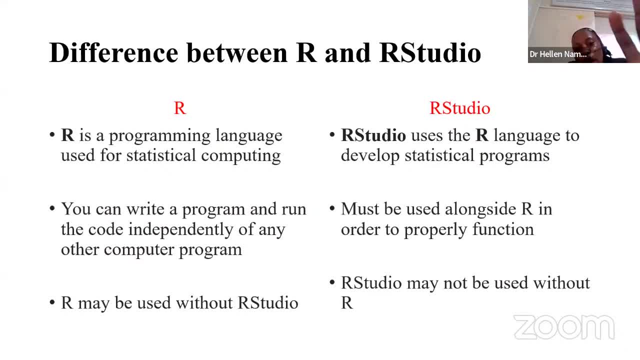 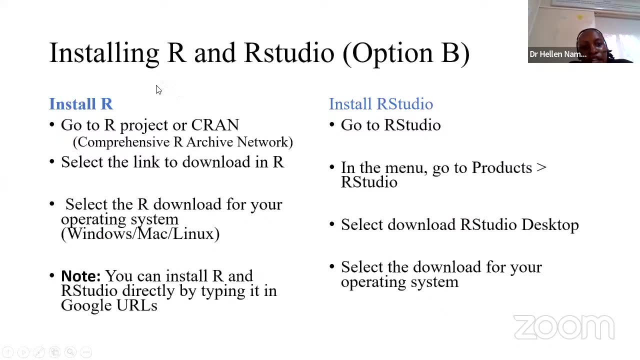 Within R studio, we are going to be able to save our codes. All the codes are being saved in R studio And then the output or the results are executed in the R console. Okay, so I talked about installing R and R studio. Of course, there are various options that you can. 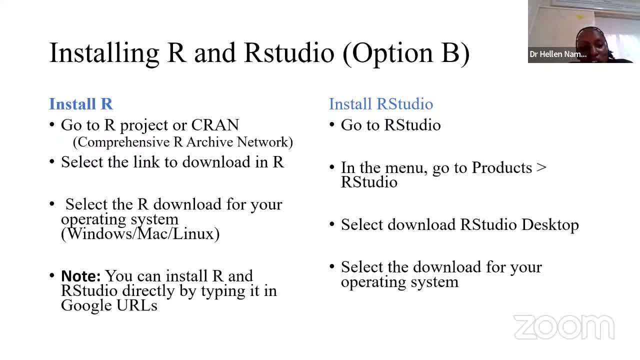 use. Okay, these are other options, But since we already have them, I'm not going to look at that Now, the moment you, the moment you have them. I'm not going to look at that Now, the moment you, the more. 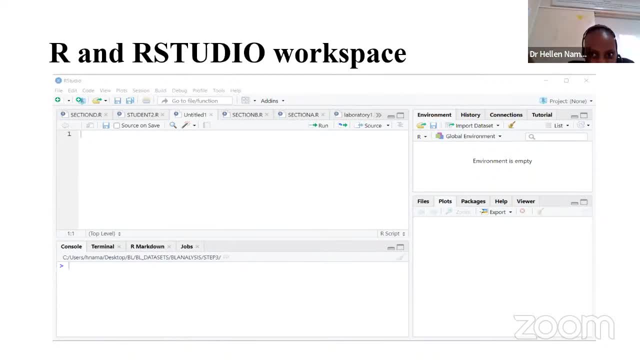 the moment you the more after installing. after downloading and installing R studio- the first the workspace that you need to see- it has to look like something like you're seeing on my screen, If both have been installed successfully on your computer, the moment you click on R studio. 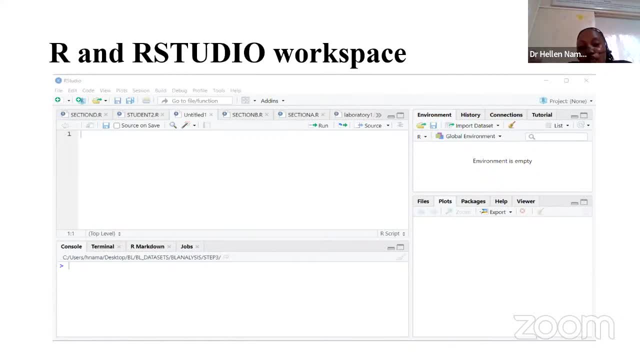 you should come up with this particular workspace which has got four windows. it has got this one here where I'm putting the cursor, then there is the one which shows that the environment, then down here where we have the file, plot, packages, help and view, And then we also have down here 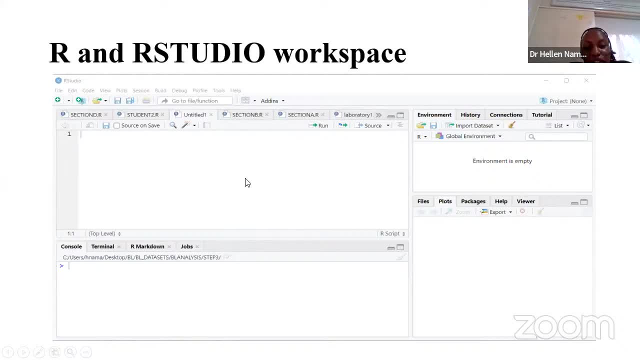 which has the console. So let me ask you the chance, in case you click on on on on your R on R studio, your computer, do you come up with such a workspace that I'm showing you? Okay, Um, yes, Yes, I'm still downloading, Okay. 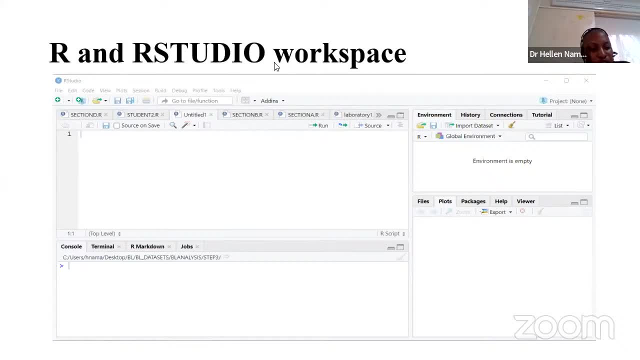 Please click on R studio and see if you're coming up with that the first time. I have three windows. Okay, That is okay. We are going to see how do we get the four. Yes, it looks like that. No, mine is a folder. 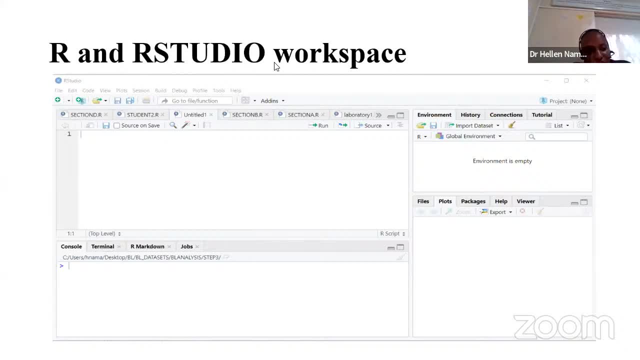 Sure, Yes, Okay, Um, there's something that I've got: three windows that is. I know why you're seeing the three windows, so we are going to see how do we get the fourth window. Jesse, finish saying that mine is still installing. Yes, though I still have 4.1 downloading the newer. 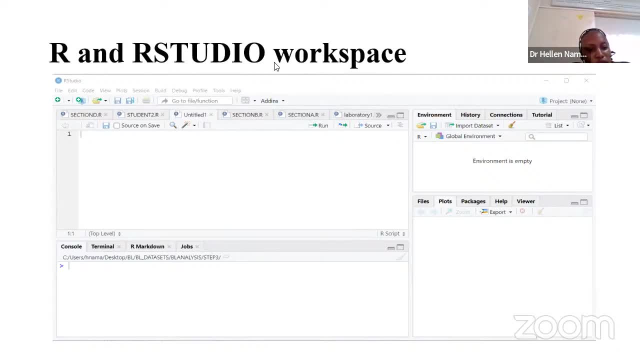 version. Okay for Windows. Fine, let's continue. So we are going to see. we're going to move on to details later. It could be why some people only it the ones that are sharing that they're not built in source files. 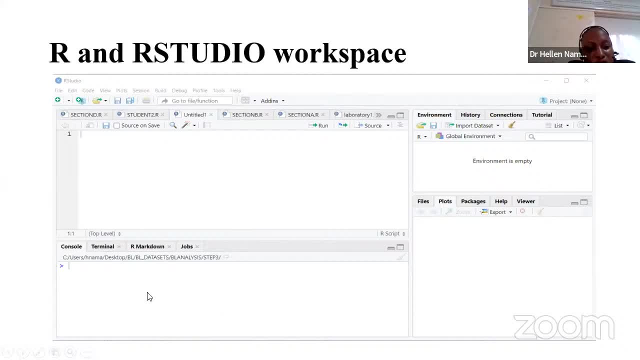 sharing that they have got three windows. it might be you're having the this window down here, the one of the r. what you're seeing down here it is the r console where our codes will be executed, and then up here we've got the r studio within the r studio. when you look at this workspace, it's where we're. 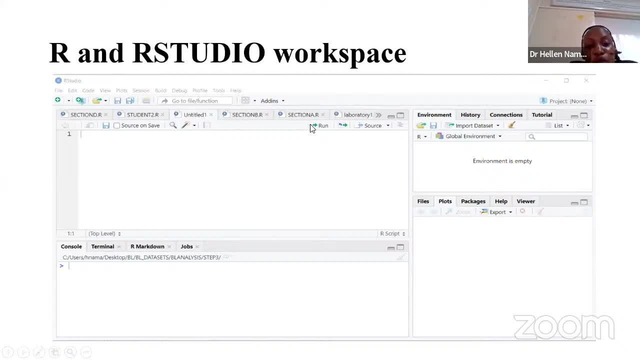 going to be writing all our codes, we save them and then we will run them and the output will be seen in the r console. then this side, we are having the on the right hand side, the upper window, where you you're seeing environment, whatever that you you're performing, all the data set that you've imported. 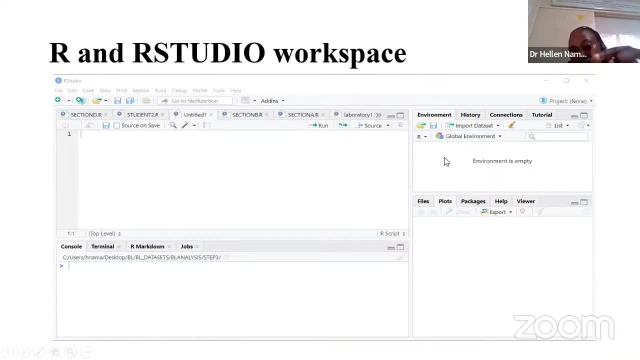 into r, you'll be able to see. you'll be able to see them stored in the environment. okay, and then down here you'll be able to see your plots. in case you're running upload, you'll be able to see upload. you'll be able to get various packages that you want, in case you. 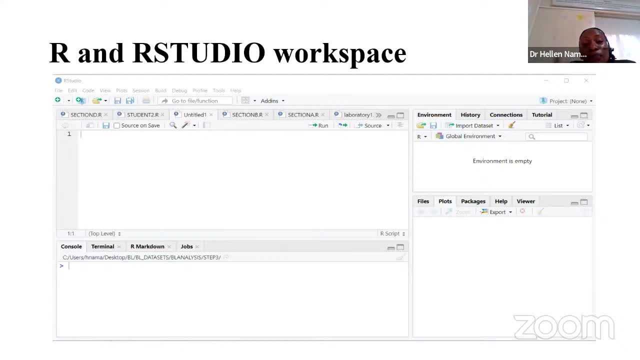 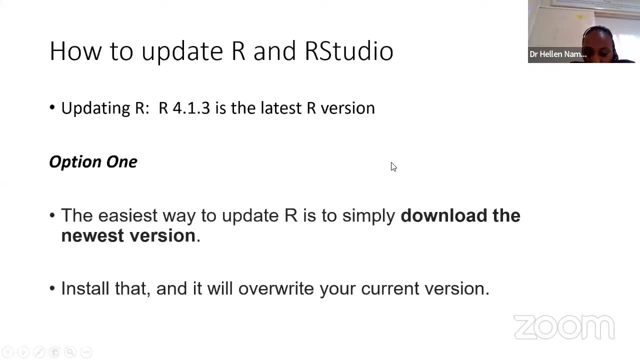 need help. ours got inbuilt commands that i can support you to understand the package more and also you can be able to to to view what you are doing. okay, so let's move on. how to update r and r studio. like updating r. like i mentioned earlier, r 4.1.3 is the latest r version. 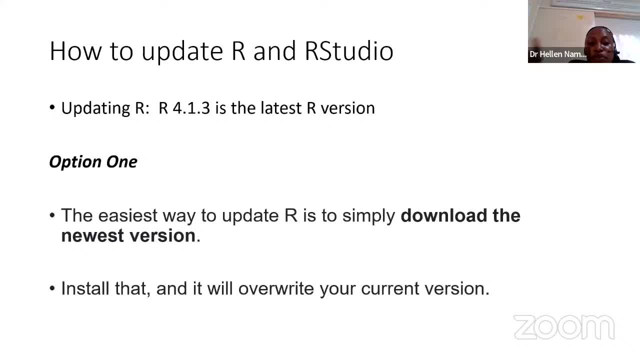 how do we do it? option number one: the easiest way to update r is to simply use the r as a method for updating the r, as an example. so i'm going to show you a simple way to update r. as i just mentioned earlier, r4.1.3 is the latest r version. how do we do it? option number one: the easiest way to update r is to simply use the r as an example. 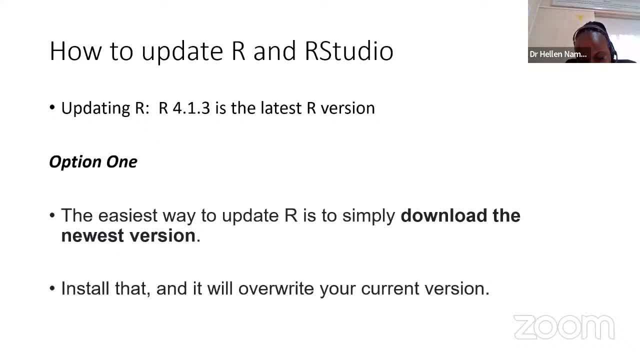 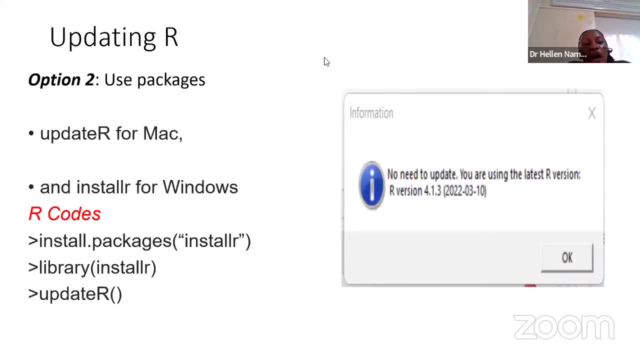 download the newest version. okay, that is one of the the quickest, the quickest ways. what does that imply? the moment you download the newest, it is going to overwrite the old one with the current version. okay, now the other one, it could be, in case you want to, in case you want to update and 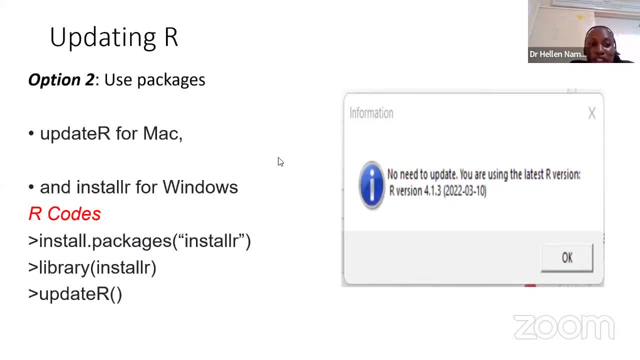 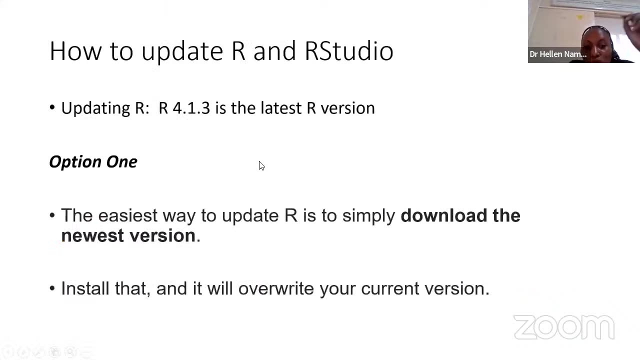 you don't want to download to, to go ahead and bother yourself with downloading the newest version. option two: what are we going to do it? but it works in both ways. open your going to your r studio, maybe? uh, let me go back a little bit. i'm talking now to people who have got r already, because when 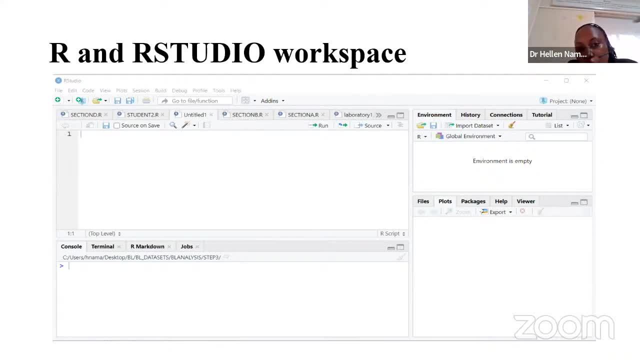 i talk about our studio, my mind tells me that at least they know, because they have got the old version. so when you open your r studio in the first upper on your left hand side, the upper window, okay, where i'm putting the cursor now here, it's where we're going to type our codes. 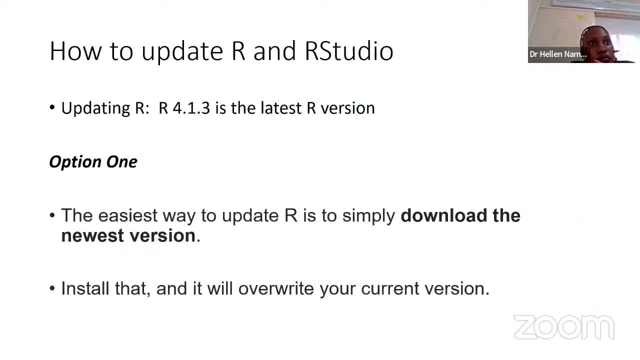 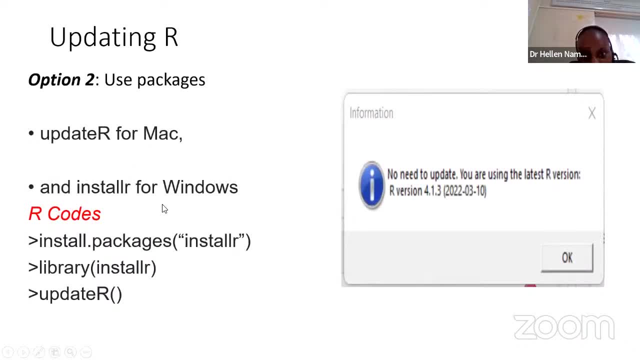 okay. so what is happening? going to your r studio? okay, and type in these three commands we are having. we need to first um install packages. installer r: okay, in case, installer r. you already have it in your r studio. okay, and type in the three commands we are having. we need to. 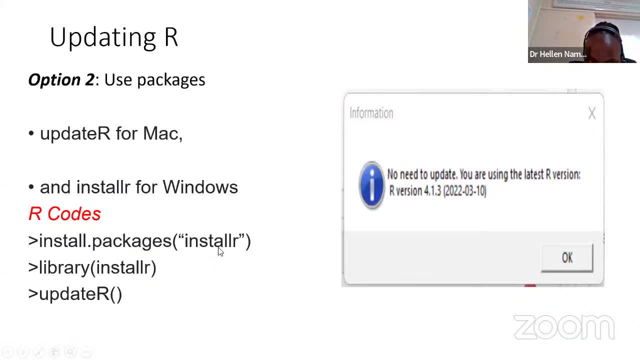 install the package. in case you've already installed this particular package, all you need to do just go and load library. you type library okay and type in the bracket you put installer. install r. the moment you run that particular line, the next step is going to be update r at the end. 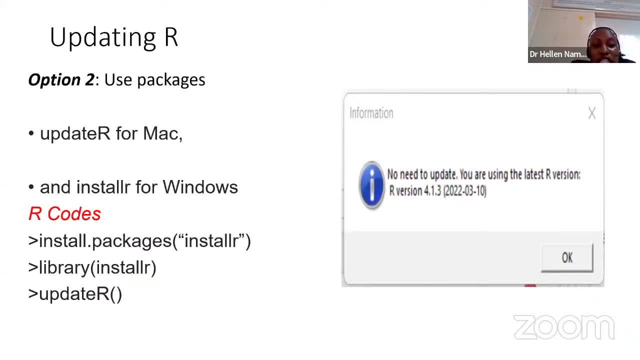 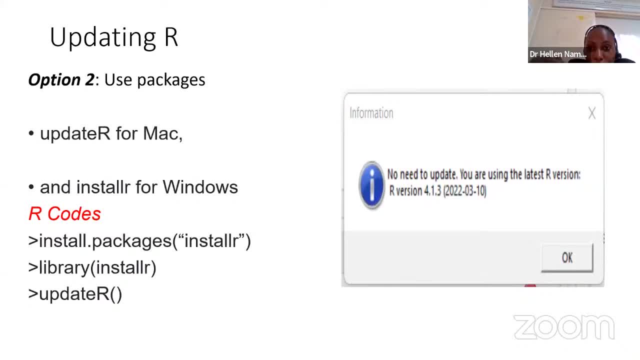 installed, so you're going to have the package installed, so you're going to have the package codes run successfully, What you can do. you can restart R again And the moment you restart R again, it will tell you. now, when you check in the R console, it will show you that you're using. 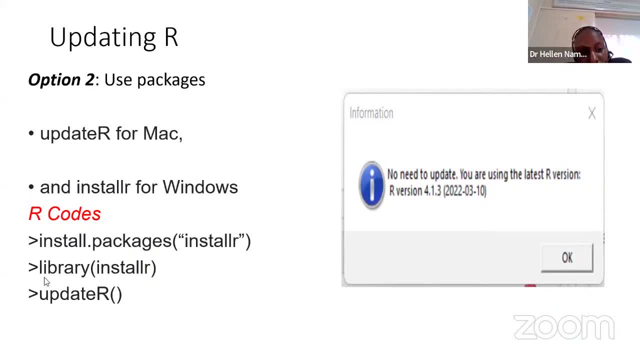 R version 4.1.3.. Like for my case, I also updated the newest version. So when I was trying to check again, this is the window that you have to get. If you're using the recent version, it will tell. 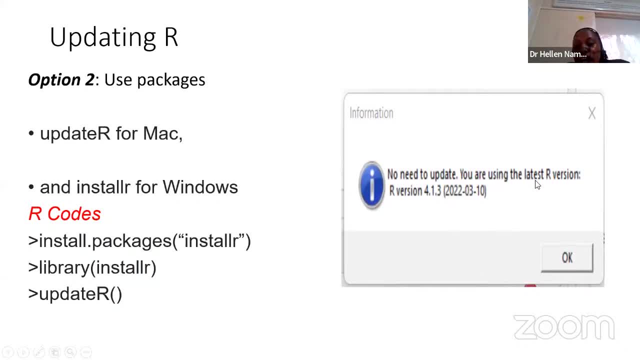 you no need to update. You are using the latest R version, which is 4.1.3.. And it will give you the date. This is the newest. It was updated on 10th of this month, So let me give you just a. 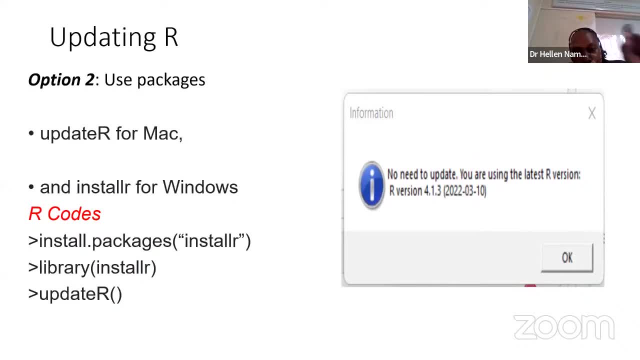 second- And I check in the chat- that go to R studio. In case you already have installer on your computer, you don't need to install it again. Just load that library, Click library, install R. Then on the second line after running the first one, 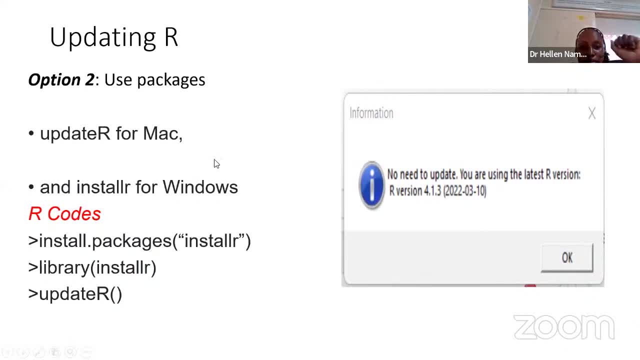 update R and check and leave it to run. Okay, Muhammad is saying that, so please record the session. Don't worry, All the sessions are being recorded And in case you miss out something during the training, you'll be able to check on. now You're able to check on the session. 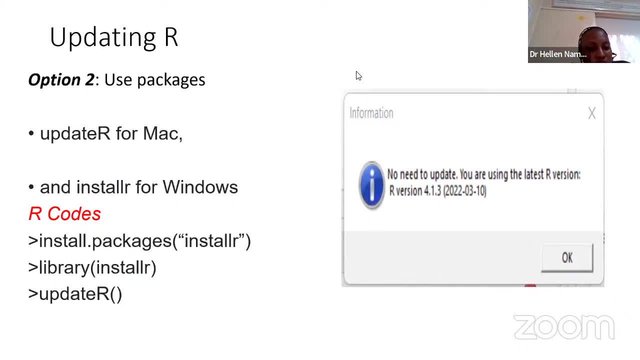 So back on the second line and then on those two columns, please check through the那個 webinar, Check through them in the webinar, the recorded ones on YouTube. Make sure they are Credits That are in your video or the public. effectivement, I only have one window. 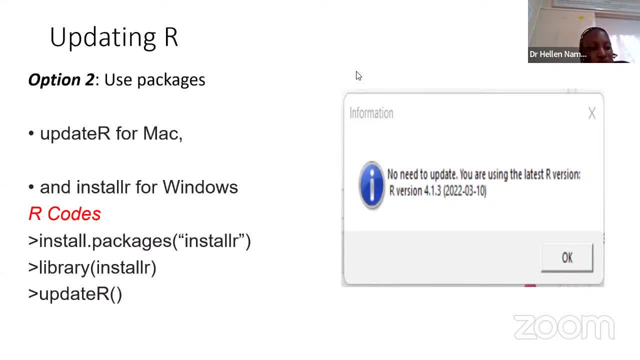 Please, you can still do it in R alone. I'm left behind. I was there for about a second, But I guess I couldn't help it. I expected that to happen to packages. What will happen to packages, I don't know, Okay. So okay, you can do that. adjustments after. 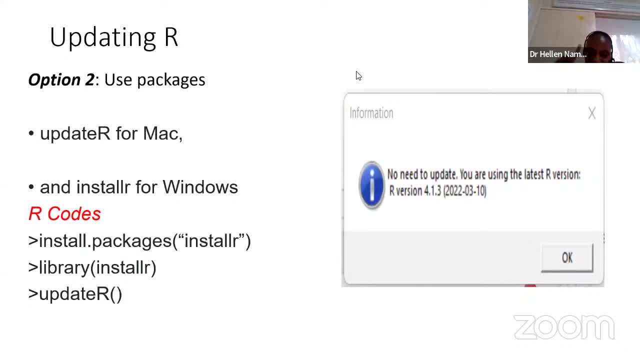 that, And when you pay $14 of money- and again I thank you very high $15 because at policymakers are a- it is updated. Of course, I will still tell you right with you updated to the new version, In this case today. this is still right. By the way, if you show them, editor components, can you see? 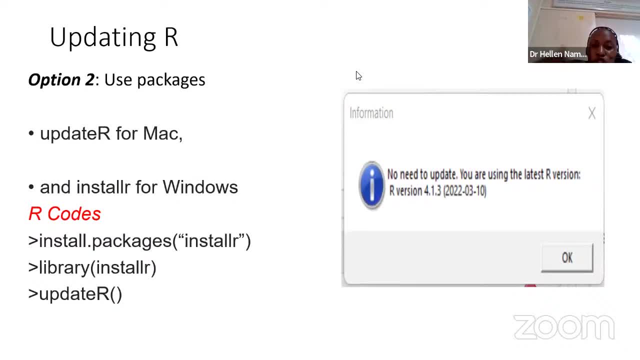 Now you see that there is version you're going to, as you're updating, to ask you: do you want to update also the the old packages? all you need to do to type yes, that you need also the packages to be updated. but of course, there are also other ways on how to update the different packages in our studio. um, hello, i can. 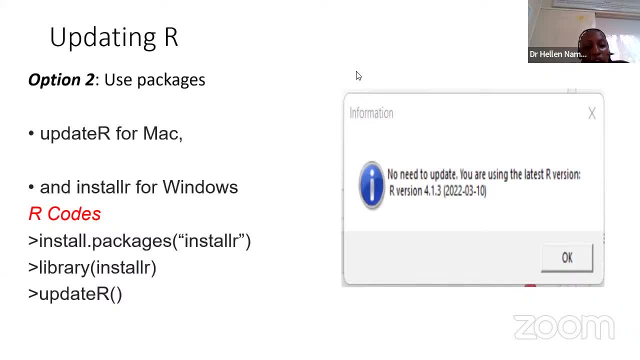 only see one window when i open r the one. when you're seeing one window, you clicked on r alone. click on r studio. r studio is integrated within r, so it will come automatically with the, with the, with the, you'll have um the r studio window, you'll have the four workspaces i'm talking about. 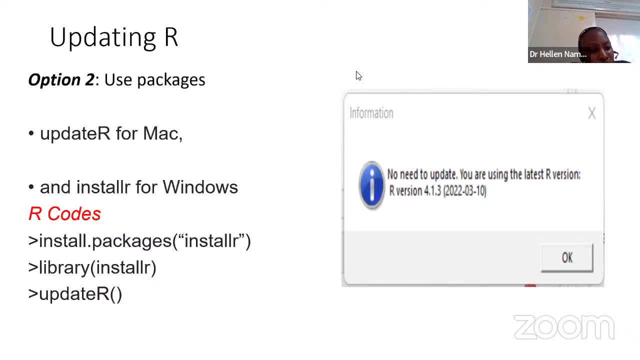 kindly post the questions in the q and a. please repeat the step to click again the step to update. i only possess the console mandat. still, within the console you can type in, you can, um, you can, you can write in the codes that are that are being uh, shown on the on the powerpoint and then, uh, you run them within the console. we. 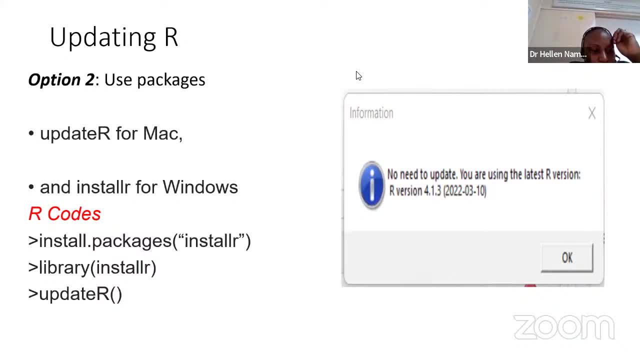 just enter within our studio. we click the run button after installing. i could not see the r and r studio on the desktop environment. please type in your get in the search window and and write our studio. the icon will come. if i download both r and r studio, it means 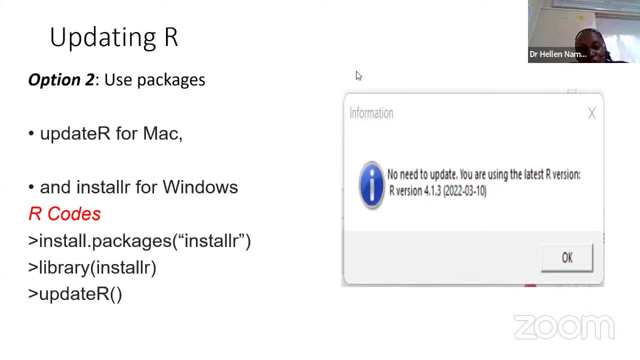 no sign of updating. um, okay, so, um, right now we are working on our, our browser. i'm going to show you the browser. uh, i'm going to show you the browser. you see the browser, the output now, the mode. i'm going to show you. i'm going to type in the word for the browser. i'm going to type in the word for the browser. 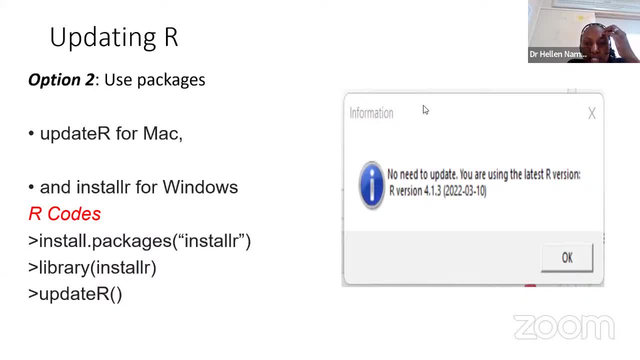 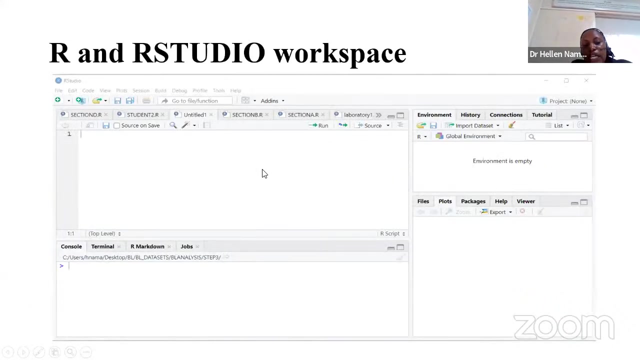 are trying to to give some little time to people who are updating their pack, to updating our and our studio. i go to our shortcuts and neither of them gives me the three, the three parts version. okay, um, maybe let me take just a step backward, in case you've got only um three windows, or three. 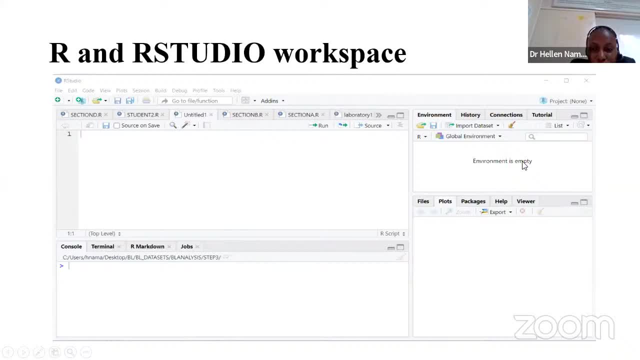 spaces, meaning that you have the r console and then you have the environment and the and the and the- this other window on the right hand but on the bottom. all you need to do just go up and click on file the moment you click file and then ask for a new one. i thought i'll do those. 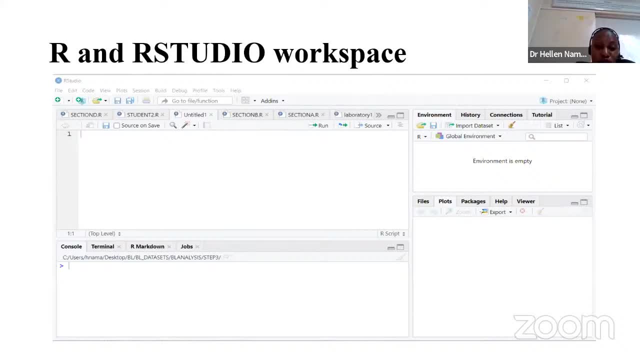 steps as we start, then automatically you'll come up with the fourth window. just go to file. then from file you'll click new script. let me first. let me first check in the chat. if you said, then i can practically go and open. okay, now this one. i said yeah, it has. my questions are not being answered. 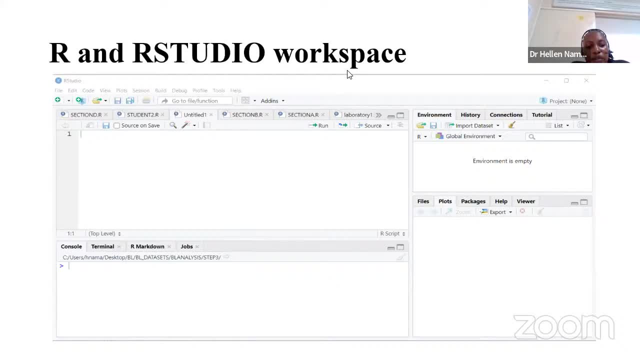 okay, um, just the one who abel. just type no if it is asking, directing you to where you can. i have now gotten a few windows, thanks, um, just go to file and then ask for a new window, ask for a new script. you'll get the fourth script, okay, um, okay, let me briefly, uh, stop sharing the the. 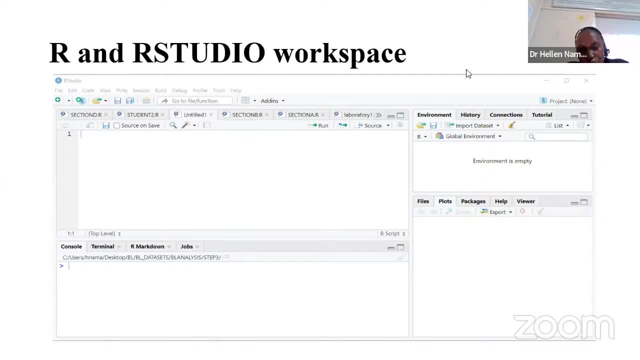 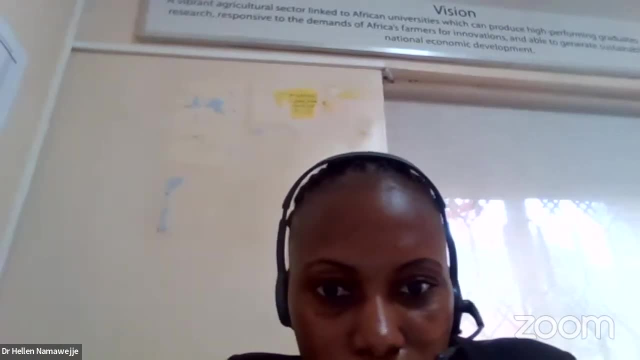 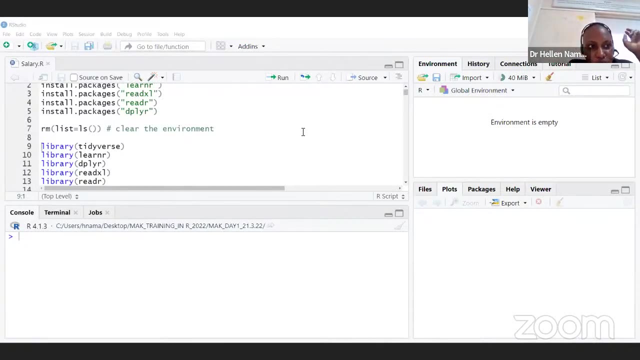 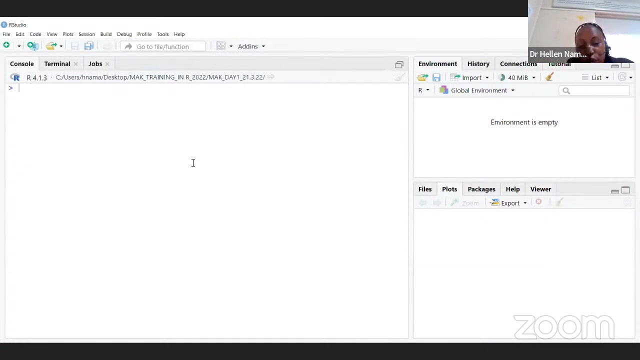 my powerpoint and i get to our studio. just briefly, then i'll get back, okay. okay, now i'm sharing my r studio. this is what i was talking about. um, let me close. people are having i seeing my screen. now i'm sharing my r studio. i'm also having only three screen, three windows. 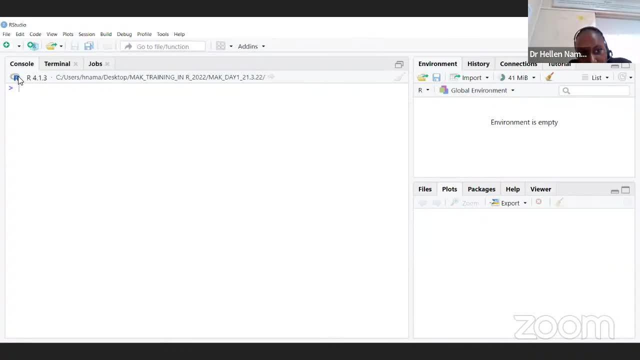 i've got the one of r and it is showing me that i'm using for r 4.1.3. i'm finding some kind of three button days- that is the latest version up here. i'm having our studio, okay, and then when i look this particular side, it is telling me environment is empty. 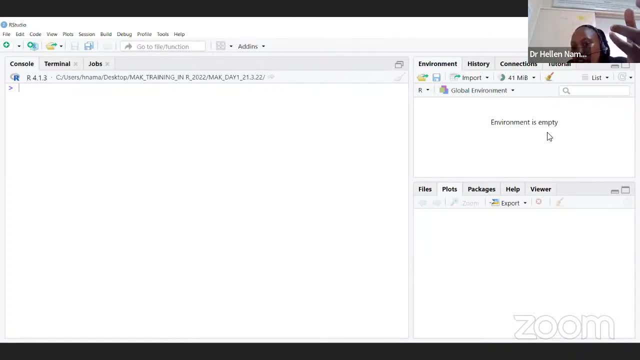 okay, so i've not put anything so far. this is the other windows telling we are going to see that whatever information you create in r, it is being stored in the in the environment, and you'll be able to see whether you've successfully imported it or not. we are going to get there and then he's. 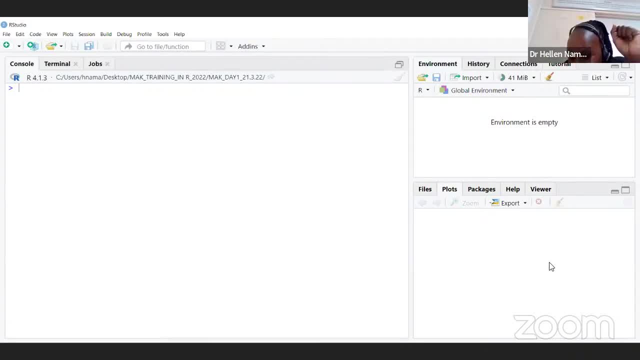 in this. in this other window where i'm putting the cursor at the bottom, where i'm here, we are seeing files, we are seeing plots- whatever plot that you will do when we get to data visualization, it is great. you're going to be able to see it here in this particular window you can click on. 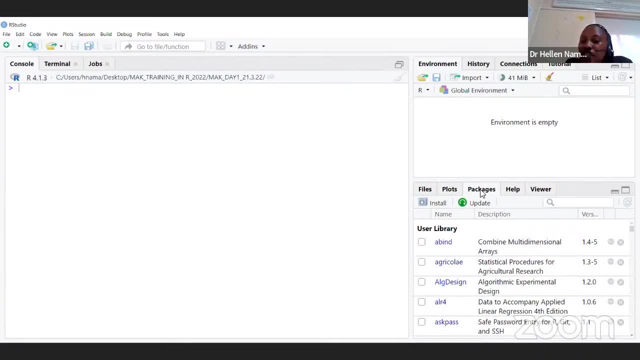 packages. it will tell you. still, some of us have been asking: what about updating packages? you can up the moment you you get to you download a newer version. it will ask you that: do you want to update the the packages in the older version? all you need to click is to tell. to tell our that yes. 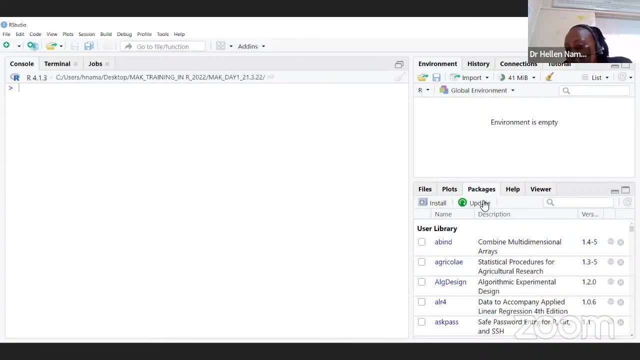 but you can also update packages from here. you come and click packages. in case you want to install a package, you can click install. or in case you want to update a certain package, okay, it is telling you that you check for updates. then you click on that. we also have the help window in case there's something, in case you need more information. 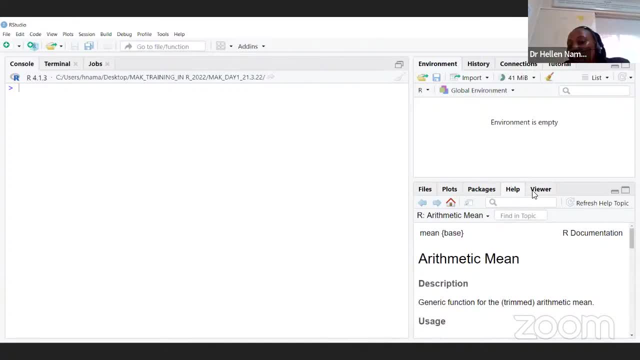 or something, how you do it. okay, and then, uh, so looking at the three windows that i have, somebody was asking how do i create the third one? just check what i'm going to do. just come and click on file. the moment you click on file on top of your r studio, then click on, move your and say new file. 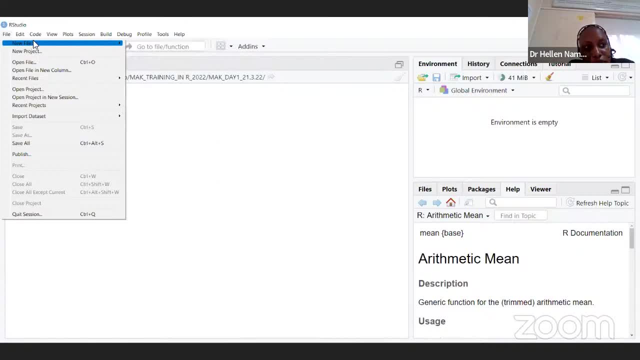 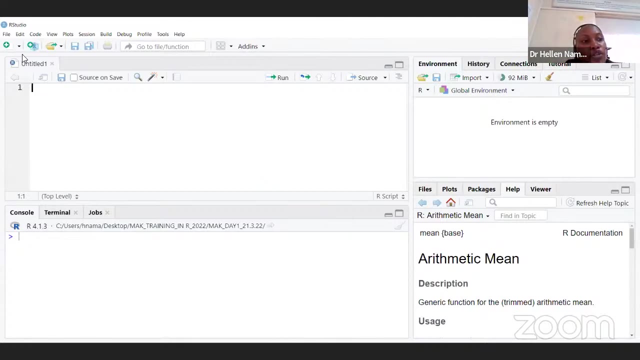 as you see the way i'm moving. then you move up to our script. the moment you click on that, it will automatically bring the fourth window. in case you see, that procedure is hard. all you need to do is click on where i'm putting. it is where i'm putting the hand. it is showing you new file. you can just click on it. 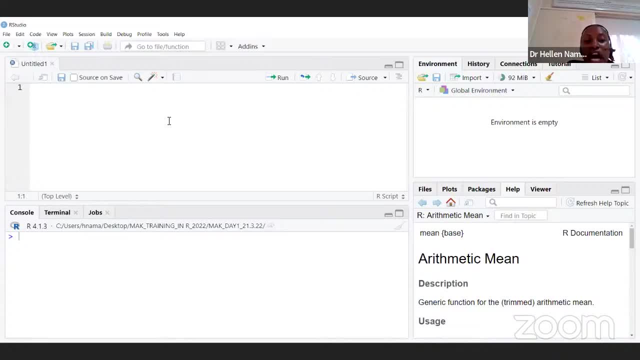 the moment you click on it, it will automatically open it and it will also bring a new, a new document, a new workspace where you can work in. so, like i said, this is in the up here, it is our hours, our r studio where you can write your packages, you. 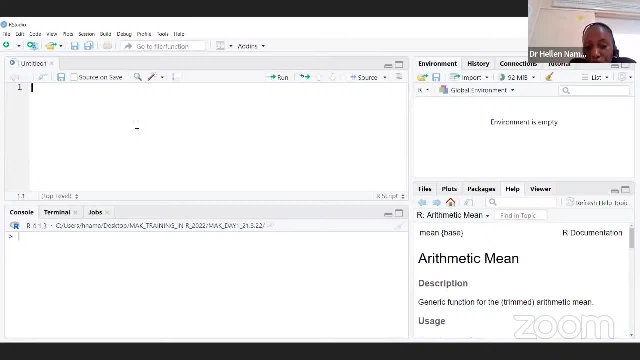 install packages. you write your commands and then you install packages. you write your commands and then we've got the run button. you're able to run all your commands. and the moment you run your commands, the results are being executed in the r, in the r console. whatever we do up here, we see the results down here. but, like i mentioned, 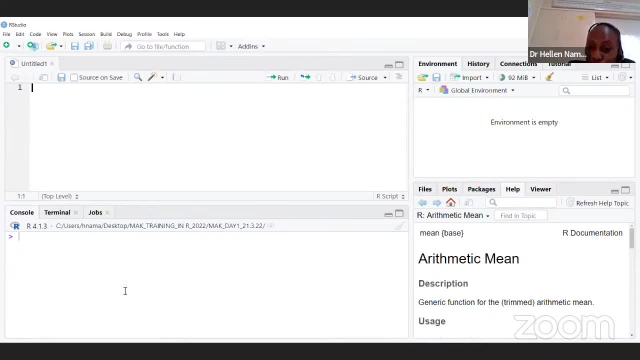 earlier. r can be used independent of our studio. you can also come and type your codes in the r console. but why we are interested in our studio is that we are able to save our commands and reuse them. reproducibility, which i talked about. we are able to save and reuse them again. so let me ask you: 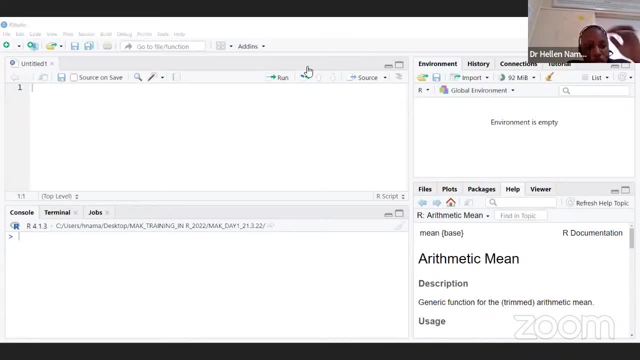 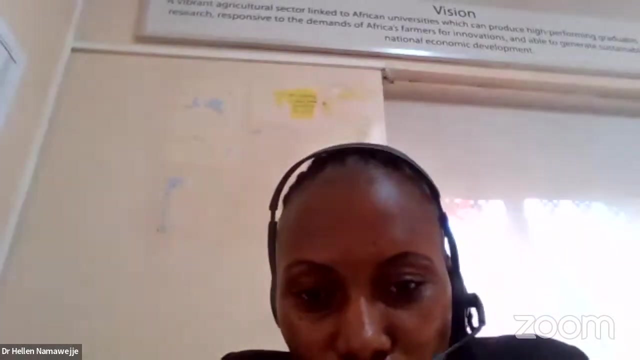 in the chat. is it okay now? um, kindly kindly direct the questions in the q and a. i was trying to read a certain question and then it disappeared, so which i think we are good to go. okay, fine, hope you've seen. uh, how now you get the full. 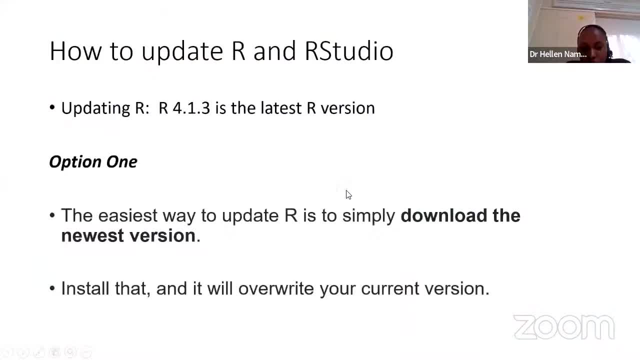 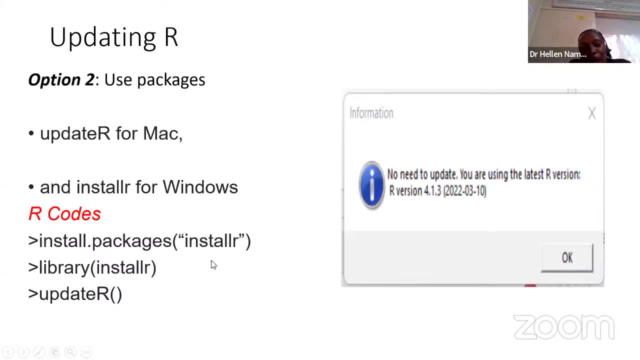 all right, let's proceed. so i'm skipping that. so, um, for those of you that wanted to update, i said, in case, um, you don't have the installer package, you need to install it. i'll. i'll talk more about installation as we move on, but i'm talking to people that want to update. 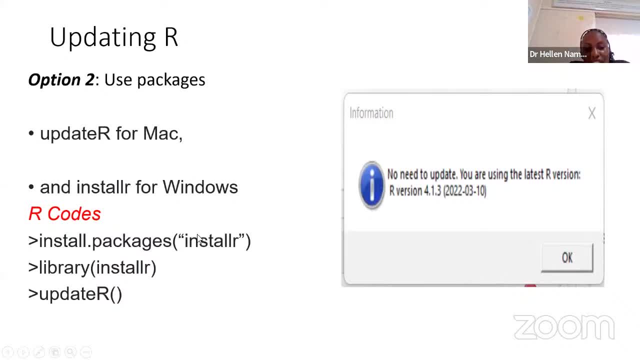 uh, you type the code is installed packages and inside the bracket, okay, you put quotes install r and then on the second line in the url console, okay, you type in library install installer, then you put updates r and then, as you follow the prompts, r should be in case after: after: um. 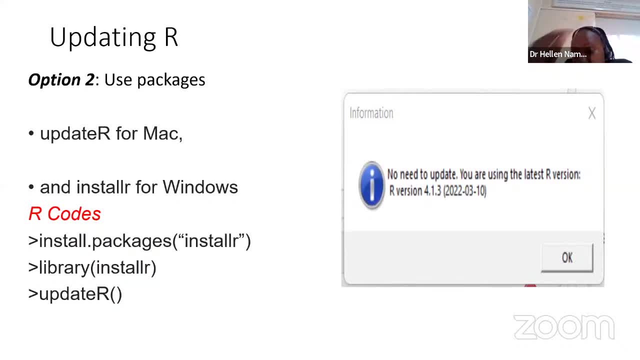 installing everything. if you're not seeing any effect, Restart R again, close that window and then open it again and check in the R console. Is it showing version 4.1.3?? The moment you see that, it implies that automatically now you're using the latest version. 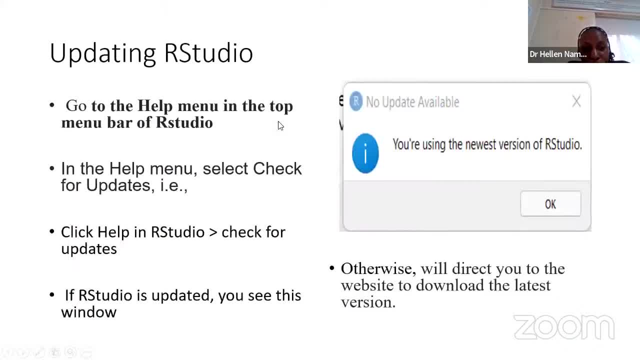 Okay, let's see When we move on. what about RStudio? How do we update RStudio? So, with RStudio, what we are going to do, we are going to go into RStudio, to the help menu in the top bar, and then we are going to click on the help menu. 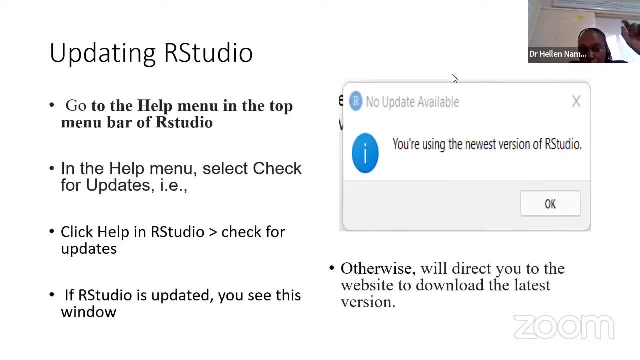 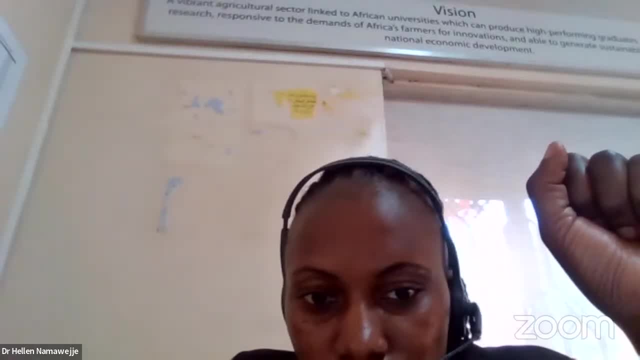 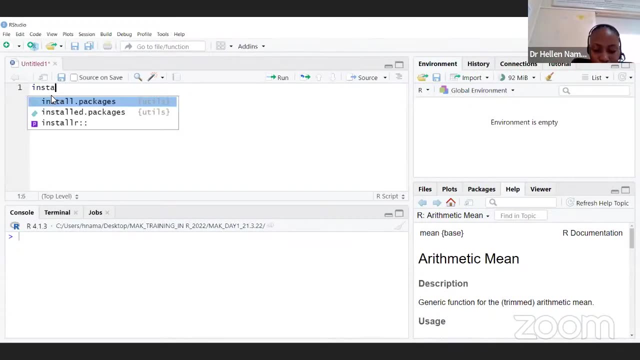 We click check for updates. Maybe let me stop here and I share my R again. Okay, all right. So for those who have been updating, we mentioned that you need to install install packages as our command, And then inside here I say that you put installer R, That is in case it is not installed. 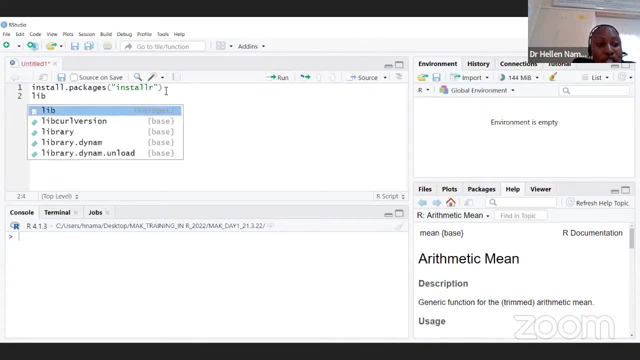 The moment it is installed. the next step is going to be to load it library, your loading installer R. I already downloaded it, so that's why I don't want to go through this particular step. The third step is update. it is update R. All you need to do is to run these particular 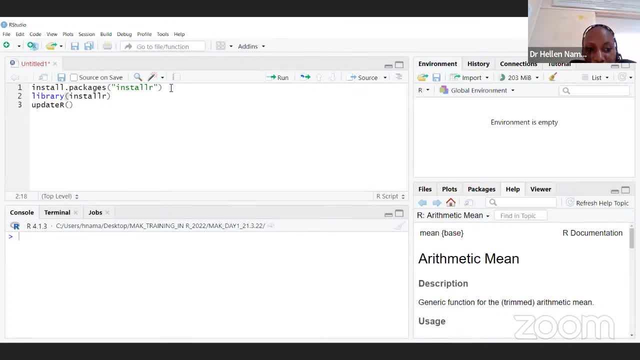 lines. I don't want to install it again because I already have the package on my computer. Then when you come to this library, install R. you just need to at the end of the line or you come to click on, you run the current line. 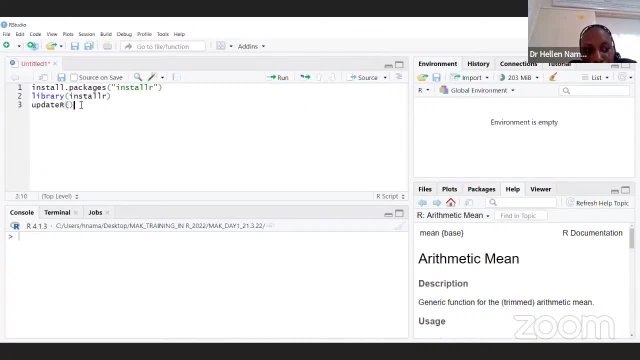 After running that, you come on the third line, You press enter, You put the cursor and then click run. The moment you run, you'll be seeing all the results down here. Like I mentioned, I'm using the latest, so I don't need to update. 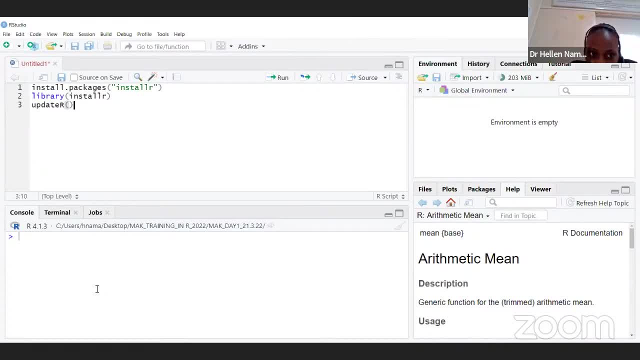 This is for the case of R programming language. The moment that is done. we've talked about RStudio. So under RStudio you come. how do you update RStudio? You come and click help After help, you come and click check for. 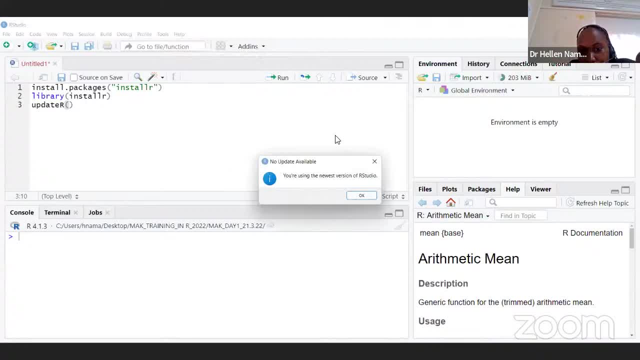 Updates. The moment you click check for updates. if you're seeing my screen, it is telling me that no update available. You are using the newest version of RStudio, But in case if it wasn't the latest version, it would have brought for me a script to direct. 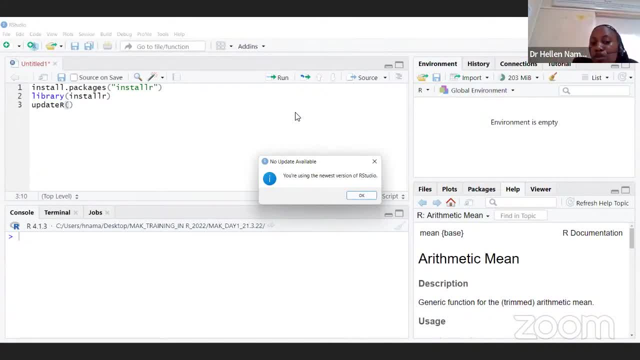 me on what to do Or, in case I had not updated it earlier, it will tell me that there is a newer version now of RStudio. Do you want to update? Then you either say yes and then you follow the prompts, or you say no. 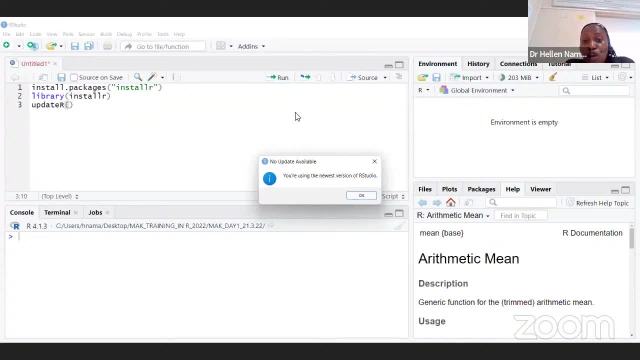 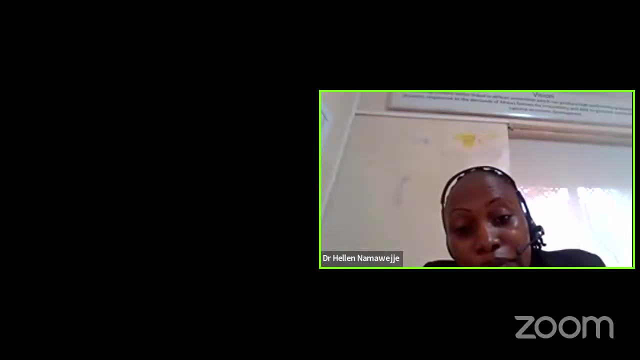 But for my case it is telling me that I'm using the last version of RStudio, So there's no reason for me to update. So here I click OK, because there is no effect of anything that I'm going to do. Click up one. 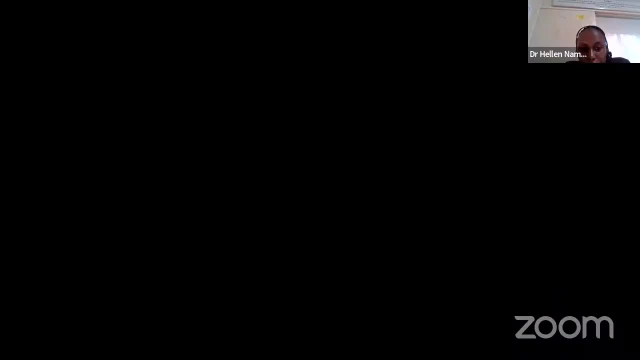 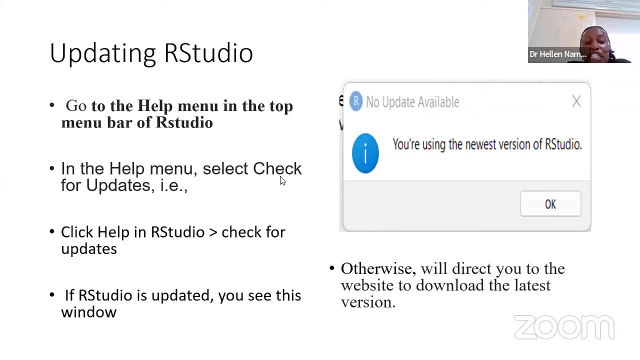 OK, OK, I'm sharing back. So when you go to RStudio, this is what it will give you: Go to help. Then click check for updates. If you're using the latest version, it will bring you this particular window, like what: 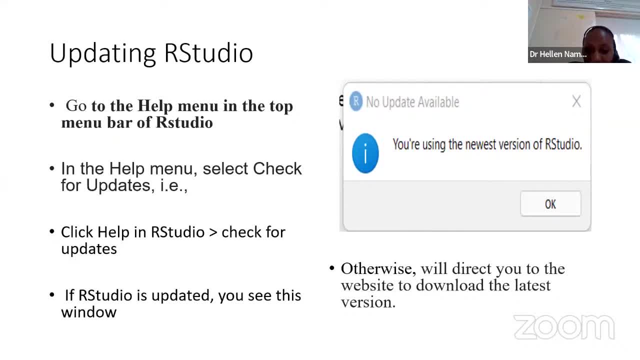 I've just showed you, OK, And otherwise it will direct you to the website on how to download the latest version On the other website which we used initially earlier on how to download RStudio. that's where it will take you. 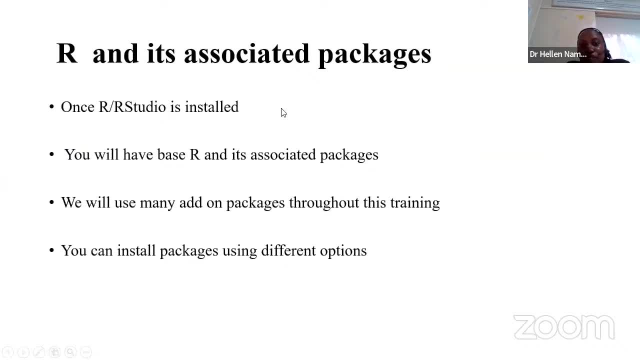 OK. Now let me ask in the chat those of you who are supposed to update R and RStudio: is it OK now? Have you been able to update? I don't know what that one means. Can I run the three commands once? 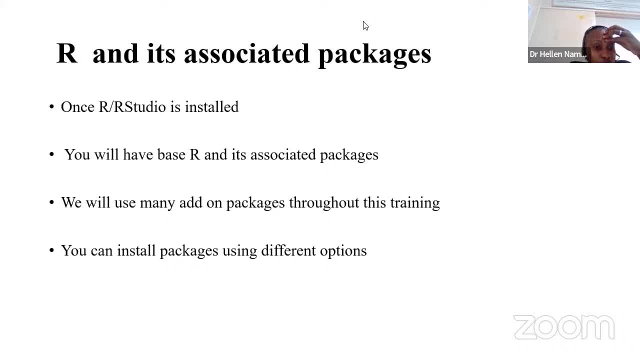 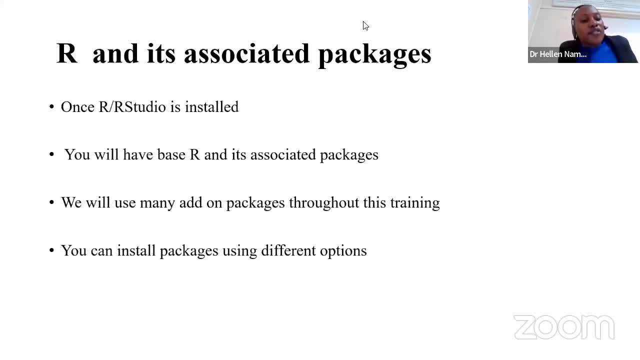 Could not come on. It is OK If you're having version 4.1.1,. I told you now for you need to update because we need the latest version. We are good to go. I have already installed the newest version. 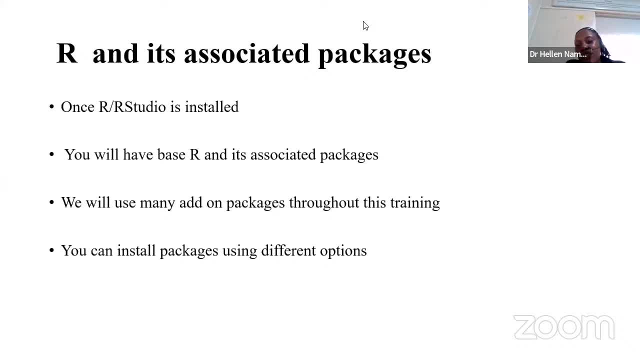 newest version. um, um, maybe i think that you have to note in mind is that uh? r is case sensitive. now somebody's saying that he's failing to install the. he's using package installer. it is installer. i mean, there is there is an error. you're typing in: i n s t a double l? e? r. 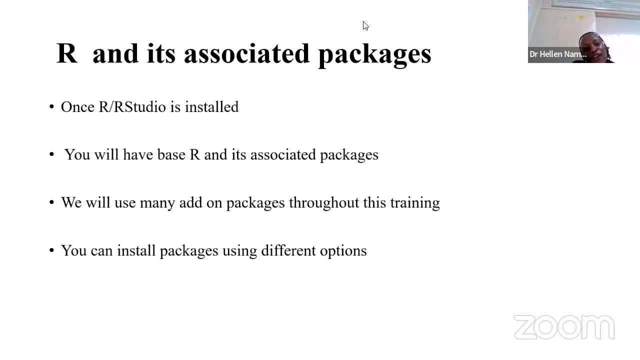 there is no e. that's why it is telling you that that package is not available. you're typing in a wrong package. it has installer r, not not installer with e. so that's the reason you're getting that error. it doesn't have it. um, great, andrew, i've seen that. 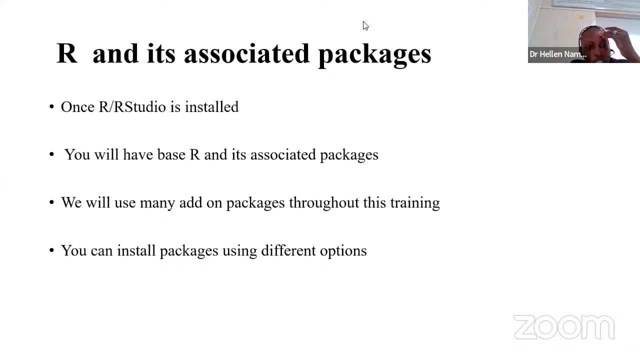 thank you. that's why i was telling him to follow you on how to update. all right, um Wycliffe, yes, also, that procedure can work. great, um Wycliffe has posted another way on how you can update our and our studio. thank you so much. like we like you. 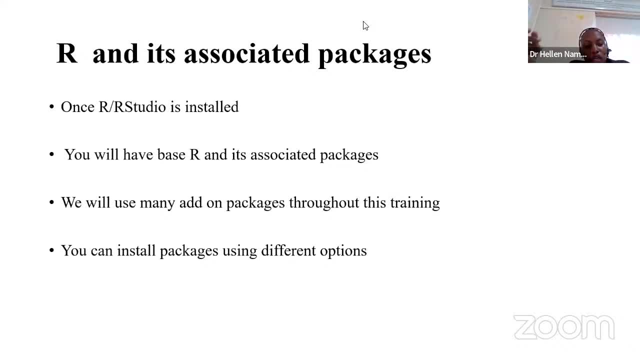 know sometimes um postman i'm. i'm giving you an answer why you're getting an error. please listen. why the why it is telling it's an error because you're typing in a wrong package. it is not installer, there is no e, it is n i s t a double l? e? r. that's why it is telling you that. 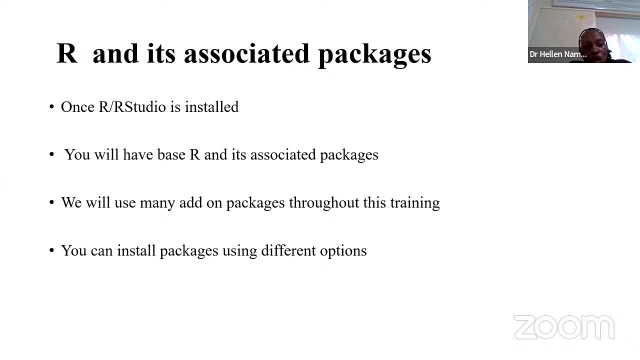 package is text, Carolina. do not say that: how many characters do you have? no, e it says base: yes, can you type it down again: 0. do not say that: okay, so can we. okay, that is great, so can we continue. okay, yes, steve, that is great. are in case you get an error. for example, it is because it is complained that he doesn't have that particular package. please Check the sparing, the sparing of the packet that you've typed in. maybe it is saying it's not whenever he would get a backup with unless he had those two. you, by by a menu, switch and do a start click. so keep this into account and leave this chapter until he is seems to care. 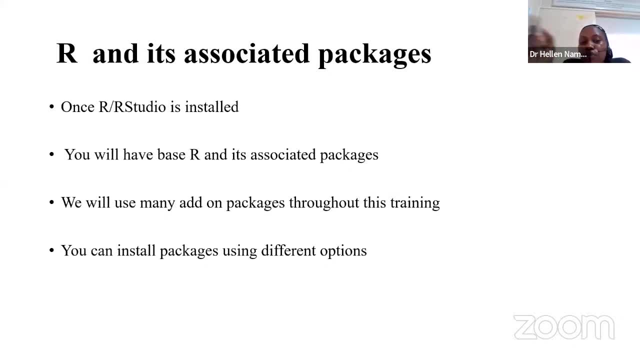 you know, because whatever you typed, it's something different from what R knows, So be very careful. R is case sensitive, So in case you used an A and then later used a capital A, those two things are being seen differently. So now let's move on to R and its associated. 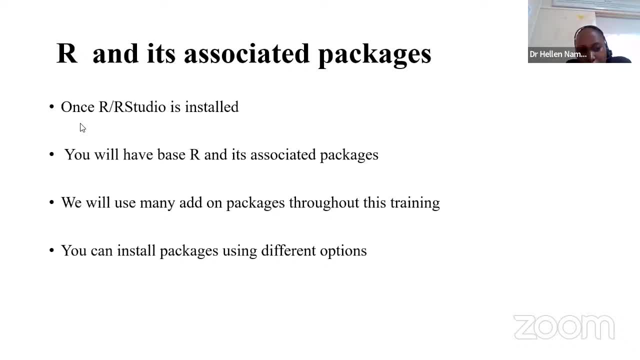 packages and see. So once R and RStudio is installed, I'm glad that right now we know the difference between the two. You will have base R. You need associated packages that are going to support you as you're doing the analysis. R has got million packages. 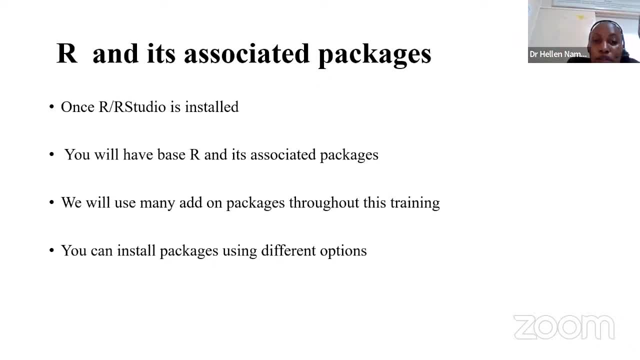 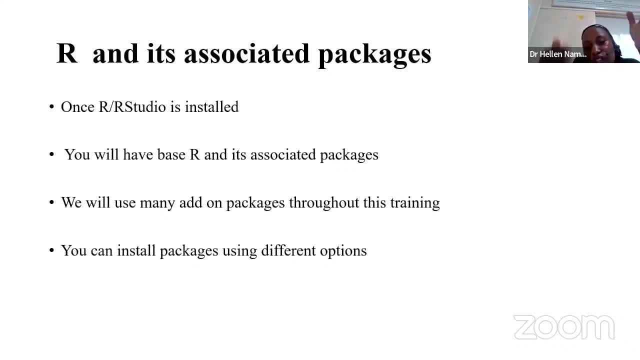 So most of the time you start with small packages, But as you build on, you get to know: well in case I'm going to run, maybe experimental design, what package do I need? And then now those particular people will get to know that well, under this, this is the package that I need. 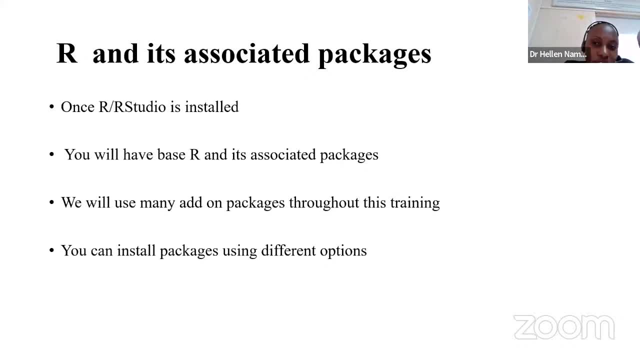 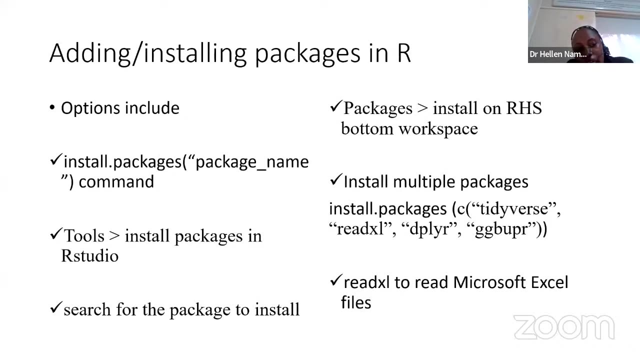 In case you're going to do regression, what kind of package do you need so that you don't just install everything, even the ones that are not necessary? Okay, So there are various options on how packages can be installed. like I showed you earlier, Most of the time we use installpackages And then in brackets. 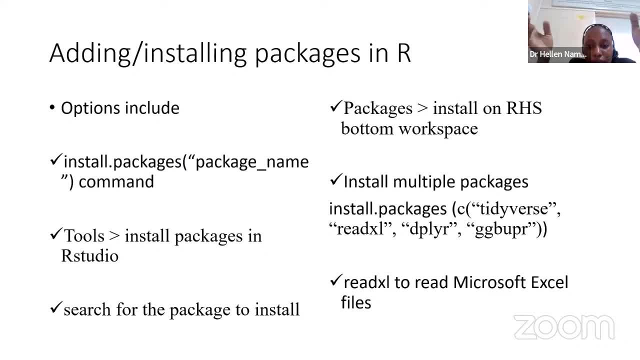 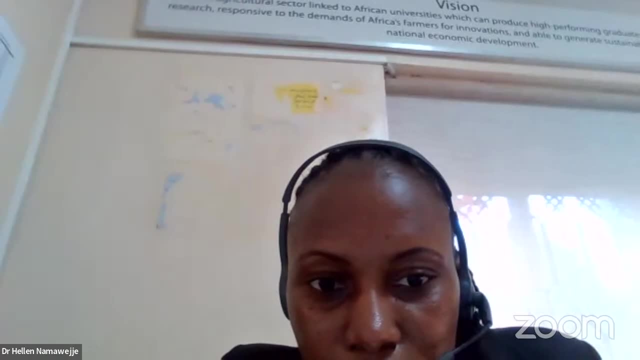 in the quotes you put the package name. That is a command, Okay. Or you can go to tools and then install packages in RStudio, For example. let me close this, And then I share my R script again. This is the script that I showed you earlier. When you come to R console. 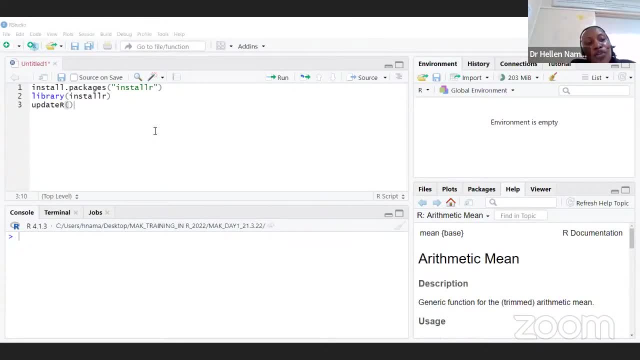 how do you install packages? I mentioned that you use the installpackages command. It is always like this: Watch my first line. Okay, So when you look at the first line, that is the command that I'm going to use To install a package. When it comes to, like I mentioned earlier, 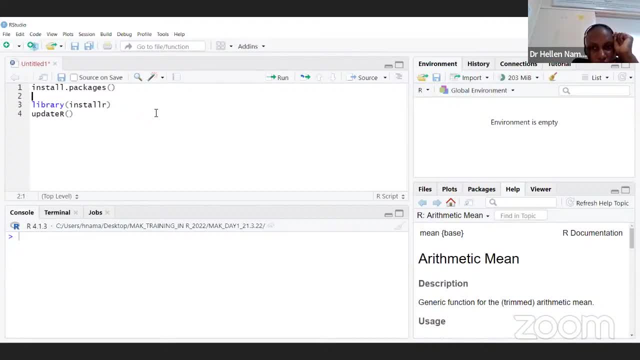 when you are going to carry out different analysis you need with R. you need to. in case I talked about experimental designs, which we are going to still learn about. It's going to be very interesting for the instructor to tell you that now, when we come. 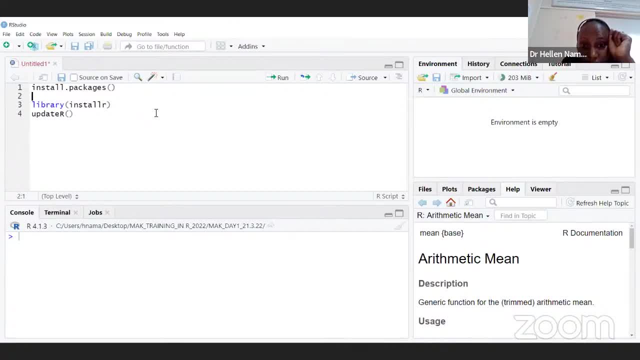 to experimental design. you need this kind of package And all you need to do is to add it on the previous packages that you had, And I said that in that particular case, we are going to use installpackages. There are various ways on how to install packages. 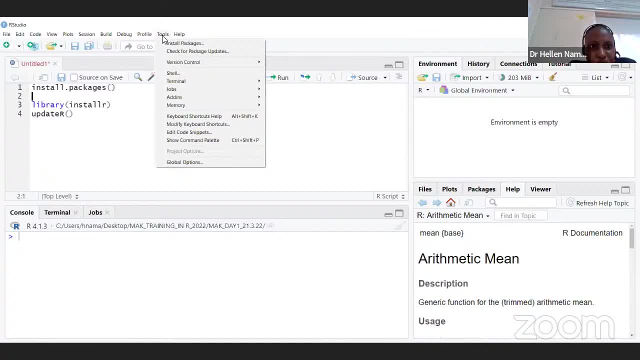 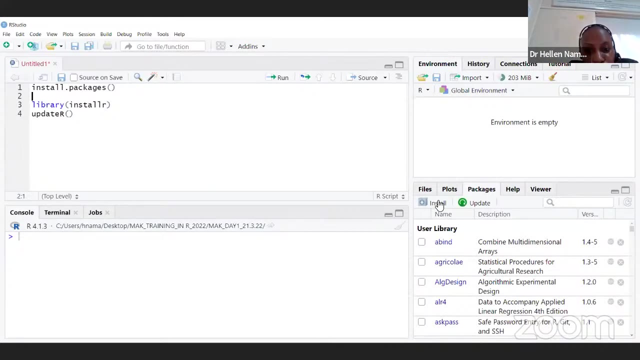 Then you can say. another option could be: you can say tools and then you click here: install packages. That is also another option. Another option could be: you come and click packages and then you come here and click install. The moment you click install, it will bring your window and then you type in the package that. 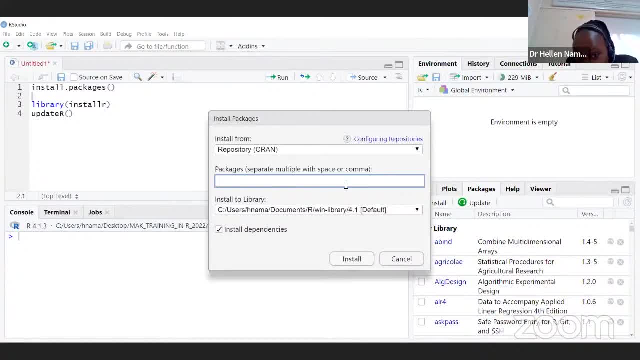 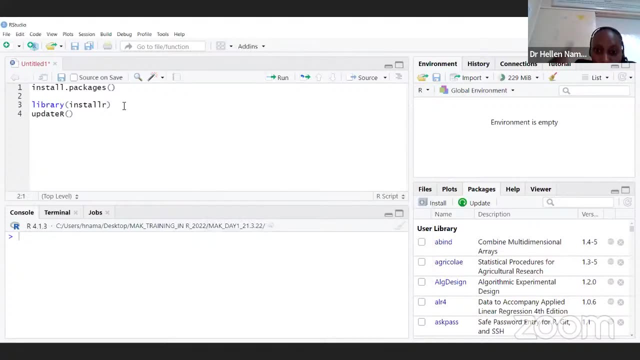 you want. You can type multiple packages at a go, or you can type one package, or one by one, And then after that you come and clickinstall. So there are various options depending on what is easy for you. So I'm going to cancel that, But what is important? 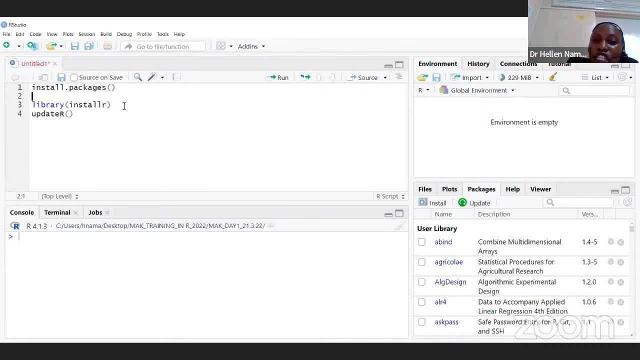 after installing the packages, Because we install the packages from the RCRAIN where, in that particular case, you need internet. The moment packages are installed on your computer, you don't need internet anymore. All you need to do is to load these packages by using the command library. 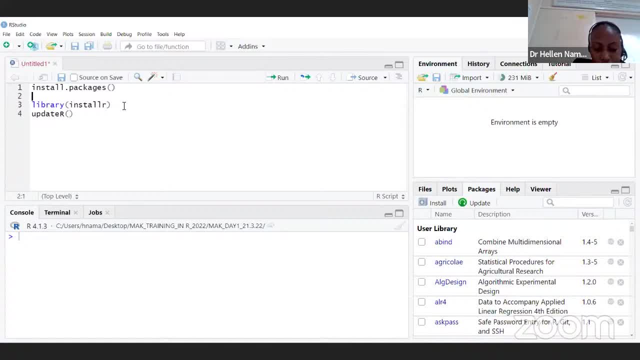 If you're seeing the word library within the library command. what you do is you load now the package that you installed. Initially. we had install r, which you put in double quotes like. install r, which you put in double quotes like. install r, which you put in double quotes like: 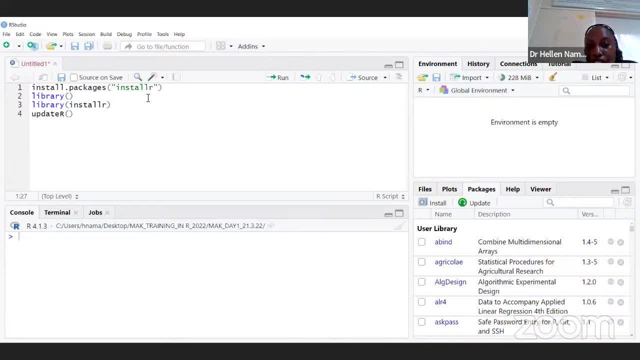 install r. Now, after installing it, what you need to do is to come and load it under the library command. After loading the package that you want, then, after you are set, to go and move on and do the different analysis that you want, Like that I mentioned, when you go to the Crane website. 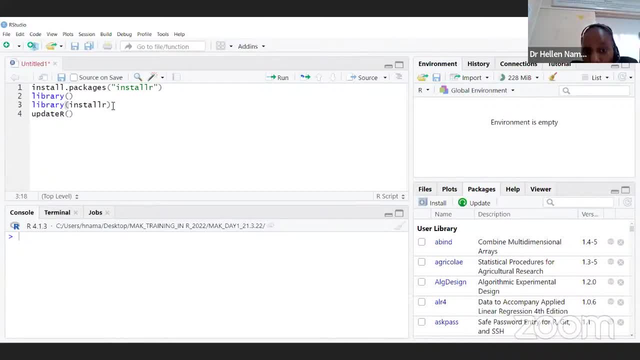 our project Crane website. there are a lot of packages- over a million packages- But what is important is for you to get to know what analysis am I going to do and then what are the specific packages that I need, But there are some common ones, For example, in case you want to. 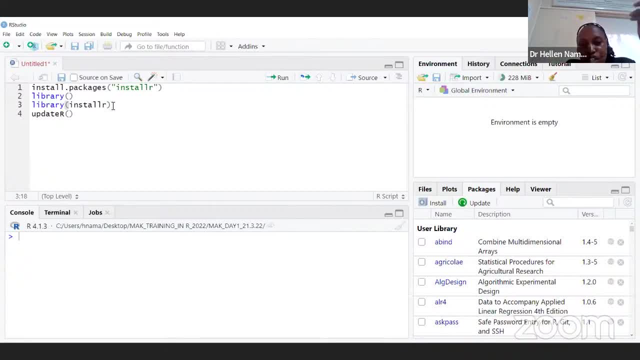 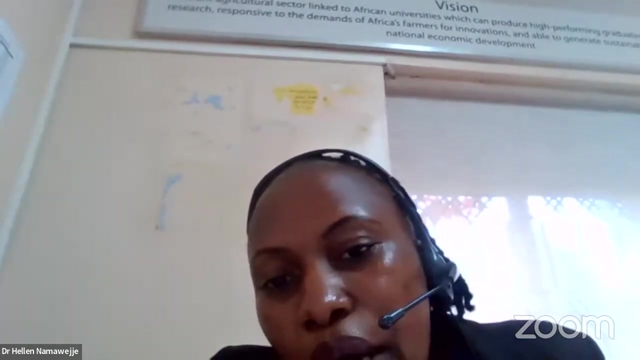 import data into r. I mean, it is the same story. You'll always use the way you're going to import r or to export data from r. Those are similar packages that you can reuse on various projects that you have. Okay, I'm going to stop sharing this and I'll go back to my PowerPoint. 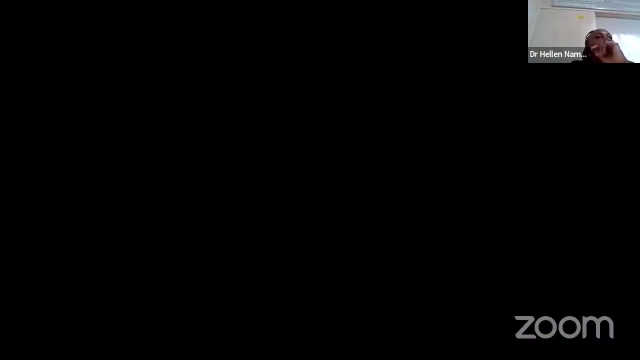 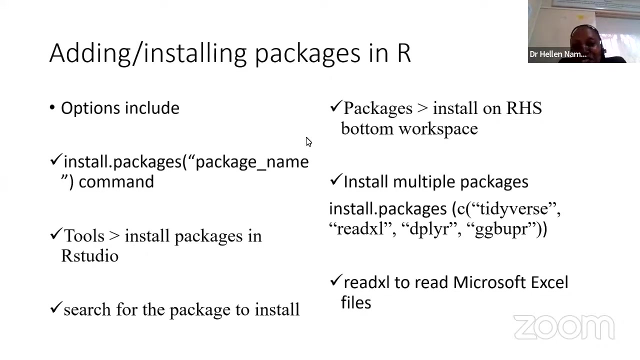 Okay, that's in case you're posting questions. please check in the Q&A. they are sending responses and then we'll move on. Okay, I've already talked about you can have multiple. you can install multiple packages. in case you want to do that, Apart from the installer, like I mentioned, there are various 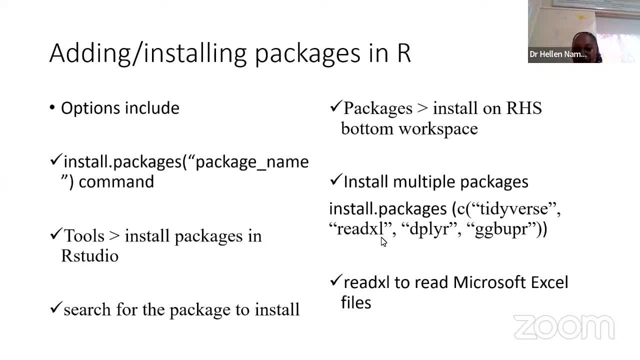 packages. For example, we have the TI device, we have the read XL, the dplyr, the ggbr and so on. But it's also good to get to know where am I installing this particular package? the relevancy. 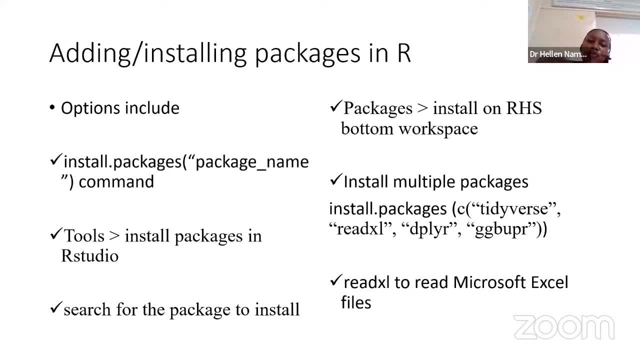 It's like that it supports you really to understand, to enable you to know what you're going to do. For example, I'll mention here that read XL package- Okay, It enables you to read files from Microsoft Excel- Okay, And we're going to see other packages that we need. for example, Tideverse is going to support. 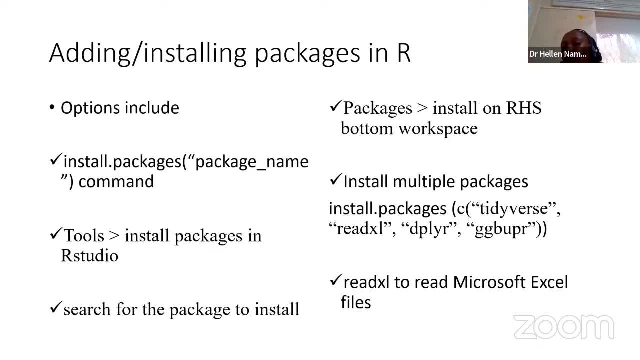 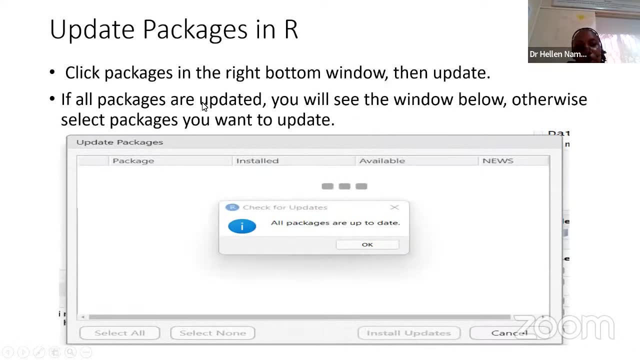 us in case you're doing any data manipulation. Okay, Or you want to do data visualization, a Tideverse package will be good for you, even dplyr. Those are some of the packages that will keep recalling every now and then. All right, I've talked about 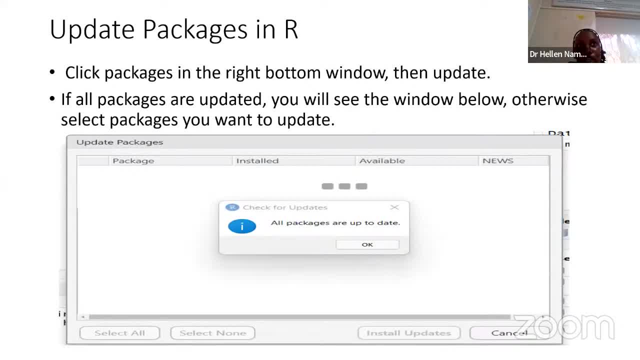 the. The moment you have packages installed, it is also good that you can also update the packages on your computer, Like updating R and then RStudio. you can as well update the what you can as well update the packages. So I was mentioning that already. 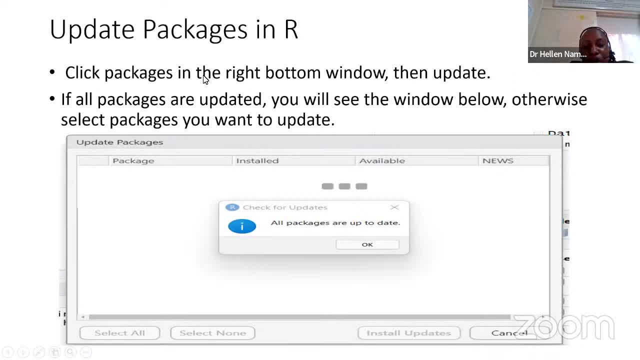 that, when it comes to, you cannot, as you're installing, as you're updating R or RStudio, in case you're downloading to the newest version, in case you're updating R, will reach somewhere and tell you, as you're updating the newest version. 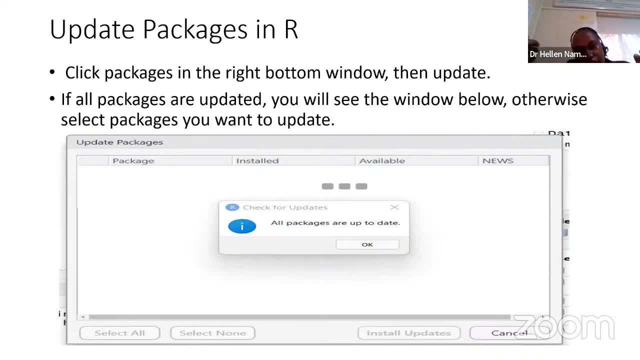 is it okay to update your packages? Then it will be good for you to state that, to click yes, so that you are able to. let's go. I call you Okay. Yes, I was talking about. you can update the packages in R. 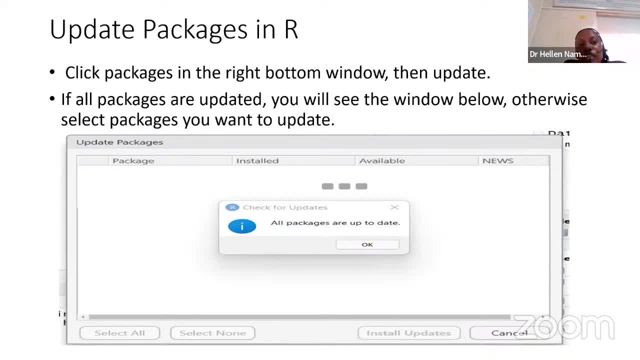 and it also in case you're downloading in the process. as you follow the prompts, the packages can also be automatically updated At this particular moment. I would like to invite the director of DGRT, Makerere University, to have a word for us. 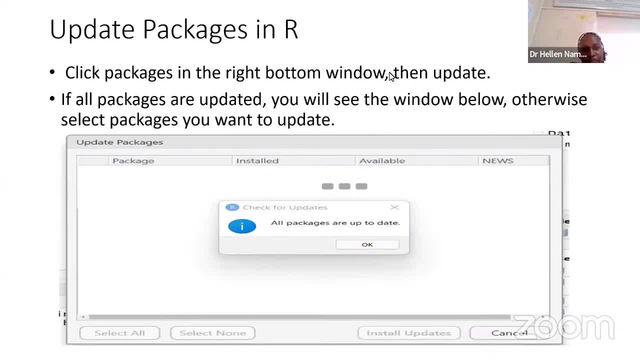 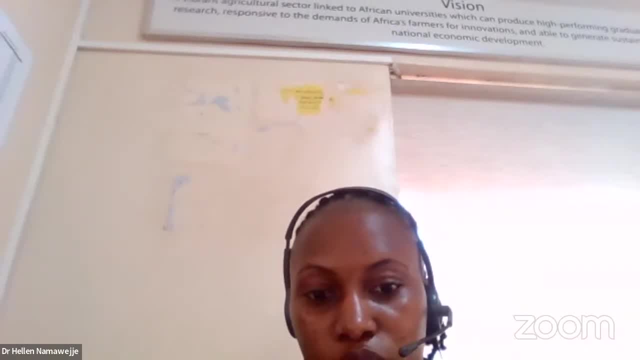 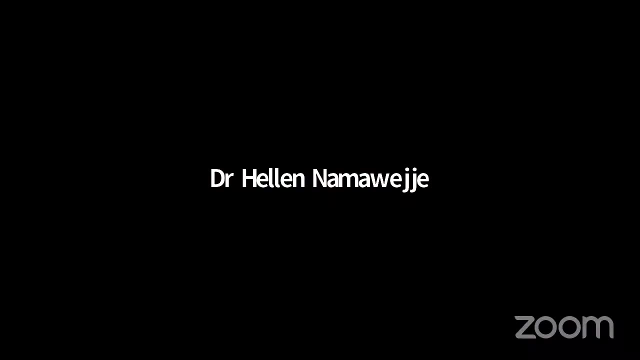 Professor Buyenza, you're most welcome. Yeah, thank you very much, Dr Namawiji. I'm very sorry for coming in rather late. I should have done this my opening remarks. I should have done this my opening remarks. 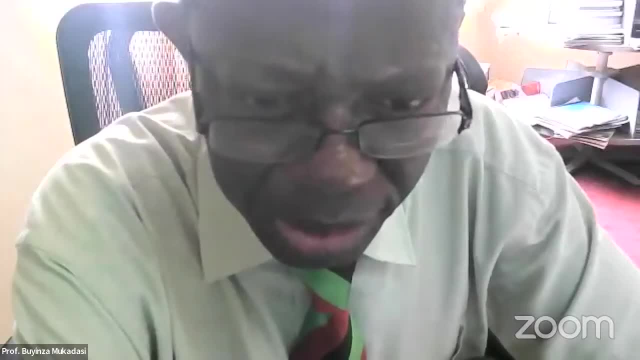 I'm very sorry for coming in rather late. I should have done this. my opening remarks- I just saw the big at the inception of this training and my opening remarks. it was just glad that. but as you may expect, 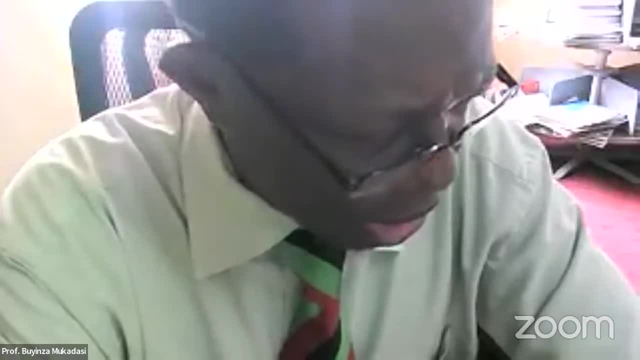 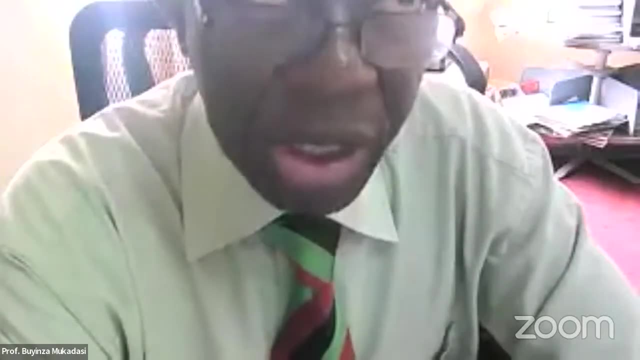 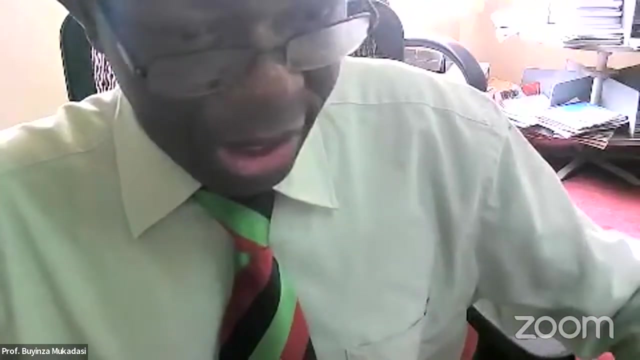 but, as you may expect, I had conflicting engagements in the morning. I couldn't make it. Nevertheless, I've had opportunity to listen to you. I couldn't make it, I think, for the last one hour, and I just feel avid. surveys of the trainees. 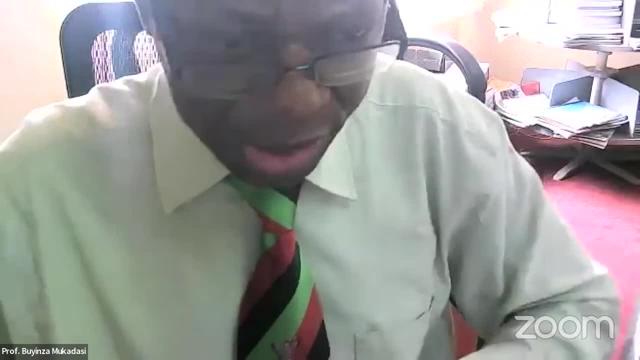 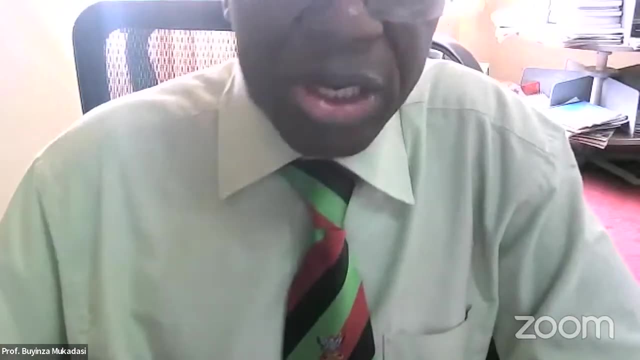 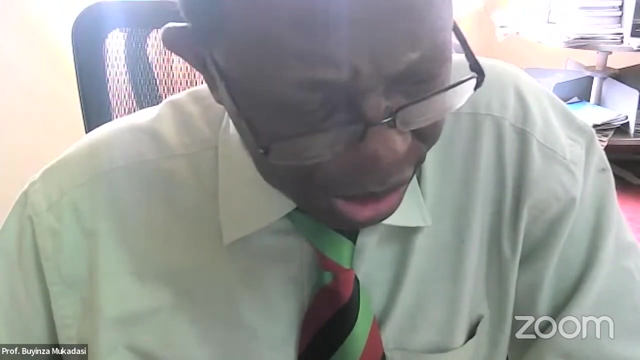 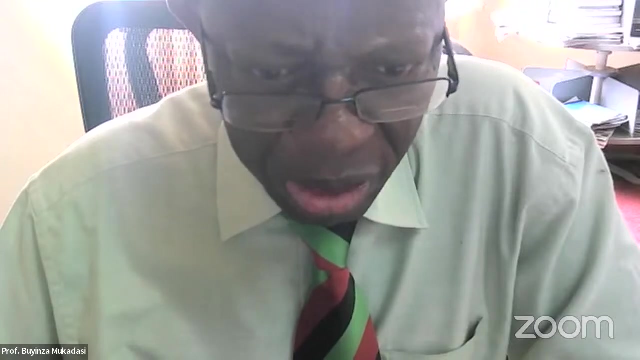 that attending this training, because this is really topical and it's quite important to anybody that aspires to be a researcher. that said, thank you very much and uh, my special thanks go to reform our original uh network that has really supported this engagement. uh, the resource persons i know- my colleague uh professor to me was there- my brother. 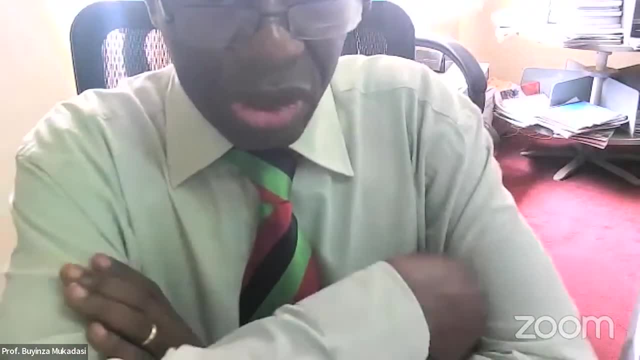 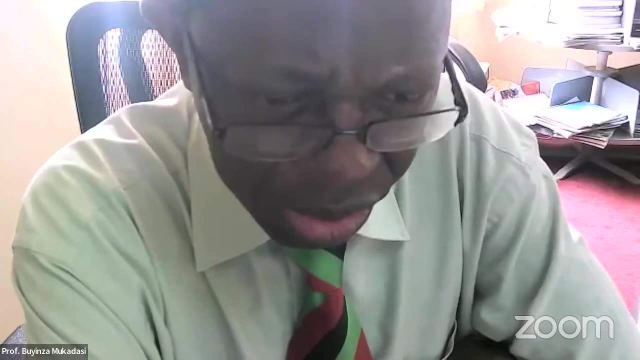 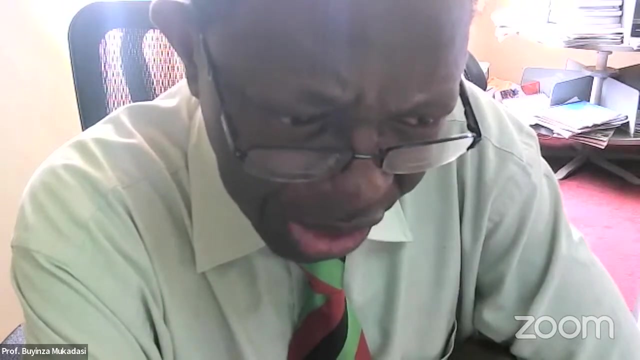 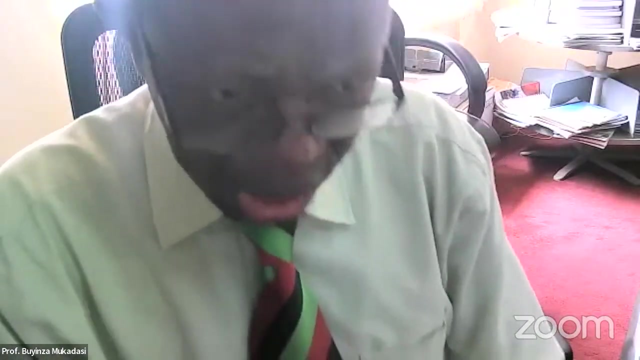 uh, dr thomas dong and many colleagues that have done the administration, like dr francis otto. thank you very much all of you for really finding time to put up this package. uh, we last had a primary training in other language. i think that was in 2015. it was uh uh, convened by the swedish universe of agricultural science. and i think that was in 2015. it was uh convened by the swedish universe of agricultural science and i think that was in 2015. it was uh convened by the swedish universe of agricultural science and i think that was in 2015. it was uh convened by the swedish universe of agricultural science. 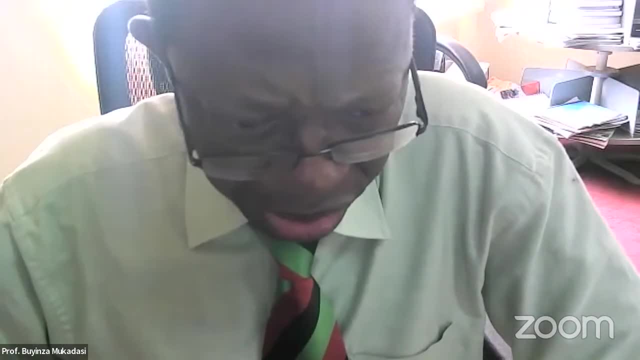 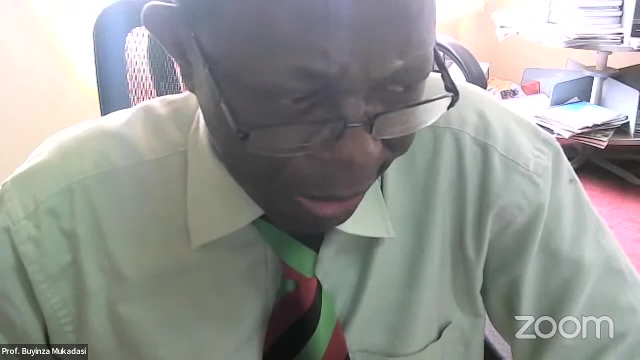 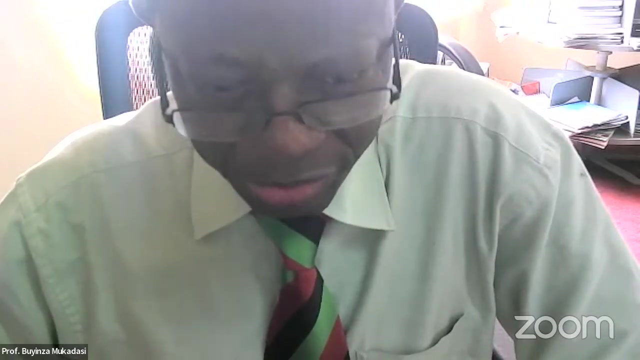 slu here at mccreary. uh, that time, of course, i attended the first two days and, uh, really, i bear testimony of the importance of this kind of training. uh, of course, colleagues, uh, many of you that are ugandan you know very well, we've had our traditional statistical packages. 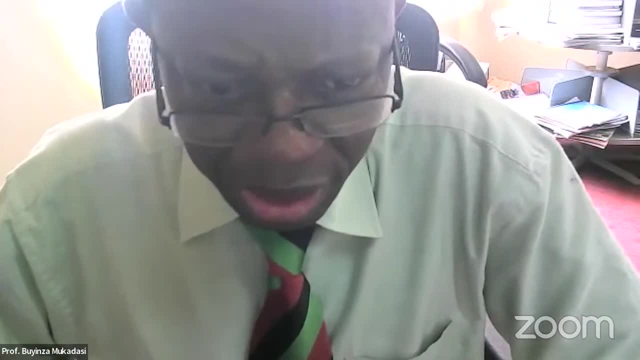 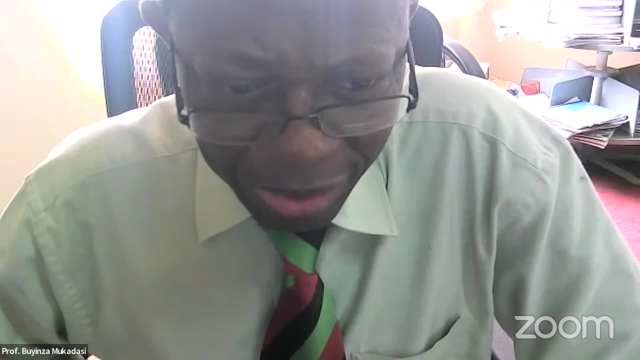 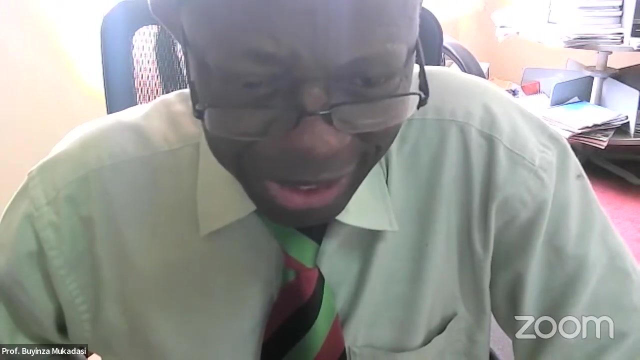 softwares, uh, that we've used over time- spss, sas and many others, uh, i will tell you that, uh, with the time- i don't know whether the data manipulation is becoming more complex- many of these have become deficient, that they may not provide the kind of interpretive capacity that 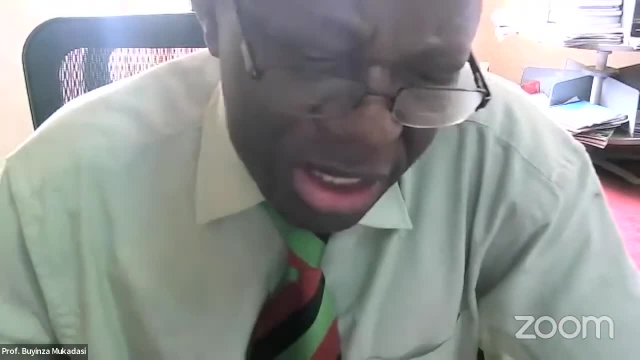 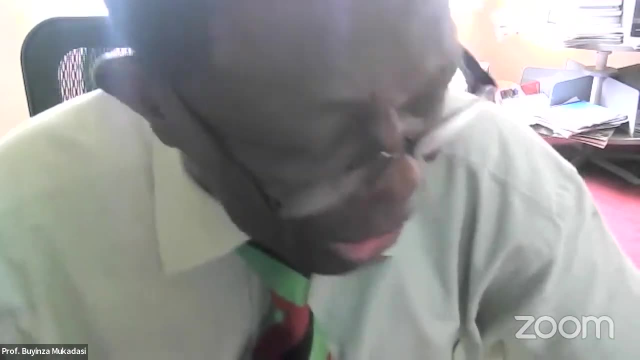 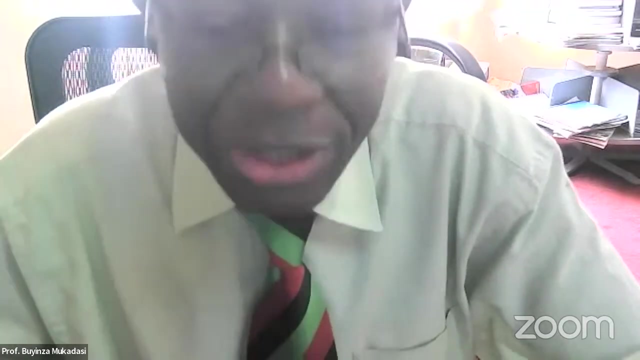 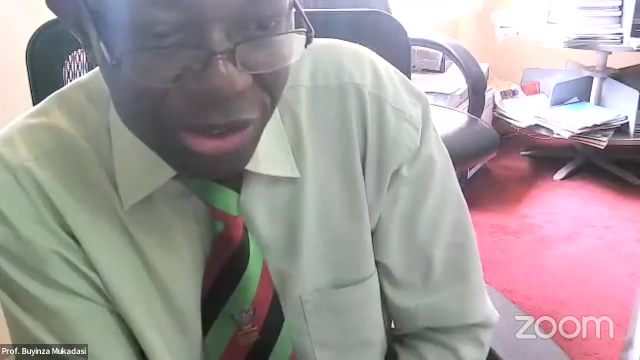 you require, uh, making sense of data. as a director of research and graduate training at mccreary, i will tell you that making sense of data is an essential skill that each of us in the academia need really to acquire. it is in our interest. uh, you cannot afford, you know, to lie. 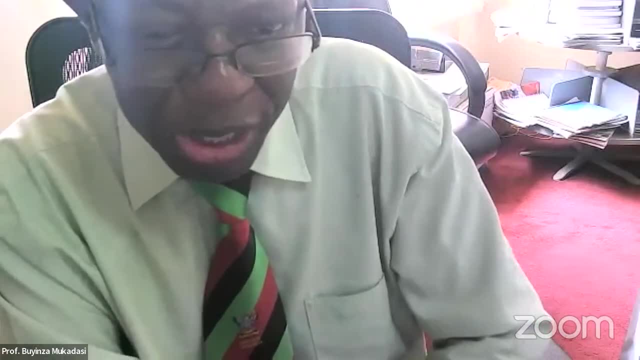 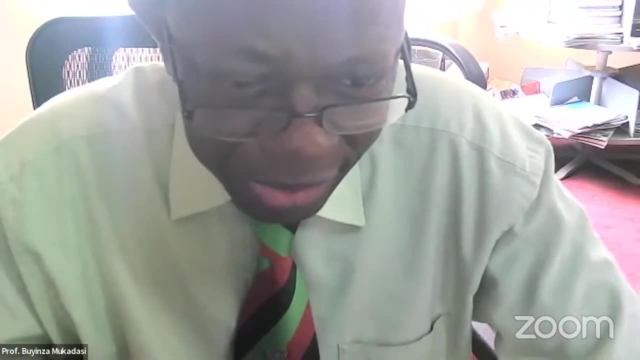 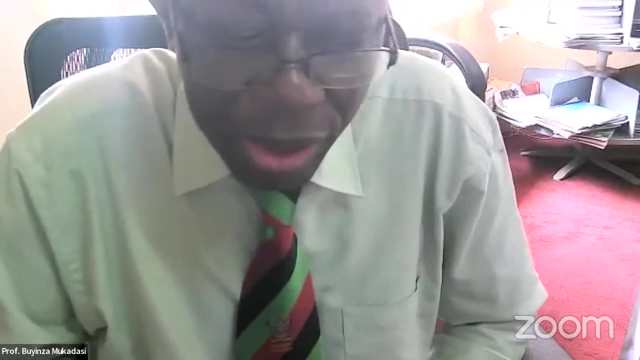 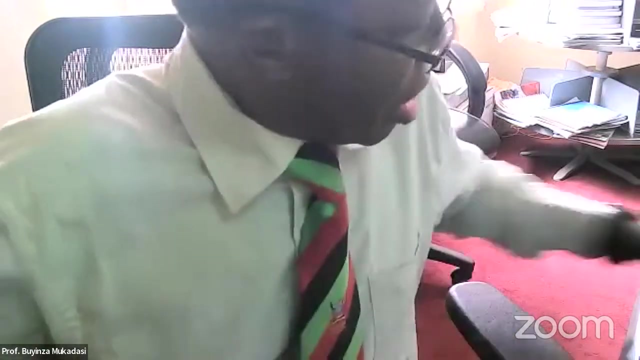 back and believe that this is for those that are preoccupied with quantitative data management. not at all, even if it is qualitative uh. following a uh dr erin here, i could see that uh, really, even if you are in a qualitative data management, you need this kind of uh language for you to survive many uh research questions in the future. 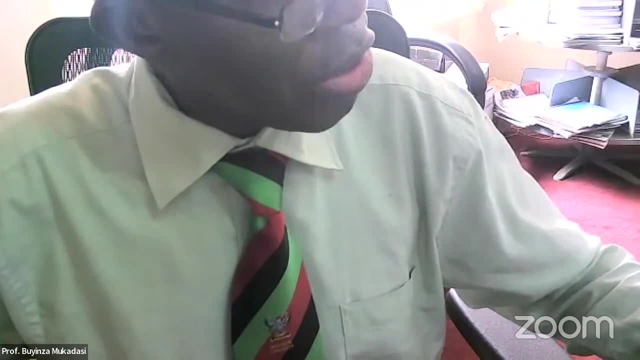 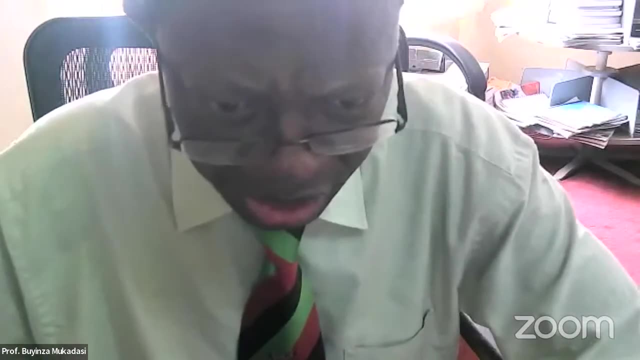 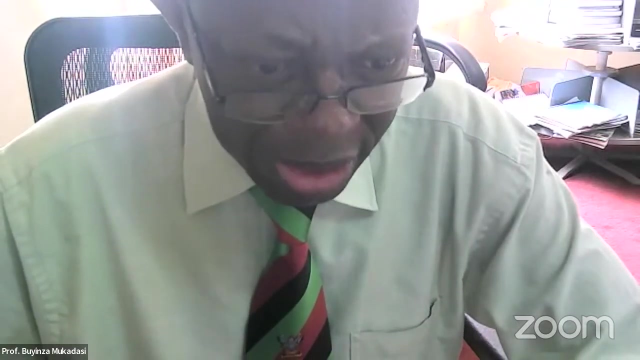 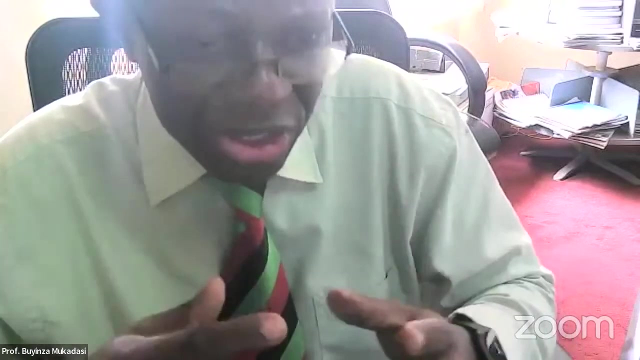 i've also noted that, uh, this is the unopening software with really many futures, as uh dr namawiji has exhibited here, and really it is only fair that you are really committed. the trainees are committed. you go through the whole entire package as it has been assembled such that you can appreciate, develop the skill and be able to use. 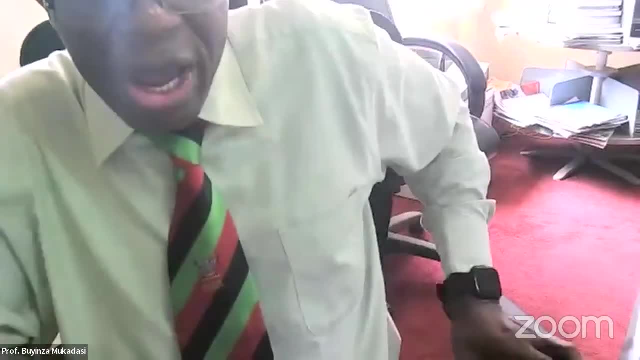 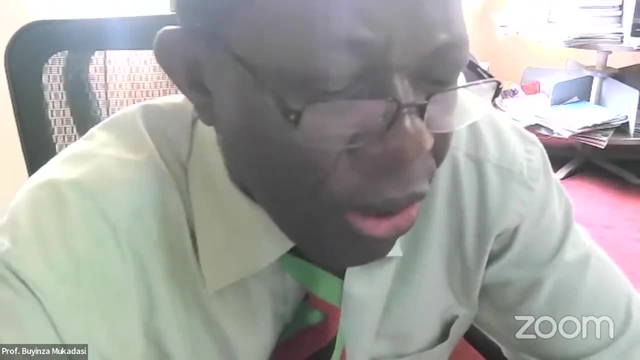 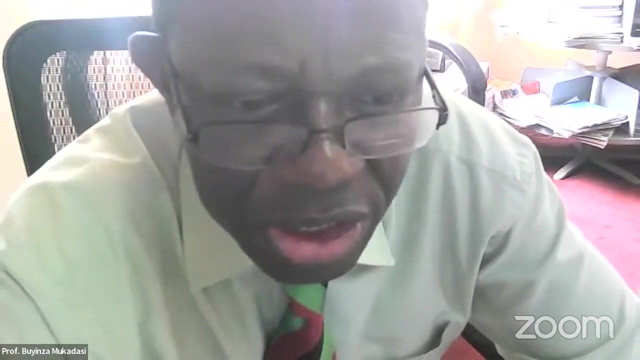 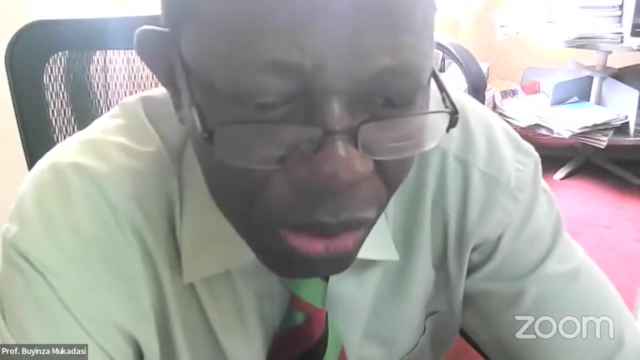 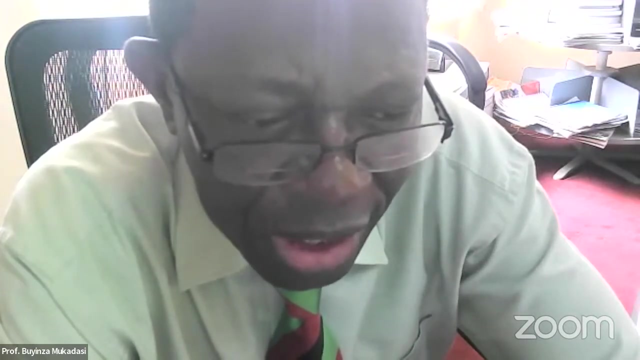 you know uh this de facto standard sort of language for writing uh statistical softwares. of course, personally, i know that uh uh really getting creating a statistical analysis solutions, getting something that gives you uh solutions uh to to our statistical challenges that we face on a daily basis, is really something that uh we should. 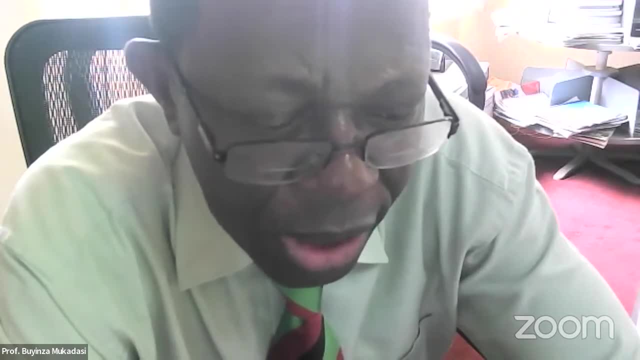 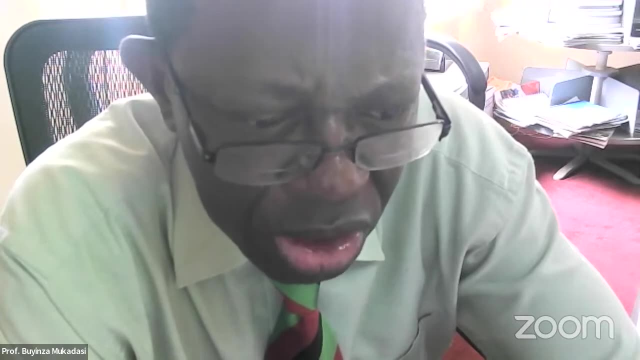 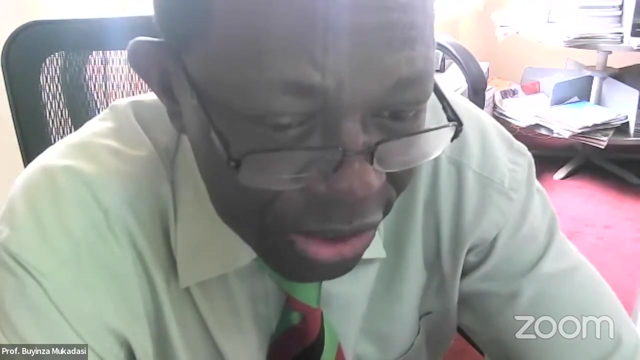 appreciate, and i think we we can only be indebted to reform- that identified uh this competent team of resource persons and also resources to enable the training to happen. uh, i know for sure, listening to dr namawiji from the beginning, i know uh that this sort of uh. 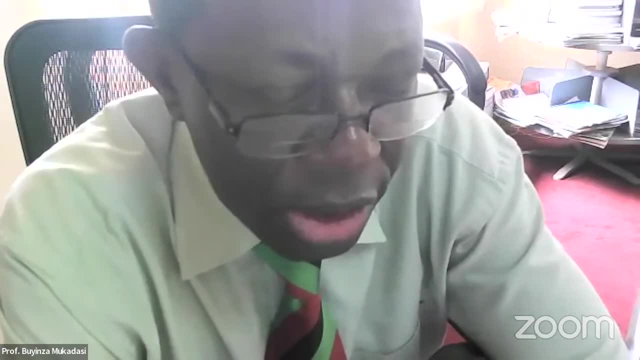 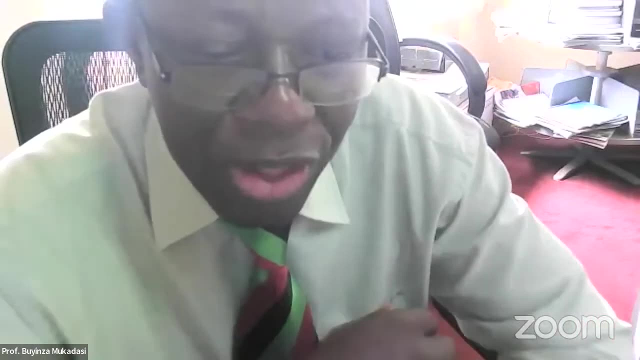 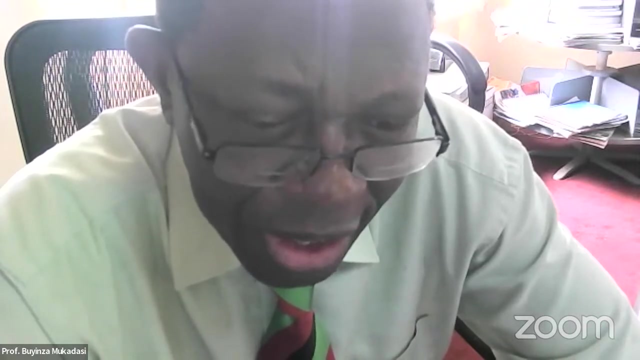 this software you can do a lot. uh, i've i've seen the- is it the ara studios as? uh, that very powerful user interface. uh, i'm not very familiar with the r as a language, but, uh, i i could only admire that interface that you get. 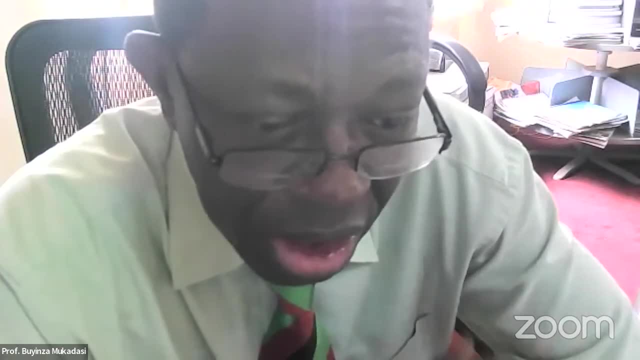 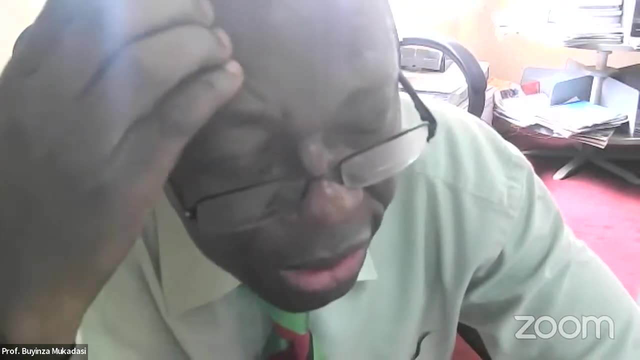 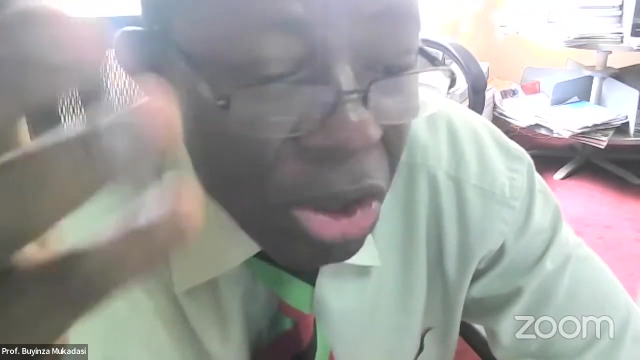 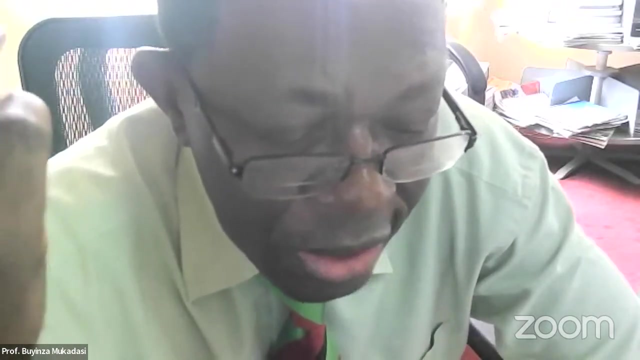 and the visual representation, the data that, uh, you know you will be able to present in different ways. uh friends also tell me that, uh, this language, they, they say, are a sort of uh language that you can be able to import, export data from various sources. you can imagine, you know, developing that capacity to manipulate independent 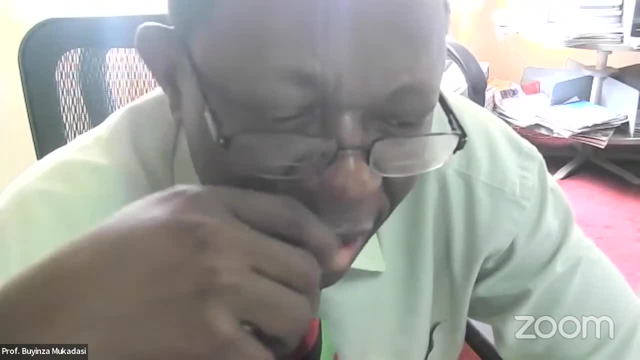 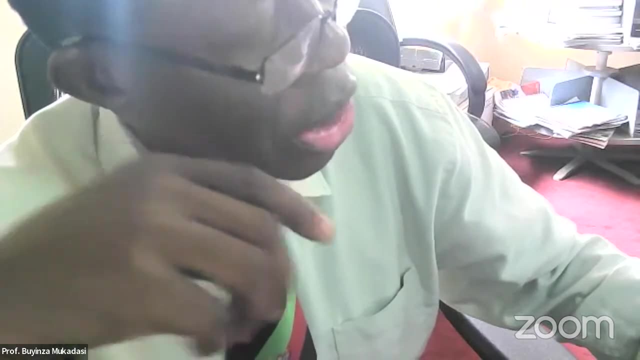 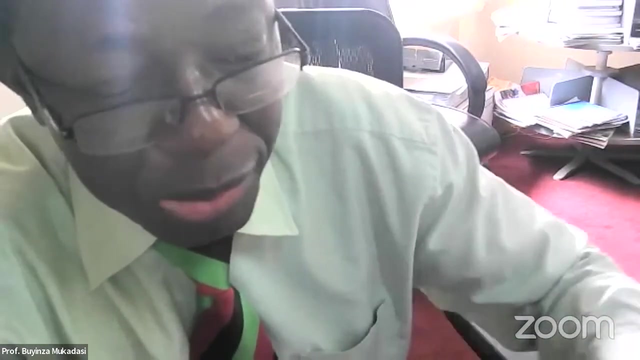 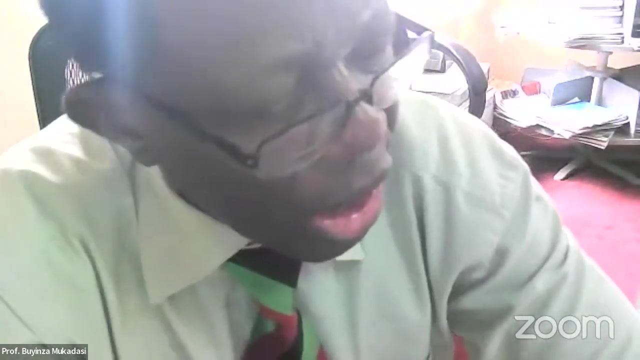 public hand setup programs, يا angry sub too, to some sets, um subsets. you know, it is really something that, uh, you should take seriously because, uh, i will tell you, it could be your only niche that will make you special compared to other academics in either your departments, okay and um, i know, i know for sure that uh, uh, many of us, of course, once you've you've worked in the department, so it won't impact you, alright. and uh, and i know, i know for sure that uh, uh, many of us, of course, once you've you've worked in the department, so it's not really Maisa. on the farklı koreanic study or any other academic study or any other method we are bound for right now, correct? 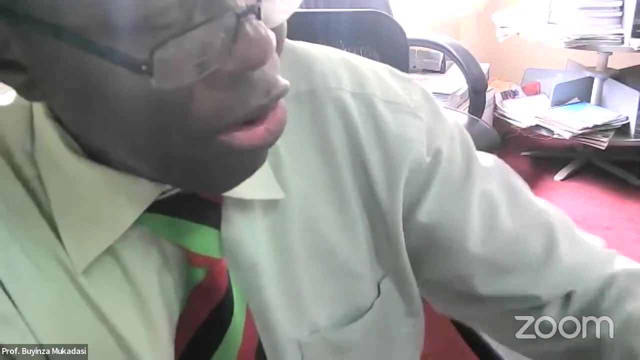 but when you introduce it as you change over to the research and process or your framework, just this will make you different. right? Who's in the role of faculty as a class? what is this me? how do we work onえ acquired the skill of using one law, one, one statistical package. then you believe you can. 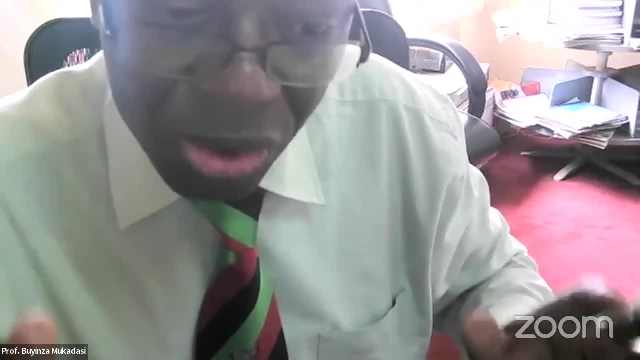 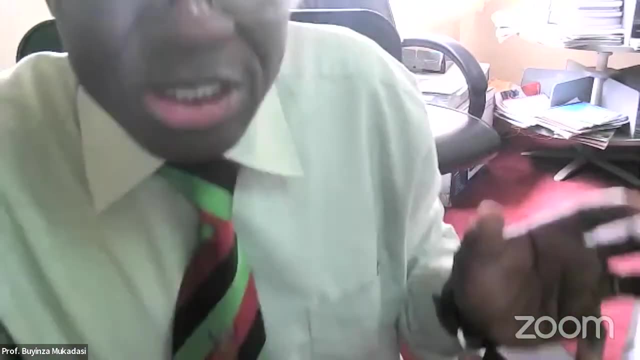 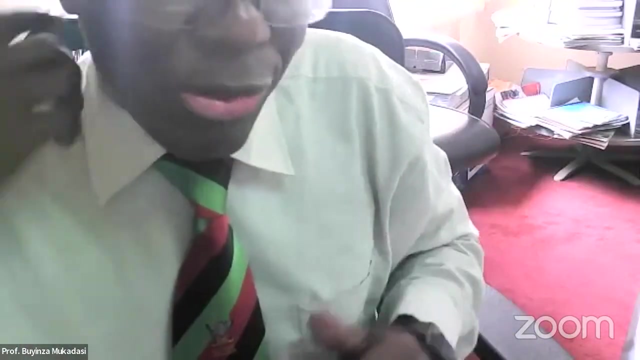 survive, you know. but i will tell you, in our field of research, which is becoming very competitive, uh, that you may find even a? uh funding agencies that may say analysis. we want you to use ara, want you to use s, we want to use you this particular special package, so you may lose that. 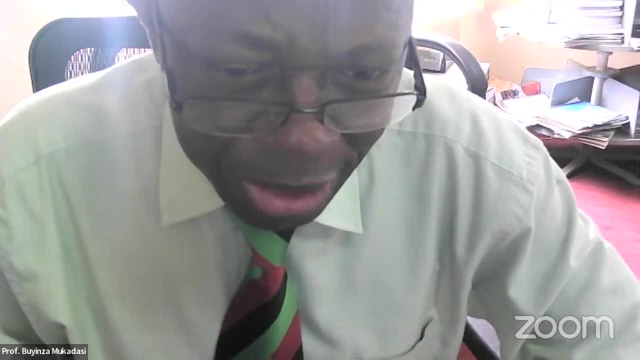 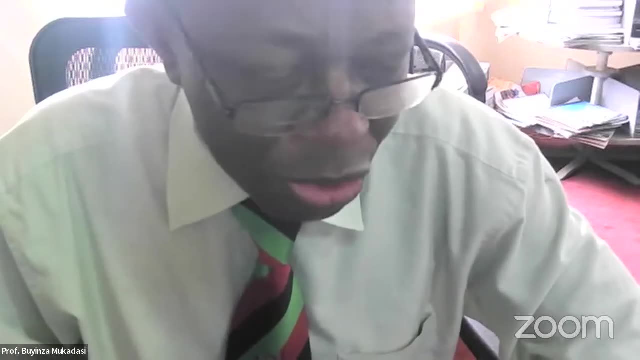 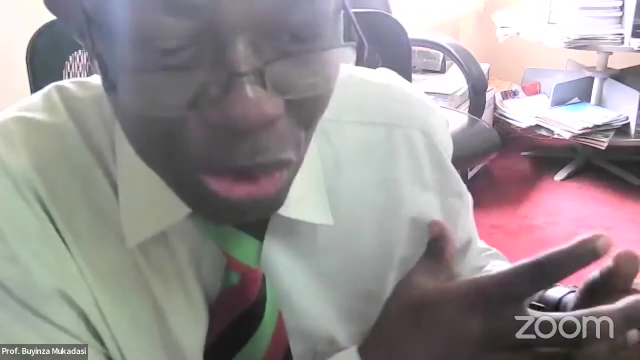 opportunity. okay, you cannot uh stand somewhere in a corner and say, after i can do, i'm very well, i i have enough to use for if i need a linear regression might for regression binary logistic, i can use this tool alone. i'll tell you with the time. you'll discover when it's late. 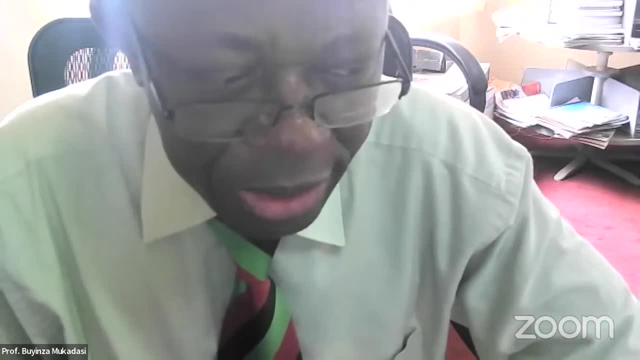 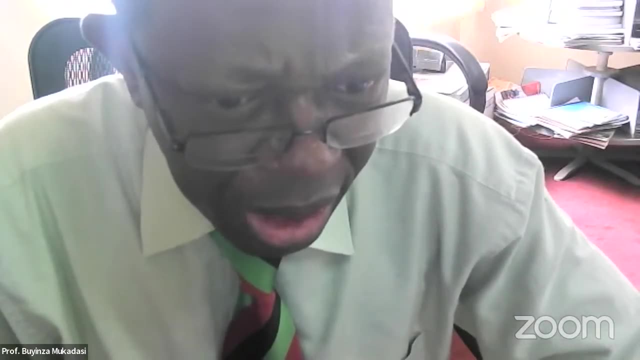 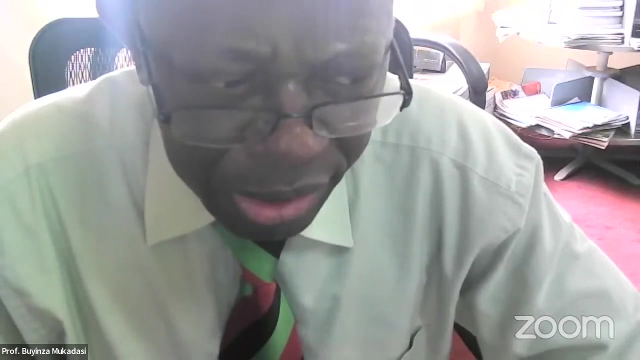 that that tool may not be robust enough as ara. so i want to thank you, colleagues, uh, and i know for sure that in the coming uh is it one day or two days- you'll be able to really show. association is in ara, for example, as well. the other century, we'll talk of the chi square. 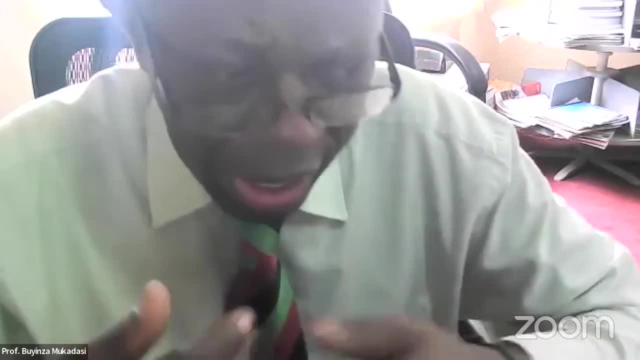 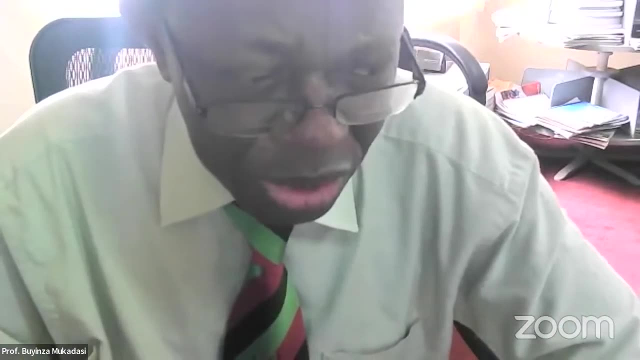 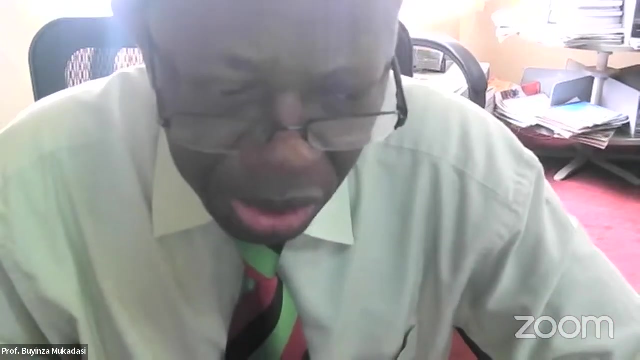 test of independence. how do i now bring it in ara? and if i'm used to pearson correlation, how do i still also survive if i use this fearman rank correlation? how do i bring it in to work with the other language? i think that will be important in addition to helping our 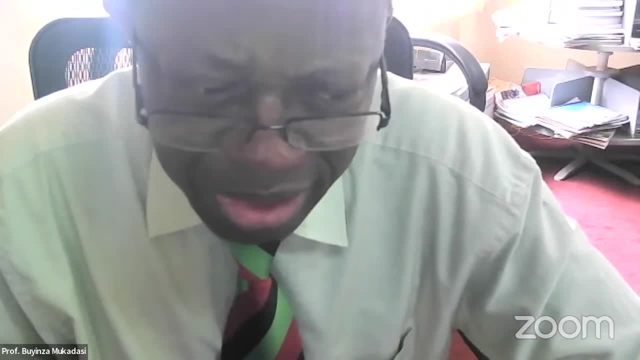 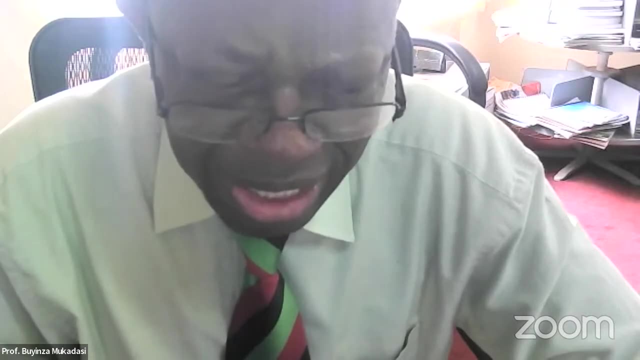 researchers do a very good data cleaning. we've had a little bit of a problem that people present data that is not clean raw data, so it makes it very difficult for you to do data framing, and our managers here, those that are doing data mining, have a very big problem. 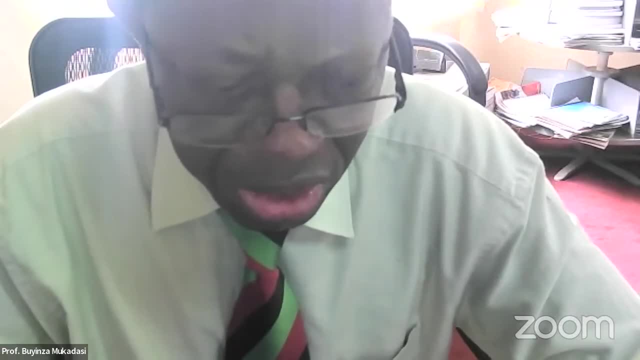 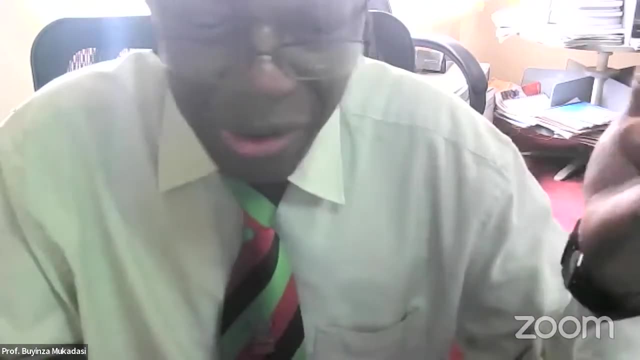 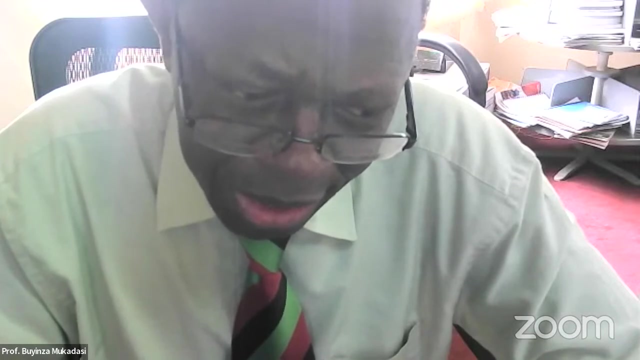 either with our phd students that are, or even a focus when they present their data. you cannot use that- that data to develop decision structures. that has been our problem here. so i'm happy that this training has come and it is being really facilitated by eminent people that i hold in highest team. 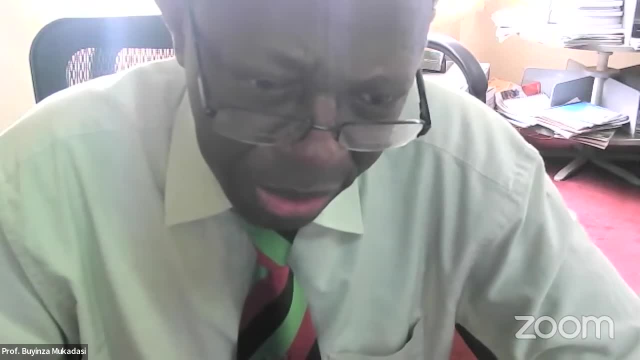 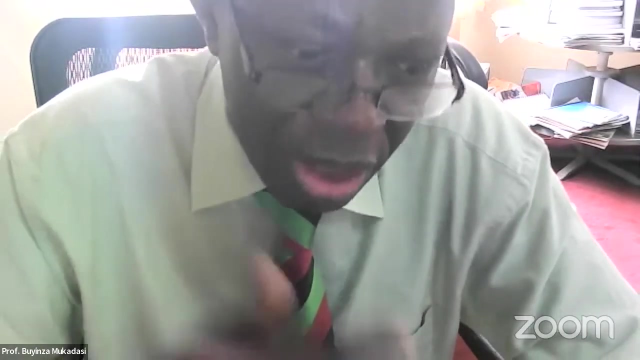 so, as mercury and director of research in particular, we really commit our total administrative support to this kind of training because it's the way to go. okay, we need to build the research capacity of students and focus at all the times, and that is. you know, it is a lifelong experience we have. 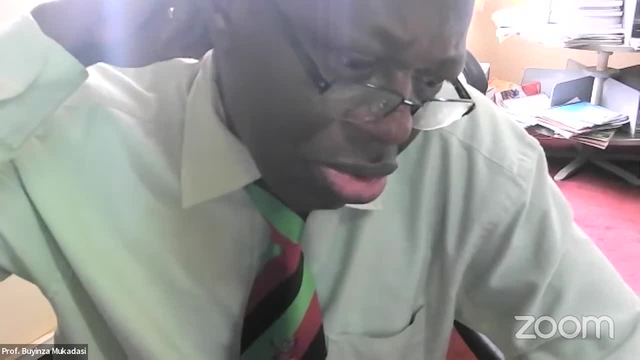 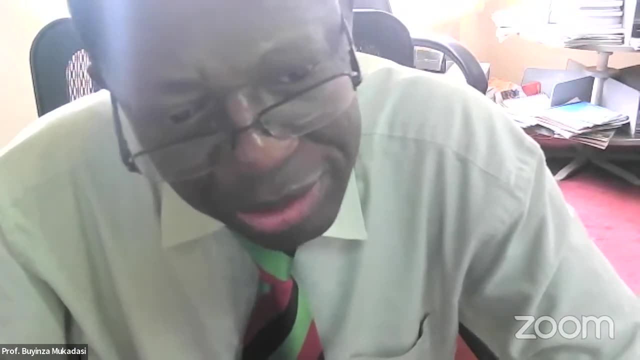 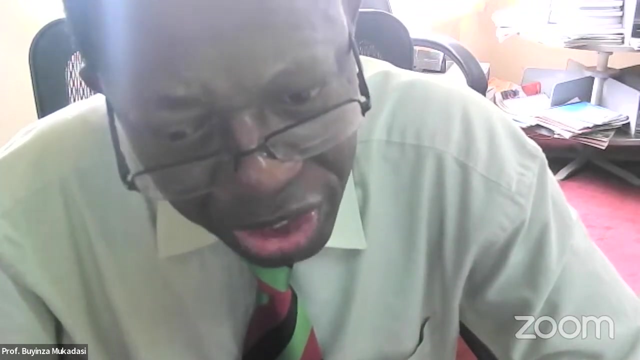 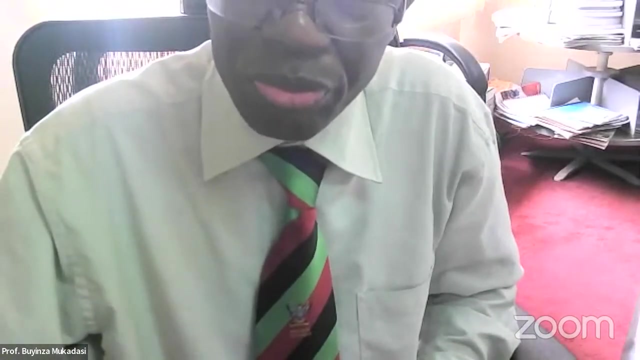 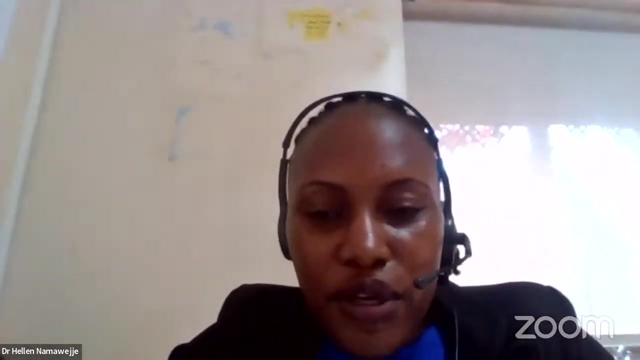 to continue acquiring and also uh returning our staff at regular intervals. so thank you very much, her colleagues. i just wish you fruitful deliberations. look forward to receiving a copy of the of this training at the end of the engagement. thank you very much, um. thank you so much, professor williams, for the great remarks, like. 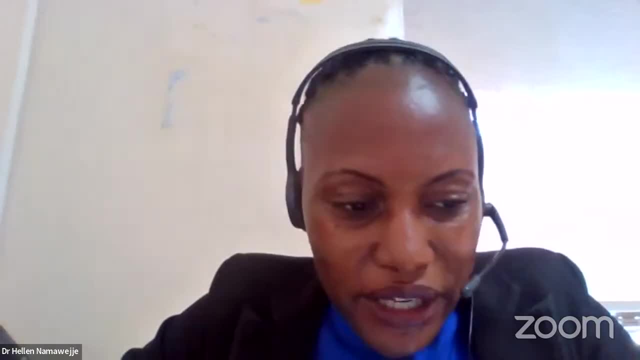 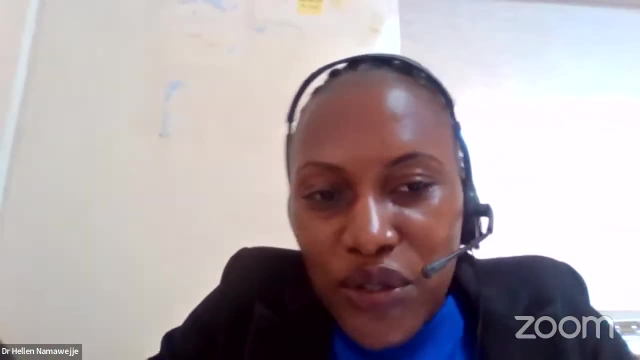 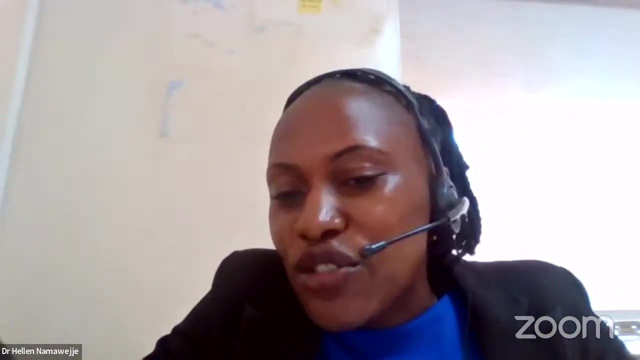 professor ruins has mentioned that it's a wonderful package. all we need to see that can we really spare time and see that we are able to grasp the different concepts he mentioned about, like how do we shift people to the seeing, the association between the relationships of the? 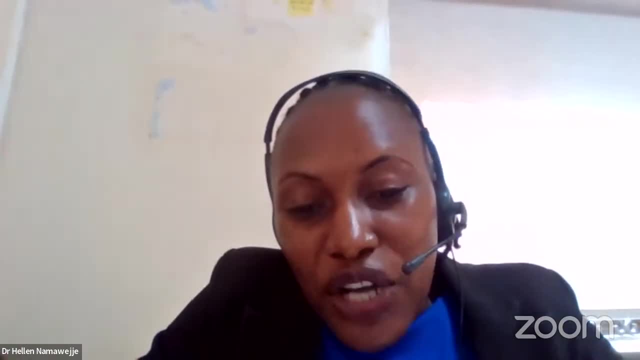 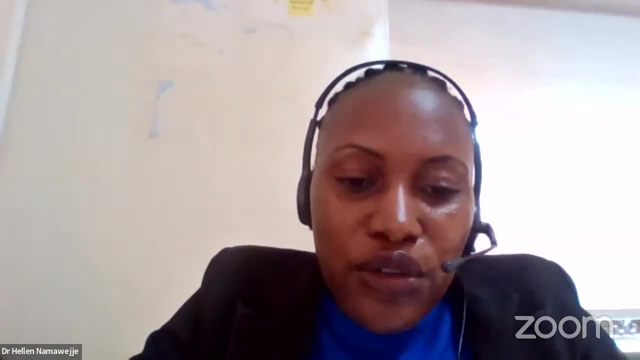 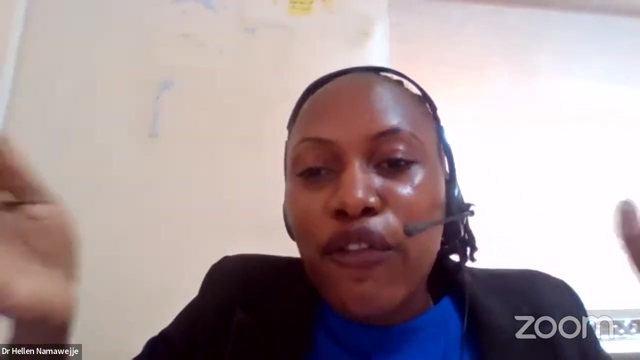 variables. i want to promise you that it's part of the training, it's part of the package, like we sent you the concept note. everything is there, but what is important, that usually on the first day a participant needs to know how do i install r, how do i download it, and then thereafter that. 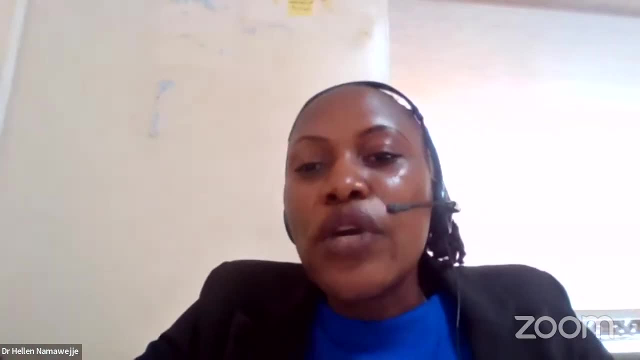 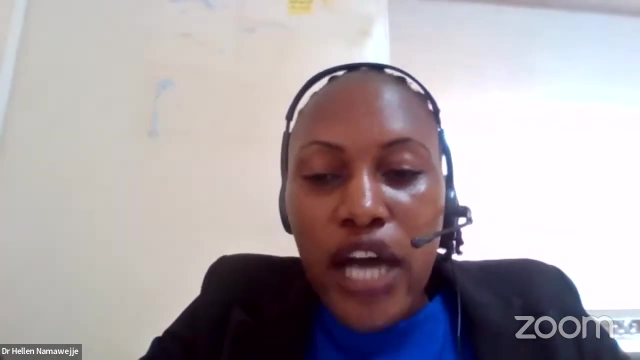 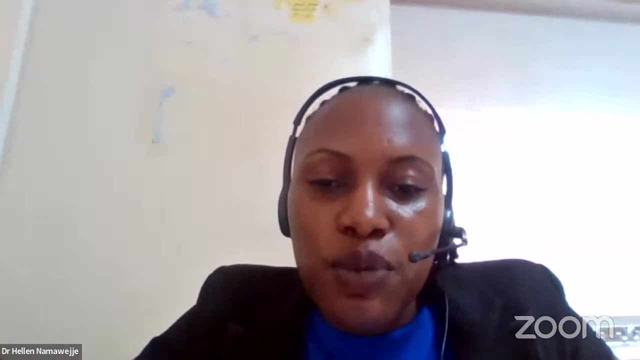 the moment that is in place and it's very clear. then we dig into how do you do the association? that is explanatory data analysis and it's going to be covered tomorrow. yeah, i, i believe that you also get. i i think that will also receive your expectation. thank you so much for your time and. 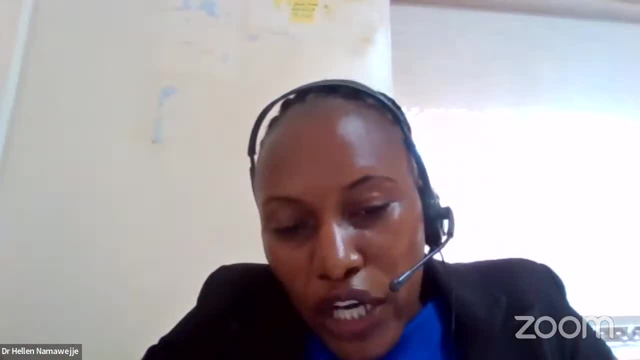 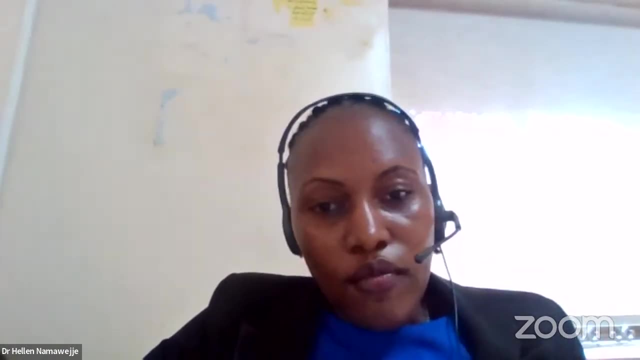 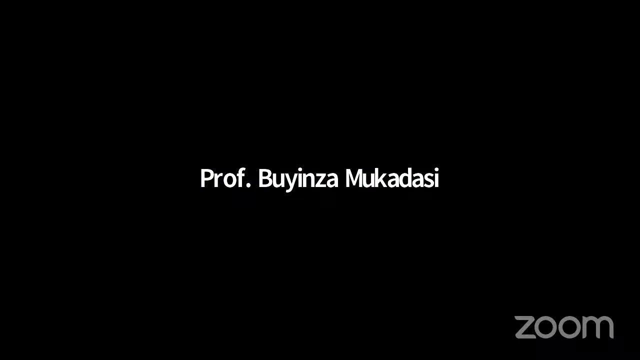 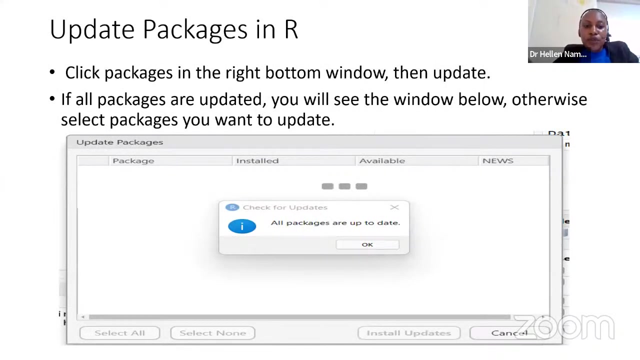 i still ask you that, in case you have time, please, um, you can join our training until saturday. thank you, thank you very much. okay, now participants. um, that was, uh, professor vienza, director research and training at mccary university, and we are still working under his docket because he deals with graduate students. so 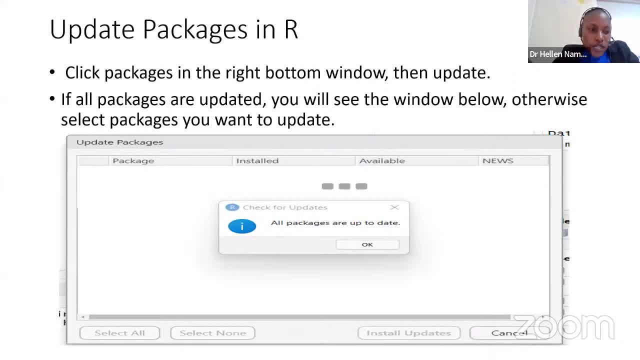 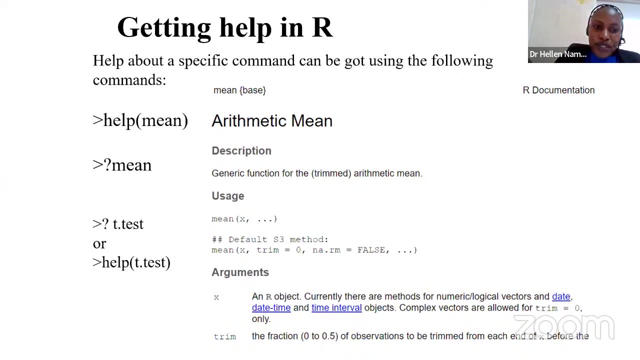 now let's proceed from where we stopped and then now we continue. okay, now, as we move forward, we have a few questions from the audience, so if you have any questions now as we move on, there is also another important concept that, uh, we can get help in our sometimes. 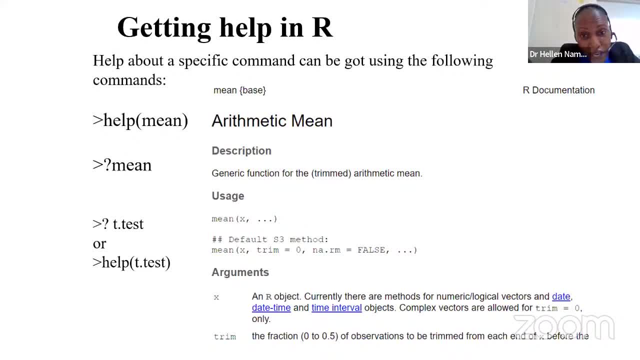 when you're trying to manipulate the different- uh, the different- softwares, for example, like we're saying that with r as an open source, maybe, as you are working, you get stuck somehow, but what is interesting, that r can be able to support you. i don't know whether we need to mute. 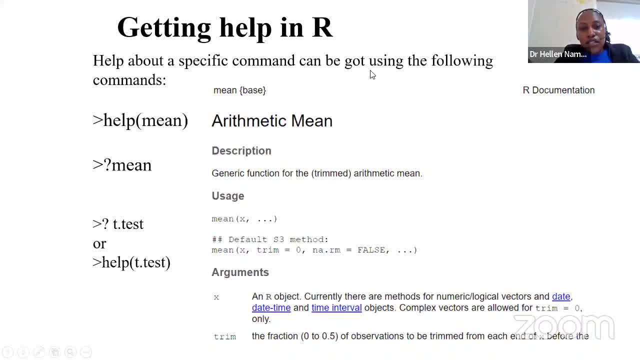 equals. is that right? um, okay, yes, we are sorting out something. yeah, i was saying that we can use r to support us to understand certain concepts. and when we get to r, how do we do that? we are going to use the help command because, um, you know, sometimes, as we know with the different softwares, maybe you 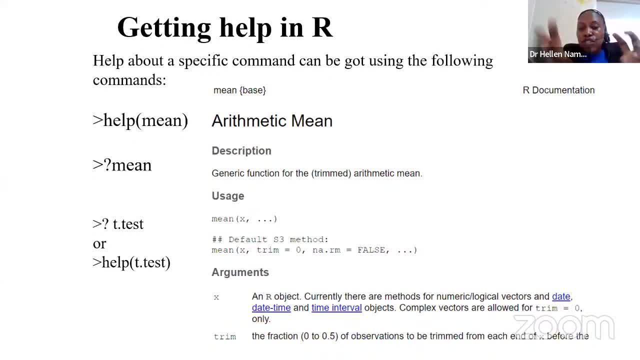 need to understand the different arguments. how am i supposed to to state my command which is supposed to come first, and all that particular information? so what happens is that r has got an r document or inbuilt material which can support you to understand on the, on the many things that you might need to need. i'm going to stop here. 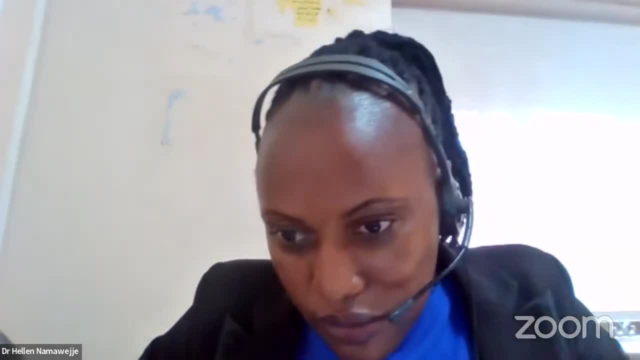 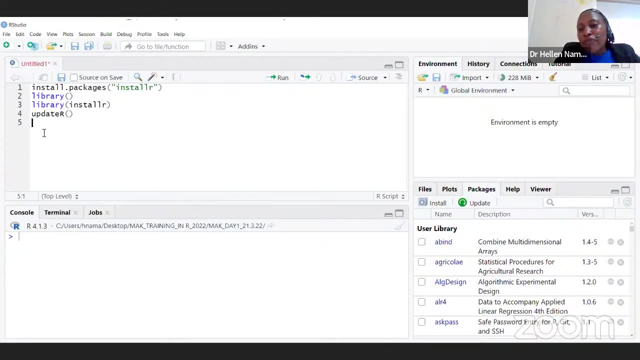 then i share my r? r script again. so, for example, when you come to our studio, you might be interesting to understand more maybe. what does mean mean? what does sky square mean and how do i use it? so, uh, what you, what we do? we usually type the help. help is the command that can support you to. 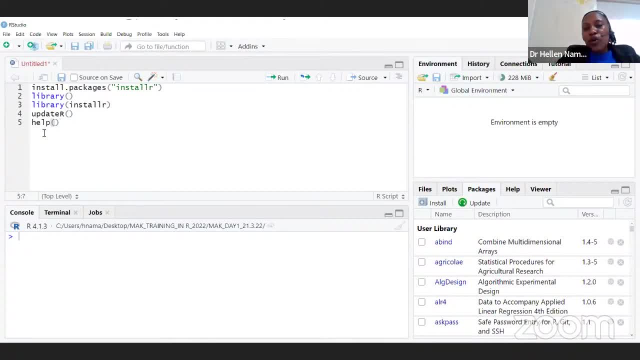 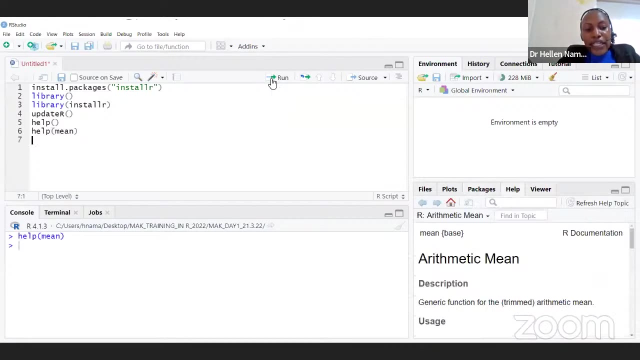 understand more, to get more details, or now on a certain interest that you that you want on about. so assuming i want to get to about, maybe i type in help mean the moment i type in that all i need to do is to come and run my line there the moment i click run, if you see very well in the r console. 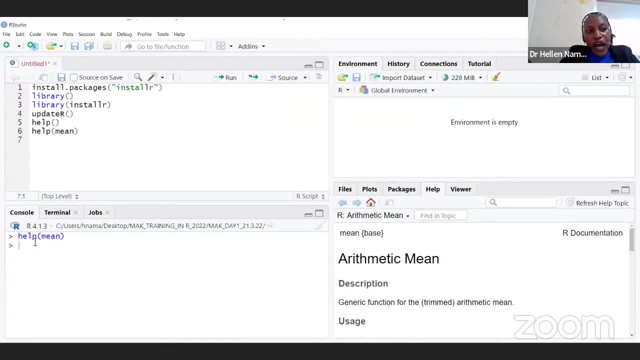 what is happening that? uh, it brings whatever you type in the r studio. when you look in the r console we say our console, you're going to be seeing the output that you get. okay, it is going to show you help mean. but when you look in the help window on your right hand side in the bottom, 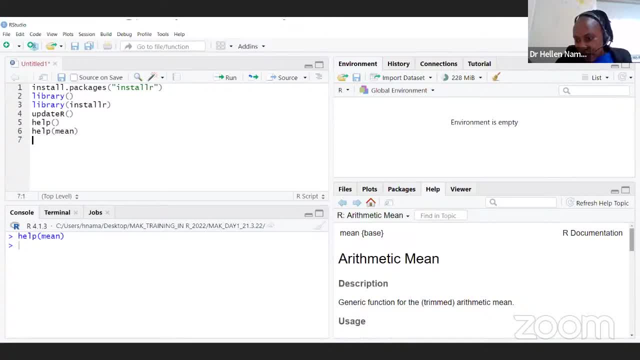 one. it will tell you that about the arithmetic name, giving you more details, and it will give you the description, the generic function of the trimmed arithmetic mean. it will give you the, the usage. how do you use that particular command, for example? it will share. it will tell you that. 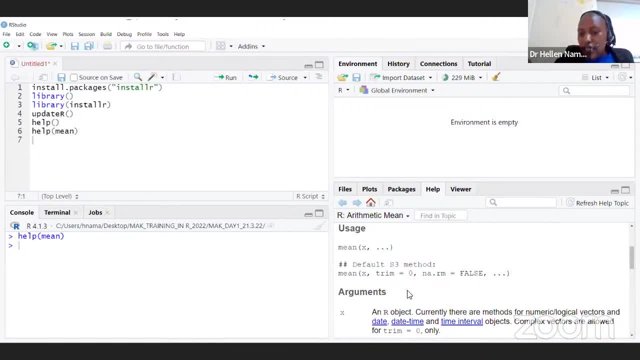 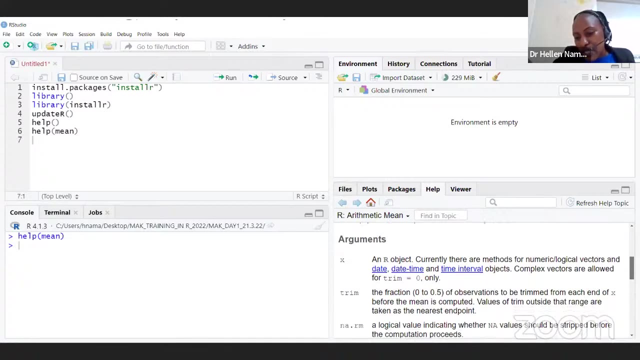 you know within mean we start with this and this, then it will. i will explain to you the different arguments that you can feed inside a particular command and it will tell you everything it goes ahead to. then it goes ahead to give you various examples that you can apply. all the arguments are: 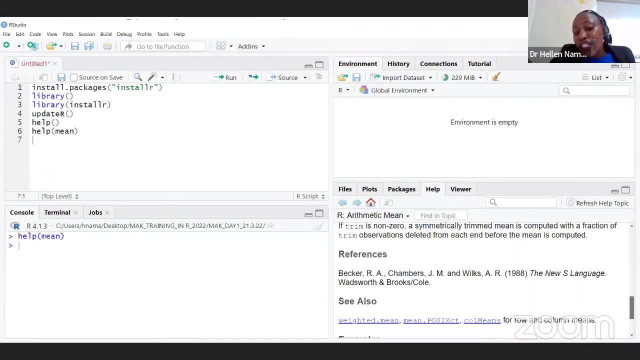 being explained, the values that you can use. sometimes it gives you the the references that are being used and also an example that can support you, for you to understand what exactly you want to look at. okay, in case maybe you're in, in case you don't use the help command, you can. 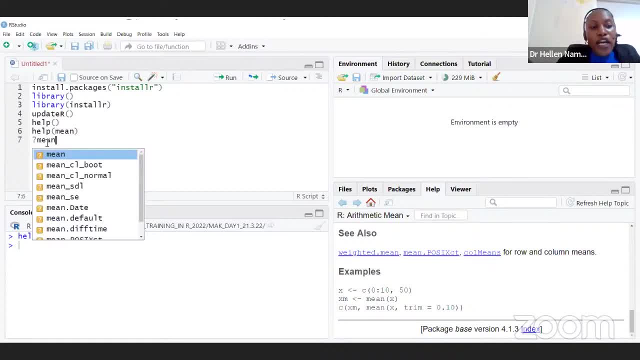 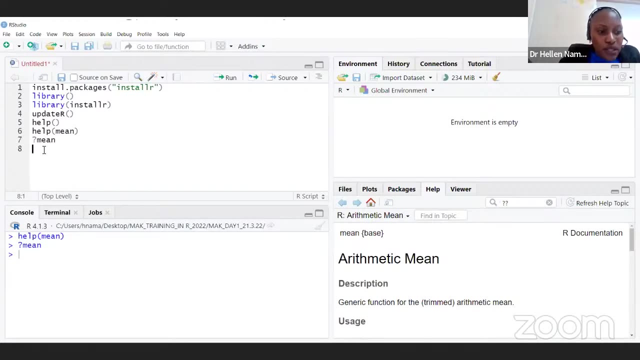 type a question mark and then in front of the question mark, you write in whatever that you want more details about. if you click on it it will still give you see result. or, for example, you can say: maybe i need the help on how to use the, let's say, the t-test. 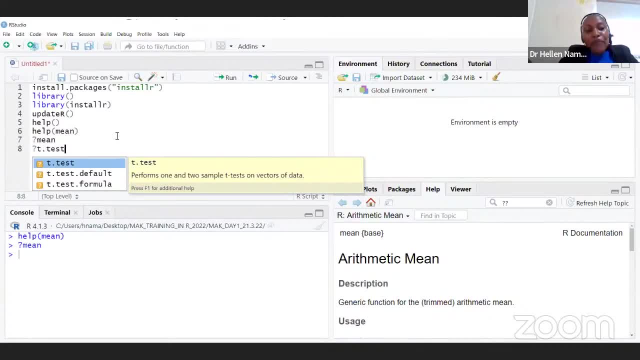 the moment you type that, sometimes automatically, r will tell you what happens: that the t-test performs one and two sample t-tests on the vectors of data, or after that. you can also, in case you want more details, you can click on it on the, on the command at the end of the line and click run. 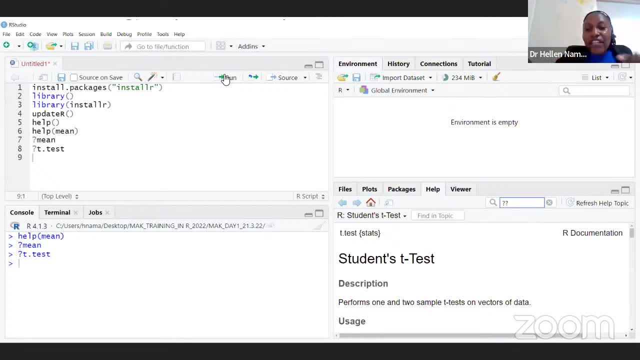 the moment you type that, sometimes automatically, r will tell you what happens, that the t-test performs, on at the end of the line and click run. your mind should run directly under the hope window, because that's where everything is happening- and it will tell you that it's a student t-test. it will give you more description. it will. 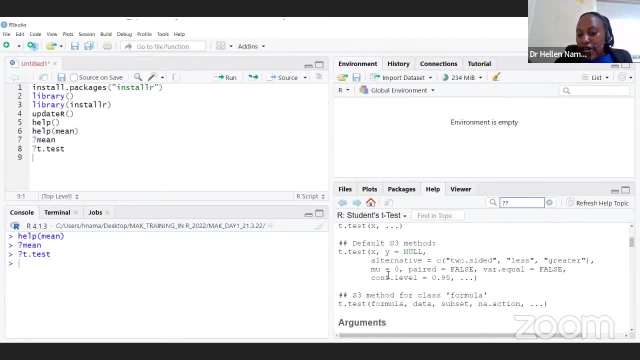 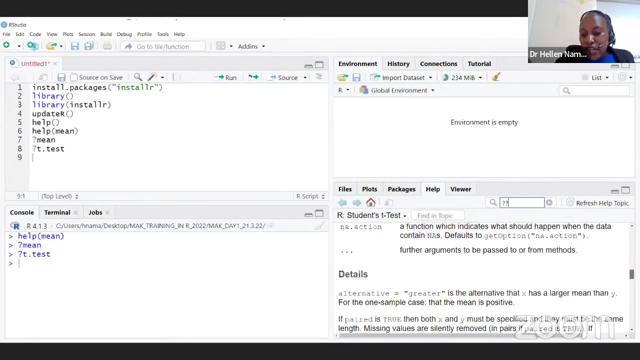 give you the usage, what the different arguments inside the command, the, the ones that can be applied, as well as there are various explanations and what they mean. it will show you more details and it will find that go ahead and give you various explanations toятся going and that 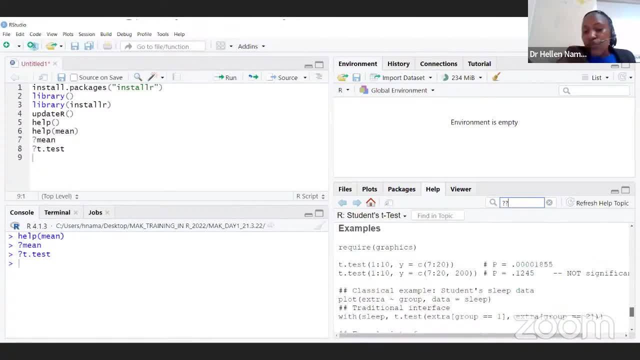 give you various examples at the end. Most of the time at the end when you scroll down in the help window, it will give you examples that can support you to understand the command very well and then thereafter you see how you now you can apply it direct on the data set that you have. That is the 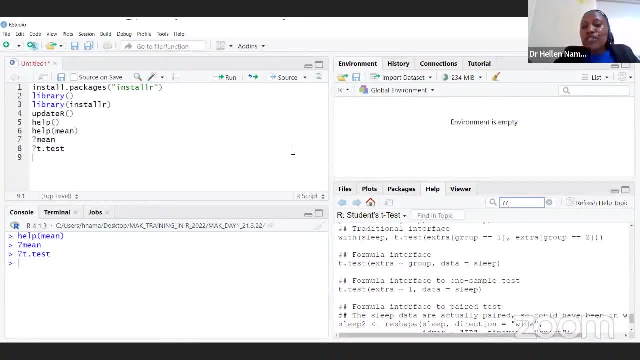 that is the help, the help command, because as you move on, at one point in time, when you're trying to build more confidence with a package with our programming language, you might get stuck. but then, if we can use the help command, there are inbuilt documents that support us to understand. 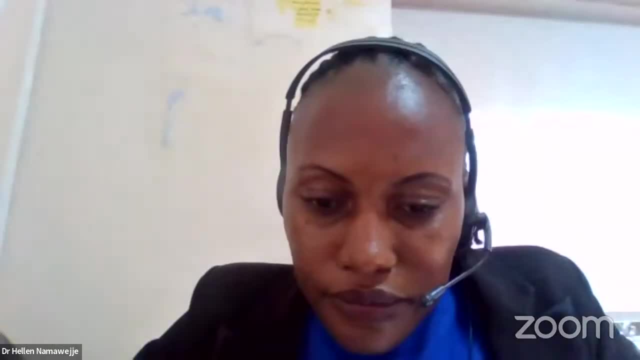 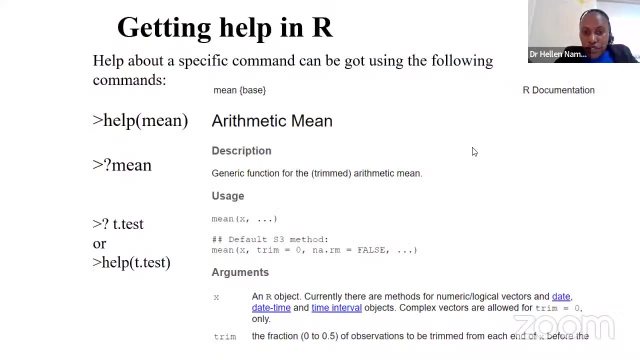 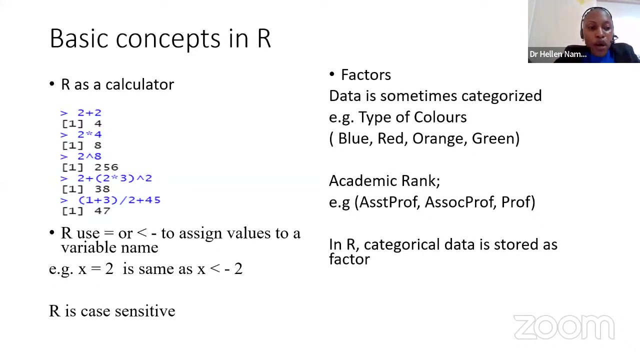 how we can use these commands. Okay, I'm sharing back my word document. that was the help, so I can move on. Also, the other thing, what I'm saying: we are saying that you can do some basics in R. For example, R can be used as a calculator. you, in case you, want to assign variables in R. 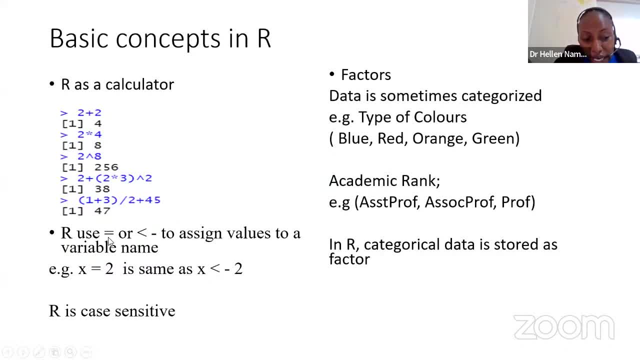 you can use an equal and we use an equal sign or a less minus sign to assign variables. Like I've been mentioning, R is case sensitive. if you use a capital S somewhere, then don't read somewhere and change to a small a, because it will not it for it to look at it as a new variable. 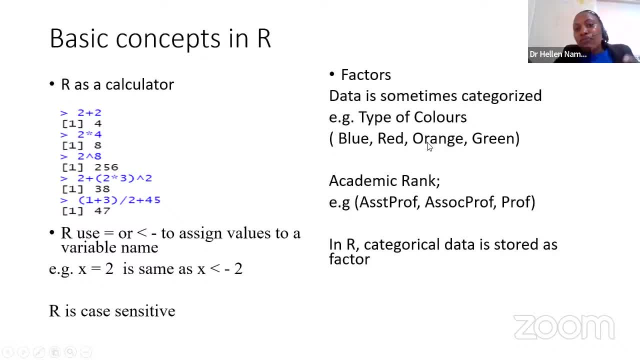 Also, the other thing that that is important to understand is that most of the time, before we step into importation of data into R, we need to understand our. we need to understand our variables. For example, most of you- I, in case you moved out for data collection- you've come across categorical data variables. For example, let's take a common 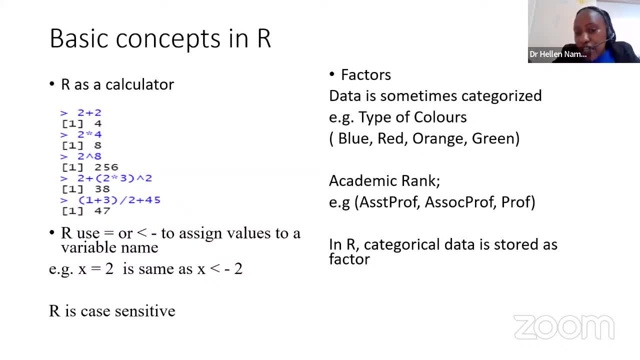 one like like, like gender Under gender, that you are either a male or a female, that is categorical in nature. So that is categorical in nature. So that is categorical in nature. So that is categorical in nature. You can talk about the type of colors and say red, blue, orange and so on. Or you can talk about an 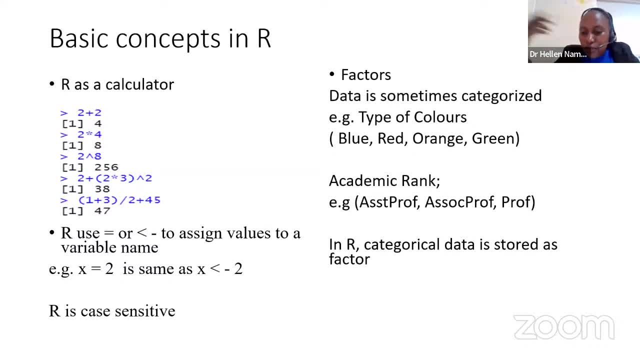 academic rank, like associate professor, assistant and then professor. So all these are categorical value variables. they are just examples, But still you need to tell R that when you come to this variable, in case you're going to analyze this particular variable, which categorical in nature, you need to tell R that it is a, what, that it's categorical. And as we move on, R calls categorical. 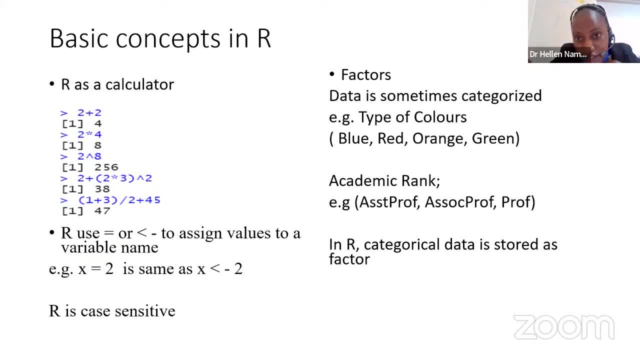 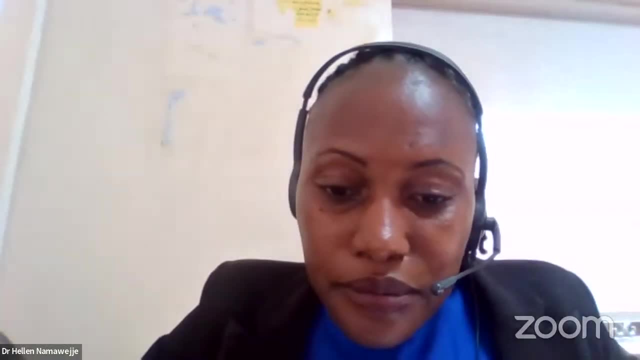 So as categorical value, variables as factors. So we'll have to tell R that we use a fact. let's look at this particular variable as a factor because it is categorical in nature. Let me first go back shortly in R and then we move on. Yes, under here I was saying that. 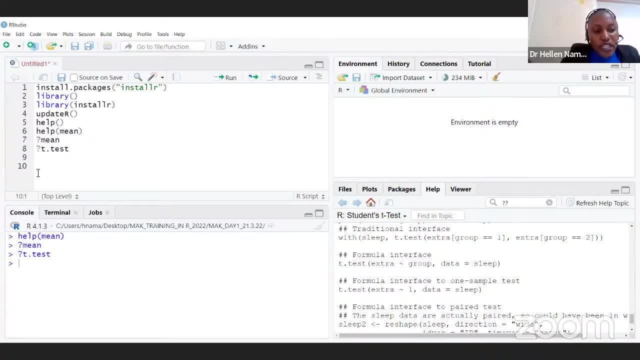 R is case sensitive. For example, you say that it can be used as a- basically, you can say that it can be used as a- basically whatever that you want. Maybe you can say two plus two. All you need to do after writing whatever, whatever that you want, you you click the, the run button and 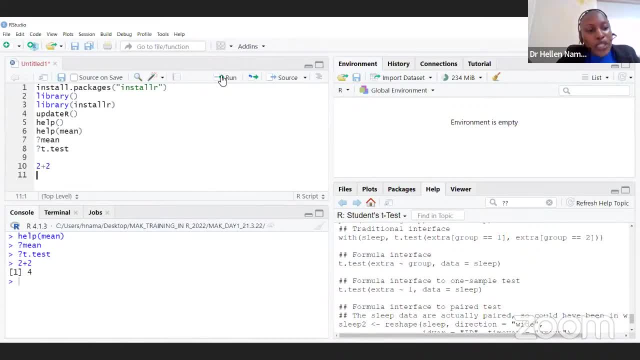 you're going to see the output in the R console. So it will tell you the code that you've written and then the output. all right, Maybe you can say that six, maybe plus eight and then and then minus four, All you do that. after writing you come and click the run button, Like I said within. 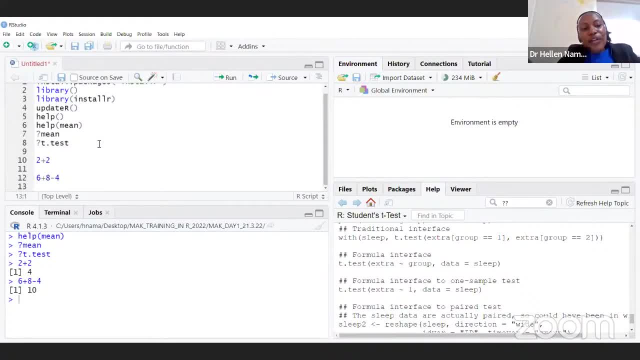 R studio. we write the codes and then the results are executed in the R console. This, this bottom window here it's R console. I say that R is case sensitive. Sometimes you might want to assign variables. You can say that maybe age. if it's your variable, that is equal to 20.. So the moment you run, 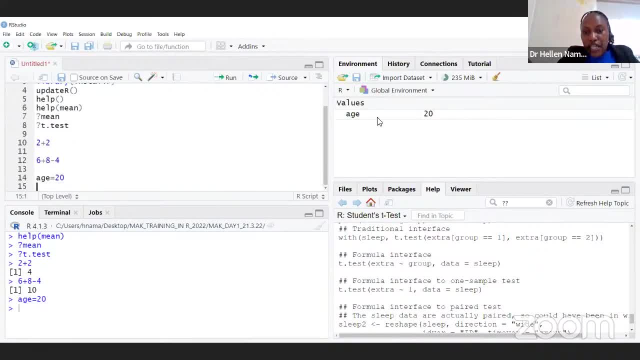 such a variable and you look in your environment, R is going to store a rate that okay, I've seen a variable age and it has a variable age. So it's going to store a rate that okay, I've seen a variable age and it has a variable age. 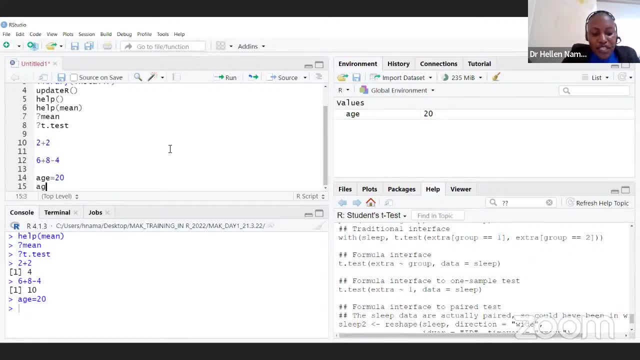 a value 20.. And the moment maybe you say that age- uh, age plus maybe three, because it is already stored on your second line- The moment you run it, when you check in your R console, it is going to pick what you stored earlier and then it it, it gives you the final answer. In this particular case it's age. 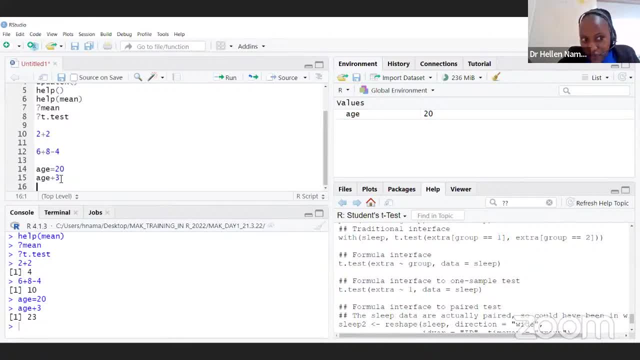 plus three, It picked the 20.. It added the three. However, for the case of sensitivity, in case you wrote capital G And you say that this one is equal to 20.. R is going to look at this particular line and then the one with capital G differently because it is case sensitive. So you have to ensure that. 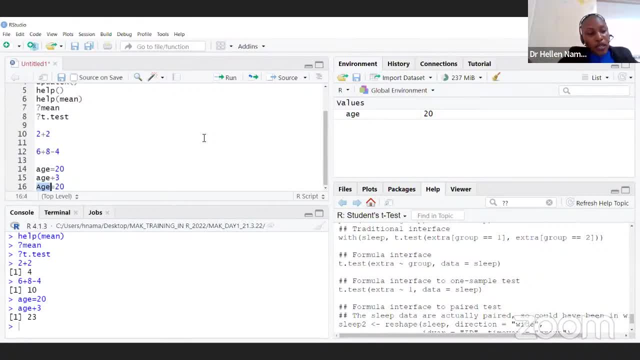 you are consistent as you're writing down your commands. And the other thing: in case you don't want to use an equal sign, you can assign a variable by saying a type in the list and then you say 20.. That, this is another variable. 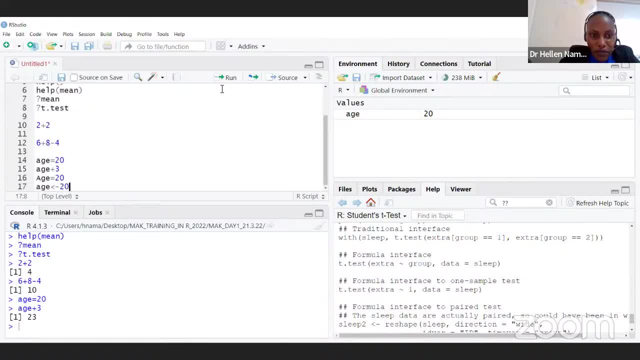 So you can use a less or or dash, But end of the day, this is a good example of how you can write that particular code of assignment And the moment okay, let's say, and say, maybe we say, let me change, let me add something else. like that, you will see the difference. 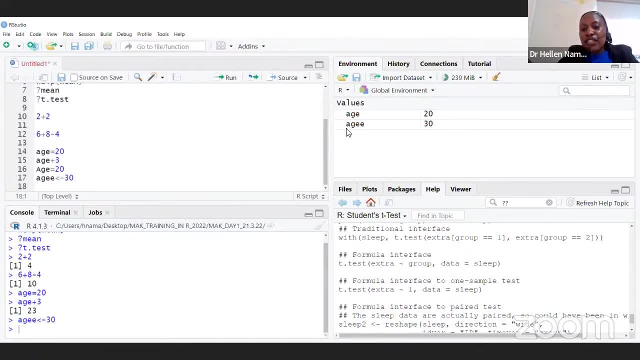 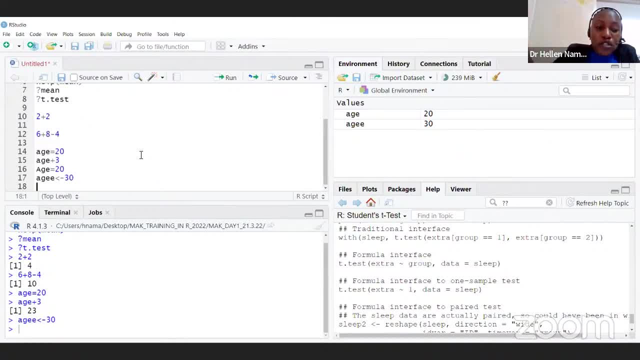 But end of the day you can use a less or or dash. As we advance in this week's training, we are going to see these words are going to be used all the time. Can you assign a particular variable? You assign it a, b, c and d. 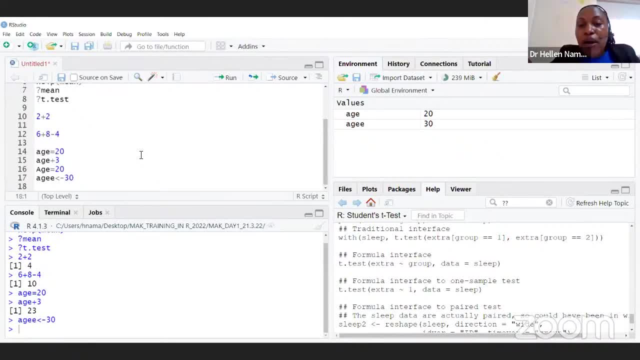 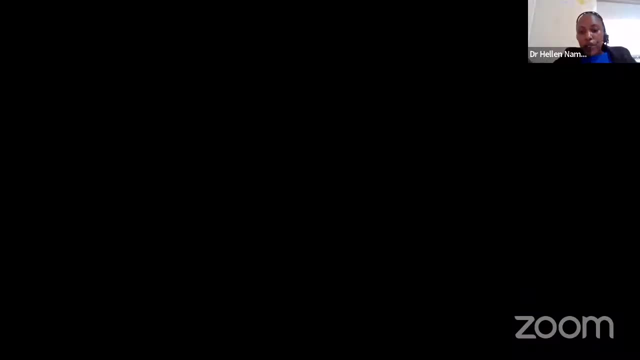 The moment they talk about a sign, what should come at the back of your mind? that you can either use an equal sign or a less dash sign. Okay, I'm getting back to the slides, All right. so this part of factor, we are going to look at it when we get r. 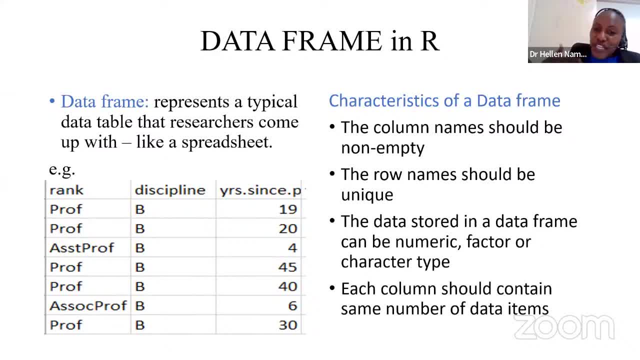 Now let's move on. It is also interesting because most of the time what happens with data is that we go to the field, collect data, put it in excel and then later we import it into r- only import it into any software. So r looks at different data sets as a data frame. 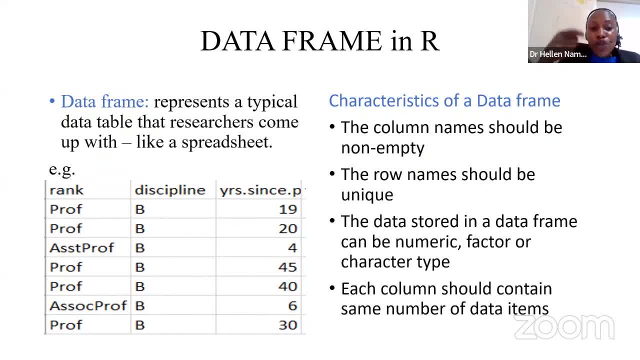 So a data frame is the language with r, So it represents a typical data table that a researcher comes up like a spreadsheet, For example, in case you, you're seeing on ours on the screen, I've got a rank as my variable, discipline as a variable, and then, yes, since PhD, 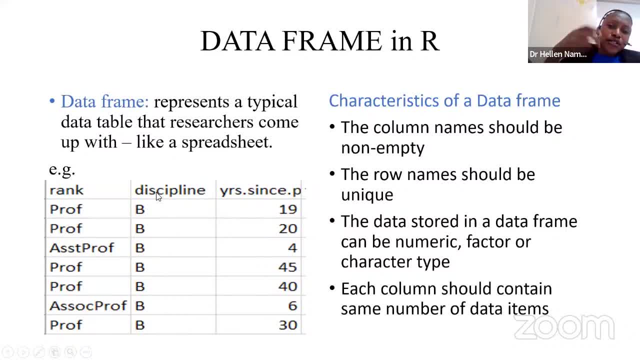 This was just data set from remember r as a programming language. It also has field data sets that can support you as you want to learn more things. So this is a data set that was picked from one of the data sets from our website. So it has a rank of a professor. it has a rank variable which is categorical. 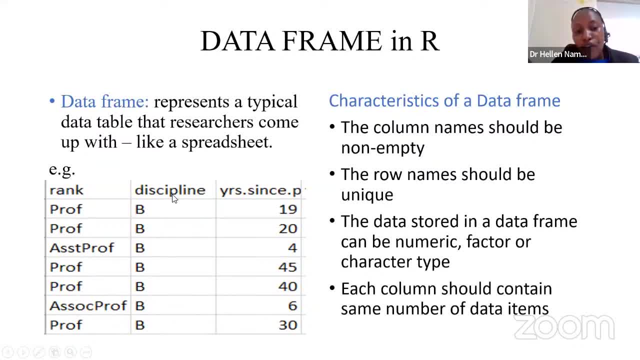 It has professor, assistant professor, then associate. It has a variable of discipline which has B and A, And then it also has yes, since PhD. these are numerical in nature. We are going to see. how do you read such variables in R. 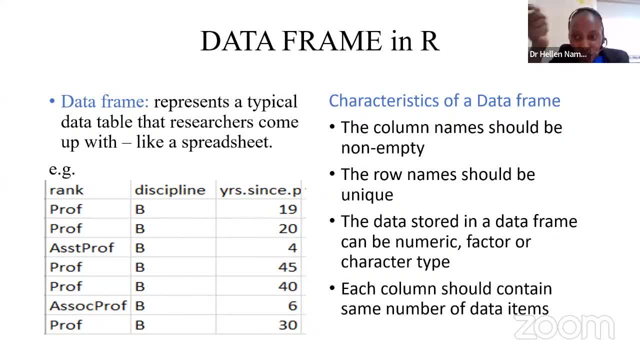 It's always important to understand the characteristics of your data frame. The moment I talk about a data frame, just have at the back of your mind that it is a data set. R refers to data frames as a data set, The data set that you're going to use. most of the time. the column names should be non-empty. 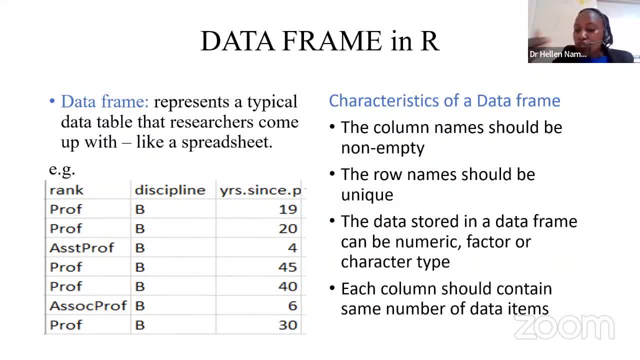 And then the row names should be unique. Those are the respondents that we get. And then data- The column names stored in the data frame, or call it a data set can either be numeric, can either be a factor or a character. 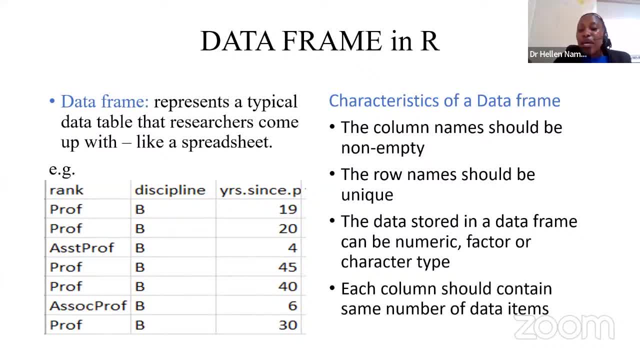 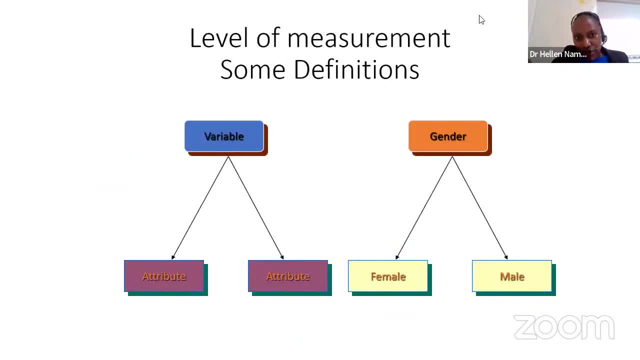 And then we are saying that each column should contain some number of data items. So we are going to look at that. Now, when we move on to the level of measurements, it's also everything rotates under the same thing: understanding your data. 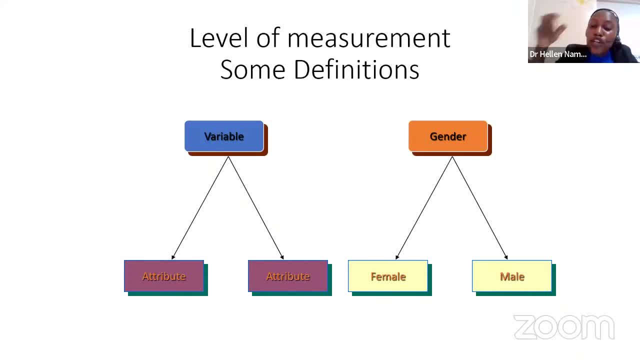 It is very important that before you do any analysis, you know what your data is all about. I was talking about A variable. maybe you're the variable in this particular case. I give an example as a gender, And then the attributes are being involved. 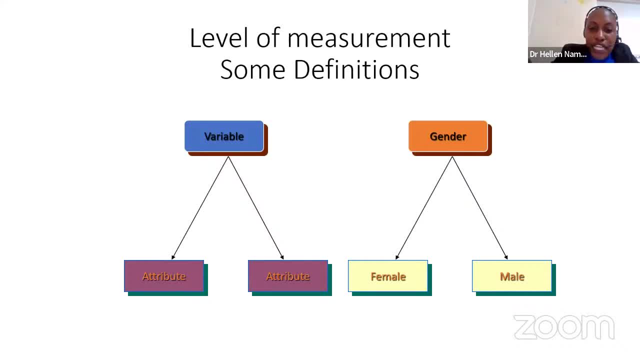 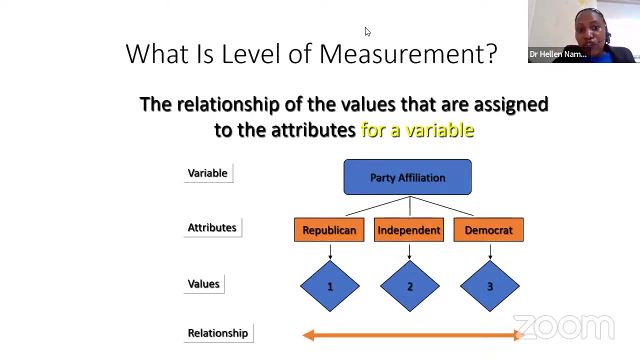 These are the various levels of that particular variable. like for gender, it could either be a female or it could be a male. I talked about colors, which has good. you can have the different colors that you are interested in. Another example: when we are looking at the level of measurements, it is important to understand the relationship of the 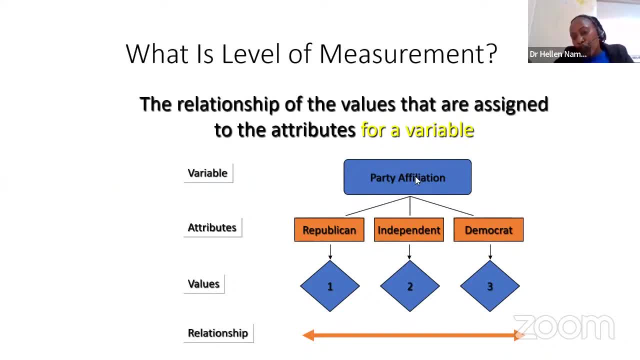 values that are assigned to the attributes of a particular variable. For example, maybe sometimes if your variable is party affiliation and the various levels or the attributes, one could be a Republican, could be independent, could be Democrat, And then you can assign ones, because there are some packages, for example now in R, you can work at both levels: either you leave the names there as attributes or you can use the what, you can use their values. 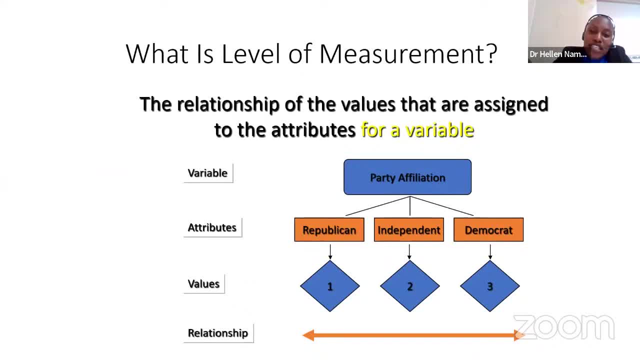 But when, at the back of your mind, you know That when I'm executing my code, one means this, two means this and then three means this, so such that we're able to see that particular relationship of the between the values assigned and then the variable that you have. 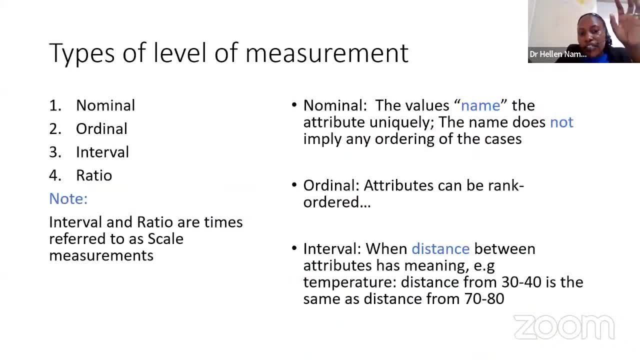 And it is also important to understand that. the types of levels, for example, everything is back on the data sets. like I mentioned earlier, before even you move to go to the field, what variables Are you going to collect among the levels of measurements? we have the nominal, the ordinal, the interval and then the ratio. sometimes the interval and the ratio are referred to as scale measurements. 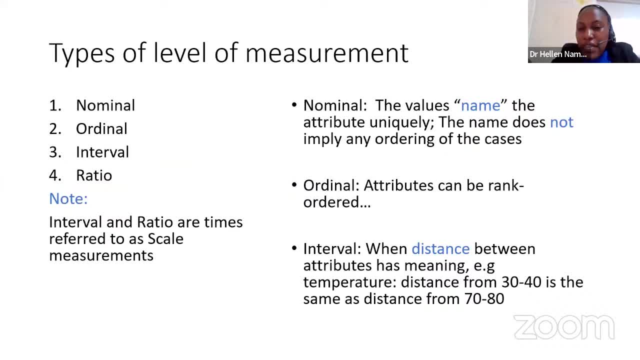 And in case your variable is nominal in nature, it implies that the value of the name or the name doesn't. there is no orderling. no orderling is. orderling is not important. so the name does not imply any form of ordering. it doesn't matter. for example, maybe if you're talking about 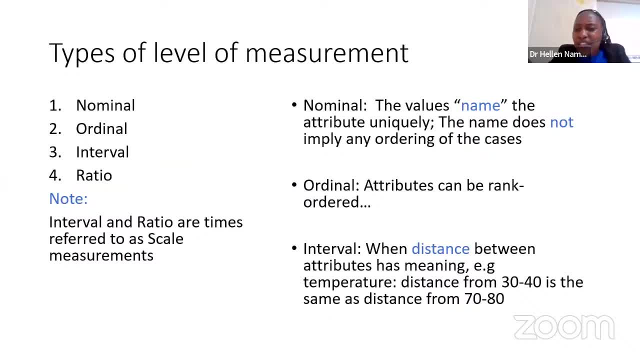 gender. You can say that gender is nominal in nature, because there's nothing like order. whether the first one is a male or a female, it doesn't matter. talk about colors, talk about types and so on, Whereas with ordinal variables, in this particular case the rank or the ordering is very important. so you need to check that in case I'm collecting my particular variables- does this particular variable have any kind of ordering in it such that, as you analyze it, 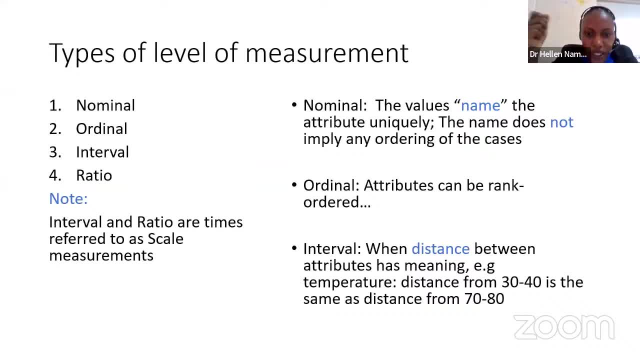 also supports the kind of analysis that you're going to do. For the case of the interval and the ratio I talked about, you can look about the distance in between. maybe, in case you're looking at temperature and and you get to, you're looking at temperature maybe. 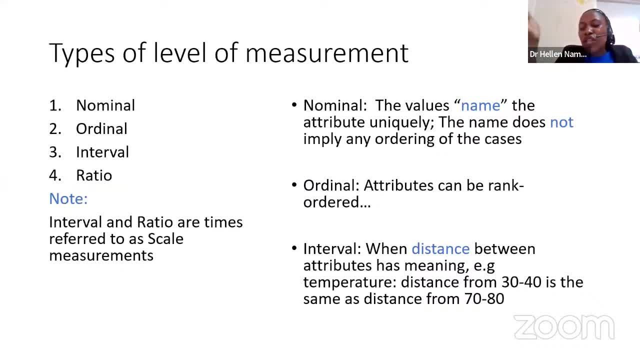 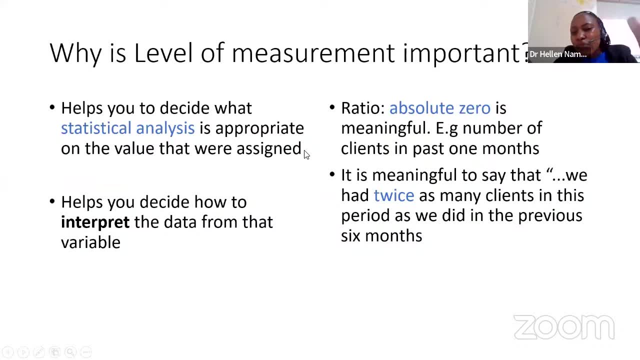 And then you're looking at also the distance between certain points. maybe between 30 and 40 is the same distance from 70 to 80. Okay, so why is it important for you to understand the different levels of measurement? Like I mentioned, it helps you to decide what statistical analysis is appropriate for the study that you're going to do. 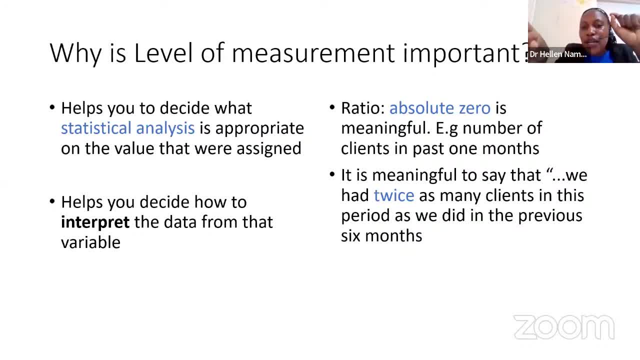 Otherwise, if you don't, you'll end up doing wrong analysis. Remember, you're feeding into R. whatever you feed into R, it will give you a result Most of the time. if you feed in wrong results, automatically, you'll come up with wrong things. so everything starts on your data, the data set that you're having. 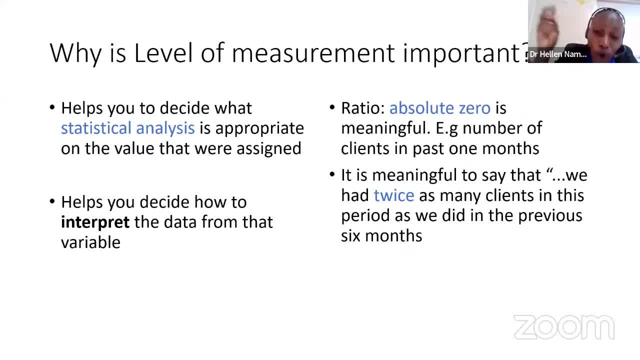 It will help you to decide the kind of analysis you're going to do and Also, how are you going to interpret your result, because it is always important after getting the results. you've gotten the right analysis. you've gotten the results or the output? how are you going to explain them? 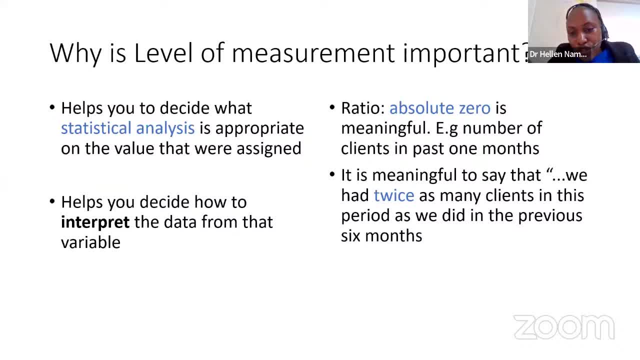 There are some variables. for example, when I talked about the ratio Under ratio, an absolute value is very important. Maybe you can say: we did not receive any client in the past one month, so implying that it was zero clients. so in that particular case it's very meaningful. 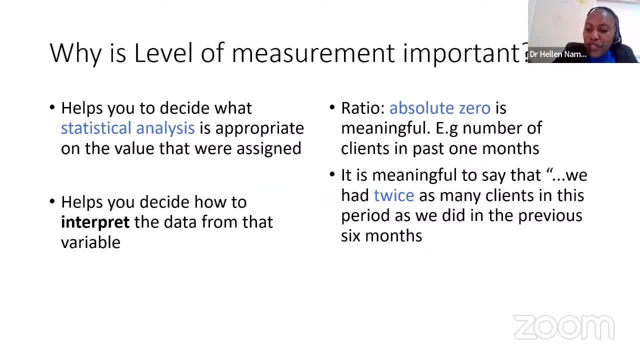 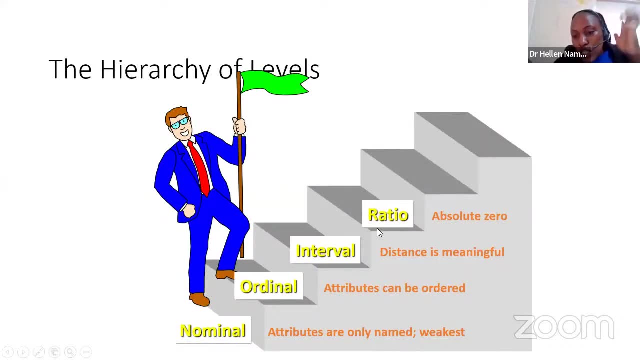 So still in your data collection, if your variable belongs to a scale, does maybe a zero have a meaning or it's a missing data point. So under the hierarchy, the different levels, all you need to understand in your data set: is it nominal, is it ordinal, is it an interval or is it a ratio, Interval or ratio, those are scales. so most of the time, with the nominal or the ordinal, 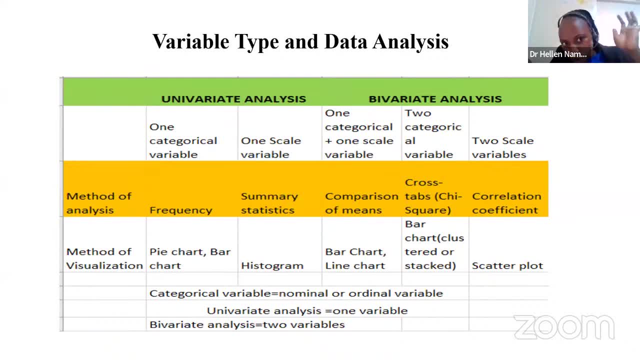 we are going to have a scale, So you need to check whether they are categorical or not categorical As we move on. it is also important to understand the variable type and the data analysis that we are going to do. We are going to see all this in this particular week because now we've moved on to how to analyze a data set. 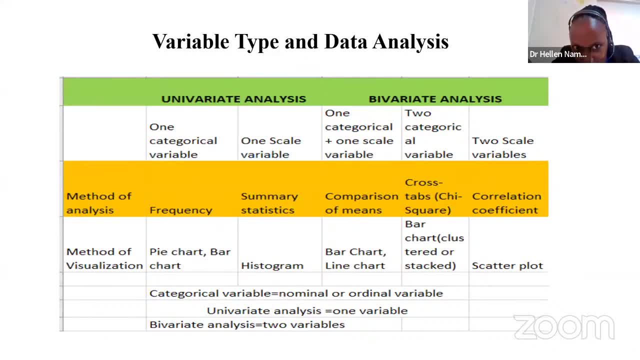 Okay, we're having what we call univariate analysis, In case uni means one, and you need to understand within my data set is the variable type. Okay, we're having what we call univariate analysis, In case uni means one, and you need to understand within my data set is the variable type. 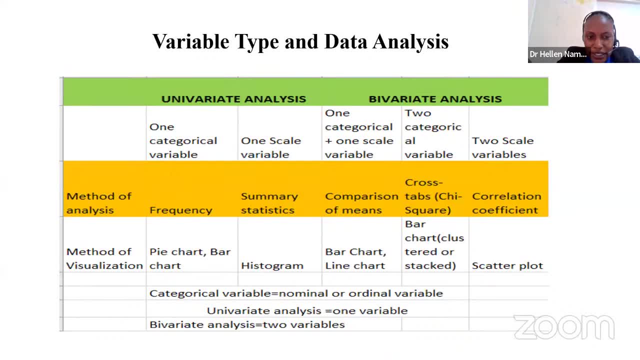 Okay, we're having what we call univariate analysis, In case uni means one, and you need to understand, within my data set is the variable type. So a variable I'm considering is it categorical or is it a scale? If it is categorical, then what method of analysis am I going to use? 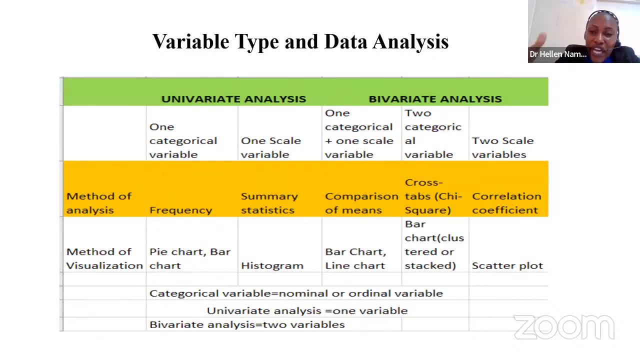 These things should be on your fingertip, because it is the basis of all the analysis. It doesn't matter the field you're in, whether you're in agriculture, whether you're in economics, whether you're in social sciences, but all these things apply the same principles. 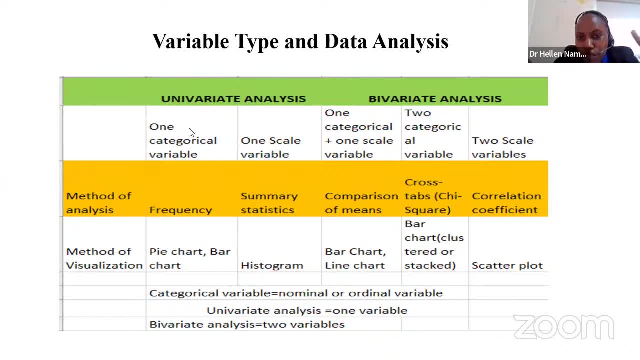 For example, in case you're doing one categorical variable- we are going to see this in more detail- The method of analysis- you're going to run frequencies and you're going to get percentages, And you can represent one categorical data visually with either pie chart or a bar chart. 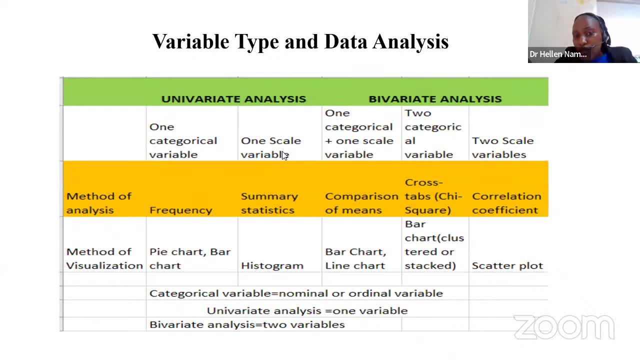 If it is one scale variable. for example, let's talk about age. In case age is not categorized, you can do a summary statistics as the method of analysis And then, with visualization, you run a histogram. That is for the case uni. 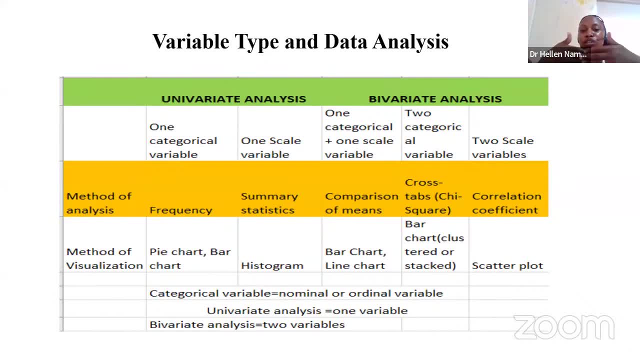 You can have like 10 variables, but sometimes you need to first understand what is the behavior of the variables that I want. Then, after considering one at a time, With bivariate, as we are going to move on, we are going to see in case you're using one categorical and one scale variable. 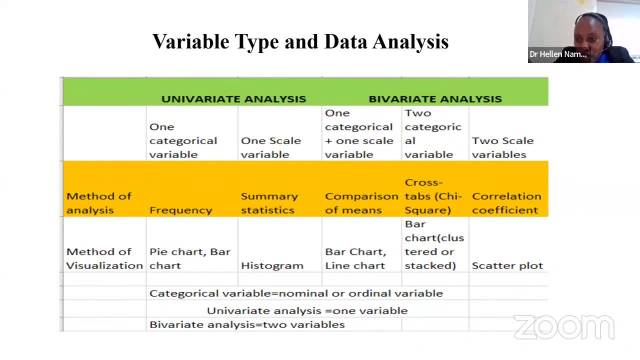 we are going to run the method of analysis is compulsion of means or an over analysis of variancy, And most of us- I think you've heard about this particular bit theoretically, Maybe during the lectures or in class, but now we are going to see how we do it in R. 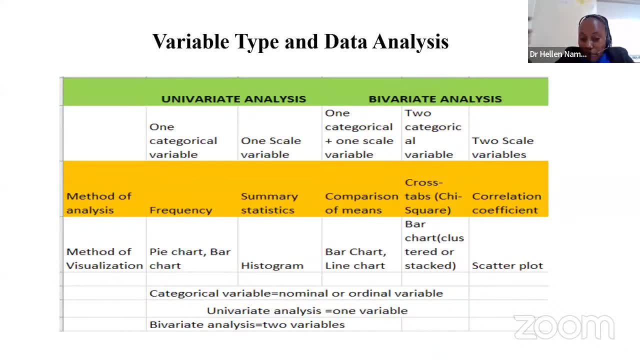 And then with visualization, we can do a bar chart or a line chart. If you're having two categorical variables, we do what we call a cross-tabulation or a chi-square. This is what the director was talking about- And then visually you can have the bar charts that are clustered or stacked. 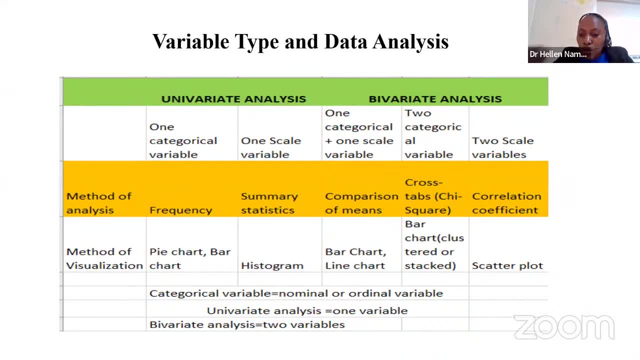 And in case of two scale variables, we are going to do correlation coefficients, the Pearsons and so on, And visually you can have a scatter plot. So basically, when it comes to nominal or ordinal variables, most of them are categorical in nature. 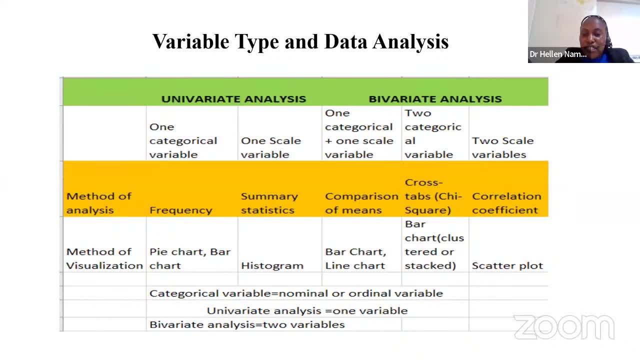 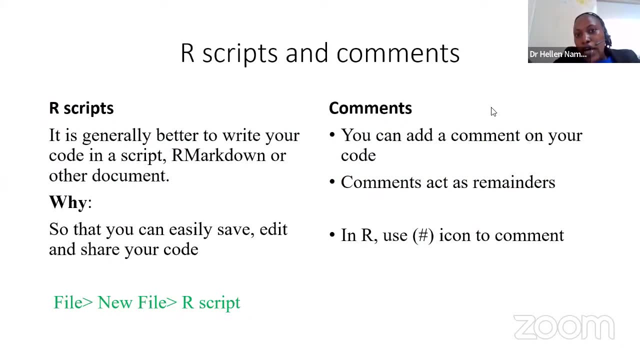 But you need to distinguish between the two. With the invariant analysis I said it is one With bi, you're looking at relationship between two variables. Now, as we try to move on to R, we're going to see R scripts and then comments. 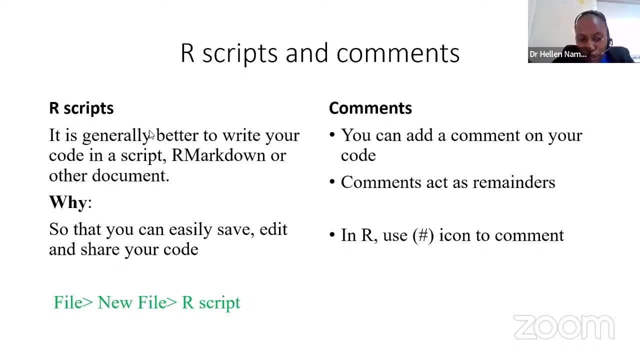 How are we going to get the R script? I've already shown this, but I'm going to show it again How you move to file new script and then R script. So it is also important that, as you're opening your R scripts, 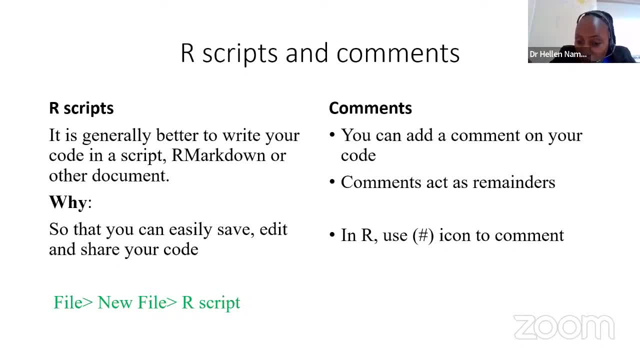 you add comments- The comments the actors remind us they hope you to. Maybe you can take like two days without opening your R file, But in case you had put comments, you can quickly read through and you're able to be reminded and move on very fast. 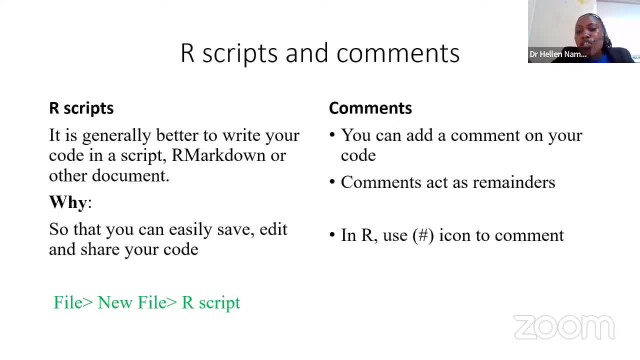 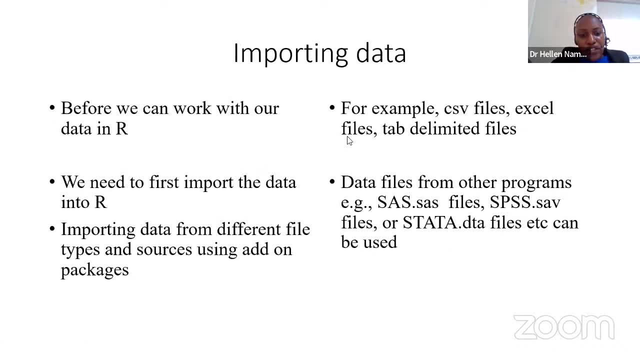 So the comment icon, which is in form of like a ladder. it is always important and we are going to see that in R as we are running. Then here we are saying we are moving on to also something very important: importing data. OK, before we work with our data in R, we need to first import it wherever it is. 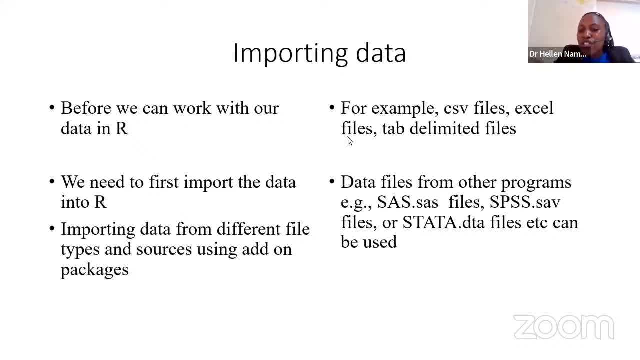 And it's quite interesting. I'm so impressed that even the director knows that you can import various, whatever files that you have and bring them to R different data files. it could be in SAS, it could be in SPSS, it could be in Stata, whatever- because it can work with the various packages. 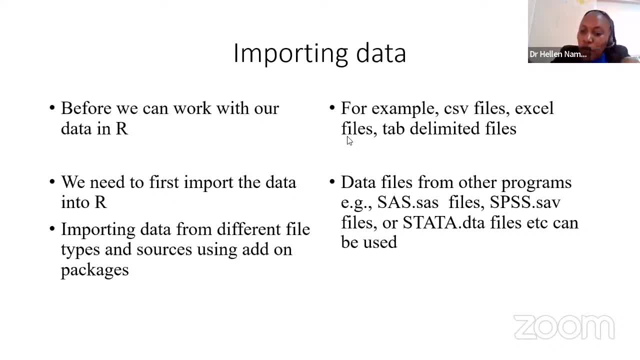 All you need to do. in case you have your data set in SAS, you can import it in R. If you've got your data set in SPSS, you can still import that particular file in R or Stata and you will be able to use. 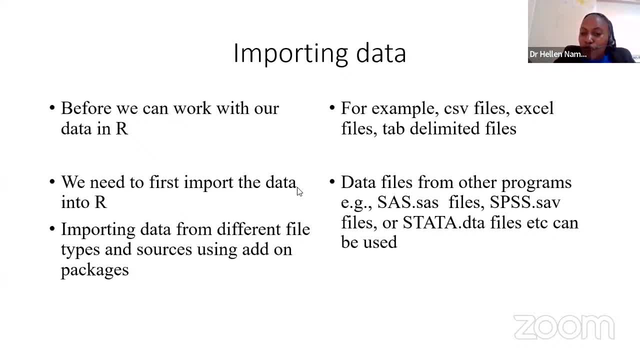 that. So now what is important here is that there are various. there are various ways of how you can import your data in R, But also it is important to understand how those particular files are being stored such that you import them in R. All right, so what I'm going to do? 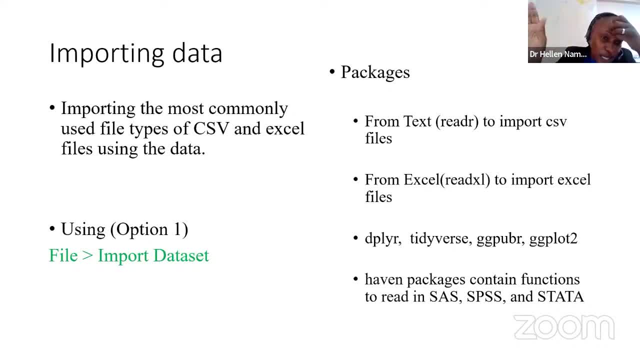 we are going to basically the mostly common used saving styles that we are going to use in R. Sometimes you can save as a CSV or you can save as a XISX, So we are going to see how do we import data in R and in the moment data is 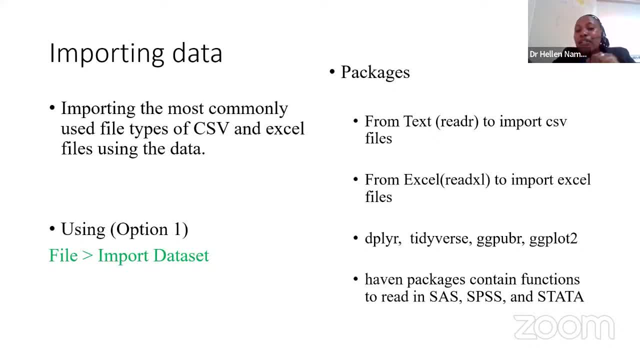 imported. how do we move on with the analysis? Among the most important packages that we are going to use is the read R- This one it's important when importing data set that is being saved with an extension of CSV file in Excel. Then the read XL is the package is going. 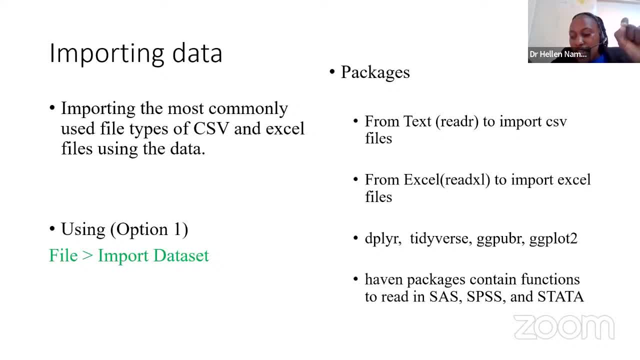 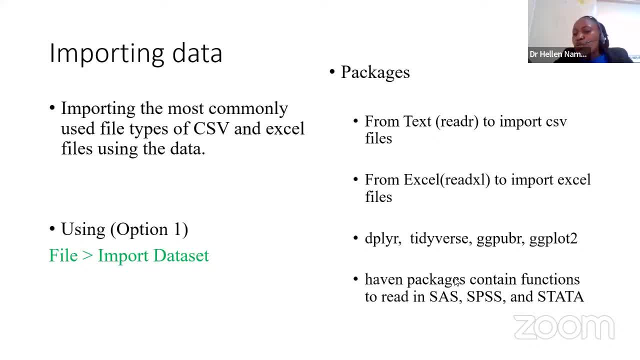 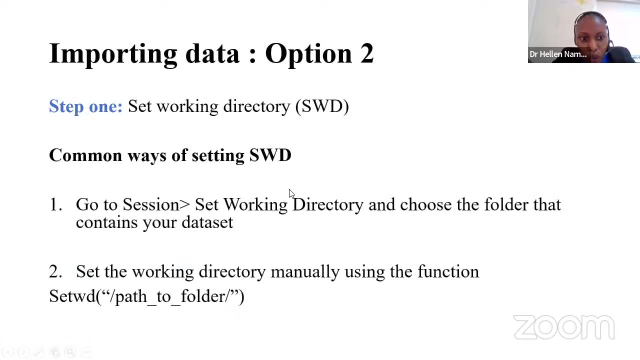 Among others. I've also mentioned that having package also support us in case you're importing data from SAS, SPSS, Stata and so on. But, like I mentioned, it is always good to use a package. that it's it's really that is important for you. Now we are going to go into R and look. 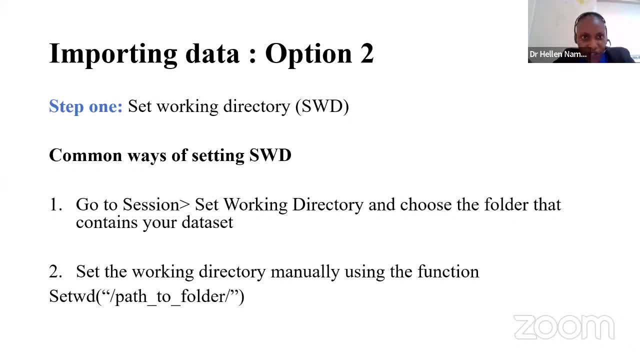 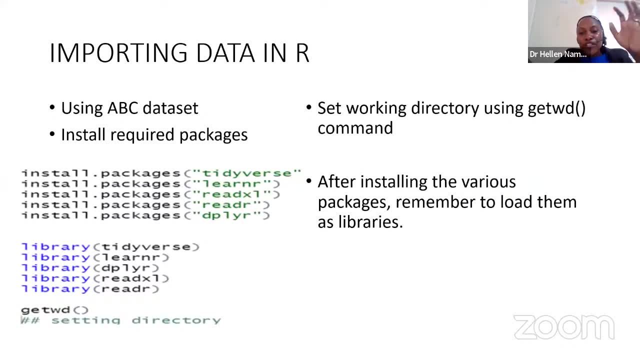 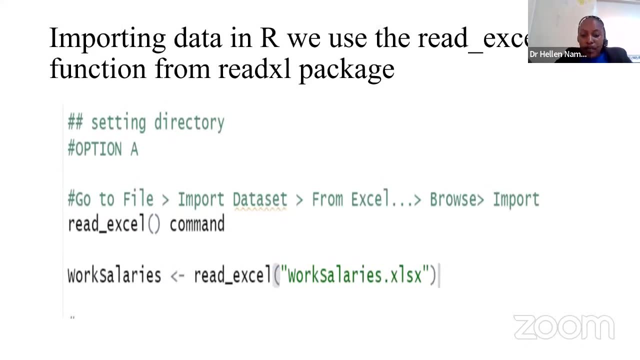 at various ways of how we can import data, Then after that we'll do- we are going to import various types- and then we will move on. We need first installing the packages that we need And then thereafter we'll move on: how we load these packages and do the importation. 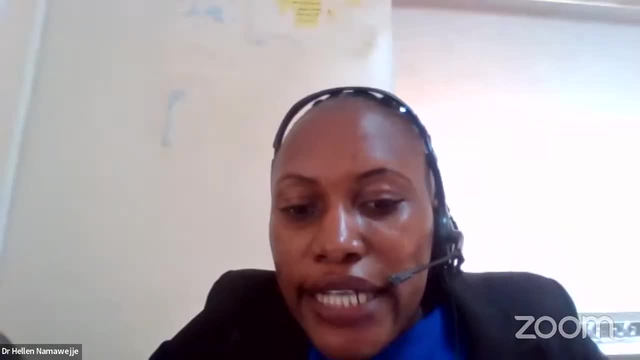 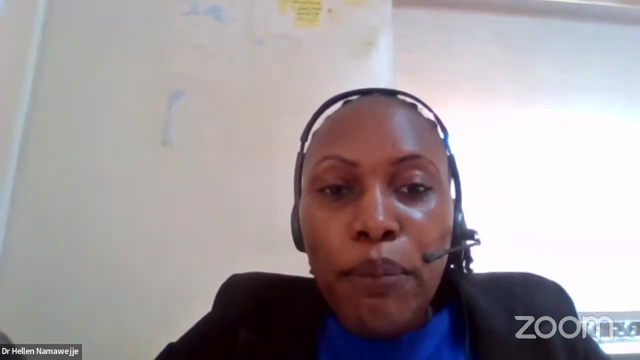 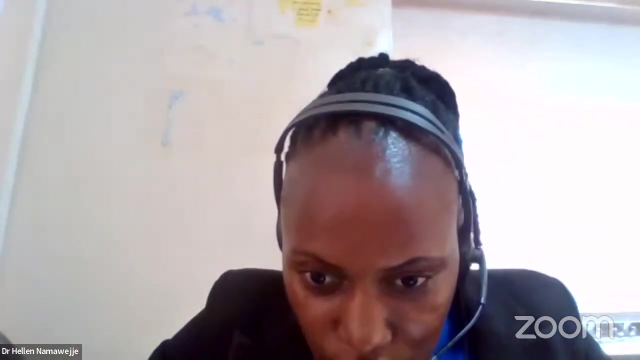 I'm I'm going to close this. I kindly ask you go to the folder that I sent, which has got the one material on your computer, and then open the salary script. it has salary dot R. script is what we are going to use. 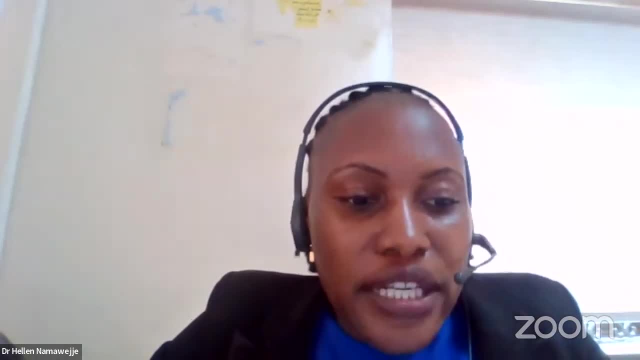 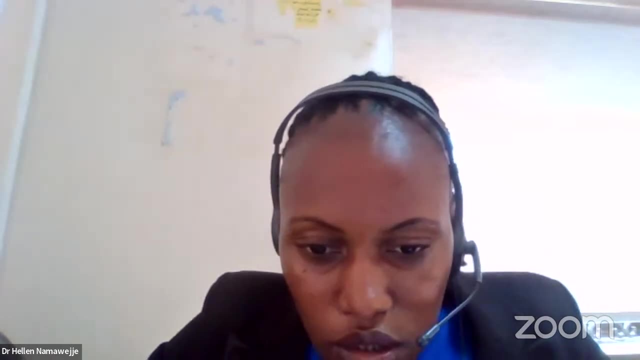 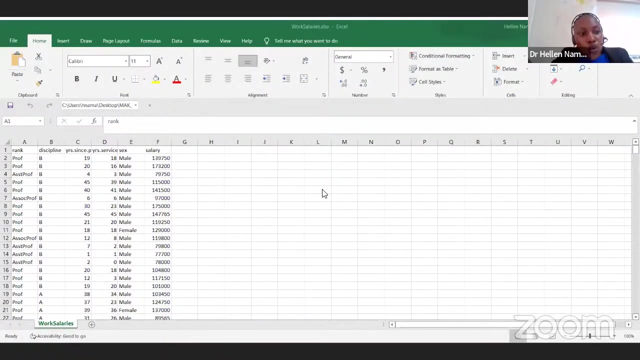 Within that same folder there are two data sets. maybe let me first share one of the data set that is there Within the folder that I sent. we've got this particular data set. It is which I which I named work salaries as the the name that I saved. 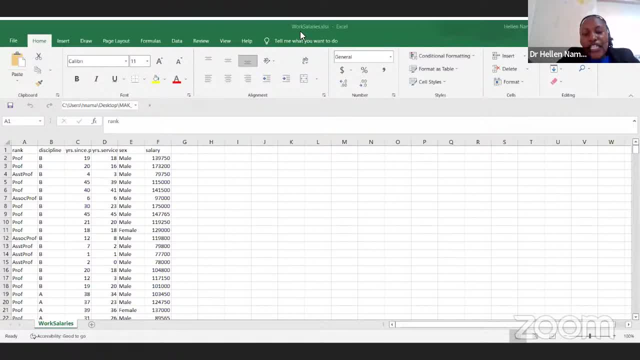 When you look on the top of that particular data set, it has got work salaries dot XLSX. that is the extension file it has. Most of our Excel files are saved with that particular extension. OK, and we're also going to see another, another, still the same, still the same. 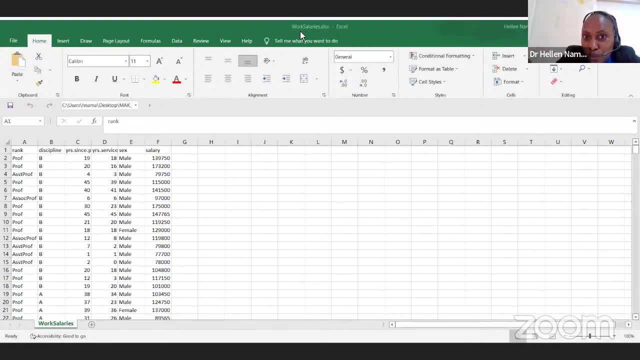 the same Excel sheet, but saved also in a different way. All these things are being done in case you're going to the field and you have you have your data within an Excel file. this is how it looks like it has got. It has got on the first row. 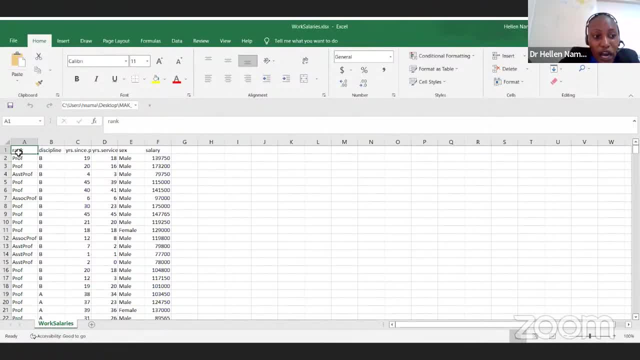 It has got the the description of the variables. we have Look. we have discipline. We have yes since PhD. we have yes, yes Of service. We have sex. We have salary. We are looking at, we are looking at the different factors that affect the salary. 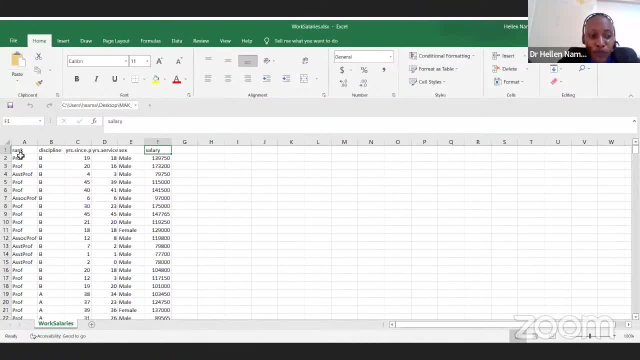 of an academician, especially in the rank of a professor, assistant professor and an associate professor. So this is how the data looks like And it's what we want to import in R, Like I mentioned. just a reminder in the Google Drive. 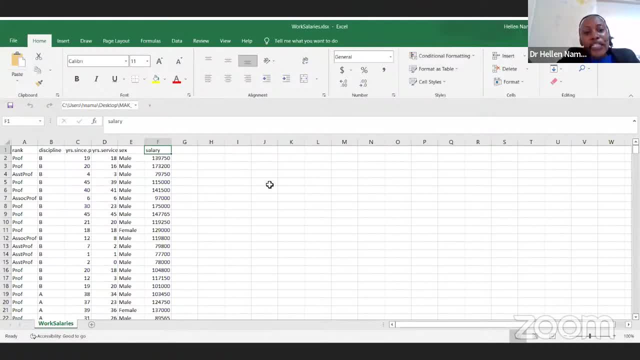 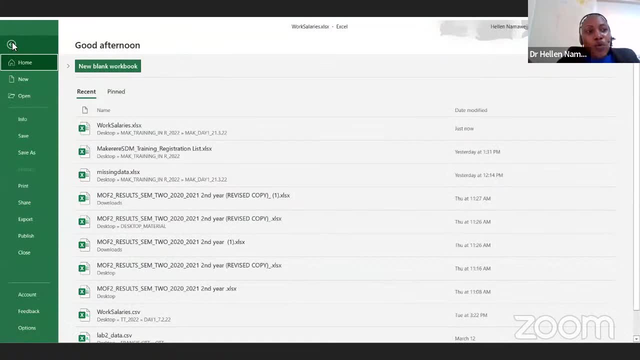 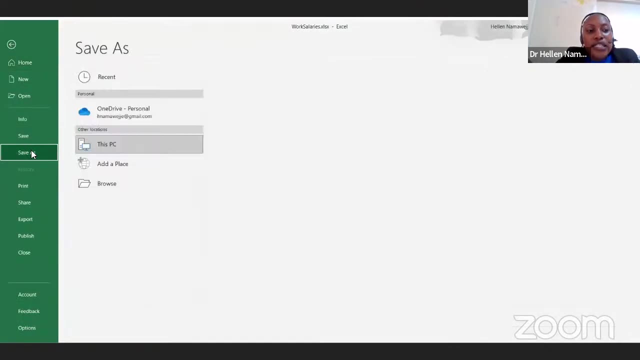 This data set is there, OK in case. in case, you're wondering how this data was saved. most of the time what is happening is that on the top of when you look at this particular Excel, go to file and then come and click save. as the moment you click save, as it will ask. 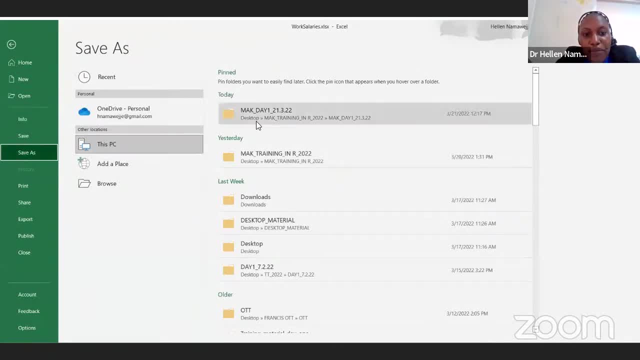 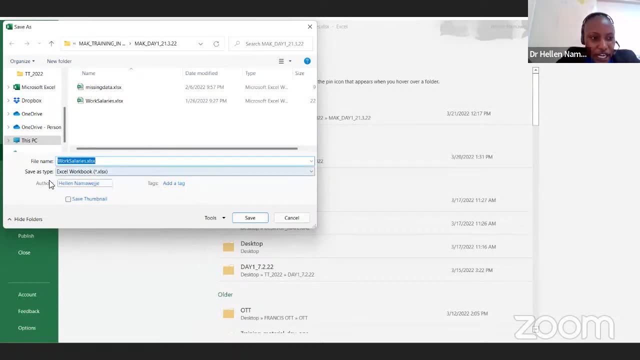 you. where do you want to save your, your Excel from? Maybe I can pick a certain folder on on my computer. When you check the point I'm driving home. It's about the different saving types. When you come here it is showing you save as type. 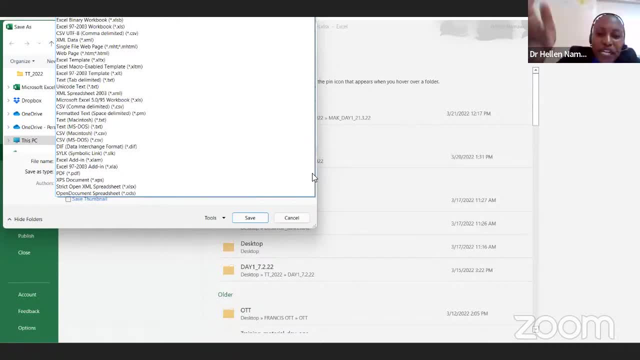 When you click here, it gives you various forms on how you can save your data, But I said, with the common ones in R that we are going to use, we are going to use the Excel workbook, which is that the dot Excel SX. 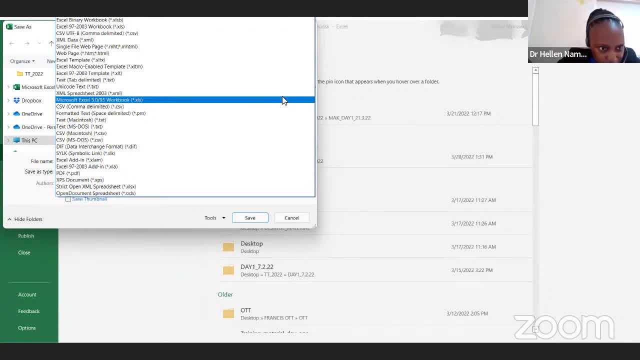 And then we have the other one that is called the CSV, which is the comma delimited, The one that I'm highlighting, And so the moment you save your file, it will have that particular extension. So we are going to work with two kinds of the saving cells that we are having here. 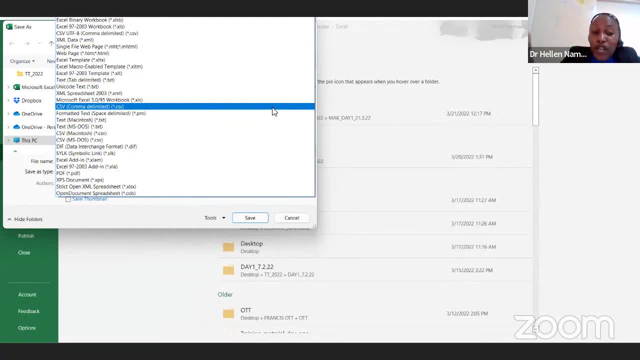 But also, I guess you have your data saved as a text. You can also still import it in R, It doesn't matter. You just need to know what format was my data saved so that I'm able to import it in R. All these things are important so that you are able to know the right package to use. 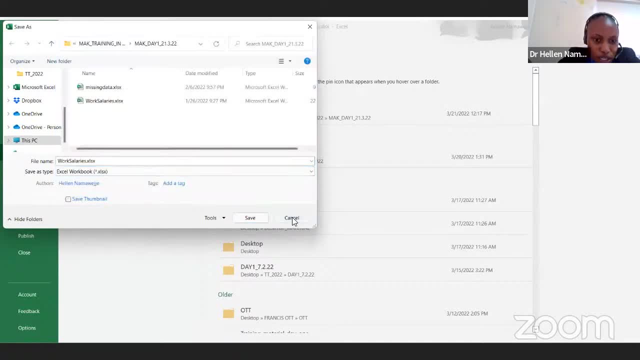 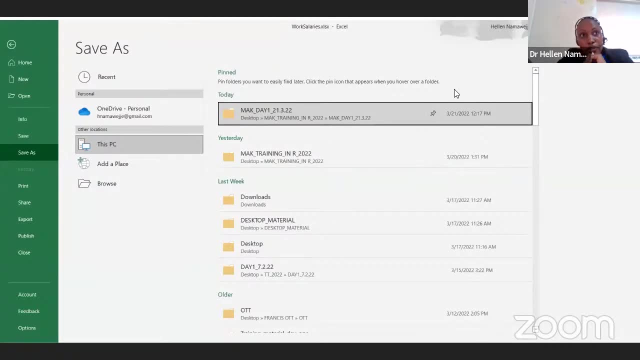 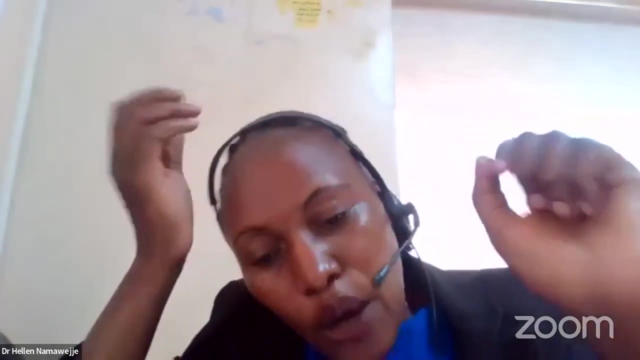 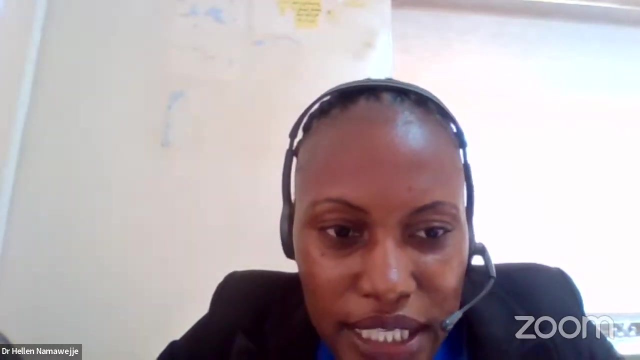 So I'm going to save this as just showing you what to do. I'm going to just cancel that, Sorry. OK, now that I'm going to answer that now in case, still, let me also open the share, the same data set saved in a different style. 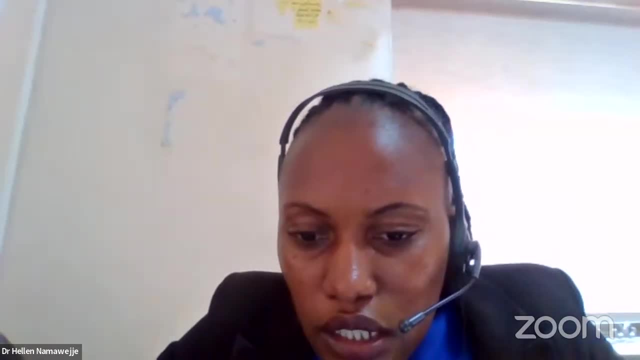 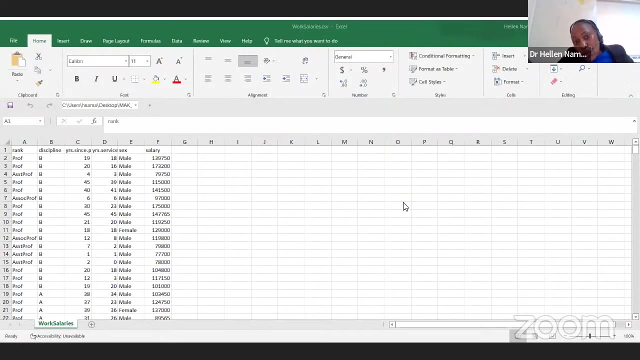 I'm going to recap, to recap that And let me share this, because I share again my Excel sheet. Now, this time around, what I'm showing you, it is the same data set, But when you look at the top it is served as work salaries. dot. CSV, comma delimited. 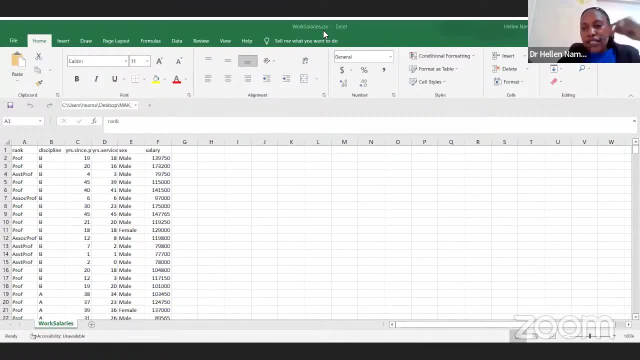 And still, we are going to see how do I import my data in case it's saved as as an, as an XLSX, the work, the workbook, Excel, And what about the one with CSV? OK, somebody is saying that I recap on how to save. 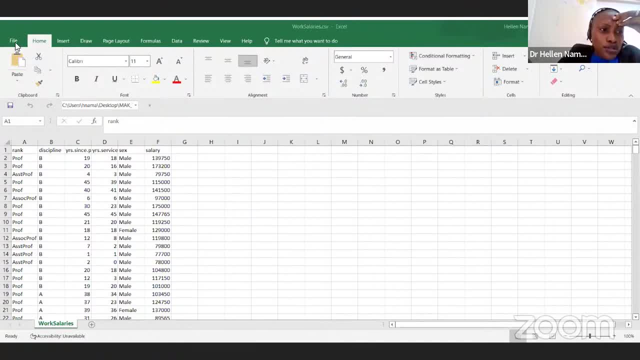 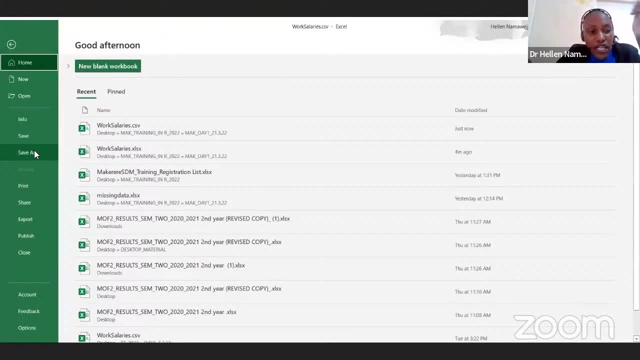 Like the way we've been saving our usual documents. you know all you need to do: go to file. the moment you click on file you- I'm going to use save as, because it is already saved- I click save as I pick any folder on my document. 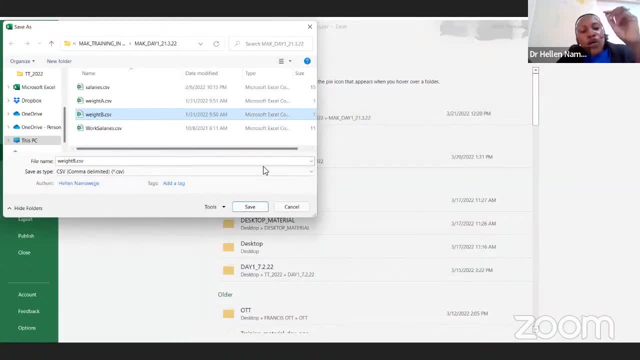 For example, in case I choose that folder Automatically, it is telling me that my save as type It is CSV, comma delimited, which is what I'm interested in. But in case I wanted to change the saving type, all I need to do is come at the end. 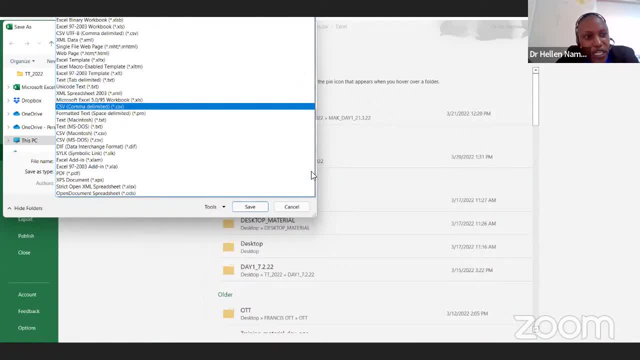 and click on the, on the, on the drop, on the drop down, It will bring you various saving formats that you want, And then it will be up to you to pick the kind of saving style that you want, which that you want to use to support you as you're getting data in in R. 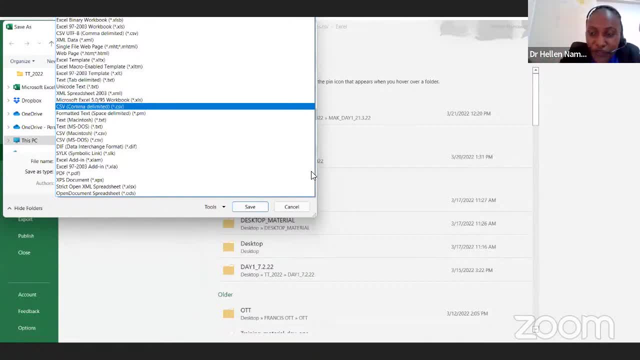 Hopefully that is clear. I don't want to save because it is already saved And when you check in the folder that we sent, it has got both these two files. it has got the work salaries, which is saved with an extension of XLSX and then an extension of the CSV. 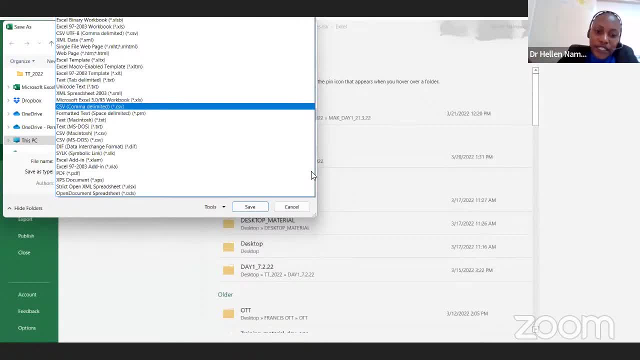 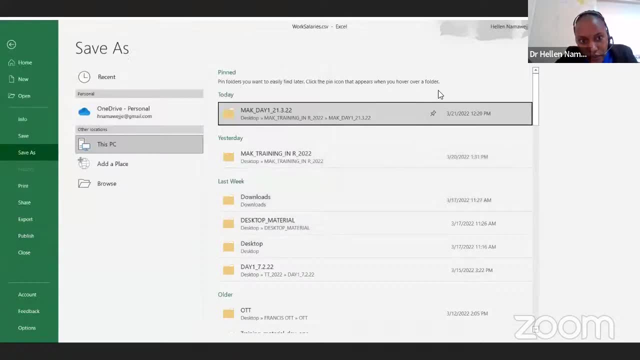 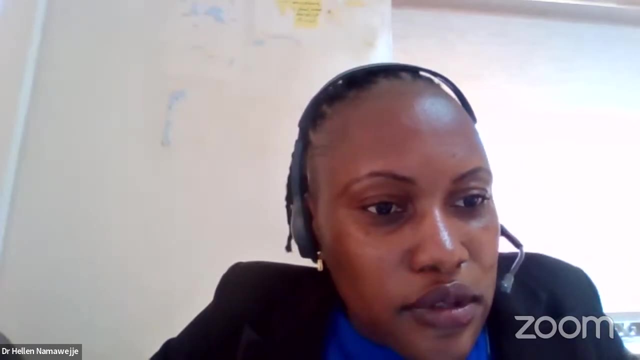 because those are the common one used, one of the ones that we want to learn in this particular training. I'm not going to save, I'm going to cancel and then we'll get back. OK, let me ask in the chat: Can I get video of the lecture? 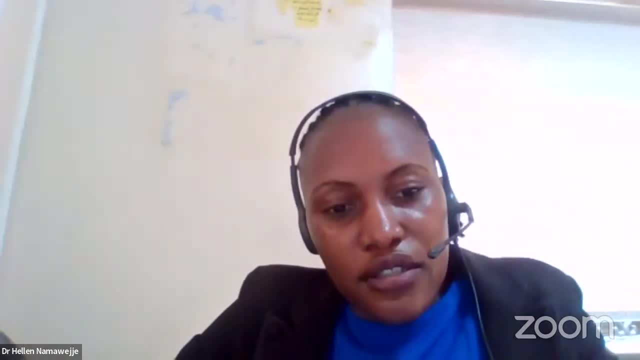 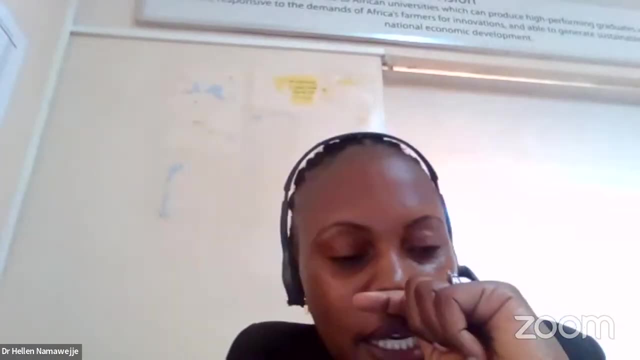 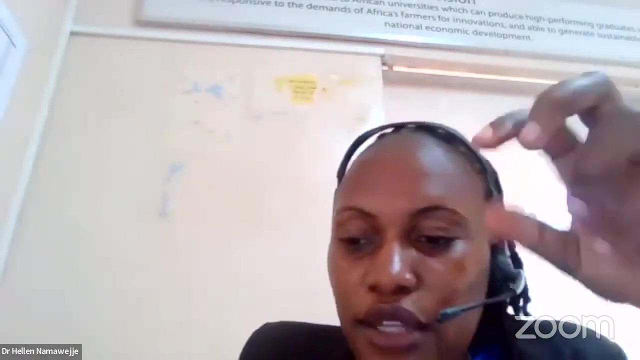 OK, my R studio does not have to run. OK, I will still encourage you. kindly post the questions in the Q&A and you'll get an instant response, Professor Susan and Dr Thomas on the computer answering all the questions that you're posting. 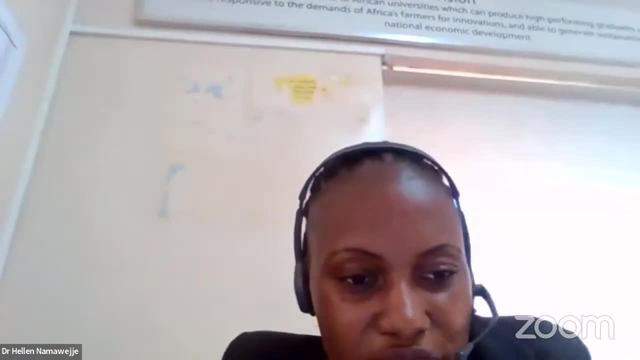 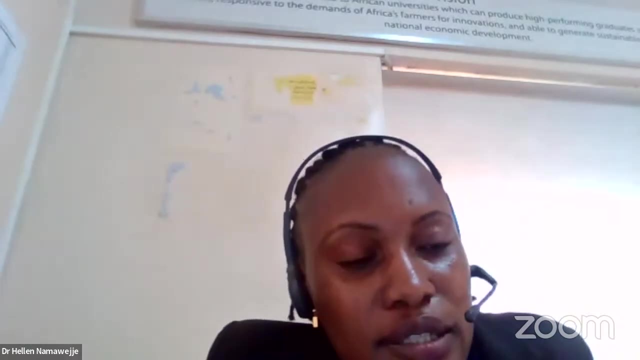 that we're able to move on the same page. So I'm asking the chat: can we now move on to see how we import data into R? Are we on the same page up to this particular state? OK, some is saying that. yes, Andrew, yes, of course. 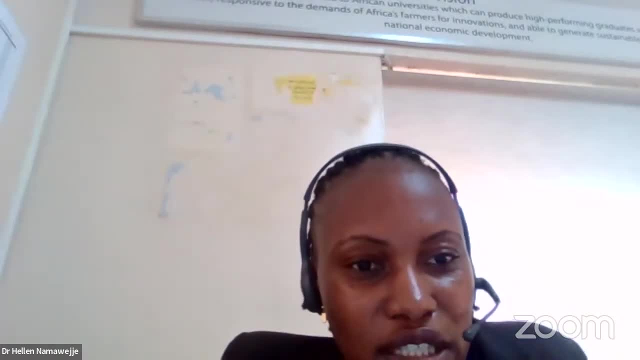 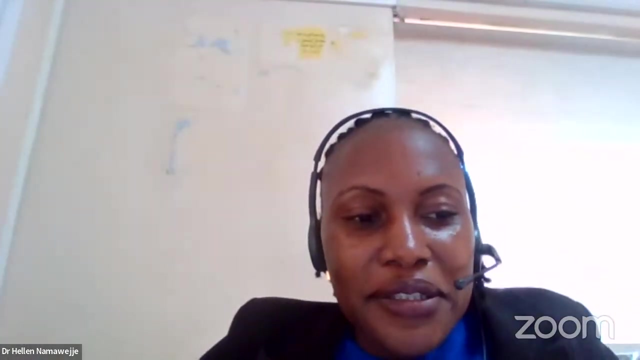 Yes, absolutely Great. We are good and learning. OK, All right, let's continue. I'm not seeing any no, so it implies that we are all on the same page. OK, now let's go on. Hussein is saying that. no, kindly post in case you have a question. 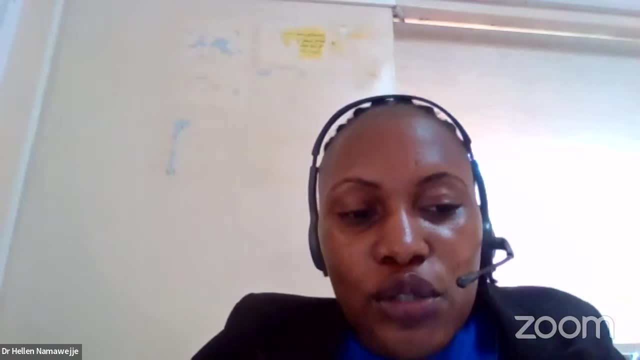 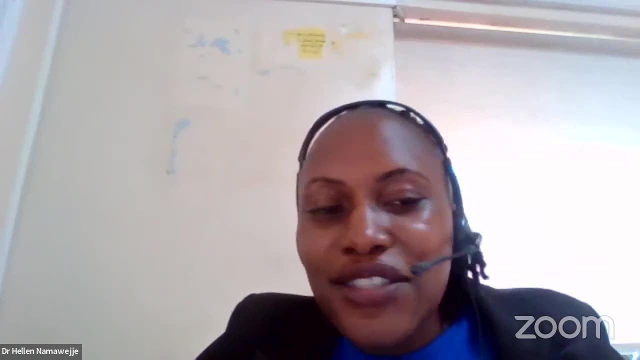 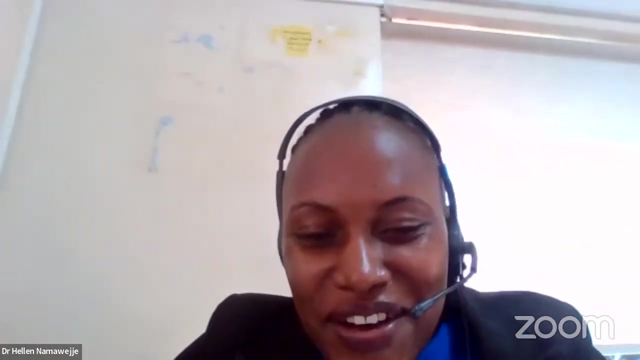 please post it in the Q&A, then you'll be able to get a response immediately. Somebody is saying no and yes, so you will answer. So I don't know what that means. You're saying no and yes. I'm wondering how to judge that. 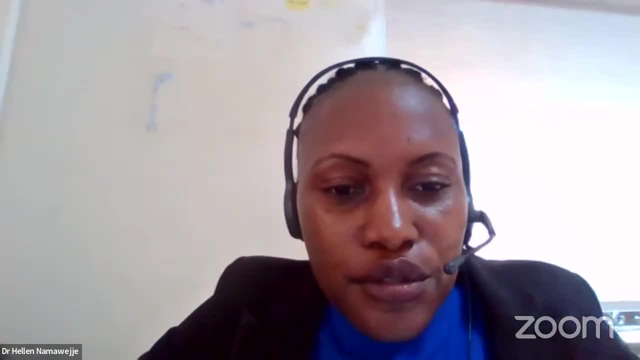 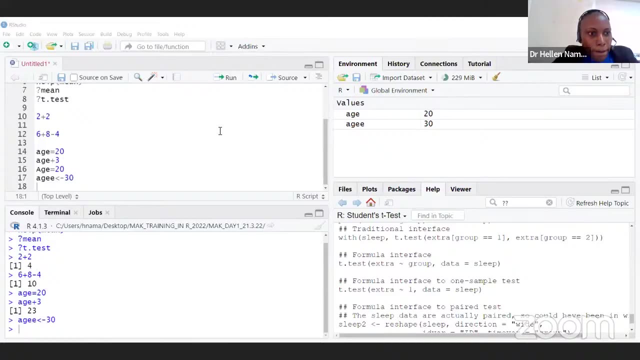 OK, now I'm going to share my hours to you. Please open your scripts, is what we are going. We are now going to start. I sent an hour script which I labelled salary, which I said Salary. OK, now what we are going to do, we've 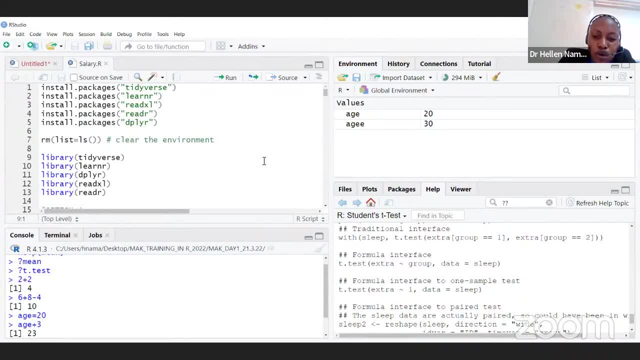 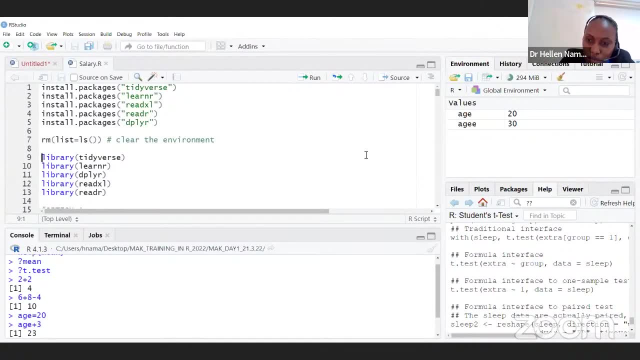 seen the data set that we want to import. All you need to know where is your data set on your computer. Have you put it on the desktop? Have you put it in your my documents, Because it is important? You need to direct our that the data I want to analyse. 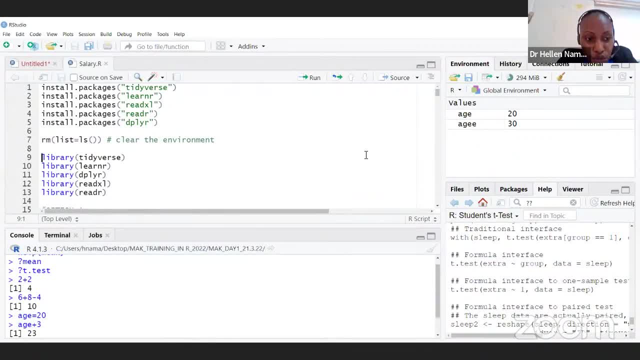 It is saved in a certain folder, So that is also very important. Remember what I mentioned earlier, that, as we are going to start that importation OK, whereby I R is referring to as a data frame, but it's a data set in our usual language. 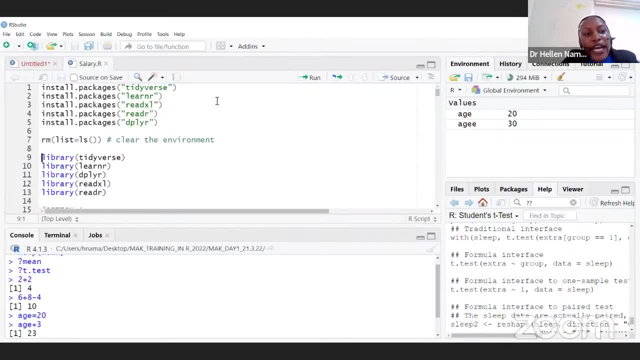 OK, we need to install certain packages. How did I get this script? Remember how I opened this one that I've been using. If you want to save it, all you need to do is to come and click save. The moment you click save. 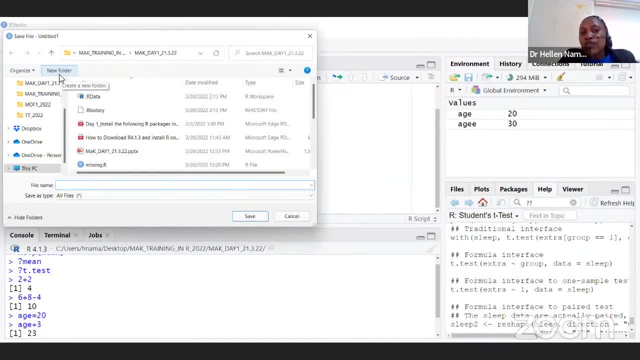 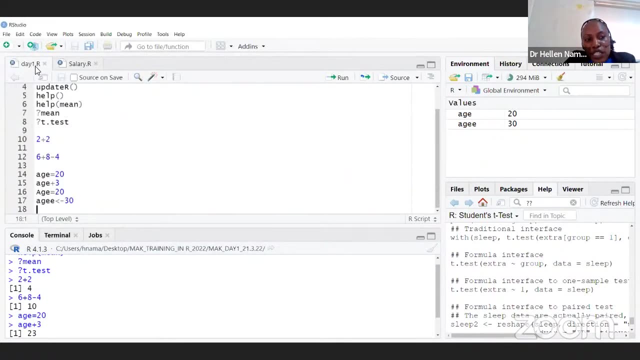 you automatically are, will you have to direct where to sell your work? OK, maybe you can type in your name. I can put, Maybe I can take the one that that is my day one. If you click save, that's why you're coming up with this particular extension. 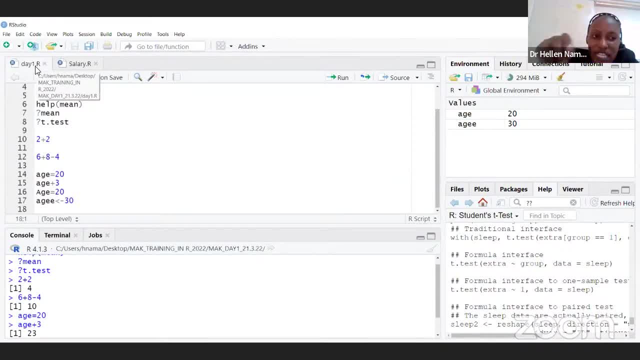 The one dot R, So all the files that you see that has got an extension of R. what should come at the back of your mind? that those are R script and you can run them using R and R studio. OK, so now in the salary script that I sent, how do we get a new script? 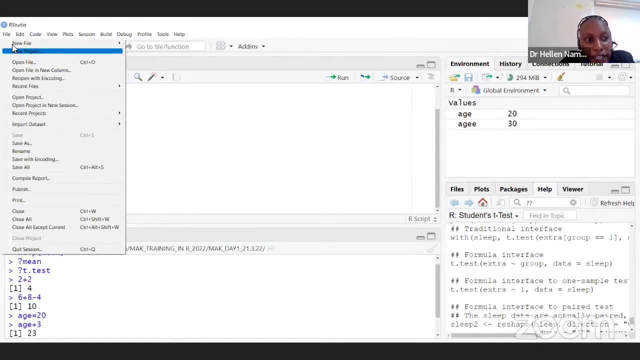 All you need to do. You can either click file- new file- and then you go and click our script. If you don't want to do that, you can just come and click here The moment you click this, if you think we have put the hand. 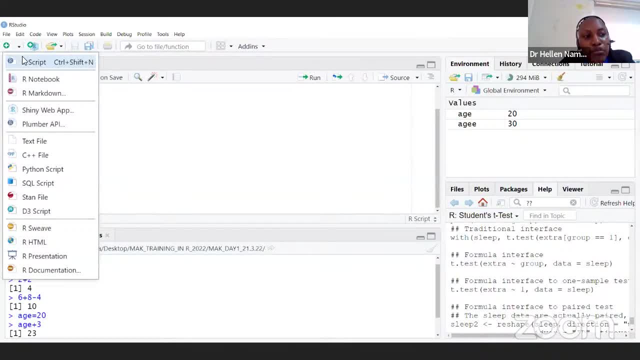 if you, if you click on it, it will automatically bring a drop down and it will ask you: do you want an R script? Then the moment you click on it, automatically you're going to get an empty one. That's why, when you're seeing on my, when you're seeing 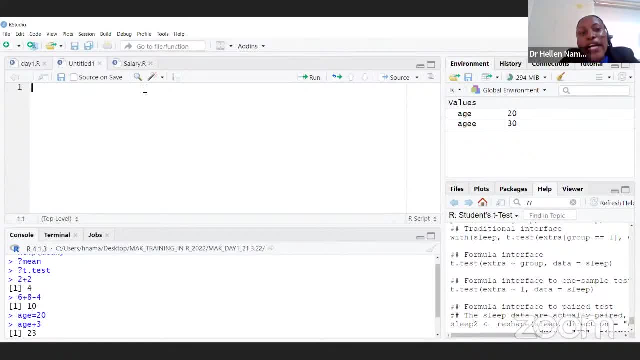 the script here. I've got different windows opening so I can have multiple windows that are being open where I can work from. So I was just showing you how did I get the salary R script. It was in the. I got in a new script. 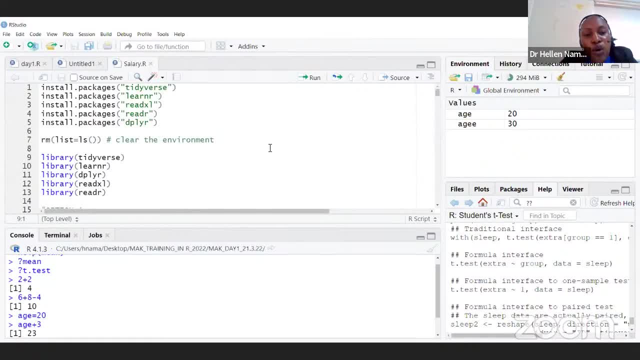 Then I saved it R script like how I've showed you. So go to your computers in the folder that you pick from the Google Drive on your computer. We are going to to see how do we import the work salaries Data set saved in different ways. 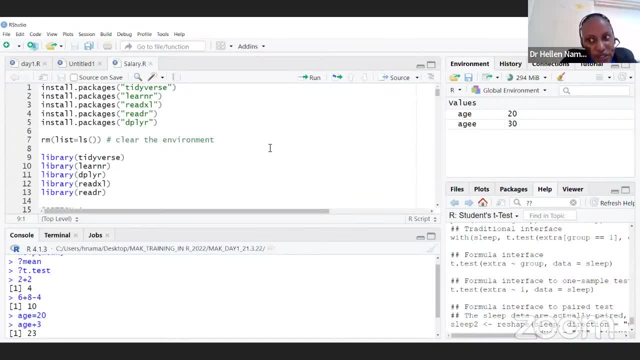 But before we do that, we need to install certain packages that are really very important. If they are not installed in case, after installing them, step number two, we need to load them. I'm using the same script that I sent you, But remember we are having different computers. 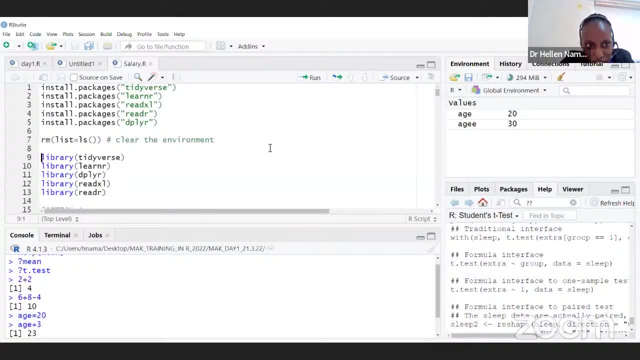 I've talked about the installed packages command- what you need. I talked about some of the common packages that you will always need in every analysis, for example, in case you're going to import data and do data manipulation, like for the case of a tidy bus. 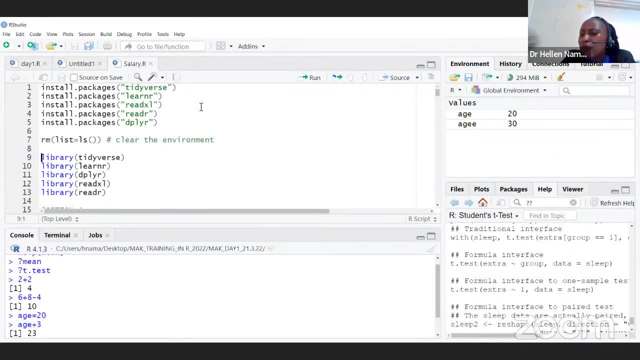 It supports in data manipulation, because you're going to do manipulation and you'll always need it. Then the read XL. That is a packing that's supporting you to read, to import data into R that is saved as XLSX. The read R. it is going to help you to. 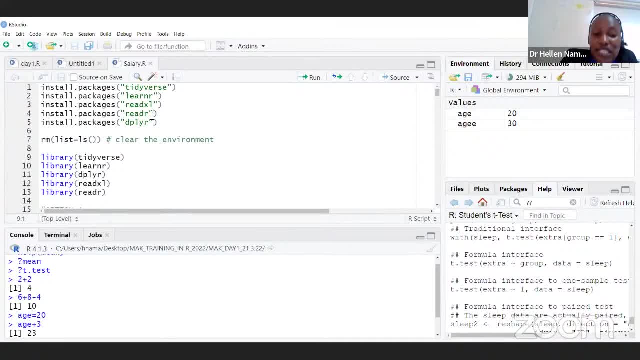 read data: to read data that is saved as CSV. The deployer is also for data manipulation. As we move on, you're going to see that maybe we include other packages like the DigiPlot, which supports in having good data visualization. 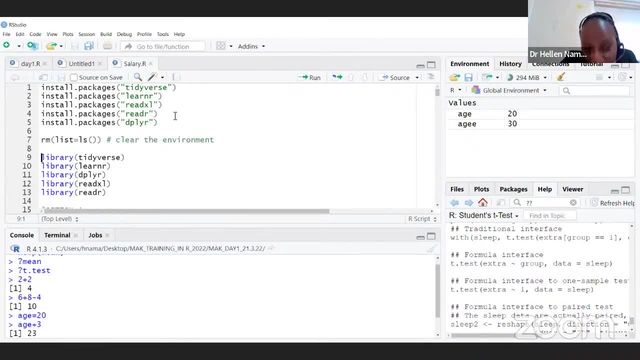 So I'm not going to install these packages again, because I have them on my computer. I've already installed them. However, in your case, if you haven't kindly run line per line, OK, for example, you can come at the end of tidy bus and then run. 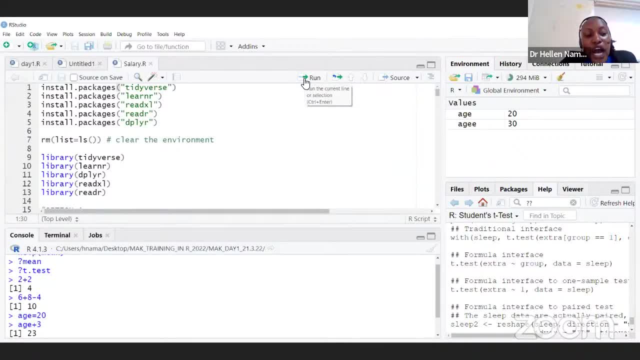 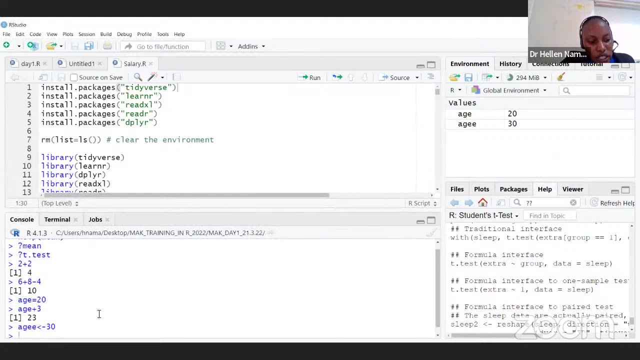 You're going to, all the results will be executed in the R console, Maybe before we move on, in case you're not, in case you want to clear your R console, what you can do so that you're able to work very well with a clear one. 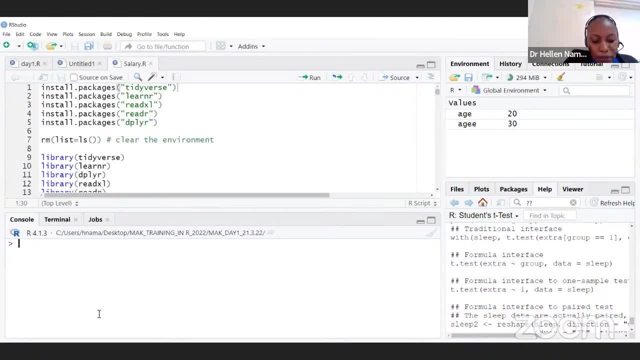 you just need to type control L. the moment you type control plus L, The console will clear and become very clean. And when you look at my environment, it has got values that it is 20,, then it is 30. If you want to clear, 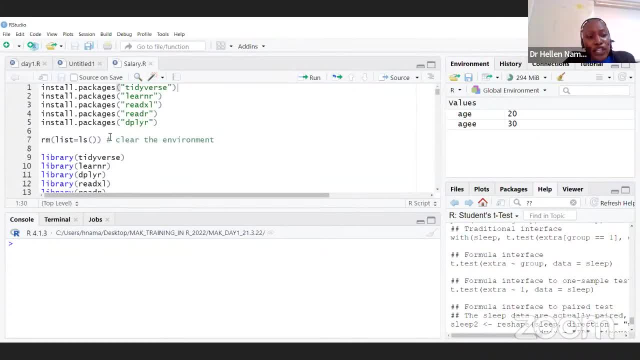 if you want to come up with a clean environment, we're going to use the command RM in bracket list, which is equal to LS. then this RM means remove. then inside RM we are putting a list. The list implies that whatever variables 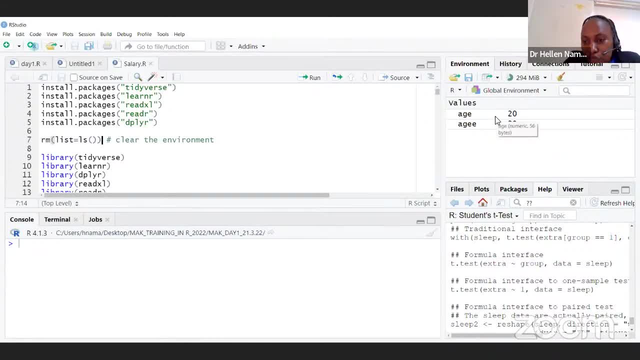 or values that are being stored in the environment. all of them remove, delete them and let it be empty. So, in case I run this particular line and I look in my environment, it is going to show me that there is nothing stored or there's nothing that has been stored in the memory. 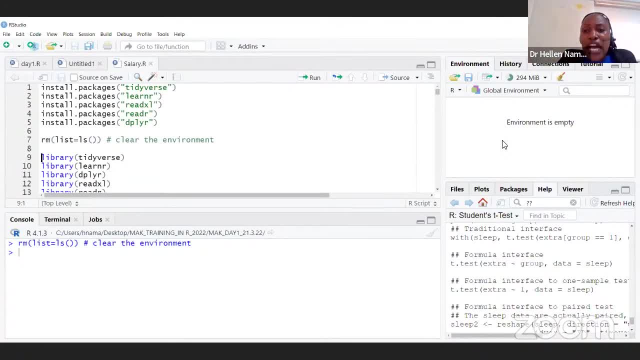 Sometimes you could be working on many or many projects and you want to see what exactly is happening, but when your environment is tied up with a lot of things, you can clear them up and then start working a fresh set that you're able to see the connection of your environment. 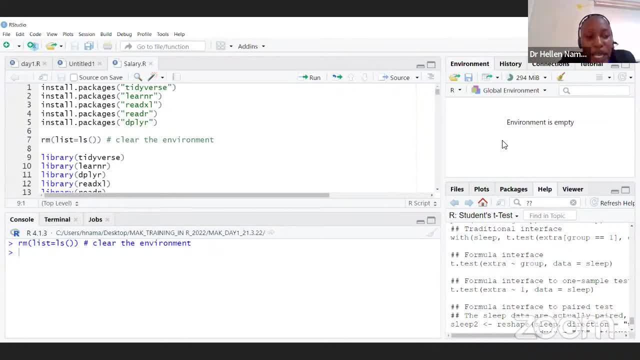 and the analysis that you want to do Now, the moment you install your packages. after installation, you have to run these packages. OK, for example, I use the library command- I can, I can at the end and then I run that line. please, if you've opened this particular script. 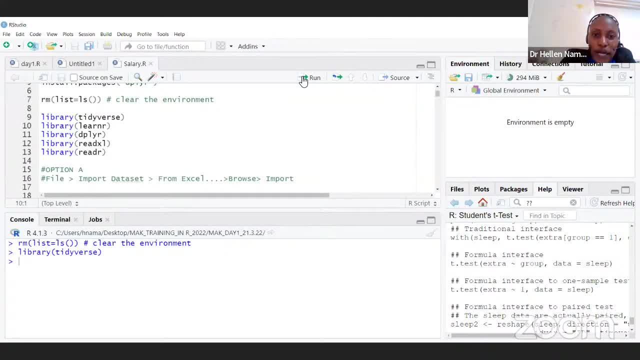 Let's Do it together. as I work out here, Also work at your end. OK, I'm going to run the next line: library Learner. are I learn the library, the player, then the read Excel each each time you run a line. 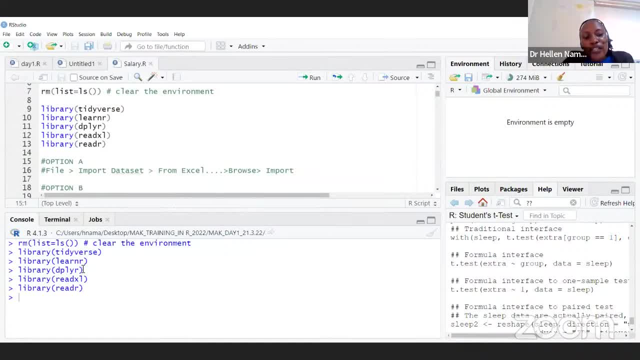 it goes on the next step and everything. I'm seeing it in the watch, in the console. Sometimes you might say like no, I don't want to run line by line. All you need to do is just highlight all your libraries that you want to use and click run. 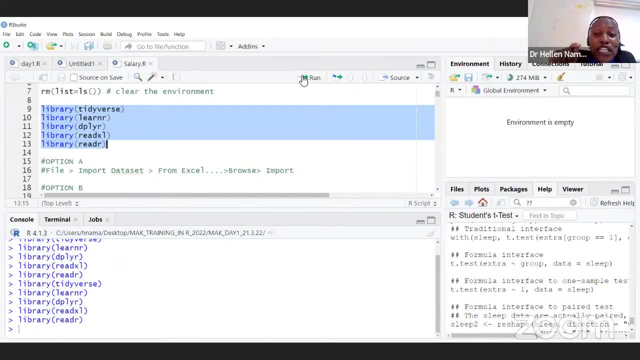 If you check them in the console in case they are successfully installed, you will. you will see only the blues in the R console. If they are not successfully installed, you're going to get errors. They will. you'll have errors in the R. 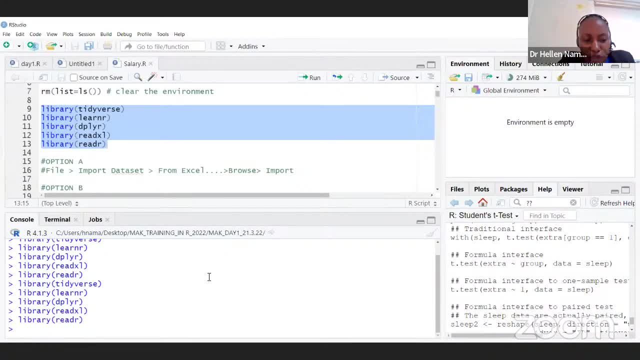 console complaining about something that you need to rectify before you move on. So let me ask in the chat: have you been able to load your libraries? Let's first follow, OK. OK, Yes, Boris, yes, we please. OK, that could be still installing. 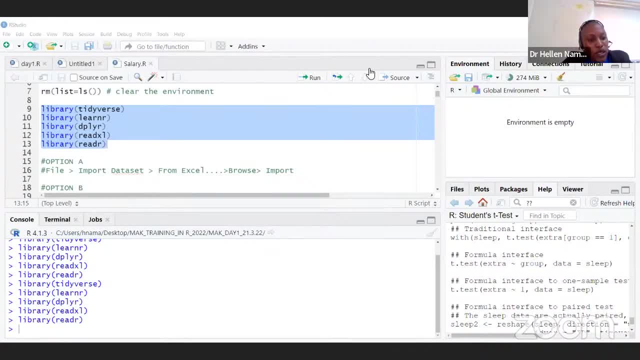 Let's first install And Still installing, not quite OK. George is asking: how do we load them? We use the library command. All right, Someone is asking for lunch, isn't it? Let's use the R script that I sent. 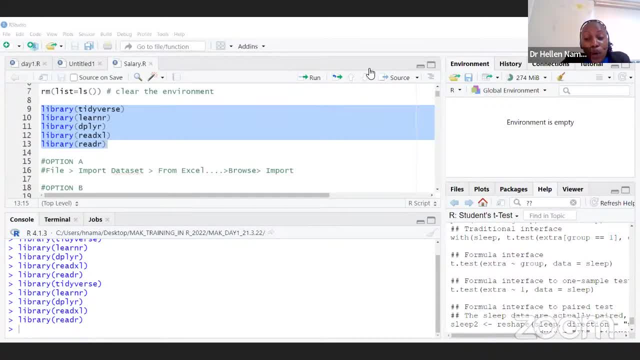 Remember one of the advantages of using R: the codes can be reproduced. So the point is understanding how to use these R codes such that after here you are able to apply them on your own data set. So Prisca is saying installing R packages is in progress. 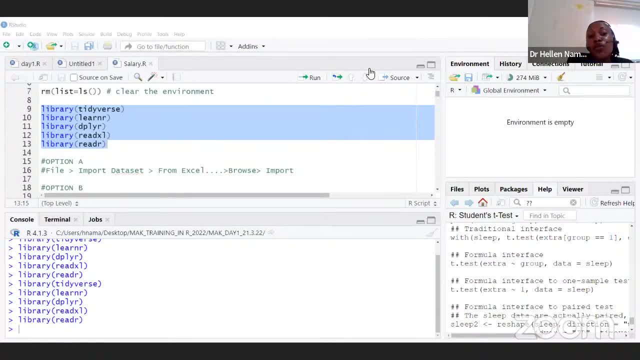 In case you had these packages before, all you need to do is to load them. If you're still installing, let me give you two minutes as you install. If you're having an error, post the error in the Q&A site that you are helped. 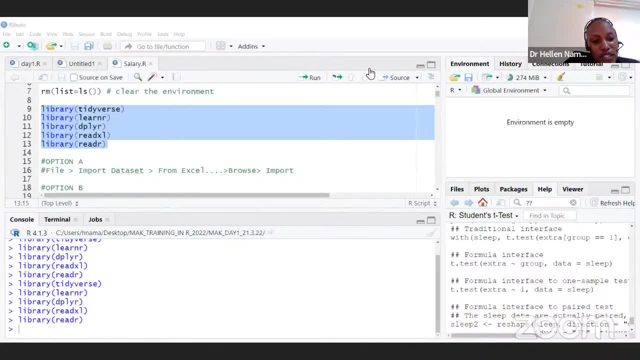 Can we save directly on CSV in R studio? OK, we're going to see. Remember, with the CSV it's an extension. It's how you saved your Excel sheet Right? So we are going to see And remember, we've put a package read R, read R is the one that is going. 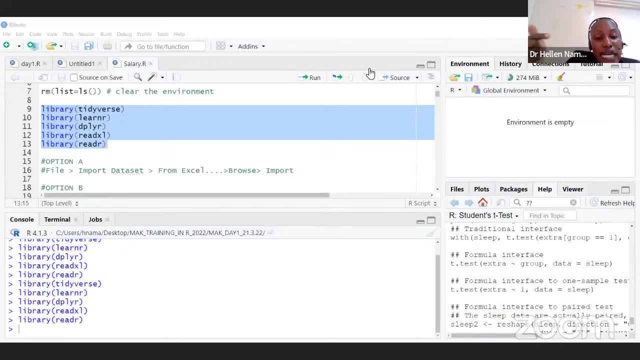 to support us to import the data set saved as CSV. OK, loaded successfully. Mohamed, you're putting that. there is an error. Just check how you've written, dplyr. You've put space. There is no space. That's why it is giving you an error. 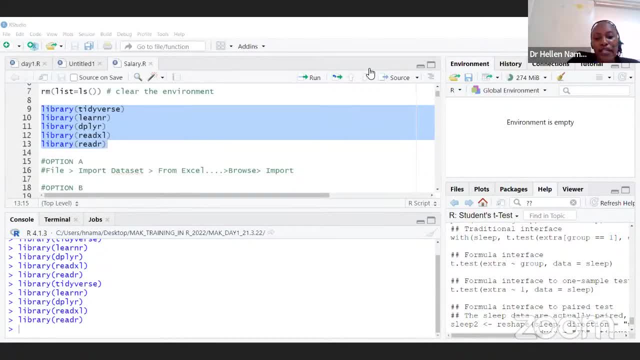 It is dplyr. Don't put in brackets, Don't put space. That's why it is giving you an error. What do you suggest? We give a break? Well, We give a break. OK, as we are. as we are, we are trying to install. 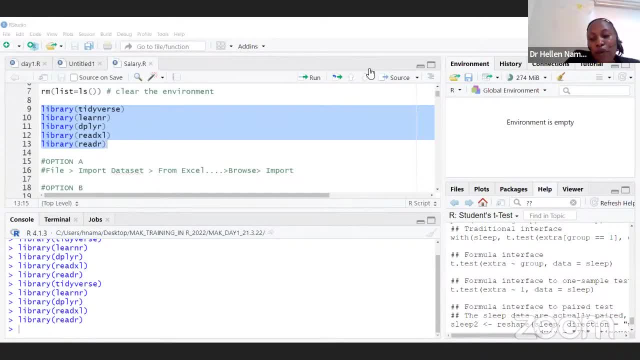 in our packages what we are going to do. we are going to take a break of 10 minutes. I know people are saying that a lot of comments are coming in a break, a break. So we're going to take a break of 10 minutes. 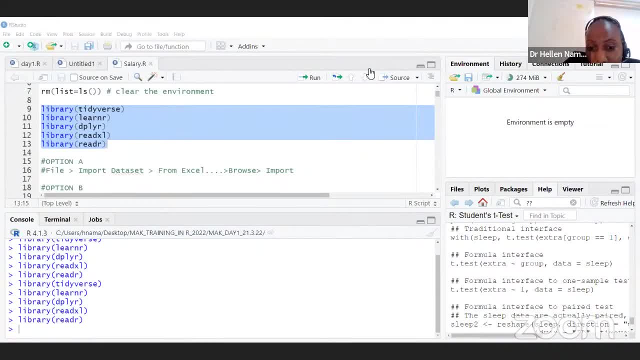 So those of you who are still installing and loading, use that 10 minutes. After the 10 minutes we are good to go. OK, install and then load using the library command. OK, So we are starting at a quarter to one. 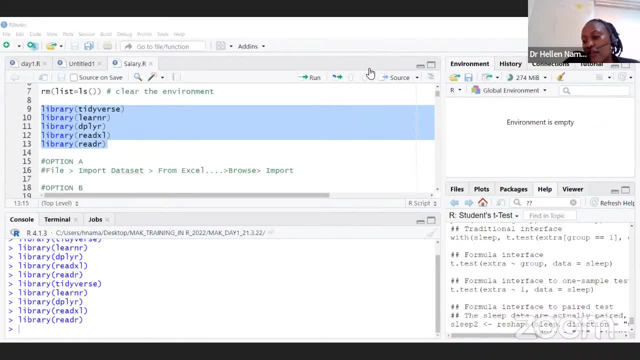 That is you're going in time. It's 12, what? OK, so at 1245.. So at 1245, we are going to resume. Yes, we are going to resume at 1245. and then now we continue. 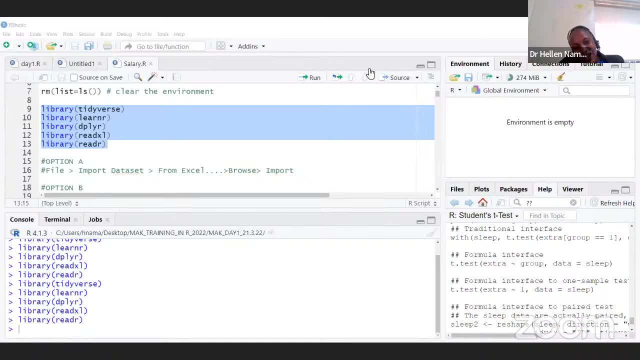 We need lunch time. Yes, Remember, we are stopping at two, So we are only going to give a short break. Some are saying that no need to break. OK, let's just take a break of 10 minutes as people are installing and loading libraries. 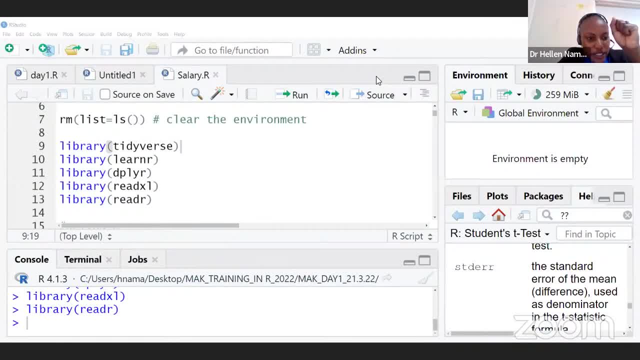 and let me hope you enjoyed the short break. we are also downloading packages. please show the command below. okay, let me just echo out some questions that i saw in the q and a. okay, okay, okay, fine, um, yes, somebody was mentioning that i was downloading and then got some reds and 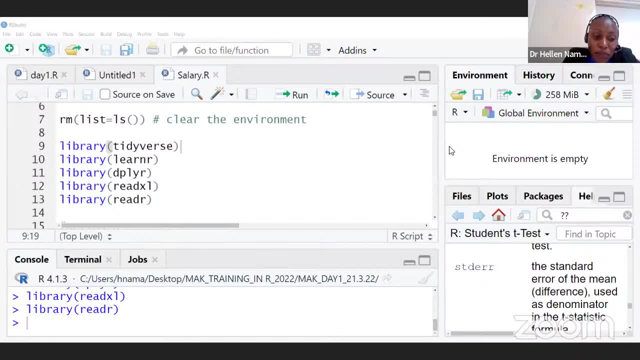 so on. so when you're downloading the different packages automatically you'll see the reds coming in. our is trying to to get to get to install for you the package from the r crane, where the packages are onto your computer. so the moment it successfully does so it will tell you download successful. so when you see the reds you 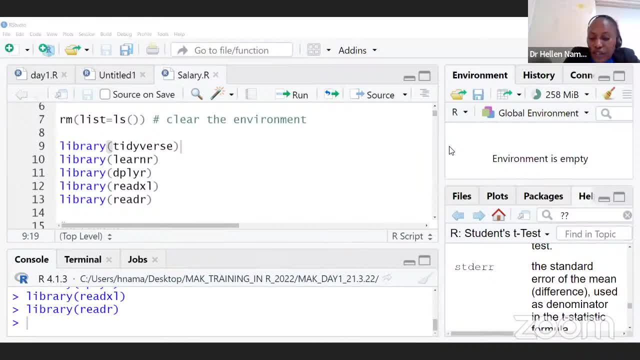 shouldn't worry, wait until, uh, the, the, the, the, the. it shows you a stop or you see a prompt that it has been successfully downloaded for you. so the reds are coming in and i'm going to show you that you're fully downloaded. and then one was asking if library is a package. library is not a package. 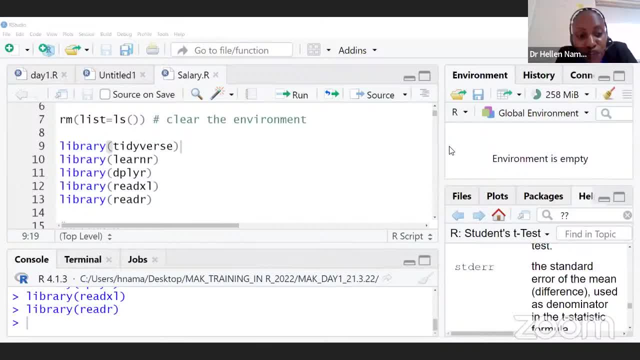 it's a command, it's the one that support us to load the different packages that we have installed. and then, uh, i would also like to encourage you, remember we say that they said that r is an open software and a lot of amendments or adjustment or updating skip going on every now and then. 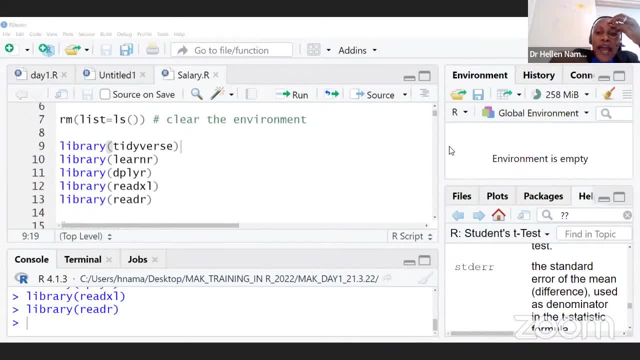 before a newer version is released, like why there is always that particular update, that there are certain there are some issues that they want to make the program better and better. so the problems that you are encountering, some other people have encountered them before. i would also encourage you: in case you get an error, just copy it and paste it in mr google and you'll be surprised. 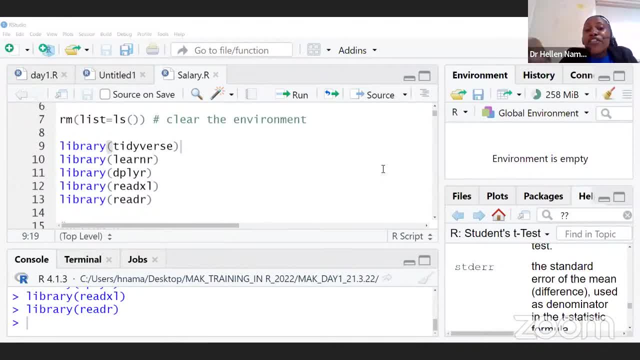 to see like millions of people have encountered that problem and they have put a solution so as they give you a new version of the program. you will be surprised to see like millions of people have encountered that problem and they have put a solution. so as they give you the various solutions. 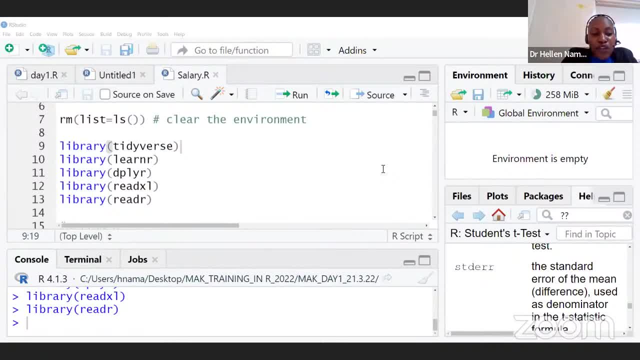 you can get one that applies your scenario and see that you solve that problem and continue. so at this particular point, i believe we are done with loading, with installing and uh, and loading our packages, so can we move on to import? do we have to download them? no, no, no, no, somebody's. 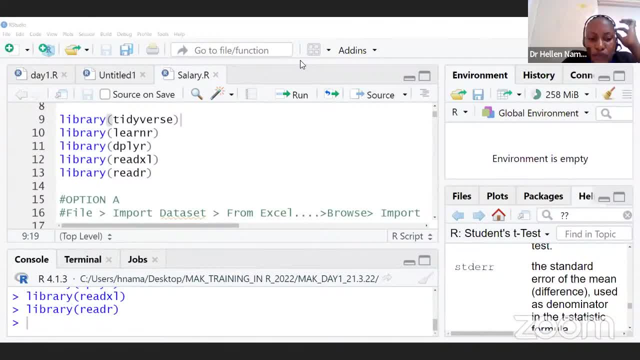 asking that we have to download them every time or they are stored forever. you don't. you download once after downloading. all you need to do is download the package and then you can see that. download the package, and then you can see that Could that be imported? and then you can just: 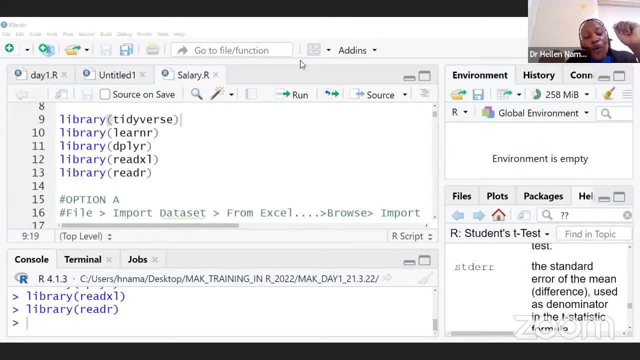 drive theай on here. so that's what we have about the executable or whatever is going on. and if you need to do is to load them each time you open you our your R studio, what you do is don't in case they are, they are installed. all you need to do is just call the library command when, whenever you're, 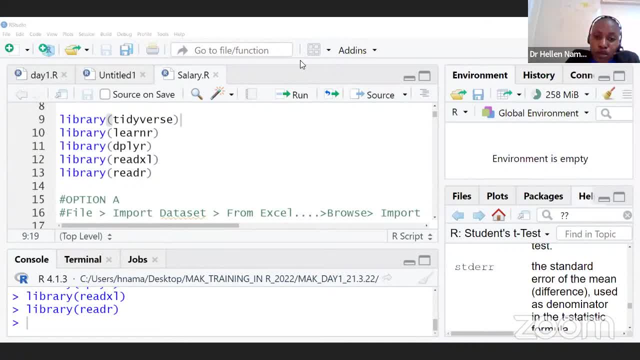 calling the library command you're. you're just alerting R that, uh, it's what you're going to use- your library. only that now on my computer i have a data set. sorry, i've got a folder where i saved my work- salariescsv. okay, so now i want to import it from there. 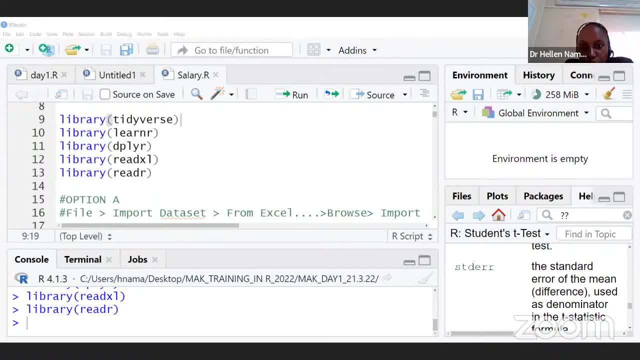 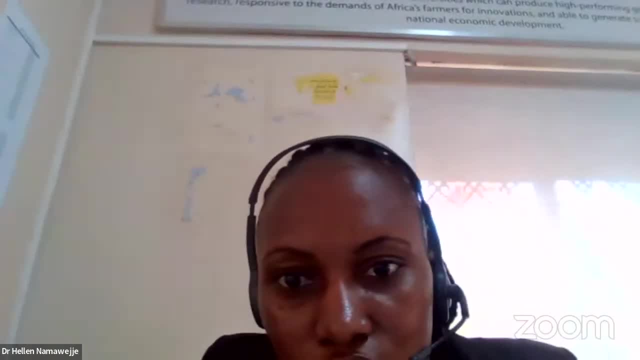 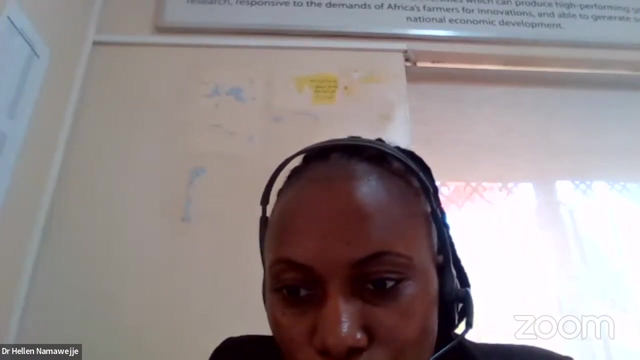 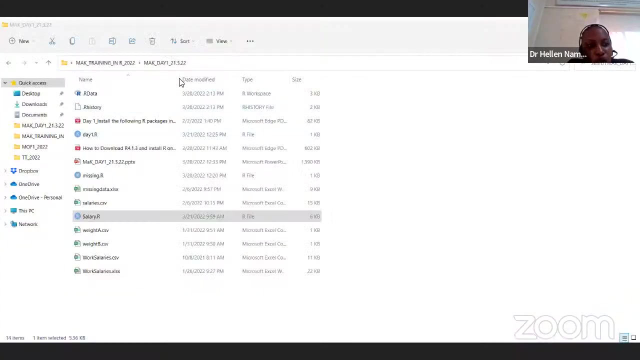 okay, for example, let me first stop sharing this and- and i share it with you- um, i want to show a folder. well, let me share this. on my desktop, i have a folder which i named mark day one and i put today's date, and it's within this folder. 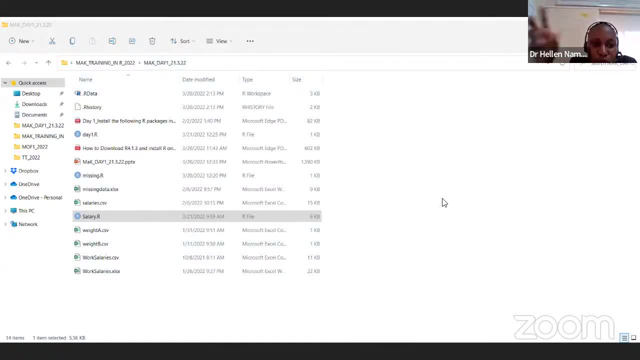 that has got all the material that i'm using in this particular training. now this, this folder, is saved on my desktop. what i want to do within this particular folder- again, if you're seeing my screen very well, there are different data sets that i'm going to use. i've got work salariescsv. i've got. 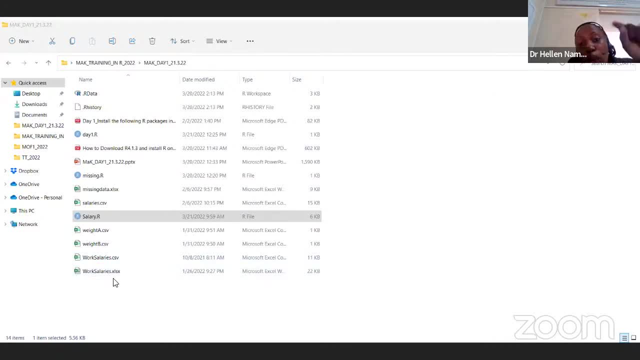 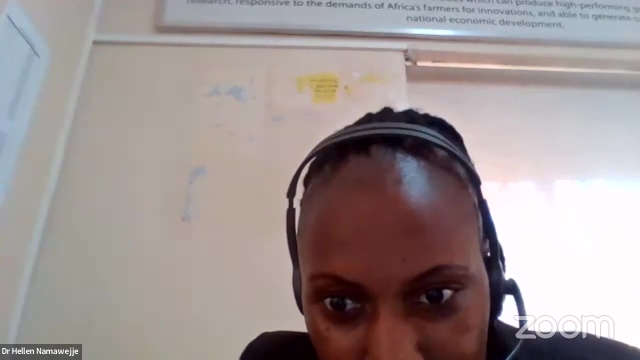 work salariesxlsx, which folder we uploaded in the google drive. so i'm going to tell r i navigate on computer and i tell it go into the mac, the one folder, and pick for me the work salaries data set. okay, now i'm going to close this and then i open my r again. 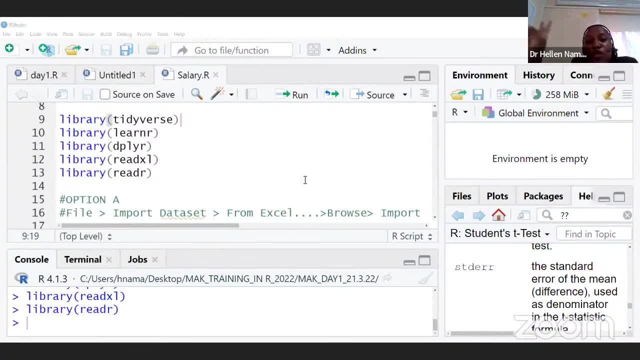 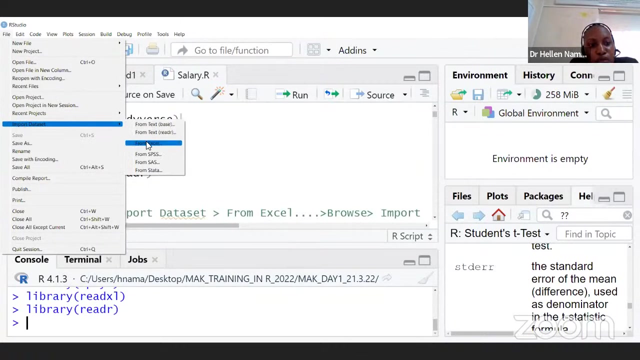 okay. so now, after loading, we are going to look at two options. let's first load our data set that is saved, as i, that has an extension of xlsx. what are we going to do? that is option number one. you go to file, move down import data. then when you move, you move to from excel the moment you come here. 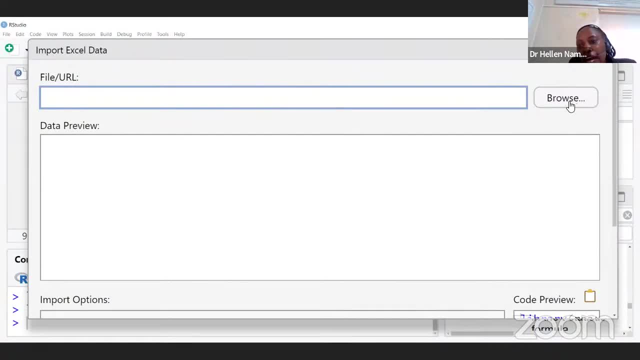 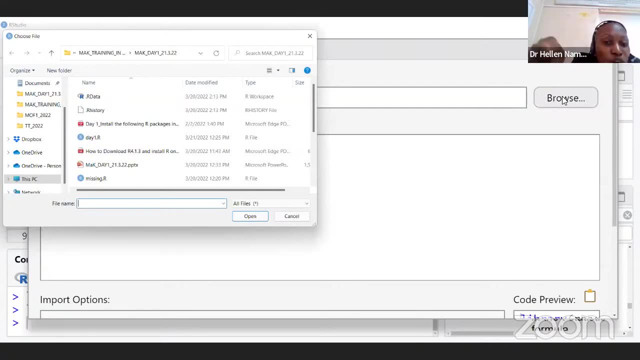 the moment you get this particular window, you move here and and check browse. okay, the moment you click browse it, you have to navigate until when you get where your data set is. and now it is telling: i. i move to the, to the mac training material, but it is within the mac. 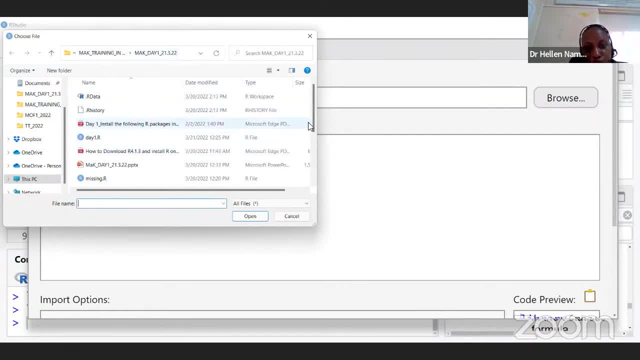 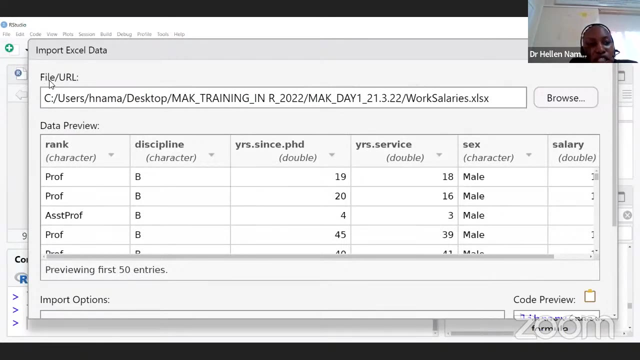 train the mac day. one folder and inside this folder i move and i and i click on the work salaries dot xlsx. the moment i click on it it appears the path appears on. if you look here, it is file slash url. it gives me the path on my computer. that how do i access? 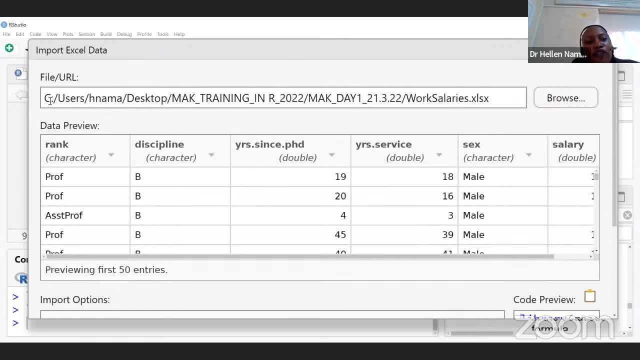 the salaries that i said. it is telling you that from my computer. go to users, go to h. now then the desktop. there is a certain folder mark training, then mark day one, and inside that folder there is a work salaries dot xlsx. that is the data set. all right, it is interesting that it also gives you a view of how your data set looks. 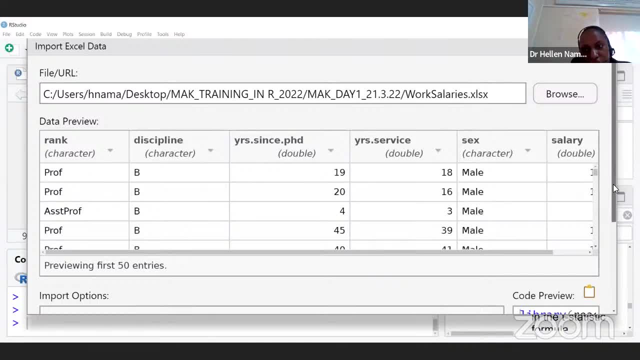 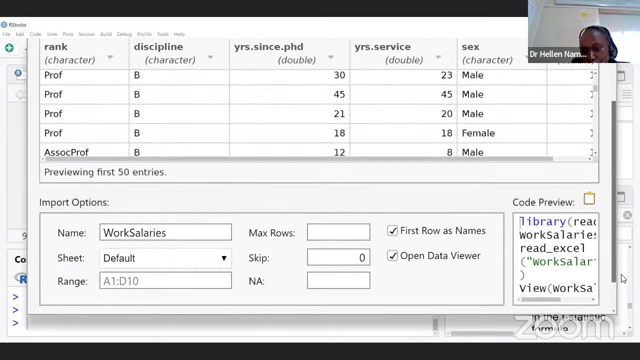 like okay, and after that we are seeing that it shows you the rank variable display near since phd, years of service sets and then salary. okay, so when you scroll down you'll be able to see your data set, but as you move down below you are able to see the code view how your your work set. 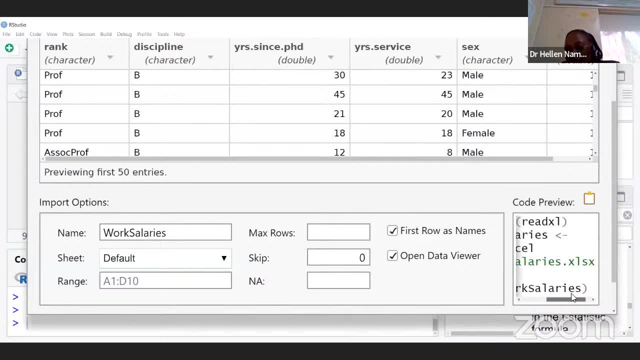 how what code was used. it will tell you that uh, it is work salaries. then it used the read underscore excel command, but if you look at it on top, it used the library read xl. that is the relevancy of uh installing our packages, and then it will. the view command: it is the one that it is. 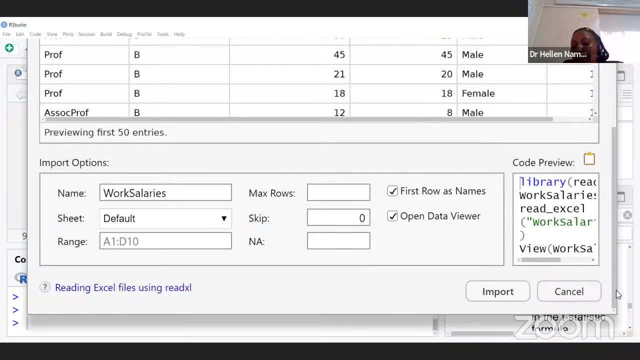 able to show you how your data looks like. so when you move down, you can see the commander that tells you the data set. so when you move down, you can see the commander that tells you the data set, its name, the web page: click on the word import. 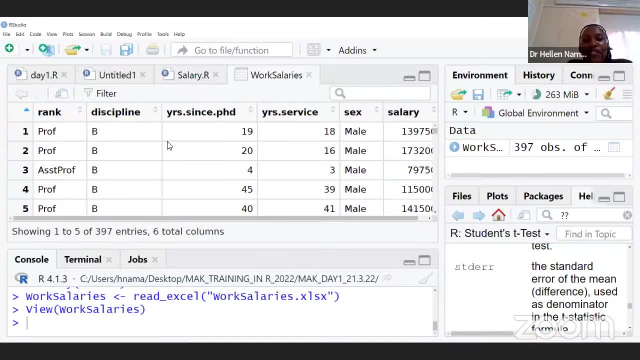 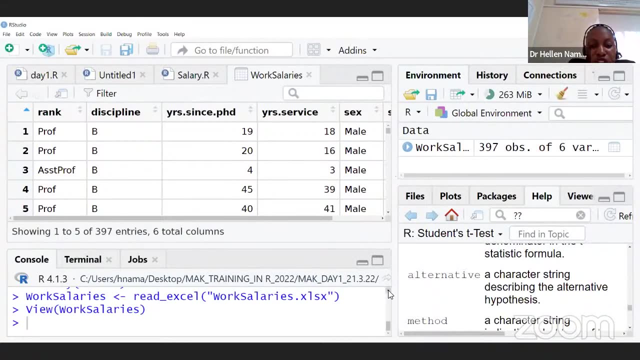 If you click on import, what happens is that you are able now to see your data being imported into R. Okay, I zoomed out. That's why you're seeing my words to be very big. When you move in the R console, it is giving you what it has done. 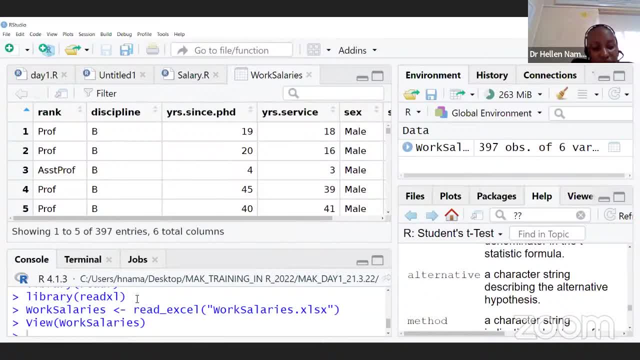 It is telling you it will use the library read XL. It imported work salariesxls using the read underscore XL command And it named the data set: work salaries. If you remember, I talked about the assignment, the. how do you assign variables? 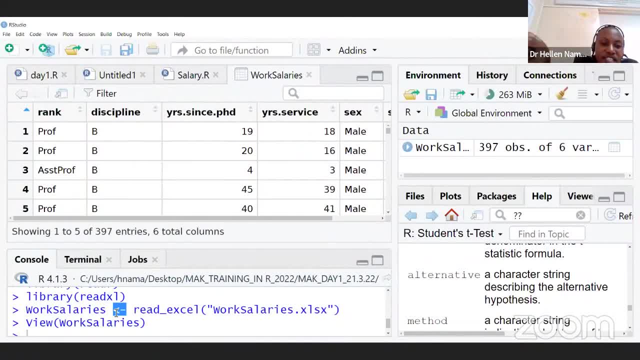 So automatically, R uses the name you saved your data set as it is the same name that it uses also in R. Okay, You called it work salaries, So it is also picking the same name: work salaries less dash. That is an assignment using the read underscore XL command. 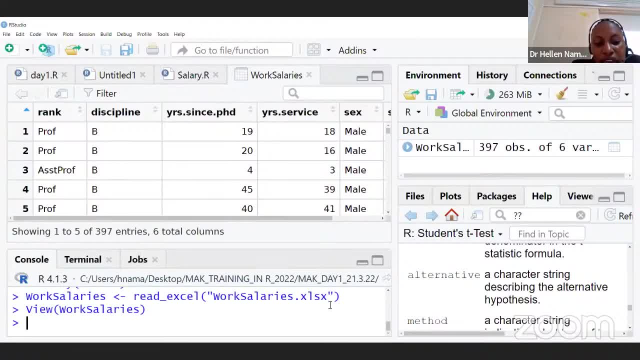 And it is bringing you the work salariesxlx data set. Then the view command. it is what is showing you here: View, seeing how your data looks like in R. If you want to see if data has been successfully imported into R, come and check in your environment. 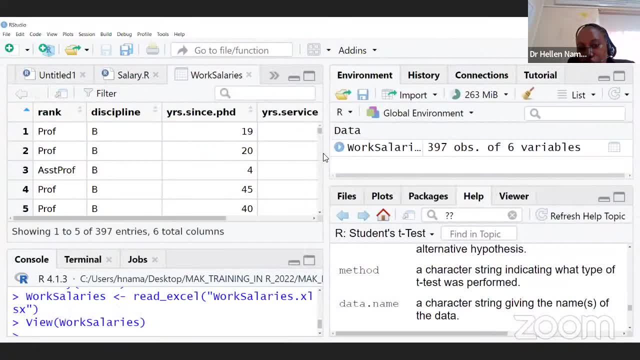 It is now showing you that, within this particular environment, you're having work salaries. It is showing you've got 397 observation of six variables. So these are the number of observation you're having And then, within this data set, you're having six variables. 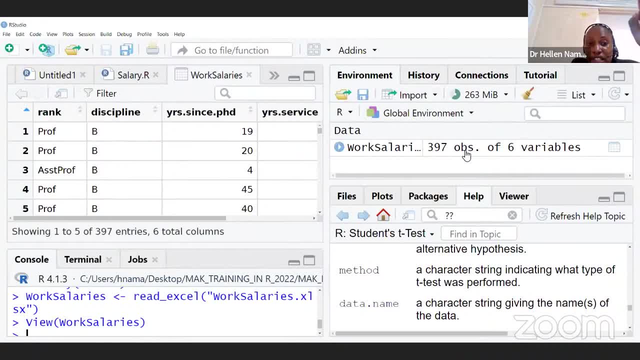 Sometimes the environment is important to enable you to cross check and see: has have I really imported the right data set When you move. at the end, where I'm putting the hand here, there is also an Excel icon which you can also click on and view your data set. 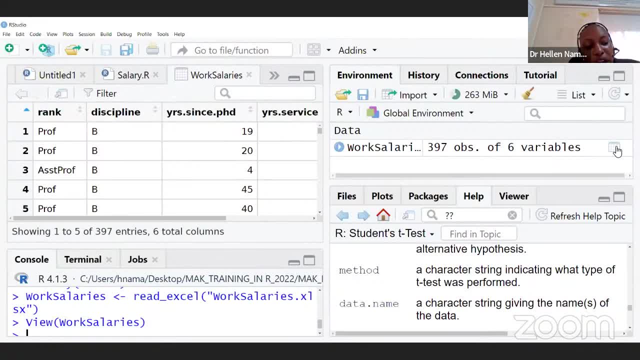 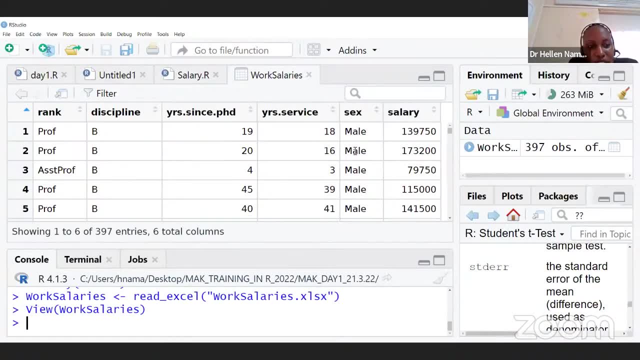 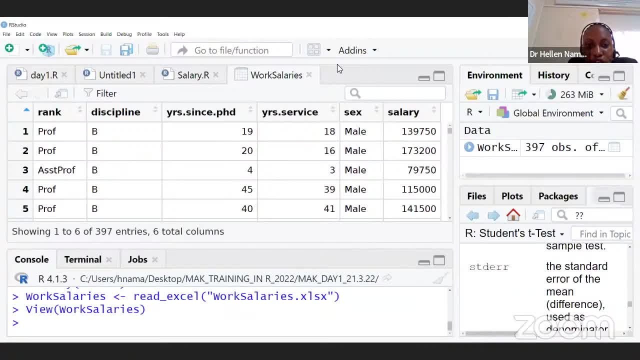 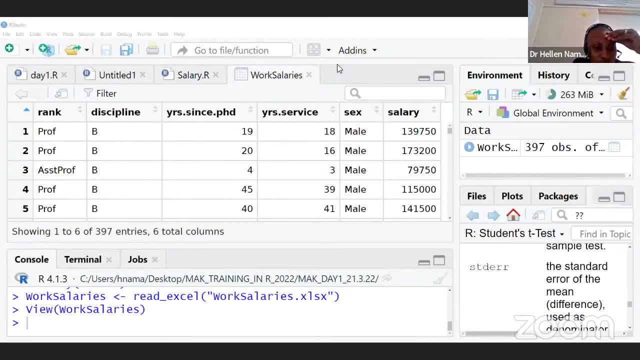 Please recap The umber: Yes, Imported, This is imported. Imported- Great. I'm seeing a big number successfully imported. so somebody's saying that I've got two work salaries. remember we distinguished between the two. no work salaries was only served with a CSV extension. 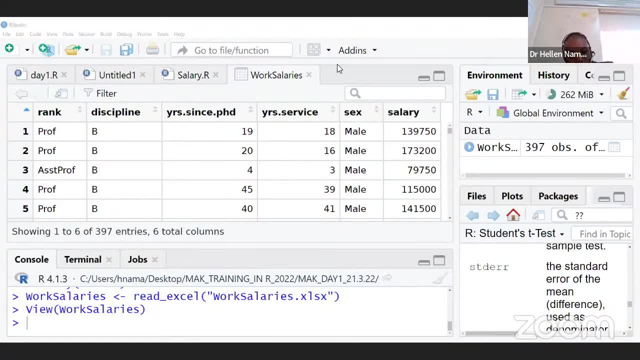 please check in that folder. you've got two types. we are now dealing with work salaries. that is served as xlsx. we are not dealing with the work salaries served with the extension of CSV. please listen as I speak. stop posting comments. listen as to what I'm telling you and you do it right. 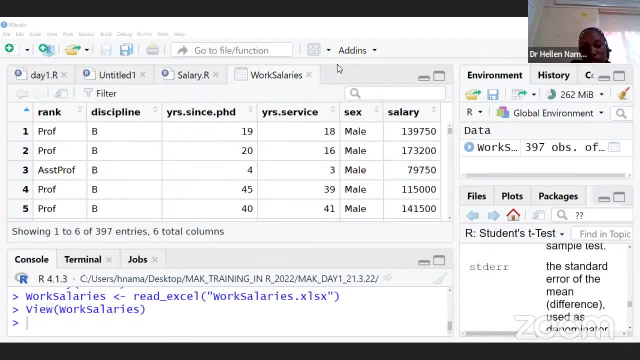 all right, okay, what is the use of your salaries? the view command you can use if you want to follow what I'm saying. so, if you want to follow what I'm saying, It helps you to see how your data set look like So that you're able to compare it. 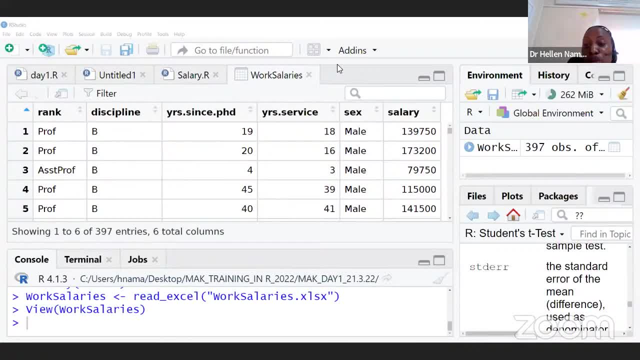 with the original data set in Excel. Does it really look at the same with what you've imported into R? In case they are different, then there is a problem. Immediately, you can be able to adjust that problem The way you hear the word view. 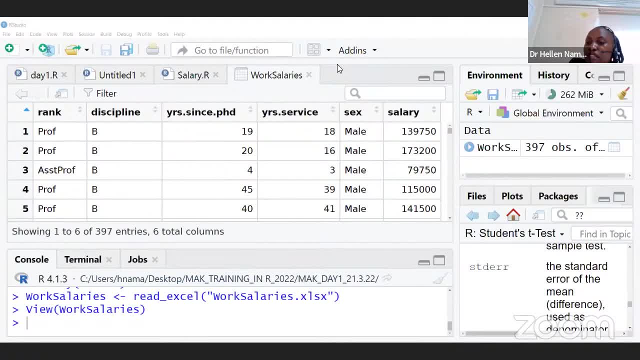 it is like seeing whether your data, set the way it appears in the Excel, is the same way it looks like in R. Okay, yes, done, Okay, Samuel, we are getting there. Okay, so can I continue All right now looking at that. 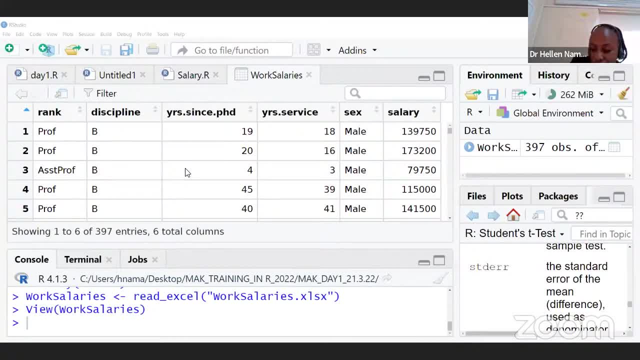 I'm glad that a big percentage has been able to import our data set, the work salaries data set. that has an extension of XLSS. It's quite interesting When you look in your R console. all the commands have been given to you. 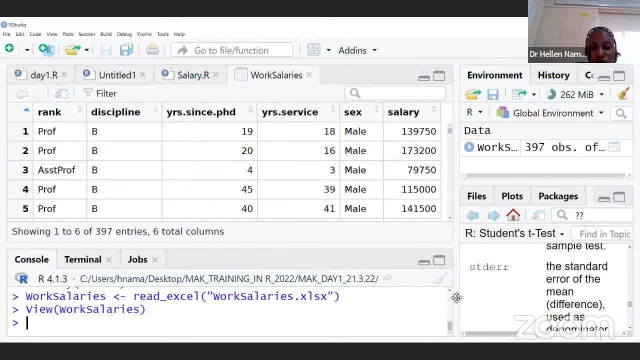 What it has. when you look through your R console, it has told you the library that it used. Then, when you look in this particular line, there's something that I want to talk about. I'll use the read underscore Excel. That is the command we use. 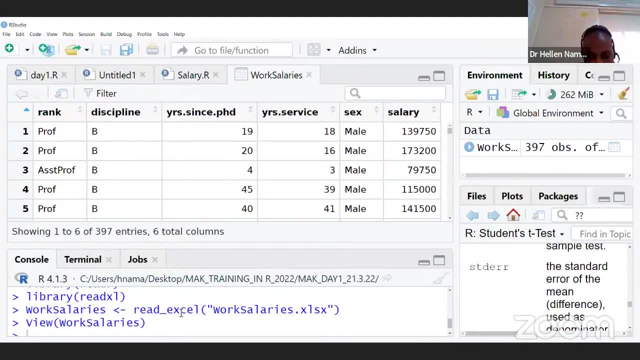 We use it to import data that is saved as XLSX. However, it went ahead to assign the whole of this particular line, the whole of this particular command. It assigned it as work salaries, Work salaries. in this particular case, we can call it the object name. 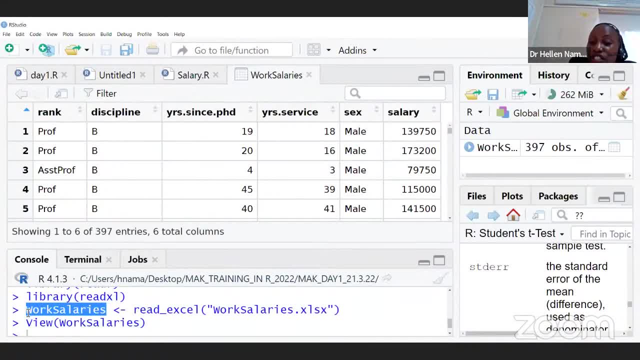 R refers to it as an object. An object name can change depending on what you want to call it, But we're going to see more as we move on, So I'm going to. I'm going to stop here. Now let's look at the other version. 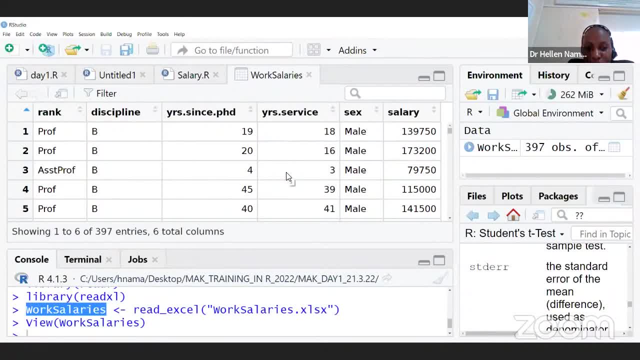 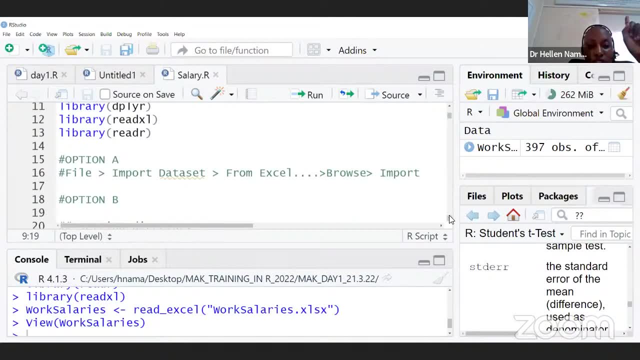 What about, in case you want to import data that is saved as CSV? Okay, I'm going to cross this. I go back to my R script. That was option A. What about option B? Okay, Now, when you go to option B. 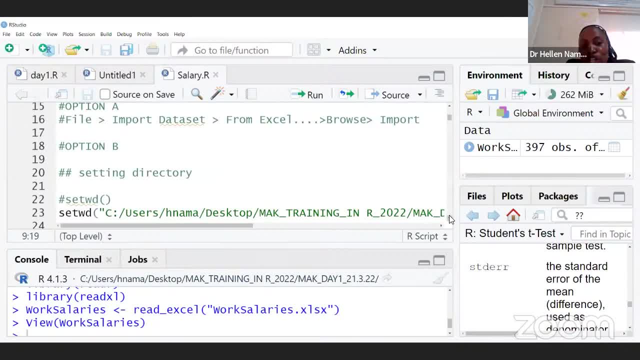 setting the working. We need to set the working directory. You can do it manually, You can do it automatically. Okay, For example now, when we are setting the working directory, because we need now to import the other data set that is saved as CSV to bring it into R. 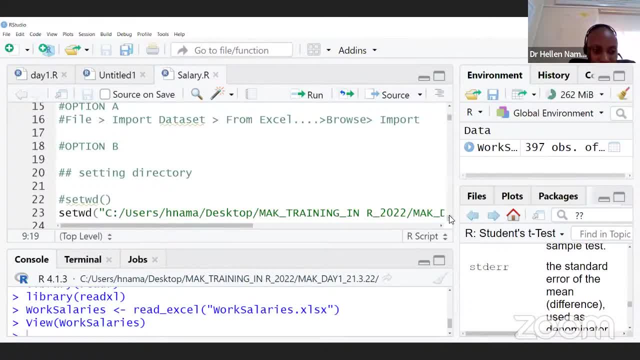 we are going to use the readcsv command. The command we are going to use- if you watch what I'm doing- it is the readcsv command to import the data that is being saved with that particular extension Each time you type something new in your script. 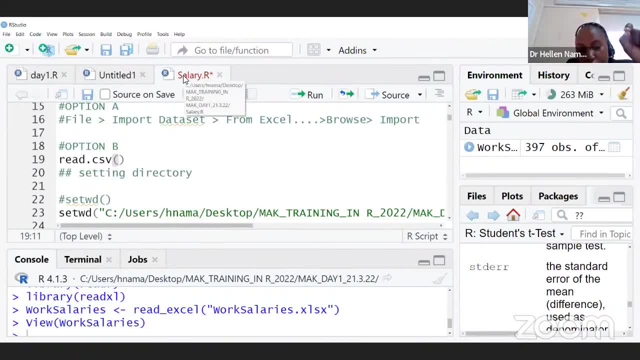 the name that you saved, your data set turns to red. The red implies that there is new information that you've put, that it is not saved. If it is not true, then, for example, when I click save, it will turn black. 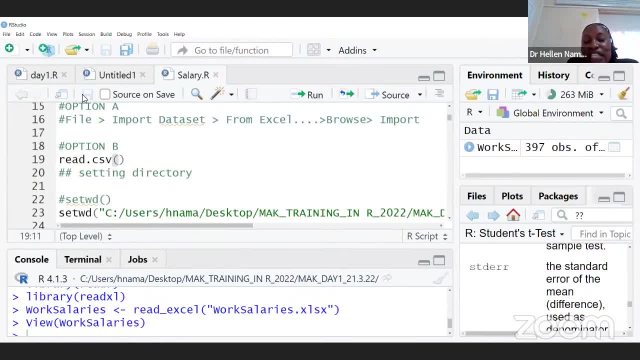 implying that whatever information that is there, it is all saved. In case I type in something new, it will turn red. So as you work, it gives you an echo that you might lose some information. Please do go ahead. and what? 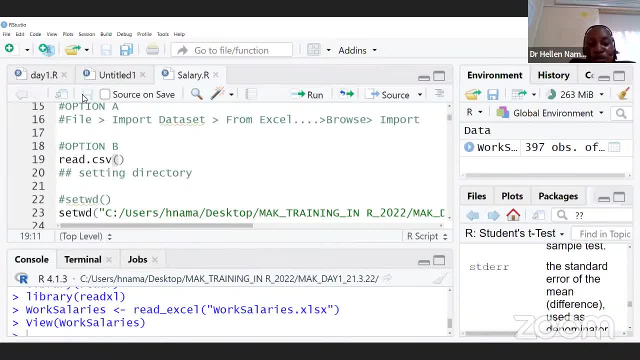 Go ahead and save. I said you can do. You can have your, You can set your working directory manually or you can do it automatically in R. How can we do it automatically in R? Then we'll see the manual bit, What you do. 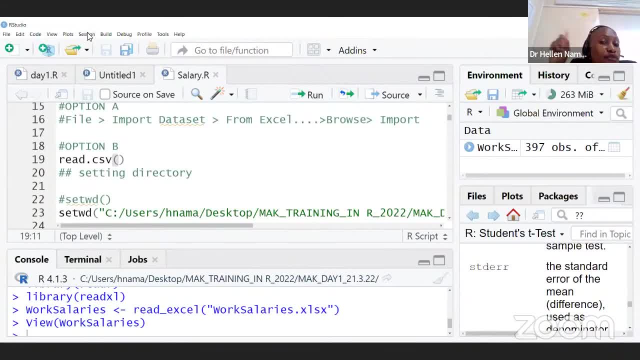 we go to session. Remember it's still the same folder. I go to session. When you click session, move on to set working directory. If you go to set working directory, you move down and choose directory. If you click, choose directory. 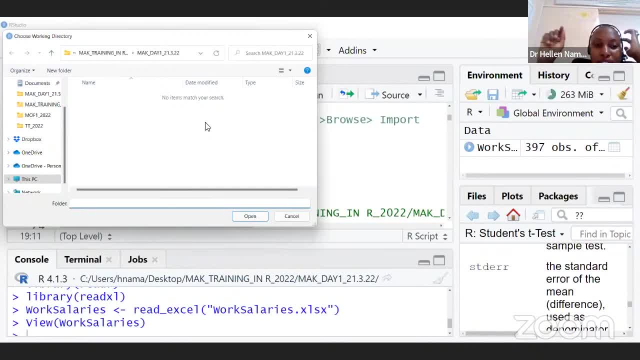 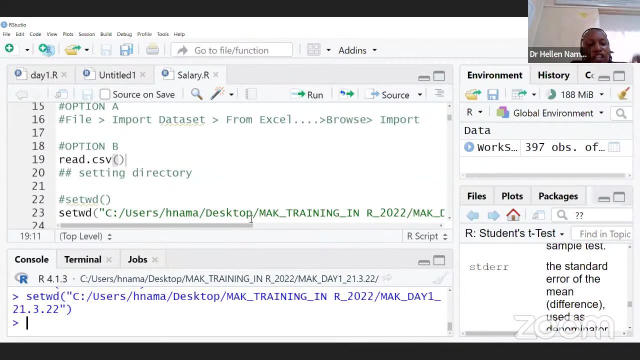 it is taking me to my folder where there is my data set. Okay, And then all you need to do and then you type open. The moment you click open, check in your console. Within your console, it has set for you the working directory automatically. 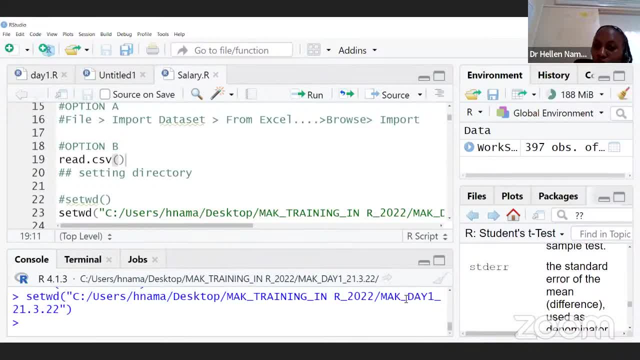 That your folder is being The document that you want to import. it is being stored in the Mac day one plus the date folder, What it does. it shows you all the steps it took to get into where that folder is, The folder that's got the data set. 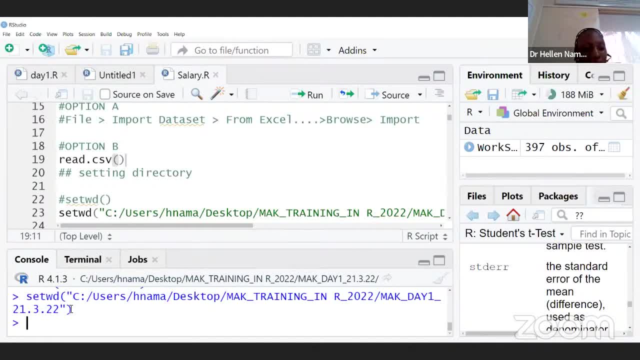 that you want to use. So all you need to do just come in the console and copy this line and then bring it in there because you want to use it. You might need to save it next time. you just run it, You copy it and come and paste it. 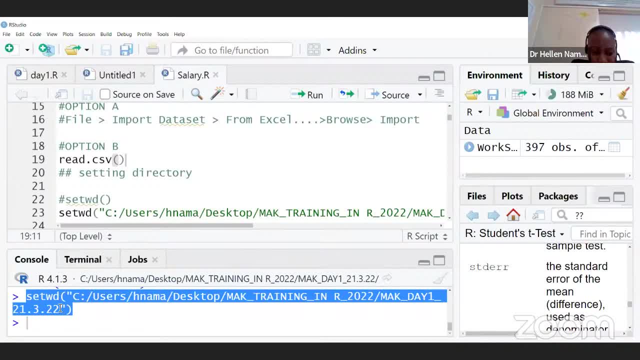 in your R studio, because next time when you come and you just run that line, it will automatically tell you the location. So it is what I did on this line: I set the working directory, then I set everything and I came up with this line. 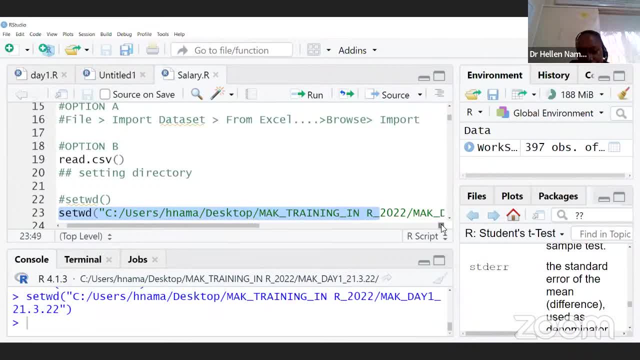 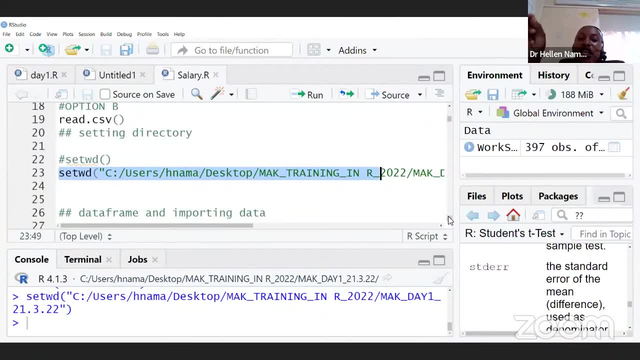 that you're seeing here. That is what I did. So in that case, I've set the working directory implying that I'm telling R that in. where you're seeing at the end, this is a folder where my data set is. So I'm telling R. 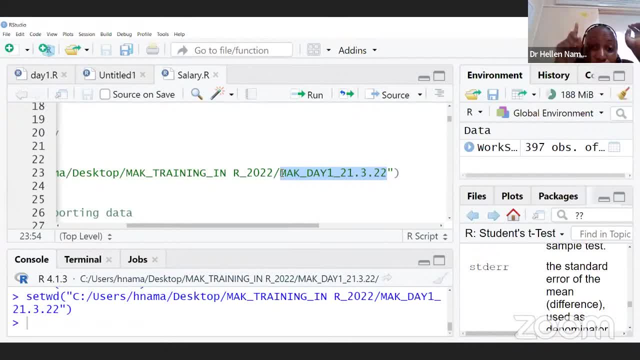 that it's within this data set. within this particular folder, there is a data set I want to bring to R. All right, So we are dealing with the. so let's see, after setting that, what do we do? We are going to use. 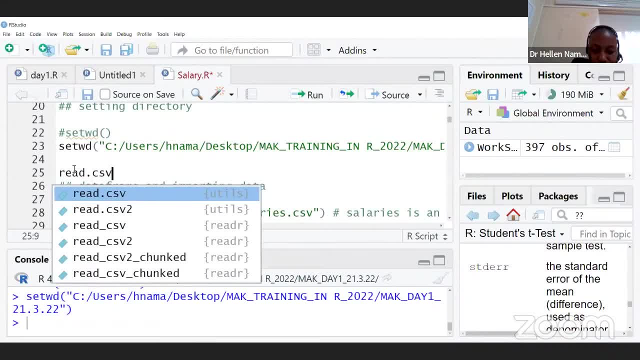 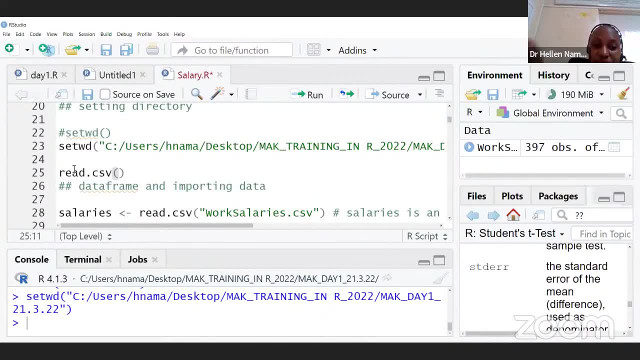 the readcsv command. the readcsv command. Inside the readcsv command you need to type in the name of the data set you are importing. In this particular case, I can say it is called worksalariescsv. This is the name of the data set. 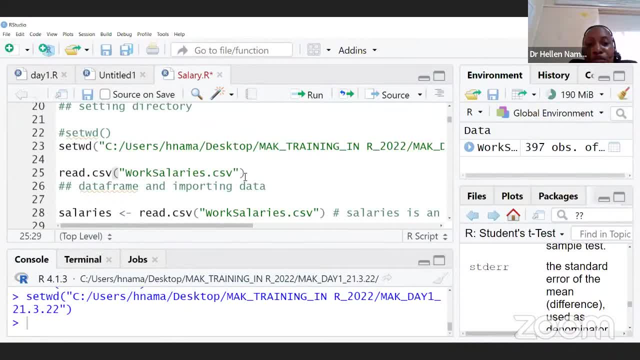 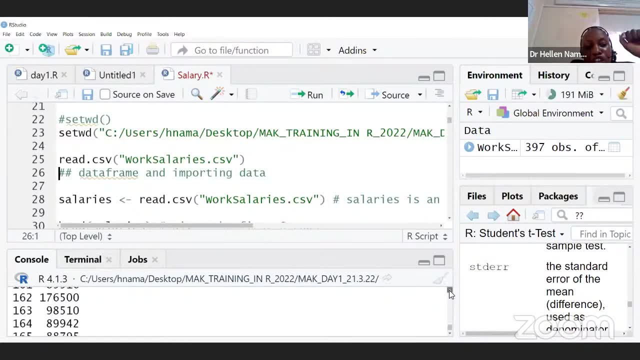 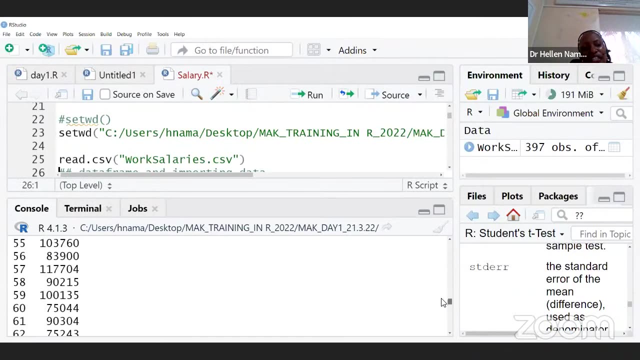 which I set with the sv extension. After that you can run this particular line The moment you run it. see what happens If you run that particular line and check in your console. the console gives you the output of it, shows you how the data set. 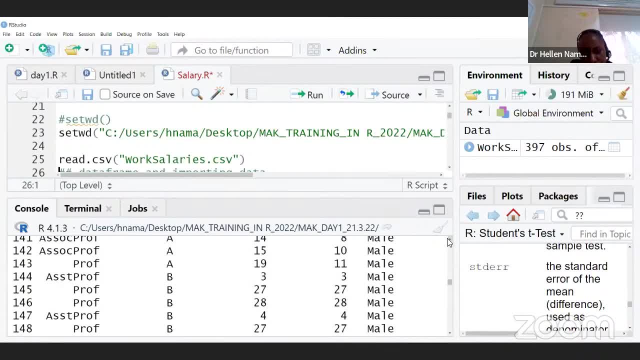 is all the results in the output, But what you're seeing here is that it is just showing you the whole data set that you're using. What about in case you're having a million data sets? Are you going to have your console to appear? 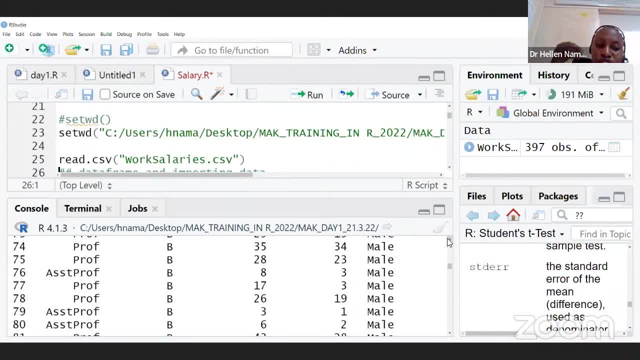 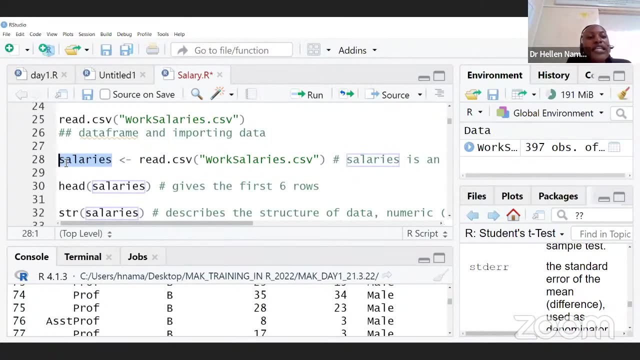 Like that. So it is always important that you save your data set in an object. For example, when you look in my second line, I said now what I'm going to do. I'm going to I create an object which is called salaries. 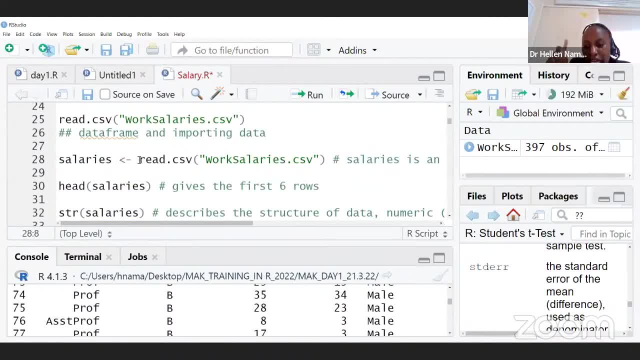 And then I say: let salaries remember my assignment. we said you can assign variables. I'm going to get a variable called salaries, Okay, Or in this case, a data set name called salaries, which R refers to as an object. 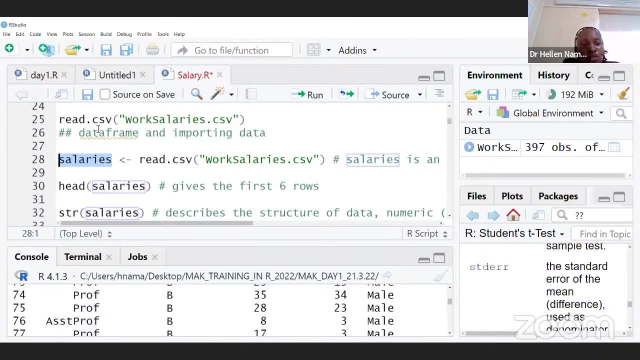 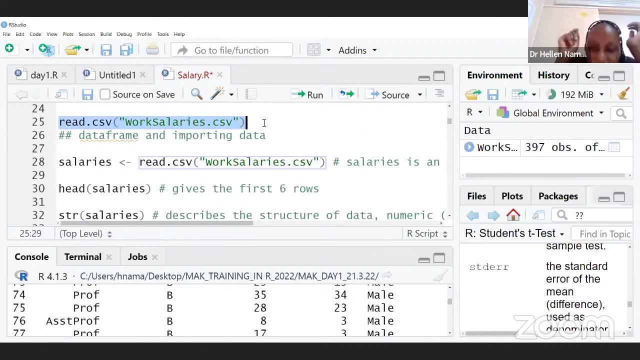 And I say that let this one be equal to, to this line here, all my data sets. In this particular case, I'm telling R that everything within the readcsv, I'm calling it salaries as the object name. So in case I run this particular line, 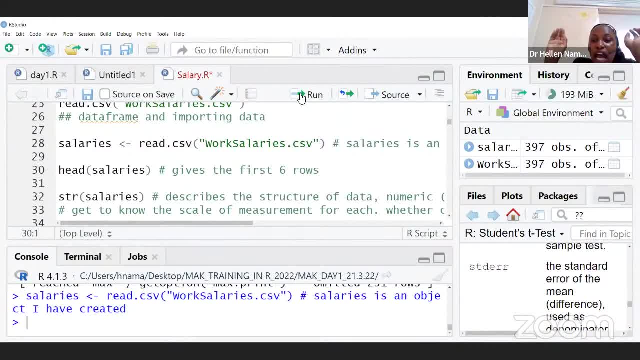 I'm not going to see anything now in my R console. However, what is interesting? when you look in the environment- I can be- I'm seeing the name that I've used- salaries- And it is also telling me if the salaries has got three. 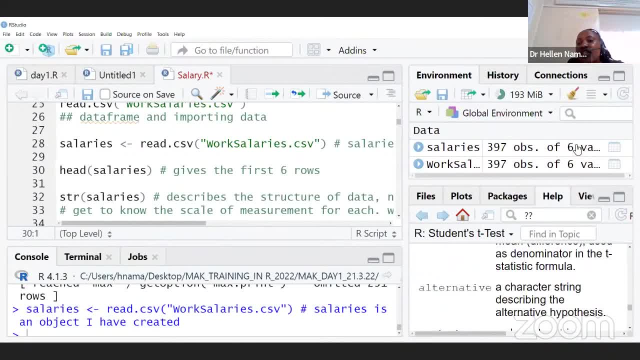 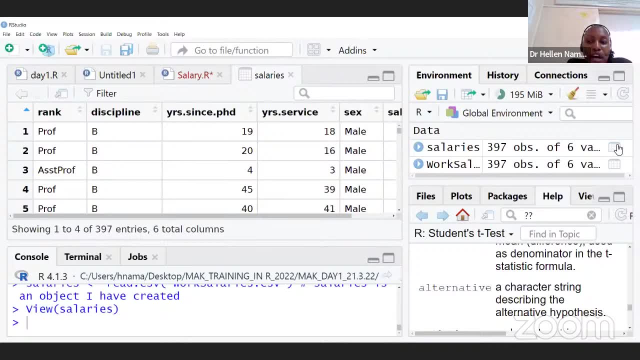 nine, seven observations and you can read further and see six variables. If you want to view the data set, you click here and it you see the data set on the icon of the Excel. If you want to close this, you come and cross that out. 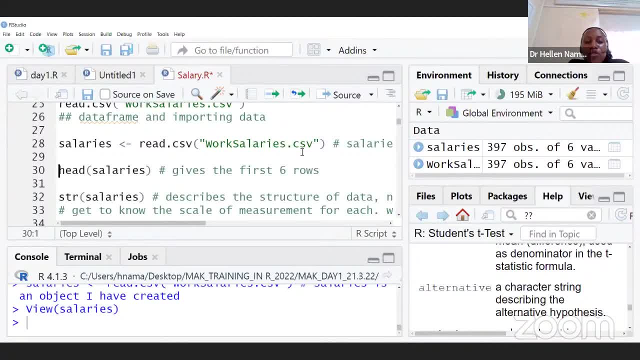 So in that particular case, you would have been able to import data successfully in R, which is saved as the csv. Okay, Let me ask in the chat: are we on the same page? Can you repeat this thing? I am no longer following. 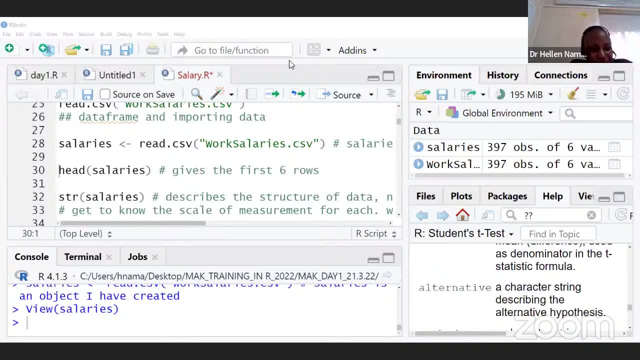 Please don't give up. I got lost. Let me see if I can see it. Yes, Repeat, Okay. I would also encourage you, like we say that we are having YouTubes or this work is being recorded. All you need to go, just Google in the forum. 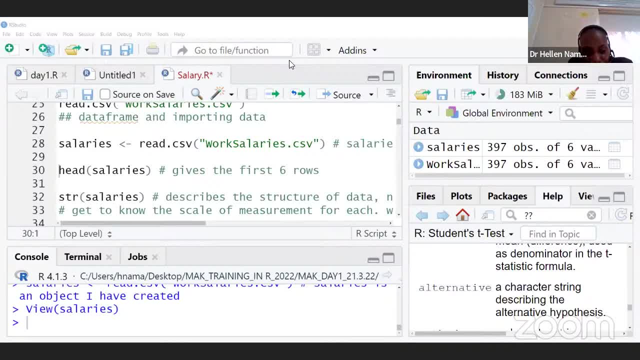 YouTube SDM series. You'll be able to see this particular YouTube and watch on your own. Okay, All right. I see a notepad. Can you repeat your two? says repeat from session. I didn't get a csv, Mm, hmm. 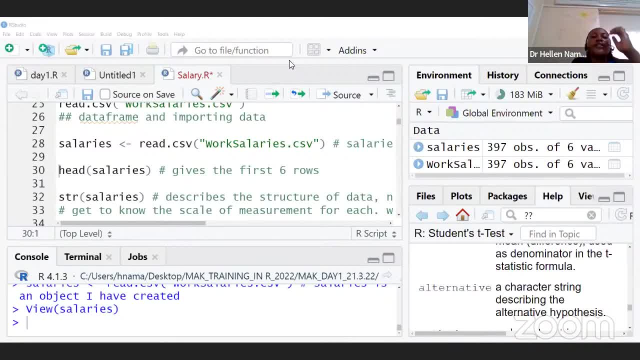 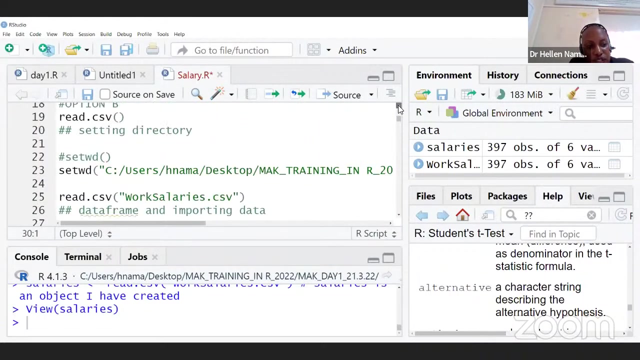 Cooked my direct but unable to pay. Wow, really, Okay. Okay, Recap from self-direct Recarry. and they said you Tube Green And send the YouTube links, like that after the session you can rewatch again. Okay, now let me redo that particular process. 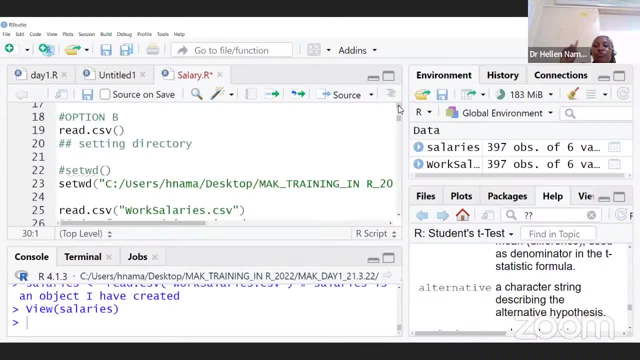 Remember, with option one, we looked at how to import data saved as XLSX, which I've already talked about earlier. Okay, the common forms. Now here we want to import data that is saved as CSV. Okay, we saw that in Excel. 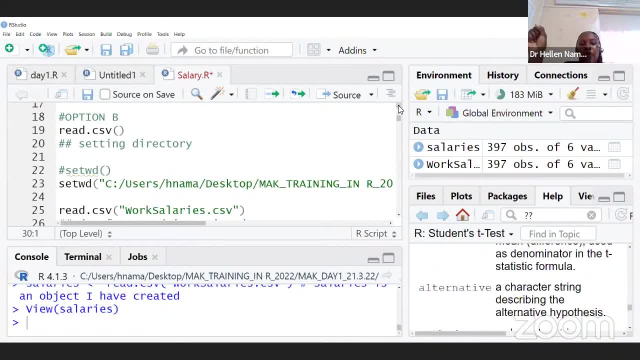 But with this kind of type we are going to use, we are going to set a directory. How do we set a directory? It's like we want to tell R that in a particular folder saved on my document, that's where the data set I want to use is. 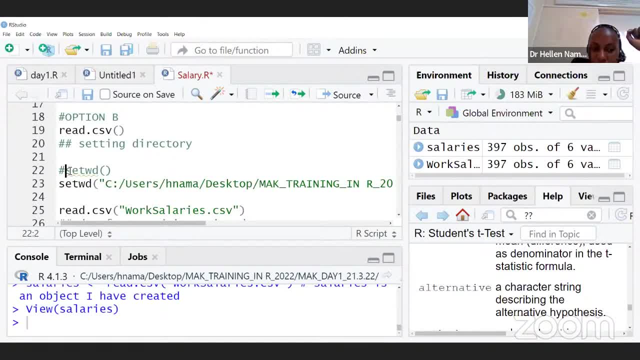 We use the command setwd, this one here, setwd. It's a command that I'm going to use to give me a particular file. It's a command that I'm going to use to give me a particular path. In this case, I'm looking for the path where my folder is. 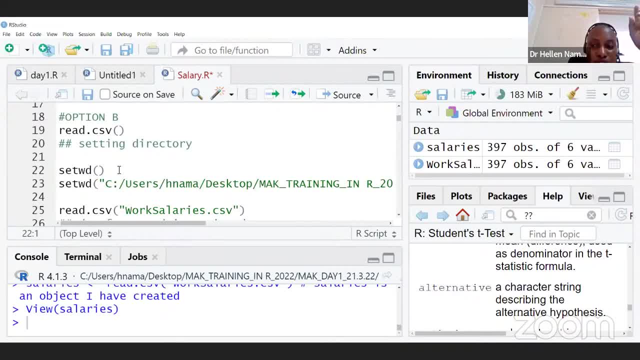 Remember even the first one. you navigate when you go to browse, So you browse and then you tell when you move from this folder. you go here until you get to the data set. I talked about comments in R, The greens that you are seeing. 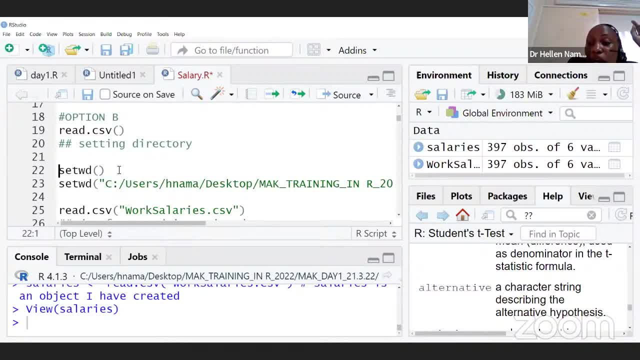 those are the comments I mentioned about. A comment is just a reminder. R sees it as inactive. It doesn't. it's not a comment, It doesn't. it doesn't react on it whatsoever. That is a reminder. It's the reason I told you. 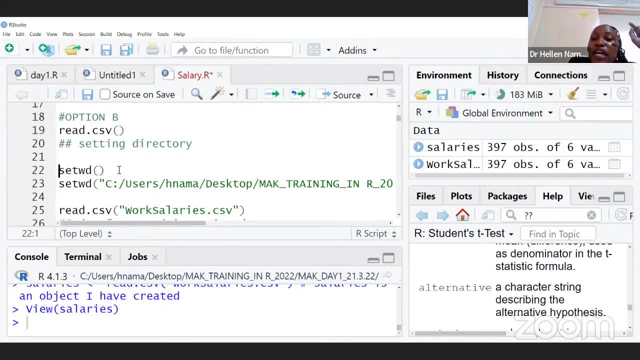 it is good to put comments like that. Even if two days pass, you can be able to come and follow up again. Okay, I can just put a comment and I say I don't want that line. So within the setwd it means set working directory. 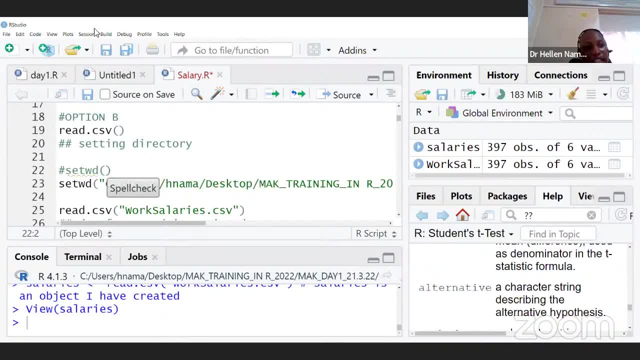 How do I do that? Let's go together What I did: come to our console, click session. Okay, After session, move downwards- Set working directory. I want to move up to the folder where I saved my work: salariescsv. 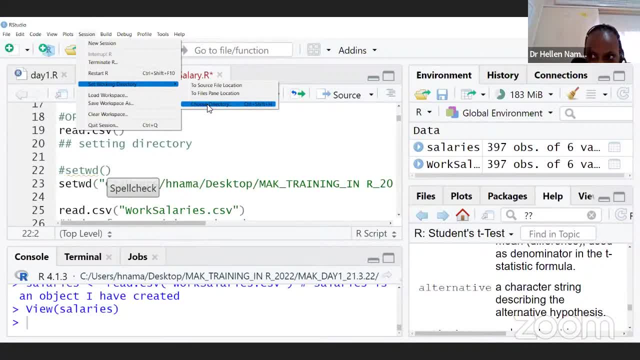 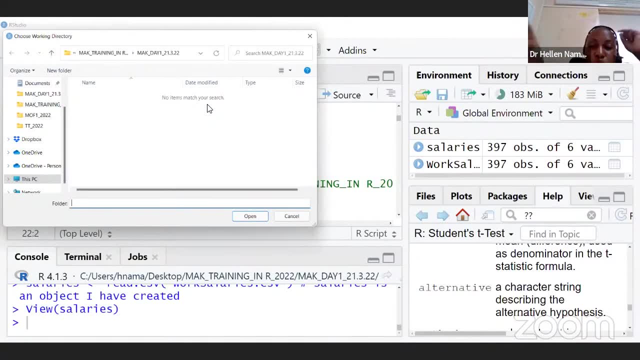 I come, I say choose directory, I click on it. The moment I click on it, you have to navigate until you get to the folder where you saved your CSV, Where your CSV data set is. Here you're not going to see it. 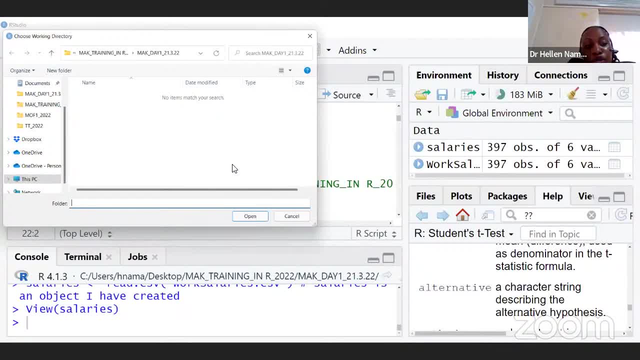 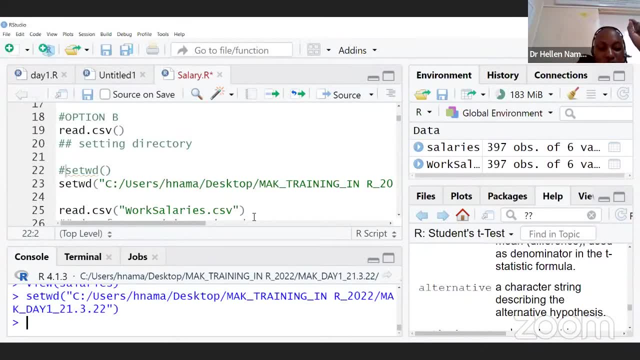 By the moment you reach to that folder, all you need to do come down here and click open. If you click open, you're going to see in your R console. you're going to see the path that you have used down here. 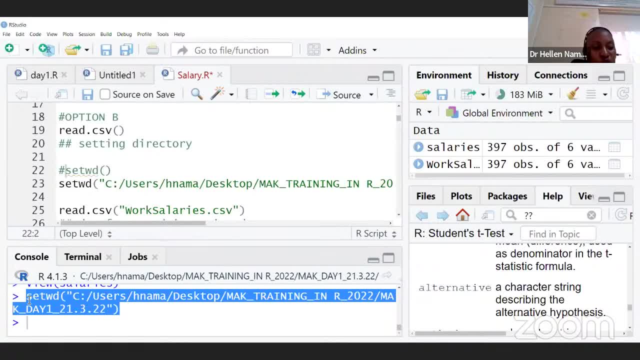 which is the setwd. All you need to do, you can click on it, You can come in case you want to store it. But even if you don't store it already, you've told it that the data I'm going to import. 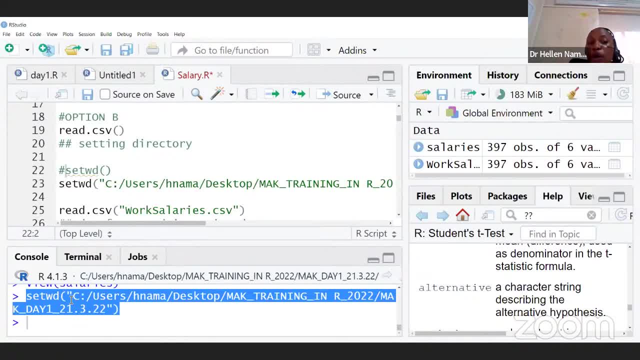 it's in that particular folder. In case you don't want to redo the session again next time, you can copy this path. You come, highlight and then you highlight, Then right click The usual copying that. we know how to copy and paste. 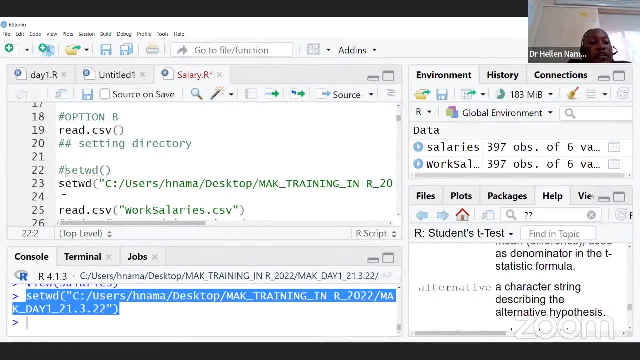 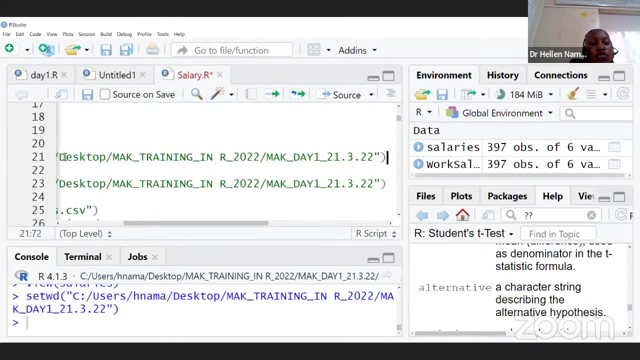 Then you can come and click copy, Then you come and paste it somewhere in the R studio. I already have it. For example, you can say control V and automatically that path gets pasted in R. Okay, The moment, such that next time, when you come, 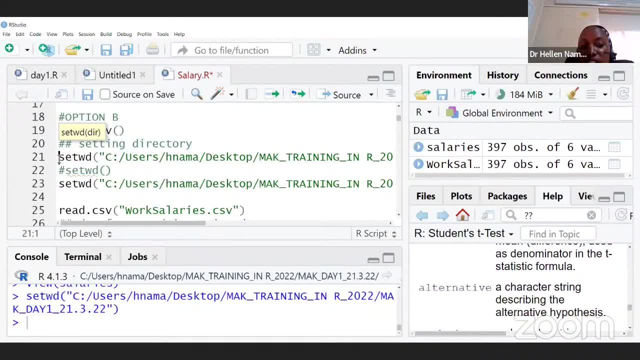 you might not need to go to session again. You just have to run that line, because it is now. it is telling you that is the path where your data is Okay. I'm going to comment on it because I don't need it. 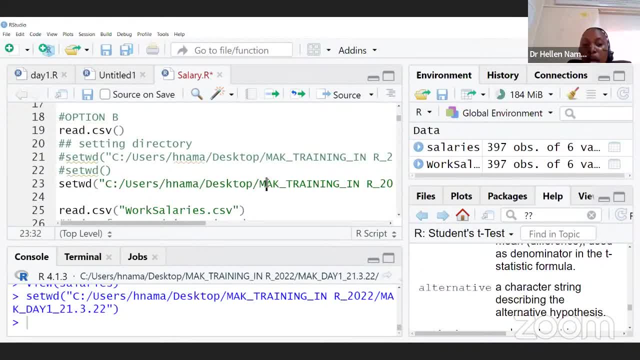 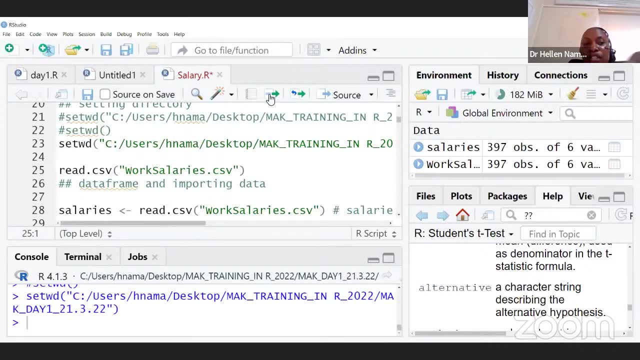 I've already. I already have it somewhere. If next time that you come, you can click anywhere and you click run, It will still be repeated down here, So I don't need to go through the process of setting a working directory. Okay, let me ask in the chat again. 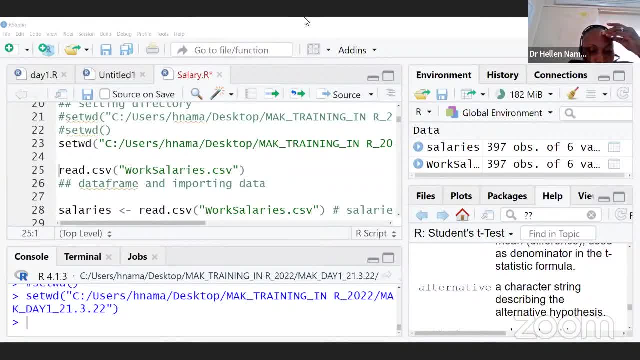 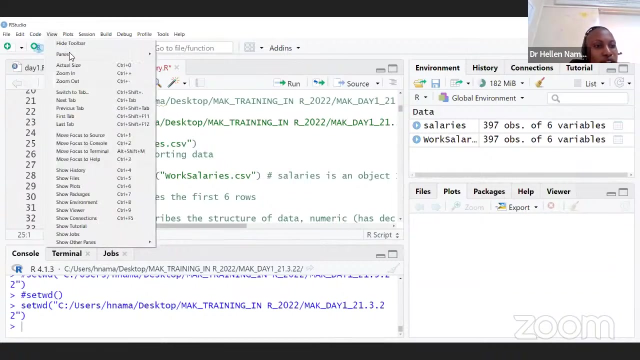 Are we on the same page? Clear your screen so as to follow you. Hmm, I clear my screen. Okay, Maybe let me try to zoom in and I reduce, Maybe, that's. but in case I zoom out, then the words are going to be small. 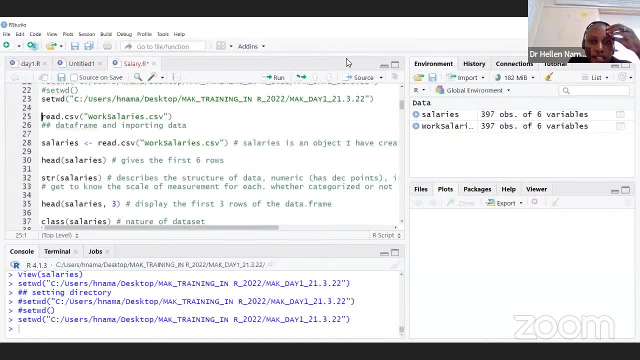 Let me ask: are you able to see the words? I've zoomed out a little bit so that you see what I'm doing. Okay, So I've zoomed out a little bit. This is the path that I copped that Ari is giving me. 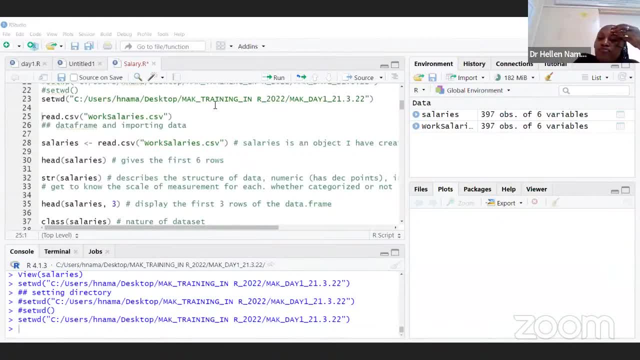 I just copped it down here after going through the session. Of course, mine will be different from yours. That's why it is important You try to do it yourself. All right, So I explained about the readcsv. This is the command that we are going to use. 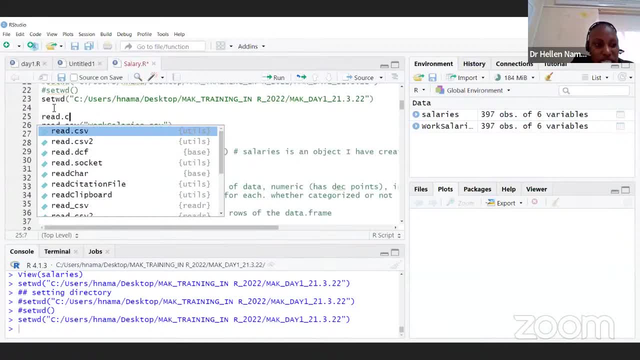 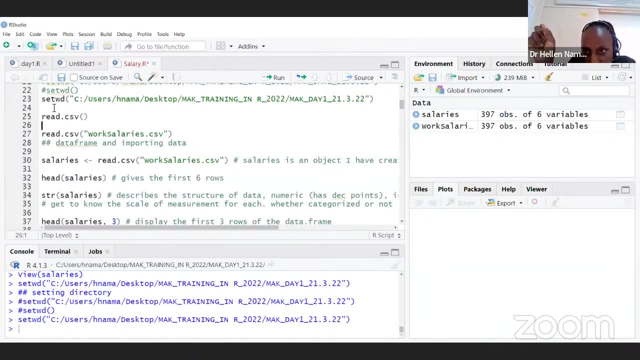 We use the readcsv command command. the readcsv command is what we are going to use to import now our dataset saved as csv. So you write the name of your dataset in the brackets of readcsv and you put them in ports. However, we've seen that, in case you just leave it the way it is. 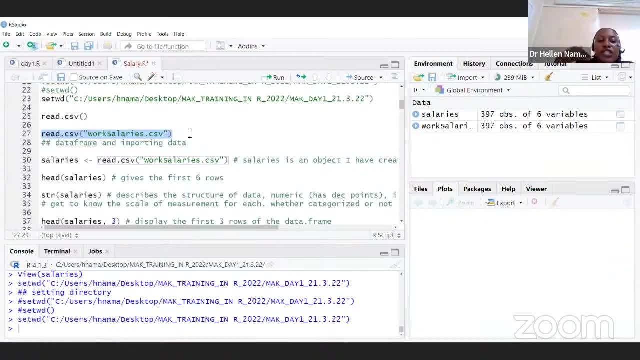 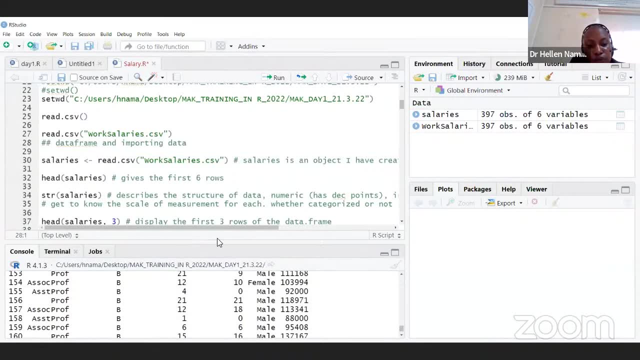 in case you just have that particular line, you see all your dataset in the R console. Like in case I click, you're going to see all your dataset in the R console. Please look in the R console and see You can also do it at your end. 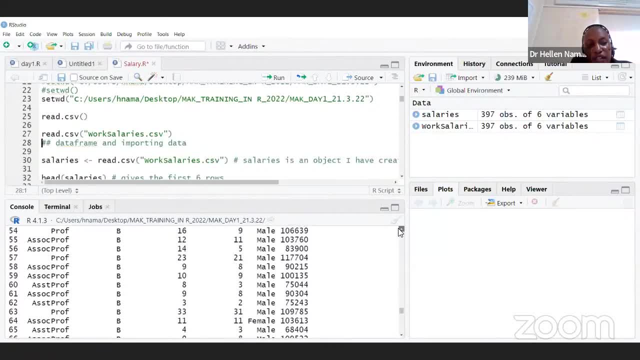 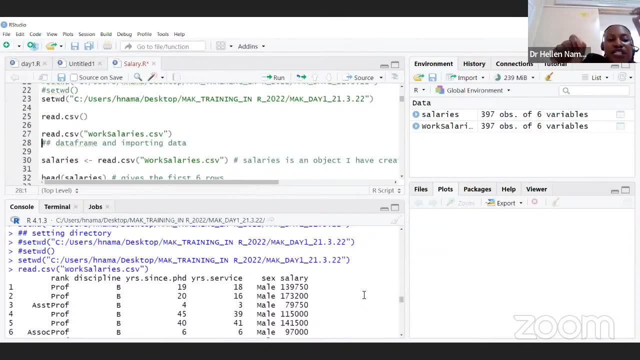 I'm seeing all my data that are being imported. So what I do? I can say that let me save now this dataset in an object. So what I do? I create an object name, which I call salaries, and I assign it the whole of this line. 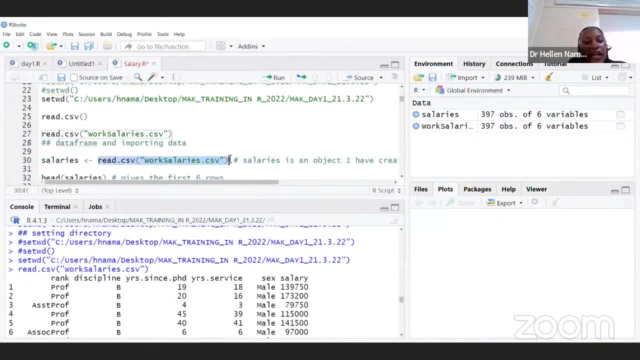 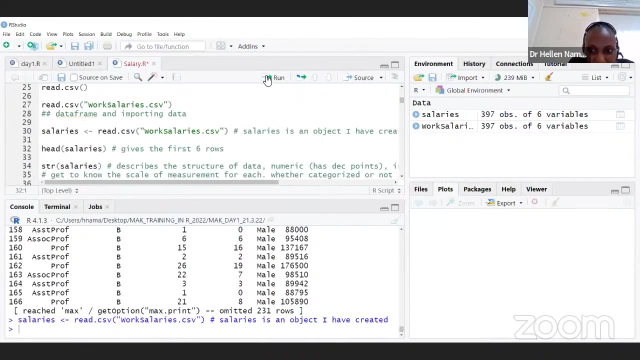 And I say salaries is equal to all my dataset. It's called salaries, by using the assignment less dash or you can use an equal. Now, in case you run this particular line, when you check here, it is showing you salaries less dash, readcsv. 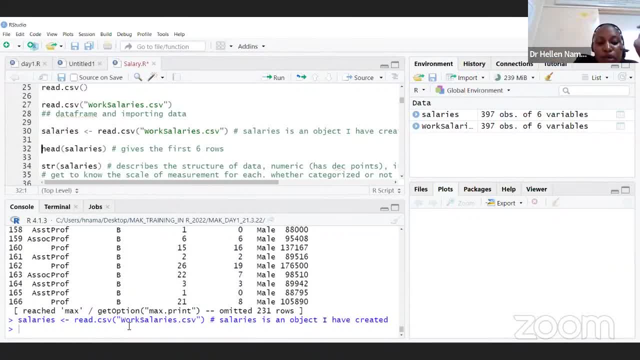 It has not brought in any error implying that I've been able to successfully import my data For you to see that you can even come and check in your environment. It is showing you the name, salaries that it has got: 397. observation of six variables. 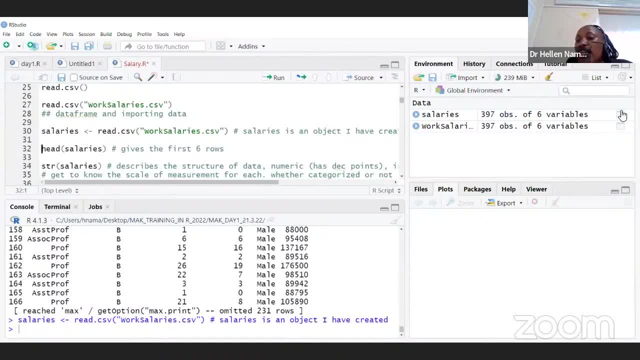 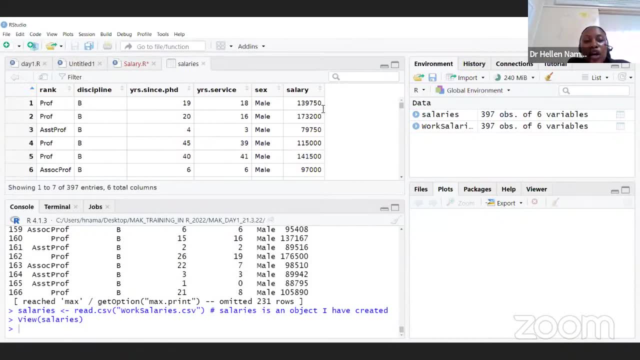 If you click here where I'm putting the hand. when you click there, you're telling our view. I want to see how my data looks like. If you click there, you'll be able to see the variable names and some of the dataset, just to cross check and see whether really the data you captured in Excel. 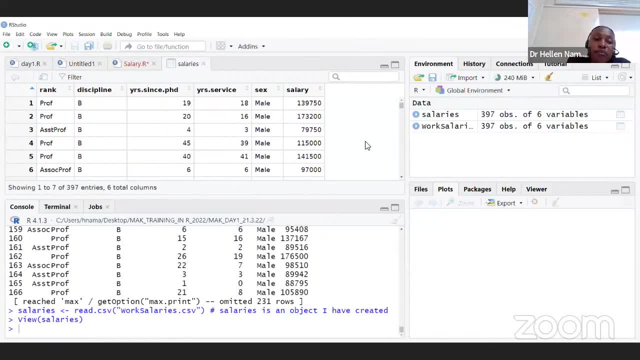 it is imported. it is the same data that has been successfully imported in R. Okay, let me ask. in the chat I was zoomed out to do internet problem. How can I get the video? Okay, so can we continue? Have we been able to? 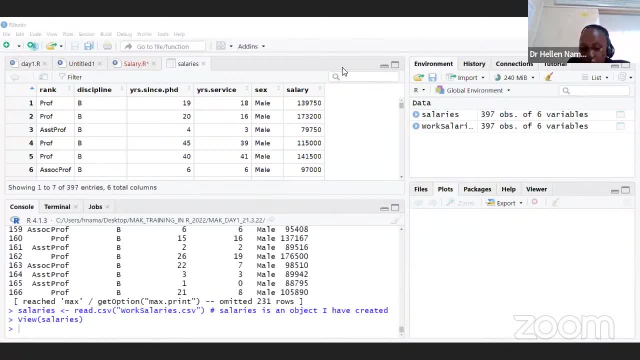 Yes, we have been able to import data in R both with XLX and CSV. I want to see if we have achieved that also for today. We downloaded, installed. Now we've been able to successfully import R. Okay, that is great. Now those are the procedures we'll keep using when we're importing data in R. 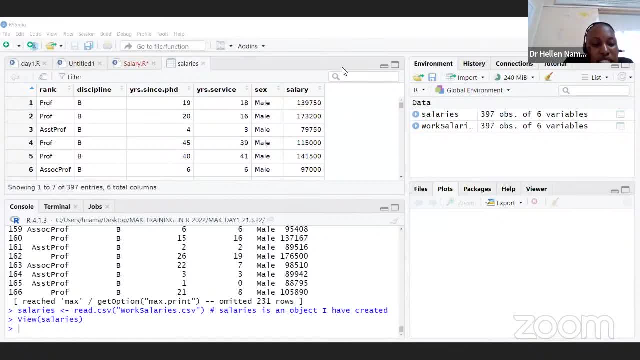 If you still feel that maybe some information is still missing, please post the question in the chat. Okay, And they'll respond to you immediately. Can we continue? If you still like I mentioned after the session, please go to the YouTube and watch again these. 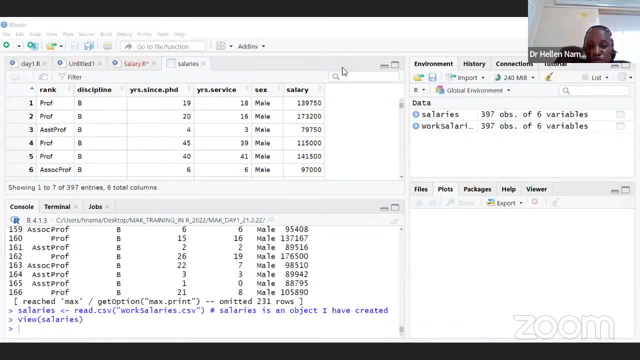 steps. Maybe you might have missed something. So in case you watch step by step on your own pace, you'll be able to follow. very well, Okay, can I proceed? Type: proceed if it is okay. Yes, continue. If you've been able to import R, okay, great. 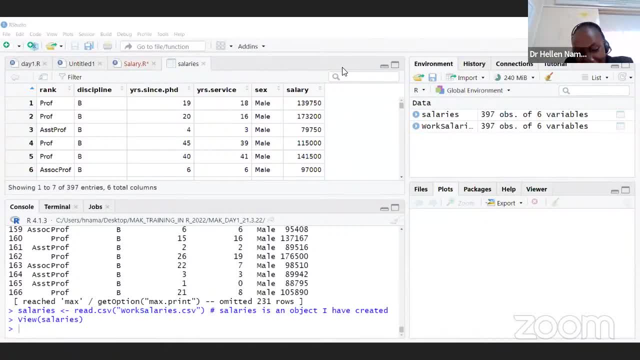 That's not. can you stop here today? Somebody's saying that. can we stop here for today, Please? we are not stopping. As part of the program, we are supposed to end at two. Uh-huh, Uh-huh. 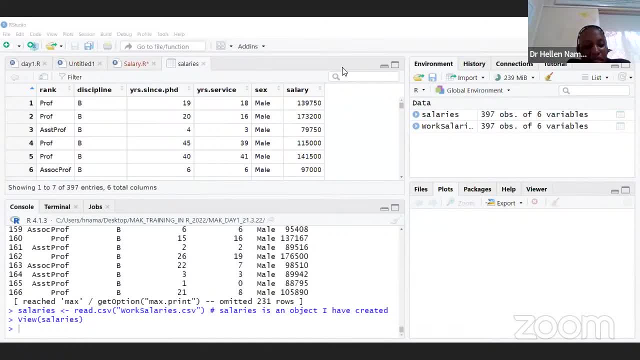 Uh-huh, Uh-huh, Uh-huh, Uh-huh, Uh-huh. Okay, Lillian, we are going to post the YouTube link, so be patient, Let's continue. We are stopping at two Ugandan time, so please bear with us. 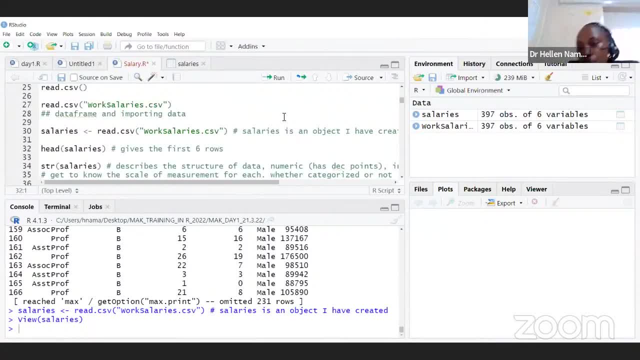 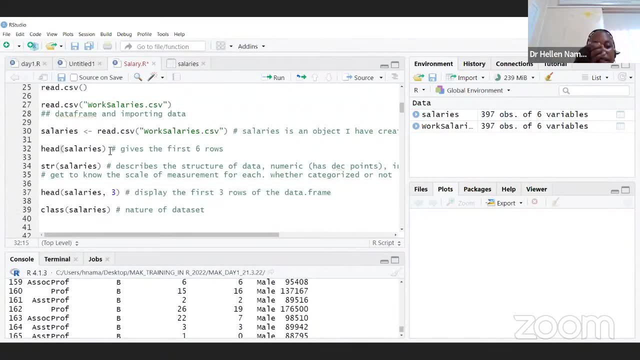 Okay, so I'm going back to the. now let's continue. Let's go through the R script that I sent And we get to know what these commands mean. Remember, now I'm calling my dataset salaries Within the salaries. it has got three, nine, seven observations and six variables. right, 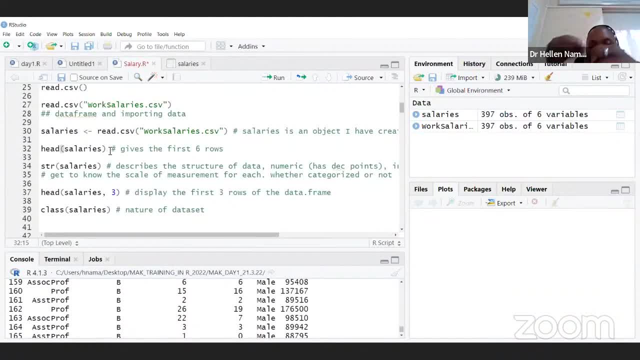 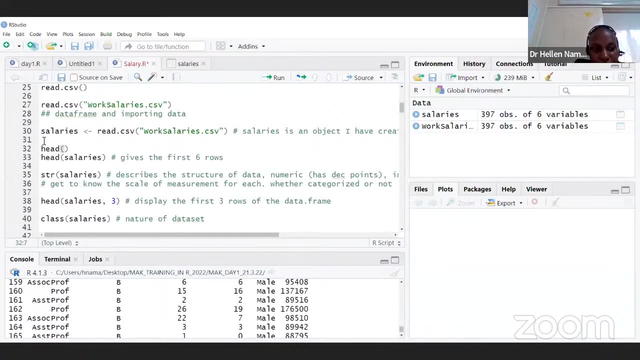 So sometimes it is good to understand how your dataset works or the nature of your variables. In case you want to see- maybe you want to see the first six rows of your dataset- we use the command head- Okay, The command head. Then inside head you type in the name of your dataset. 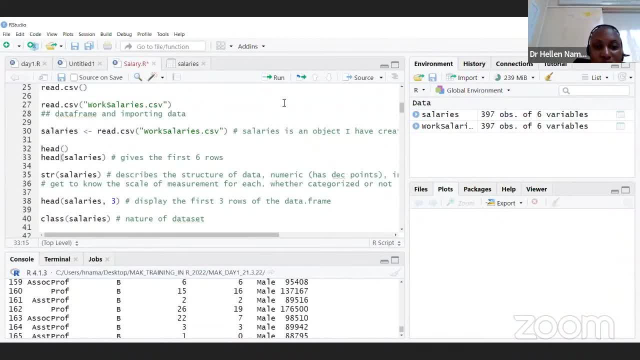 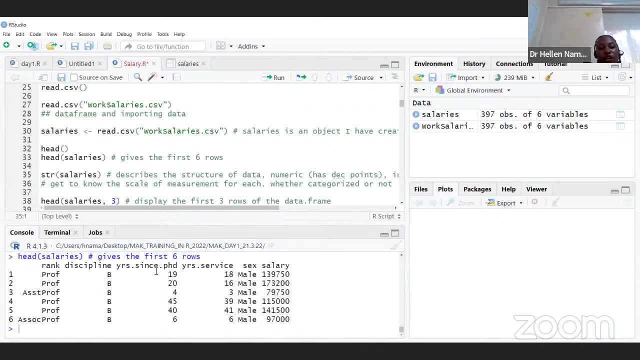 In this case it is what It is: salaries. So when you click at the end and then you click run, when you come in and check in the R console, it is giving you the first six rows. All right, You can count them here. 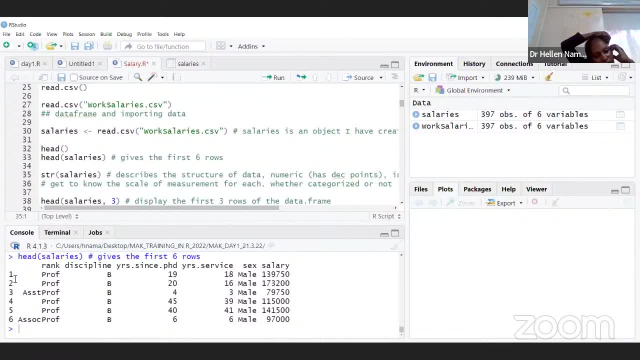 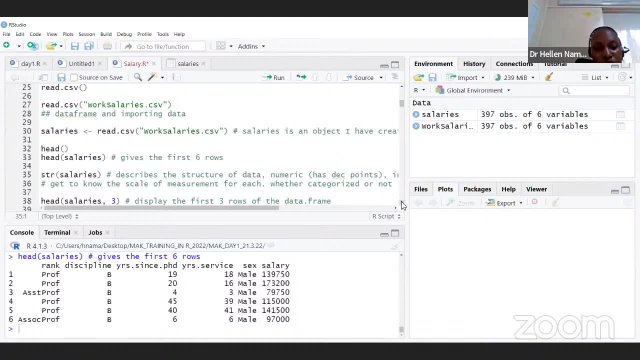 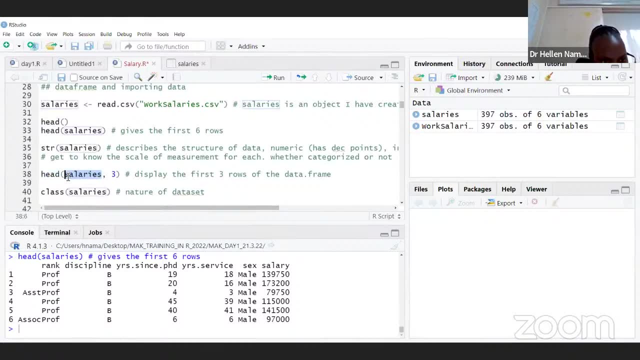 you're going to type head, you name the salaries you put in the you put, you type the command head, then the name of the dataset, that is, salaries, and then you type three. Three means that give me only the first three rows in my dataset. 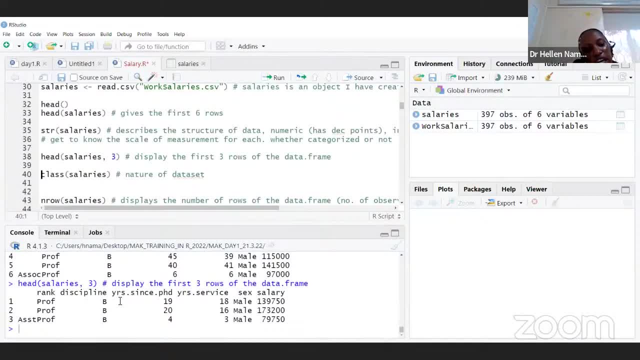 So you come on the end and you run that. When you check again in there, we say that when you execute your code in R console, it's where you see the output. So here you're able to see the first three rows. Okay. 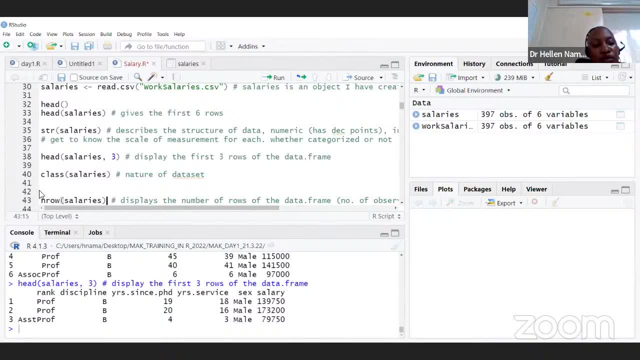 In case you're interested to know the number of the number of rows, all you need to do is to have the end row- That is the command that we are going to use- And then inside you type salaries, For example. if you run that line, it will tell you that you've got three. 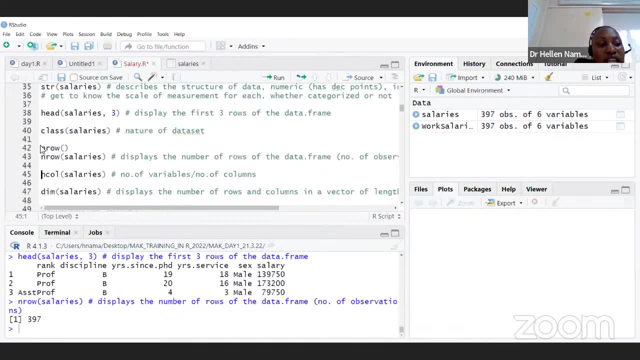 three hundred and ninety-seven rows. If you want the number of columns, you're going to have end call And then inside you type in the name of the dataset. If you click that, sorry here when I typed end call, bracket, it's, it's, there's nothing. 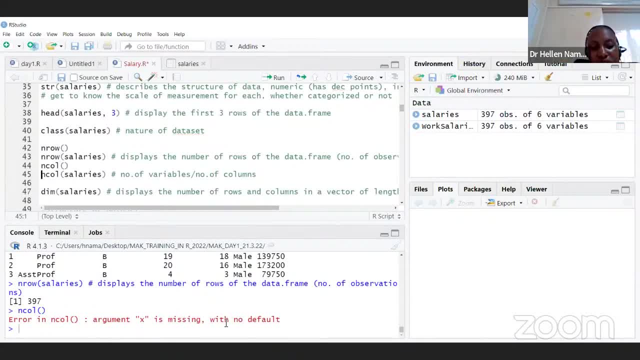 So it is telling me error in end call. Argument x is missing, with with no default, implying that I what I'm asking for. end call, but I did not indicate for what. So when I come on this particular line, n is number of columns. 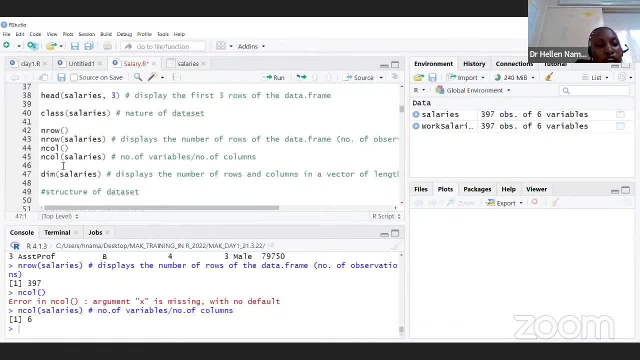 When I click it it will tell me there are six, Or you can use dime. If you type in dime and then it will give you the dimension. We place both the rows under, So I move on to remember. the other one is a code. 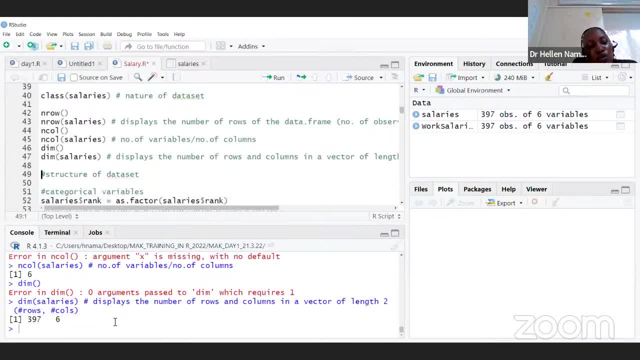 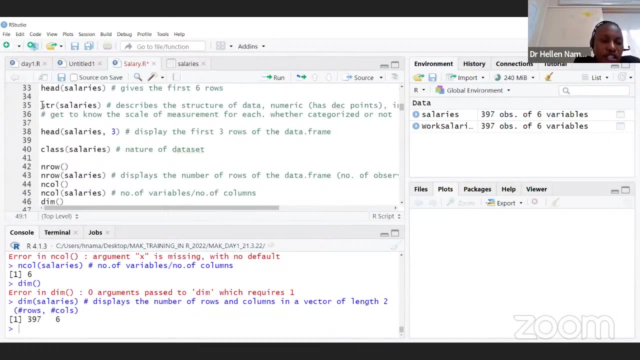 Don't worry about the reds. When you click on that it will tell you that there are three hundred and ninety-seven rows and six rows, Six columns. It is also important to understand the structure of your dataset. I'm going just back a little bit on the on the structure command str. 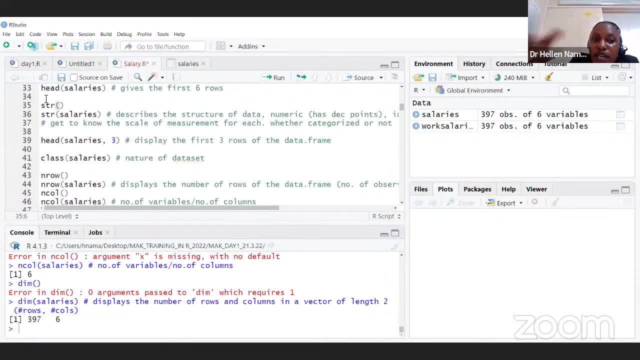 These are the foundations of r, The moment we understand them on our fingertips, then the rest of the analysis that is going to follow is going to be easy, because everything emanates from here. So the str command. it describes the structure of the dataset. 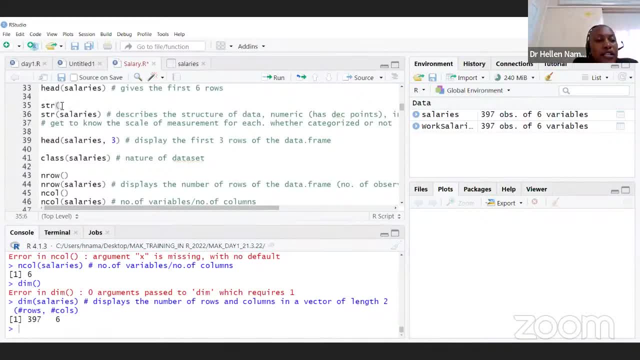 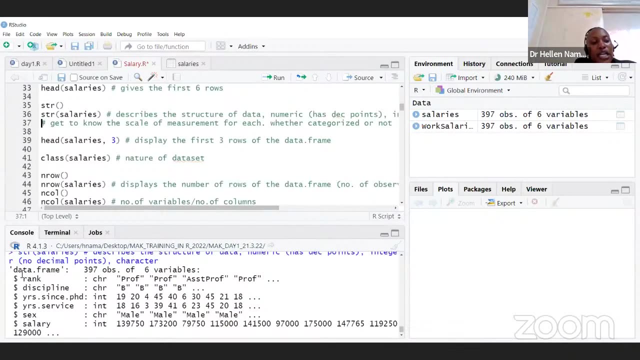 For example, inside my structure I put in salaries: Okay, I indicate salaries. The moment I run that, when I look in my R console, what I'm seeing it is telling me that it's a data frame or a dataset of three-nine-seven observations, of six observations. 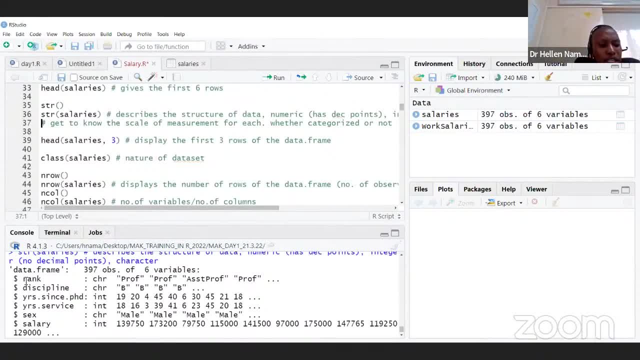 We've proved that. It is also telling me that there is a variable rank and it is seeing it as a character which has got words like prof, prof, assistant and then pro. It is also telling me that discipline. it is seeing it as a character. 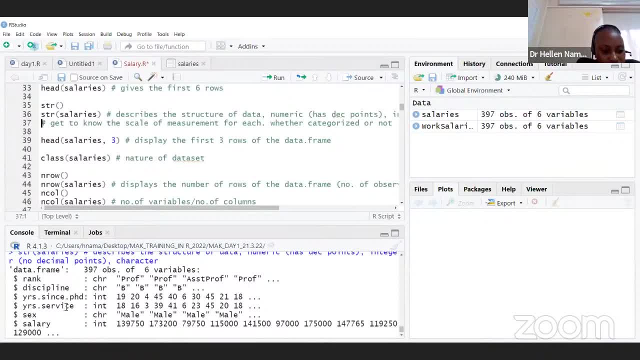 We have years since PhD is an integer, years of service is an integer, sex is a character and then a salary as an integer. Remember, with r we have either, you know the number of hours, the number of hours the. 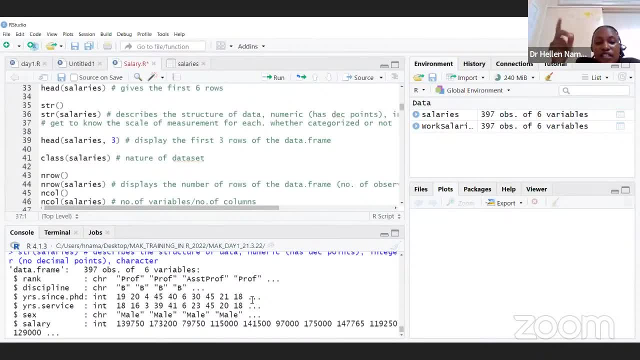 number of hours, we have a numericals. these are the integers. Like in this case, we are talking about years of service, they are numbers, And then years since PhD are also numbers, Then salary: that is numerical, It's an integer. 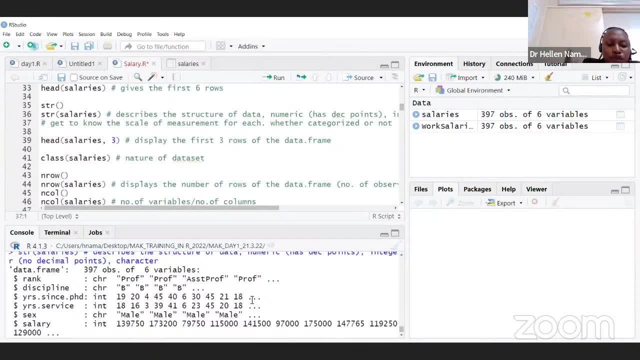 Okay, But now R is telling me that, for it is saying that rank discipline and sex are their characters. it's like they're just words. You need to tell R that. no, as we proceed on to the analysis, kindly see rank discipline. 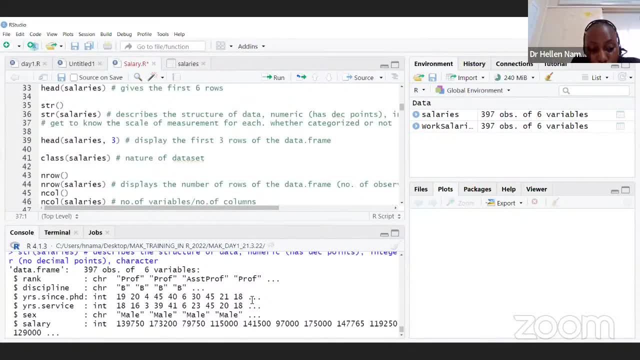 Discipline and sex as categorical variables. Remember, with discipline we've got B, we've got B and A, whereby A are the humanities and then B are the sciences. With rank, we've got three levels or attributes: We have assistant professor, associate professor and then professor. 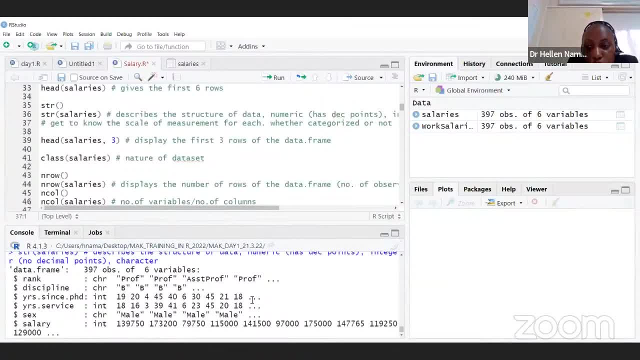 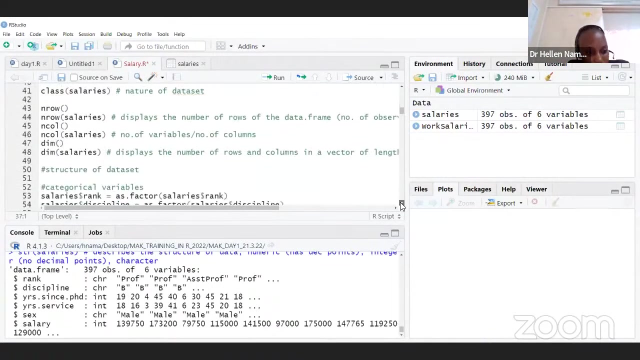 Those are three levels. And then with sex, we have two, male and female. So how do you instruct R? We talked about that. you have to tell R that you know rank. my categorical read these particular variables as factors. So we use the factor as a factor command. 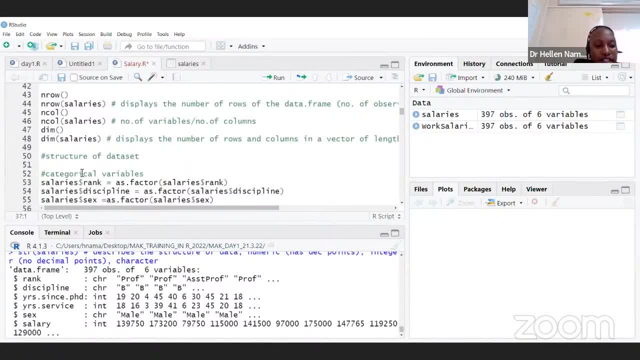 So it's what I'm going to do: telling R that the factors, the particular variables, they are factors, So we use the as factor command. This is what we are going to use, Okay, Also, it is important that, in case you're working in R and there is a particular variable, 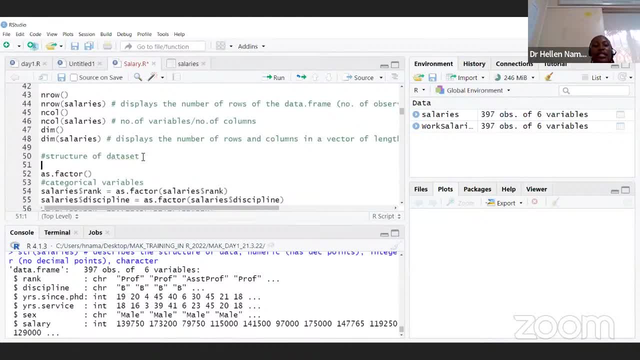 that you want to pick. for example, in my salaries data set, in case I'm interested in rank only what I do, I use a dollar sign. I tell that go to my salaries data set And pick for me. I put a dollar sign. 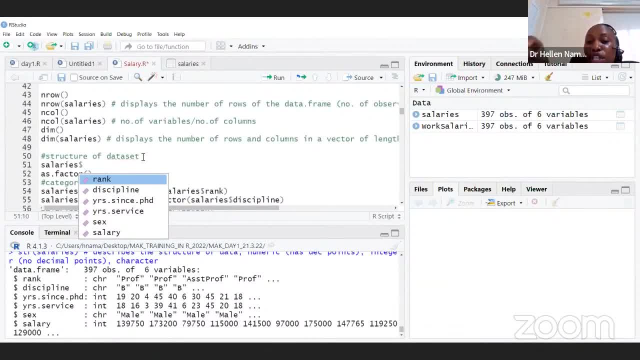 And, of course, because this is already stored, R has already stored these particular variables. So it is telling you: okay, from salaries what do you want? And I say: pick for me rank. I click on it And then I say I want you to read this as a factor. 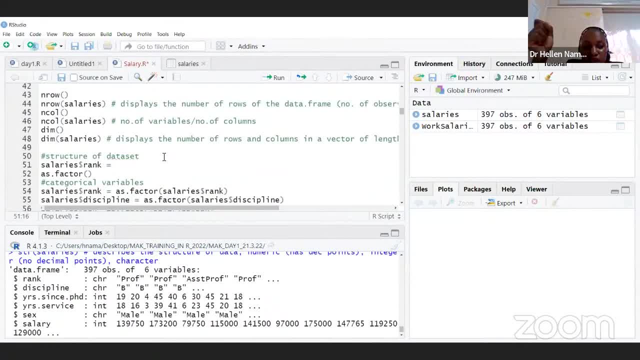 Okay, As a categorical variable. So I use as a factor command. I say as a factor, What do I want to read as a factor? Go back to it is still salaries And then read for me rank. Okay, I do the same for discipline. 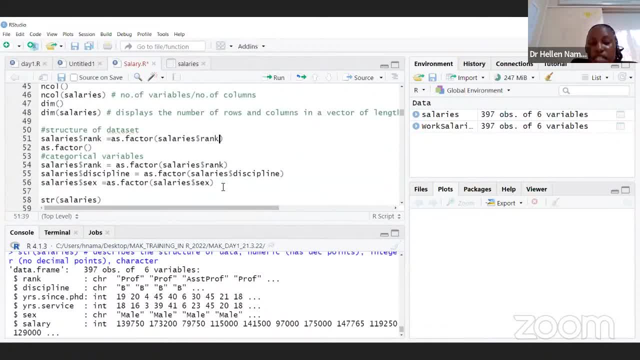 I do the same for sex. The dollar sign implies that I'm picking this in particular. I'm adding this Within this particular data set: pick for me Rank. I use that dollar sign Within the salaries data set: get for me discipline. 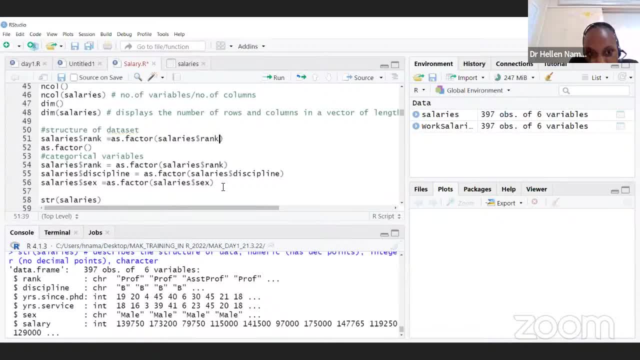 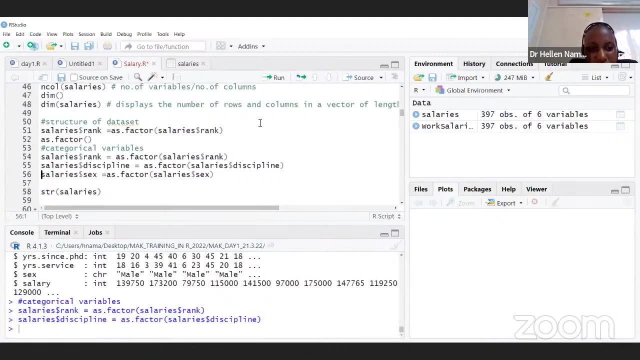 Because I want to read it as a categorical variable. So these are the three lines that you're seeing here Telling how to read them as categorical variable. So I come and I run that line as a factor, I run discipline as a factor. 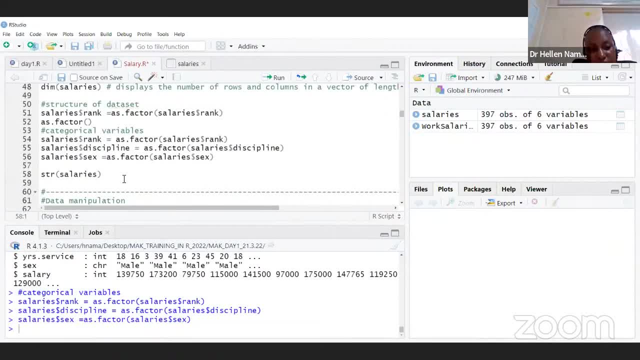 Then I come to sex and I run that Now. later I can, I can recheck again and see Now how is our seeing my three variables that are that. that are that are that. I've told you to read that as a categorical. 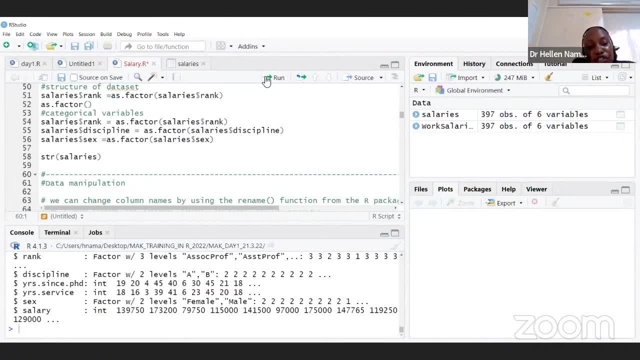 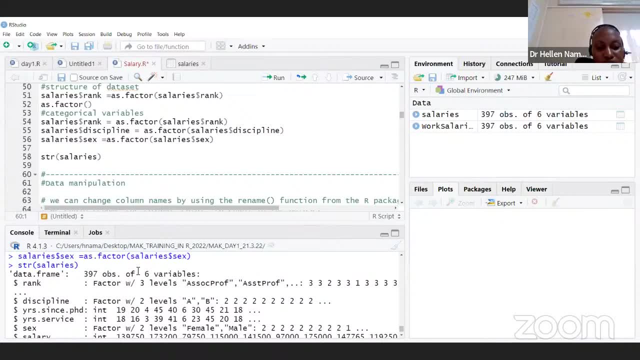 If I check salaries, if I run structure again, please see what is happening in my structure. Now it is telling me, yes, we still have the same number of observation and variables, but now it is reading rank. It is saying it's a factor with three labels. 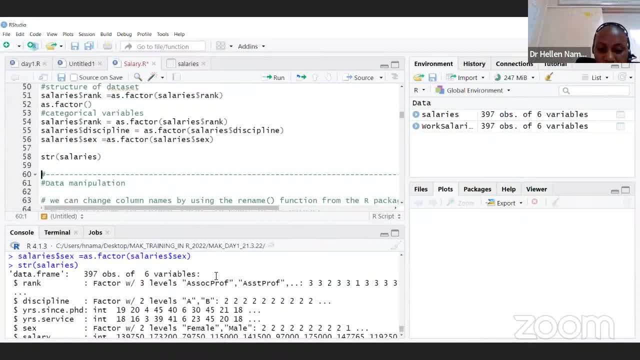 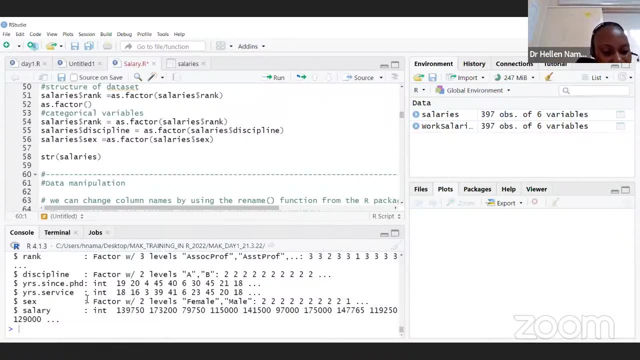 Okay, The three levels. Now it is an associate, assistant and then professor. It is seeing discipline as a factor with two levels: A and B. A are the humanities, B are the sciences. It is also now reading sex as a category, as a factor, with two levels: female and male. 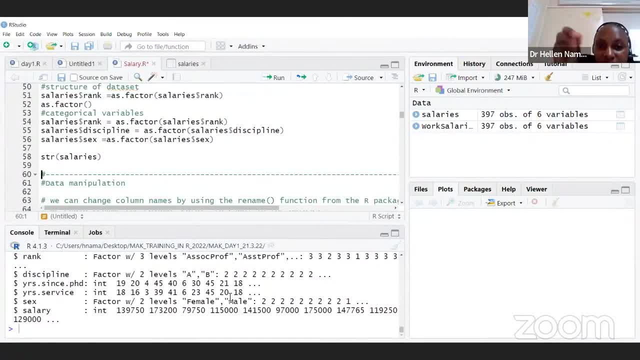 So, given that now R has been able to read the data the way you want it, you are good to go And start data manipulation, or you whatever that. you want to move on with the analysis. Let me check in the charts. Are we on the same page? 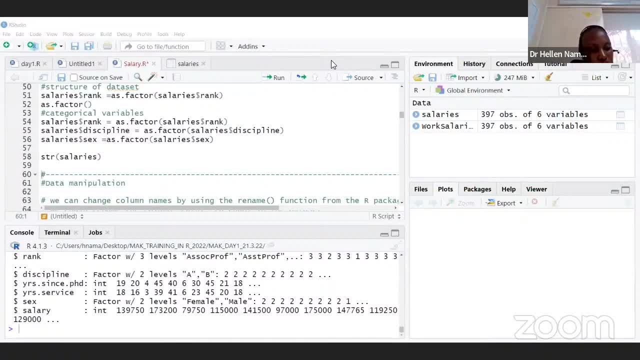 Um, James is saying no, not by me. Okay, Okay, Okay, Okay, Okay, You also need some time to run the commands. Okay, All right, Listen to seeing. uh, let me hope as you, as you're posting, you're also trying out. 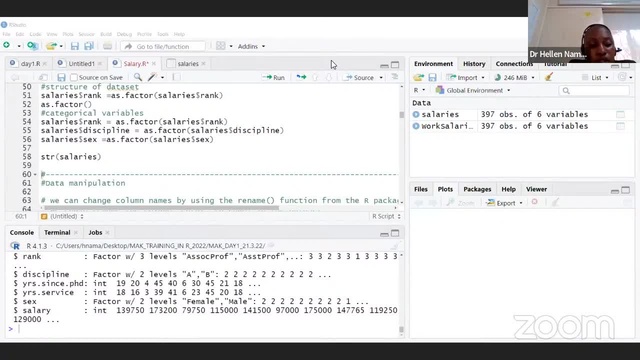 Yes, we need to run those commands. Yes, but we don't need to change the variable. Why do somebody is asking that? Why, Why, Why, Why, Why do we have to change a variable to a factor? Remember, um, initially, before changing it to a factor, I was seeing it as a character. 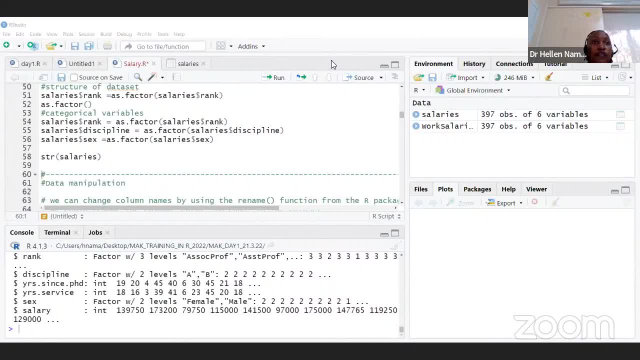 If for it it was seeing weddings. So if you tell it that no, look at this variable as a factor implies that you're telling R to look at it as a categorical variable. that is variable. discipline has got to. it has to. 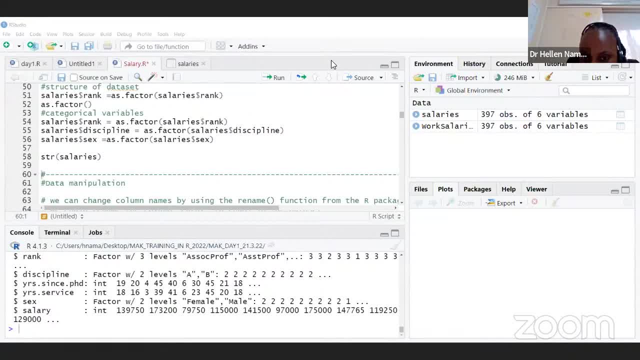 But it has two levels or two attributes, or two categories. All those words imply the same: a and a and B. Okay, Okay, Um, kindly follow through. And that is the reason why I'm I'm changing initially to as a character. 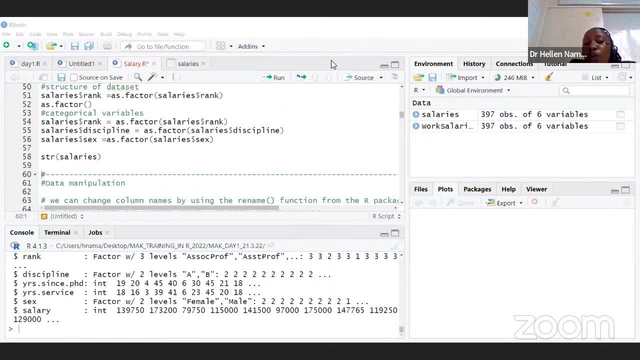 So it is always important to look at your data and see where. why is it that R is reading My data as a character? if it's a character, yet you had stated it, yet you have. you want to read it as a, as a categorical variable, then it implies that, uh, you need to combat it to a factor. 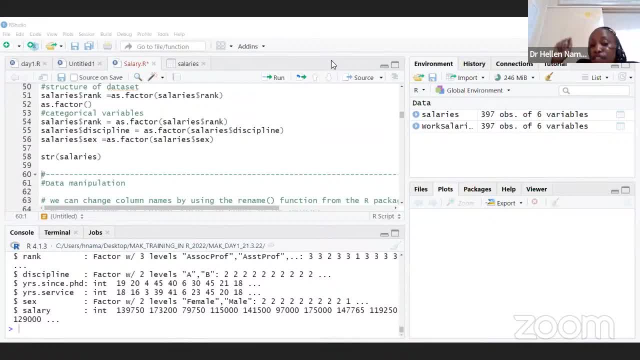 That's the reason why I mentioned earlier about the levels of measurements, Why they important. Why is it important for you to understand the nature of the variables that you're collecting? Because they're going to support you to understand the type of analysis you're going to do. 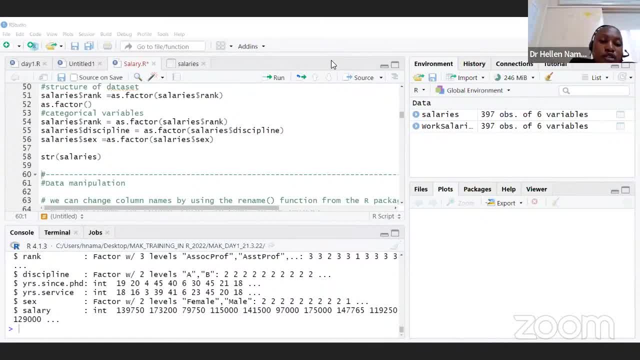 Okay, Put in because sometimes the operator says, Oh, I shouldn't go to my customer, I should first. Okay that you're going to think about your interpretation as well as the interpretation that you're going to use. Okay, Okay. 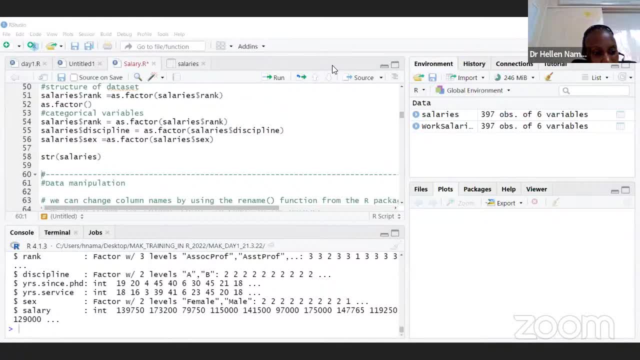 Let me ask him the chat again. Um, have you got in why we are converting characters into factor variables? Review: Okay, Isaac has also said it's fine now, but not the whole process. Okay, All right, We are getting there. 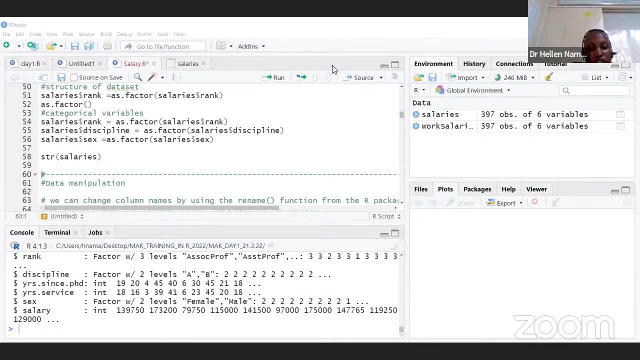 Okay, not really, In case you came in late. please, the recordings will be available. We are not going back, All right. Okay, Let me recap a little bit, just for those people who feel something is still missing Now, like I. 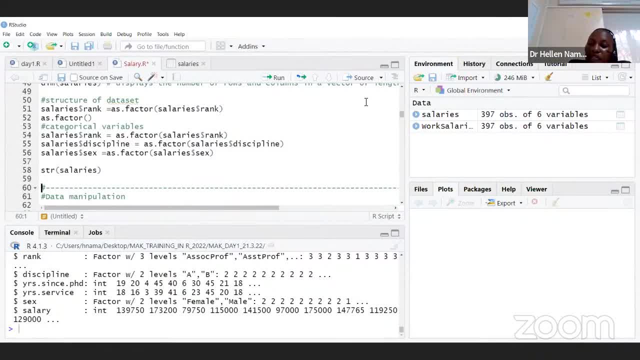 mentioned earlier the way you enter your data set. if you successfully imported your data set in R, that is very good. That is the first tick. However, it is important to understand the levels of measurements, or what your data really entails in. 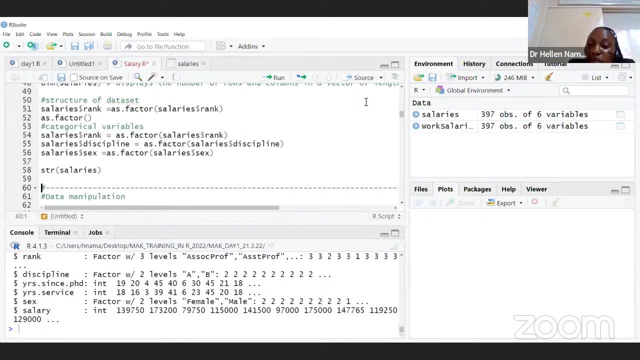 What does your data speak And it's the same language that you want to tell R. Okay, In our data set we already know that there are six variables and 397 observations. However, some of these variables are categorical in nature. They are not numerical. 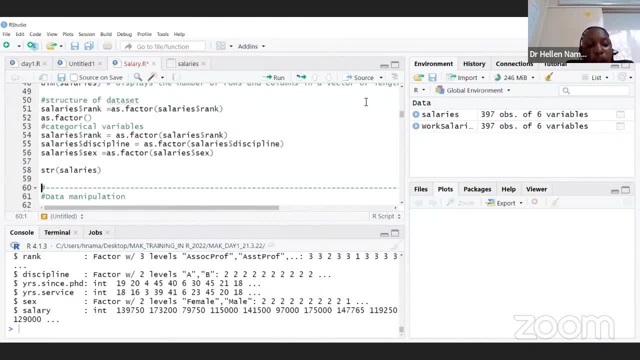 Like years of service, it's numerical, It's an integer. All right, Yes, since PhD it's an integer. Salaries: they are integers. In other words, they are numbers. R is reading them as that, But it was. 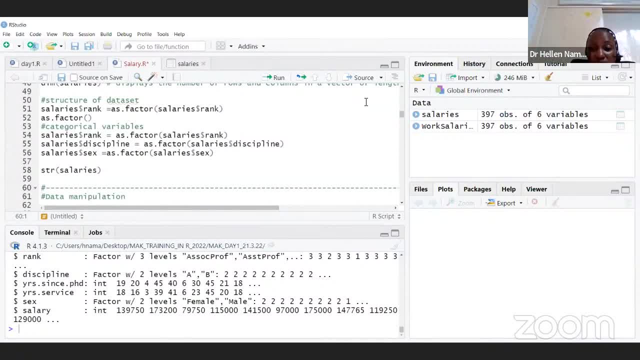 looking at discipline, rank and sex as a character as if they are just wordings. So you need to tell R that you know what as I proceed. before I proceed to the analysis, these three variables in this data set, please look at. 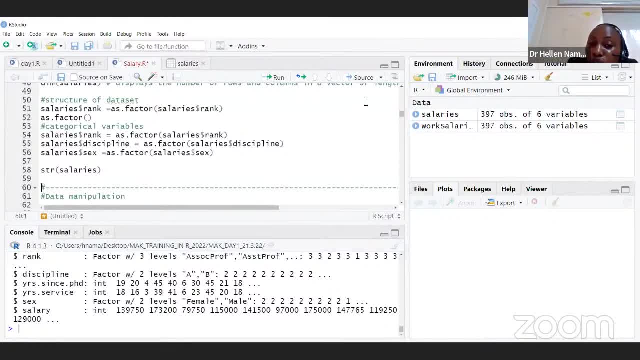 consider them as categorical. They are categorical variables, So how do I specify that they are categorical? I use a command as dot factor- This one here- As dot factor command. it's going to enable me to tell R that the variable I'm using looking. 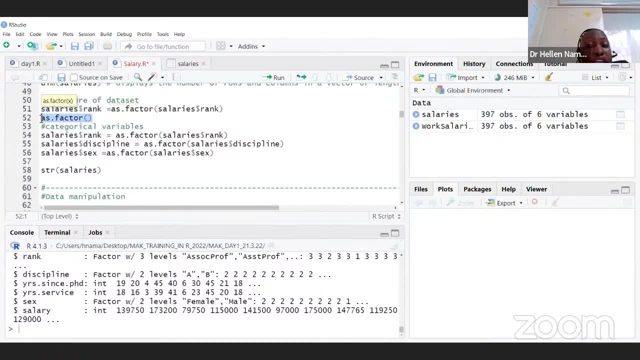 at this particular variable. I'm using R. It is categorical in nature And I say that we've got many variables, but in case you want to pick one at a go to tell R that you know what. this is a categorical variable. 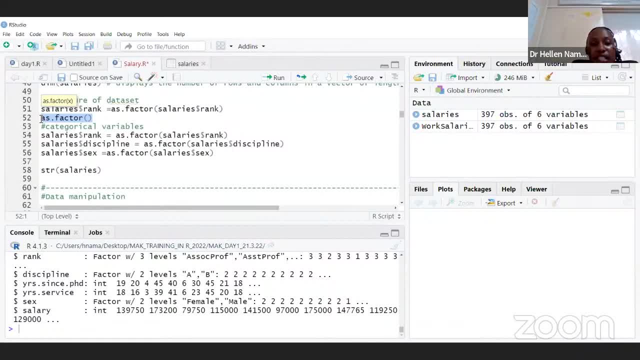 What you do. you start with the name of the data set, which we call salaries, Then you put a dollar sign. A dollar sign attaches a certain variable, a specific variable from the data set. So what I did in the first one: 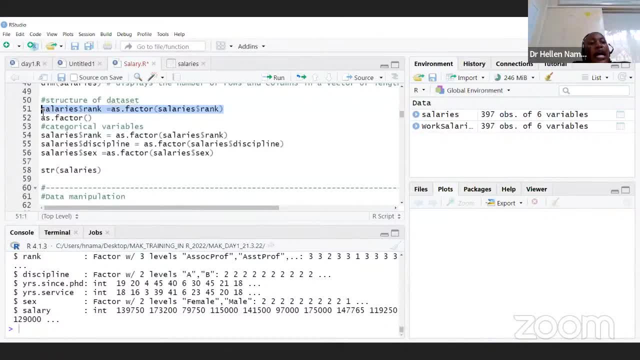 kindly follow through this line. here I had salaries, a dollar sign that within the salaries data set, pick for me a variable rank. When you pick it, read it as a categorical variable. In other words, I say that this one is equal to as dot factor. 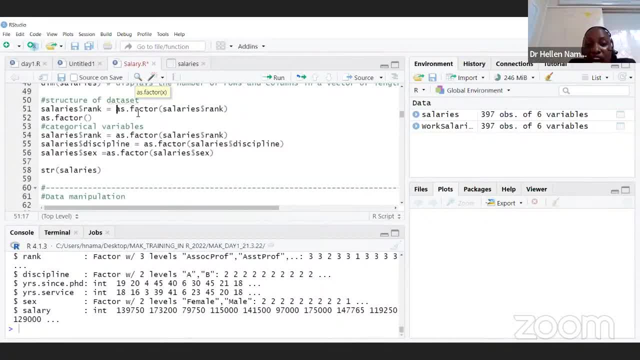 Inside the bracket, I put what I want to be read as a factor, which is the same thing here. Okay, And I said yes, even discipline is a factor. It's a categorical variable. In our language, we refer to it as a factor. 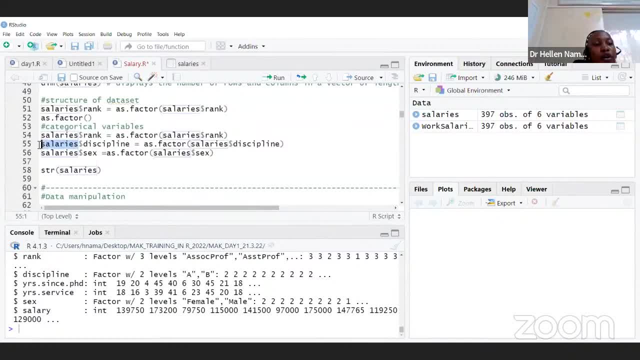 So what I do? I do the same thing. I say from my salaries data: set dollar sign, pick for me discipline, And then read it as a categorical variable by using as a factor. I do the same for sex, But from my salaries data. 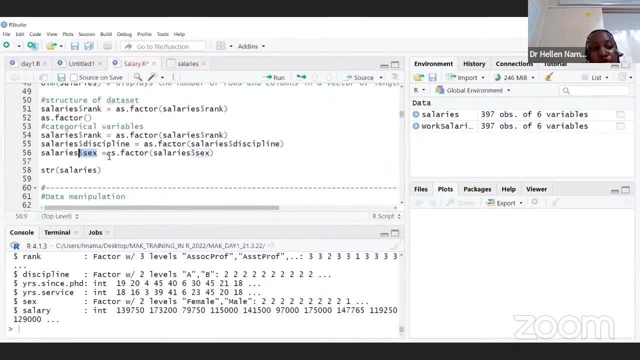 set pick for me: the sex variable. read it as a factor that it is categorical in nature, And then in bracket you put salaries, then dollar sign sex. So I rank these variables. I rank these lines again. You can read them at a go: 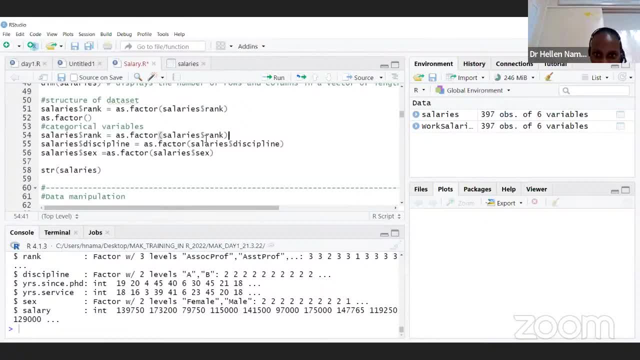 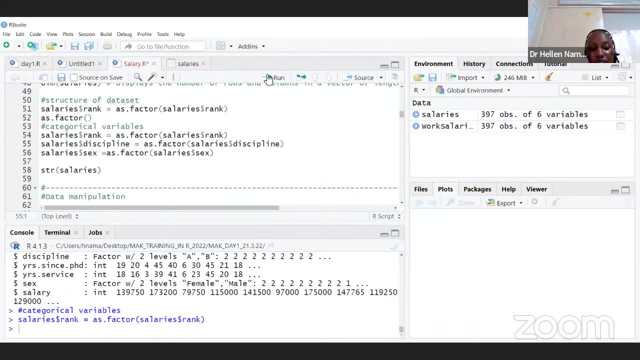 or you can read one by one, It doesn't matter. So I can run that line. The moment I look in my console it is showing me that there is no error. It has been successfully run. When I go to the second one, the same story. 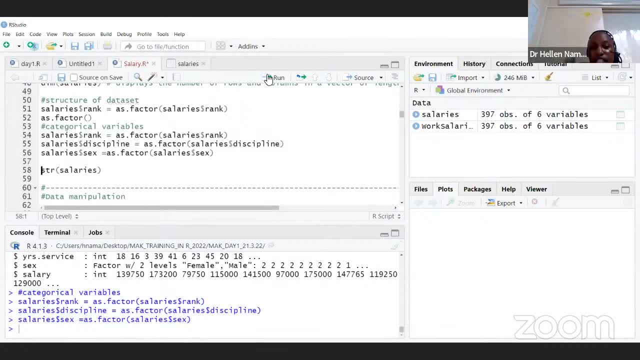 When I go to the third one, the same for sex, Then now I say let me click the, let me see the STR command again, the structure, and see whether, and check whether now what I wanted has changed in my data set If I click that. 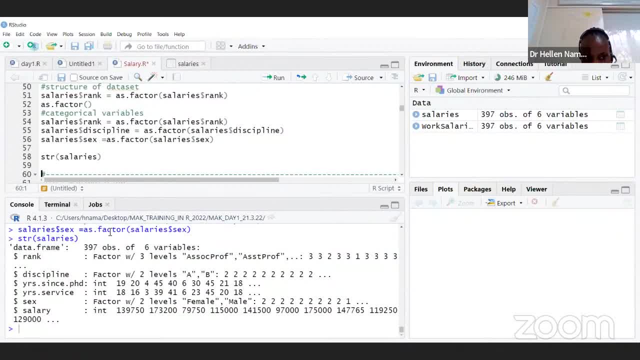 one when you come to the R console. now my things have changed. The variables that I had, which were initially read as characters, they have now changed into factor Number one. it is showing me rank that it's a factor, implying that it's categorical. 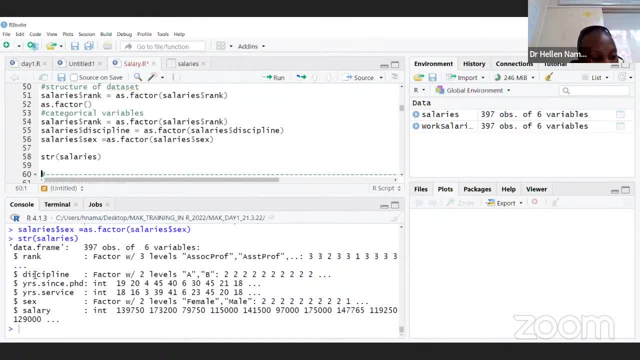 with three levels. When you come to discipline, it is showing that it's a factor with two levels: A and B. When you come to sex, it is showing me that, yes, now it is a factor with two levels: a, female and a. 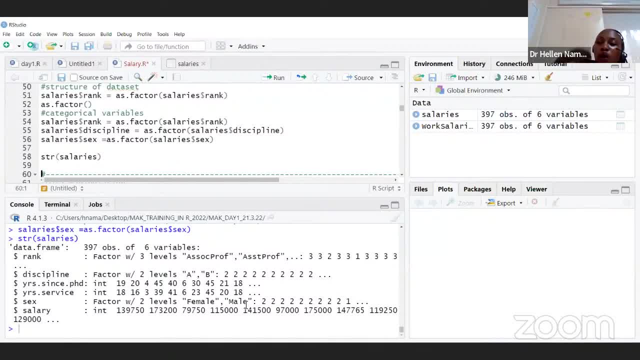 male. So now the point is: now, having put everything right, having understood my levels of measurement, I've now told R that you know what. now it is okay, I can proceed on with analysis. all my variables are read the way I want. 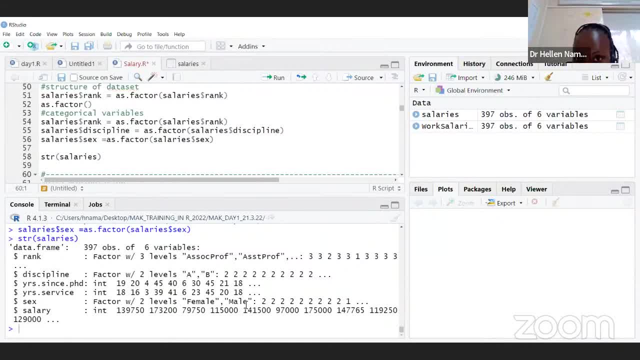 in R and then I'm good to continue. So let me ask him in the chat, is it okay? Okay, If you have further questions, please post them in the Q&A and then they will be answered If you're getting an error. 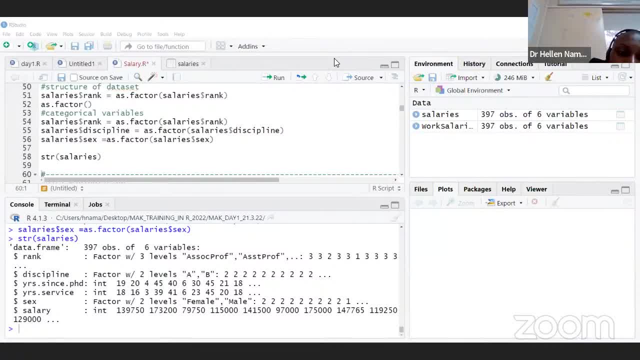 right now. it implies that you didn't load your libraries. That could be the problem, Because if the libraries were loaded successfully at this moment, I don't expect anyone to come up with an error If you're saying that you got lost a long time. 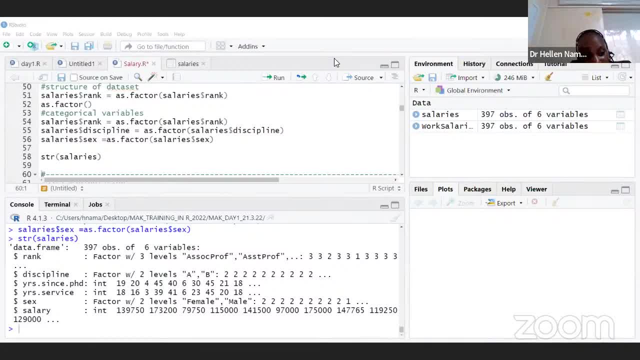 ago. please post the questions in the chat so that you're able to be answered. Let's make the learning interesting. Otherwise, if you get lost at one point and you don't mention it and you get lost, you will get stressed. Seems there was other. 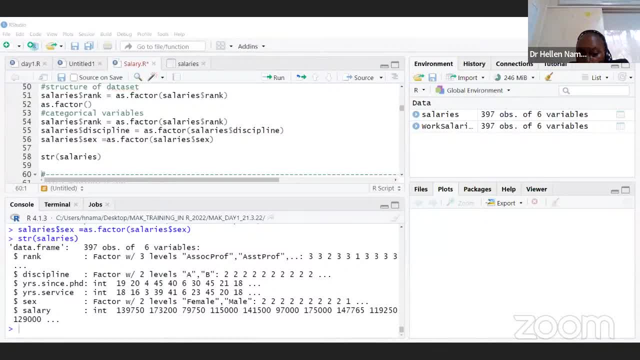 genders among the professionals? only male and female. No gender it is. we had only two, which is male and female. There are no other. Okay, Yeah, Now. do you ever think, now what is so interesting that you can do for you actually? 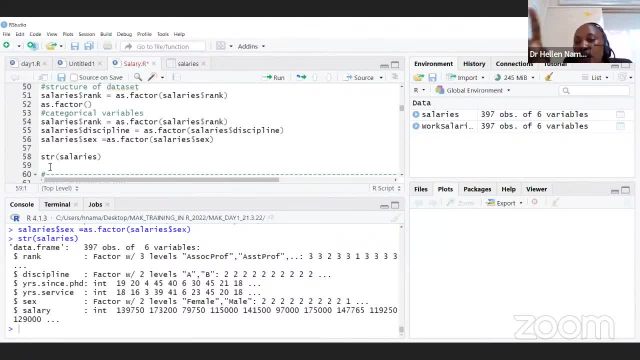 now to check if you've done the right thing, Let's run a summary command. I'm going to type summary. This is the command that is going to give me a summary of my data set. Okay, I type the summary command and then, inside the summary, 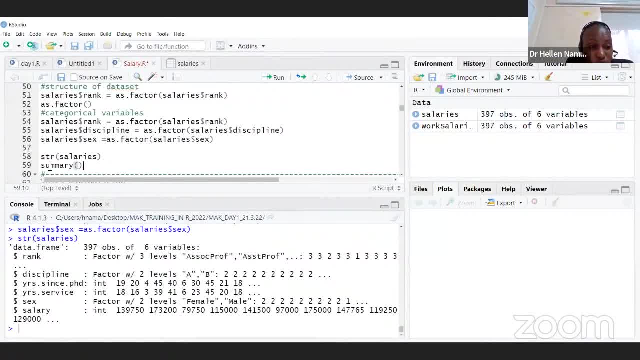 command. I type in the name of the data set, which is salaries. So I'm going to go back and I say salaries. I want to see a summary of the data set that I'm having. So the moment I get there I click. 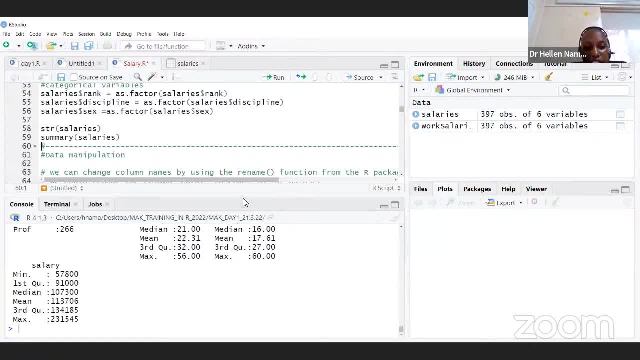 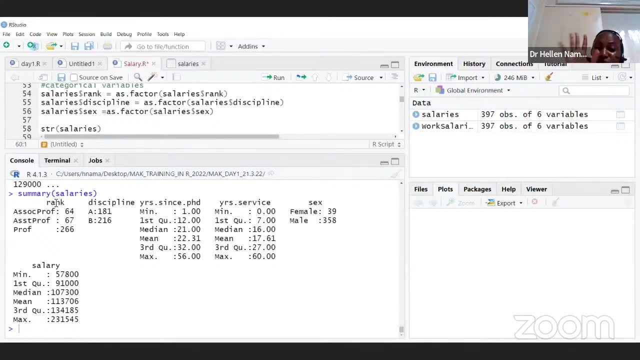 run. If I click run, I come in my R console. What is happening? It is showing me the summary of each variable right, This is actually the univariate part. It is showing me that, yes, we've got rank as a variable. 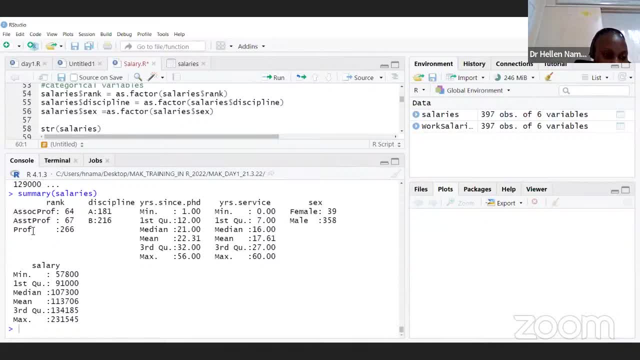 We have three levels: associate prof, assistant prof and prof. It further goes ahead to tell me the frequencies. The associate professor, they are 64.. They have 67 assistants and then 266 professors. When you come to discipline, there are: 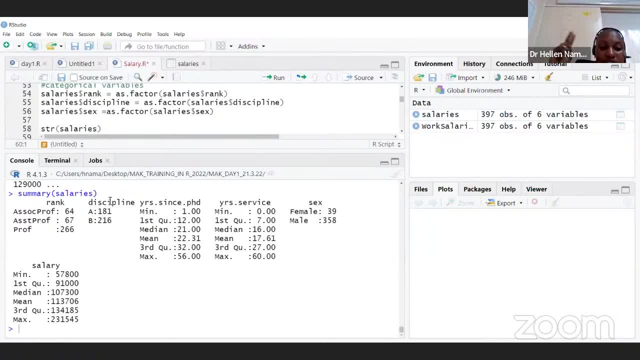 two of them, A and B: A- the humanities and B- the sciences, with the respective numbers When you come to the integers, it is giving you a statistics summary from the minimum to the maximum. The minimum, the first quartile, the median. 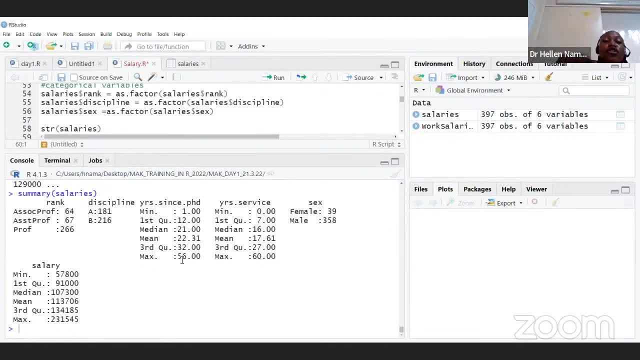 the mean, the third quartile and then the maximum. Whenever you're running a continuous variable, a numerical variable, you'll come up with always a summary statistics with five points. It is telling you: for the case of sex, we've got two. 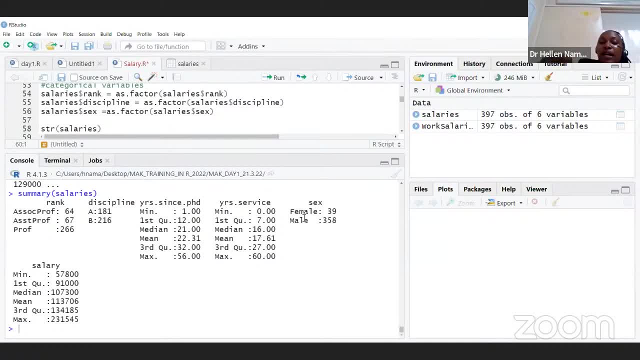 levels- female and male- and the numbers respectively. Salary was numerical in nature and it is showing you a summary: the lowest salary, the median, the mean salary and the maximum salary. That is how interesting the summary command works. I think you've seen the relevancy. 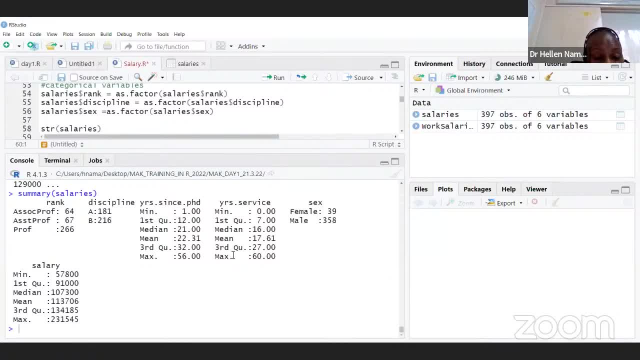 of why we have to combat our categorical variables from character to factor. Let me ask in the chat again: are we on the same page? Okay, Dr Thomas, we have attendants today, Attendants alone. We do it tomorrow, Okay, 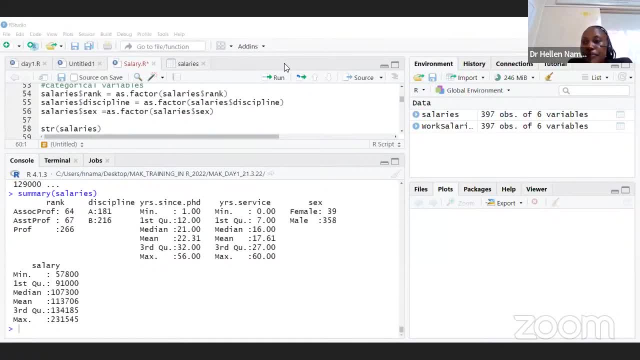 Because they're asking for it. All right, Thank you, Thank you, Okay. All right then. Now I'm glad that I'm receiving a positive response. Somebody is saying that the prayer and lunchtime praise we are stopping at 2, and then 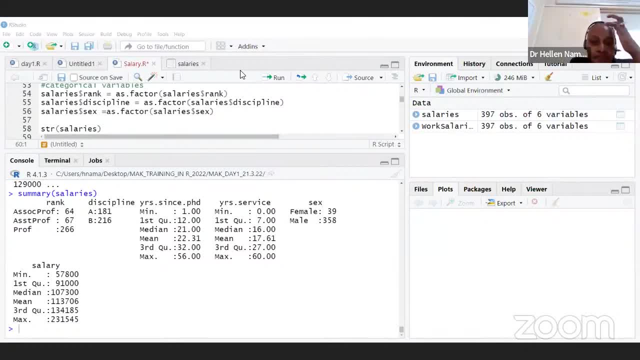 we'll break off for today. Let's try to. Raymond is saying that I see most of the syntax logic relate to Python. Yeah, you're very right, because the point is understanding the different commands and then because this language they're. 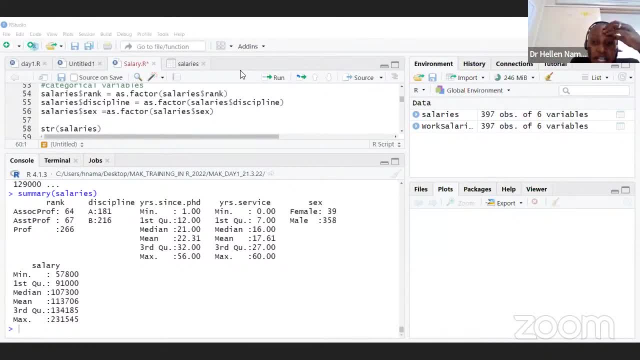 in one or another, they're somehow interconnected. So it's a matter of getting to know what you're supposed to do and what each particular command really wants, and then you'll be able to do what is right. Okay, let's continue. 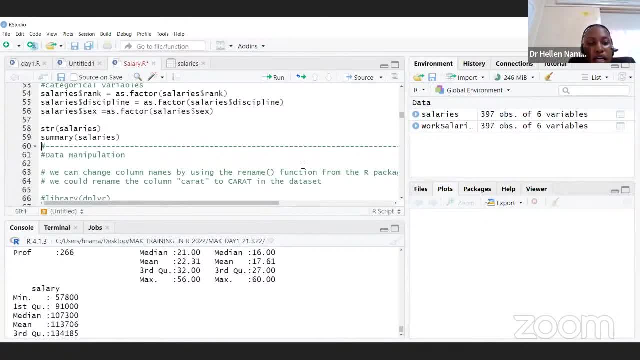 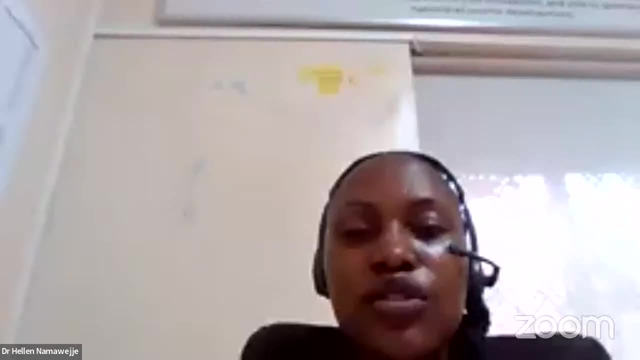 Now we are moving on to the next slide. We have two versions. The second part of data manipulation. Let me first share the word and go through it briefly. If time- I hope time will allow- doesn't allow, then we'll also. 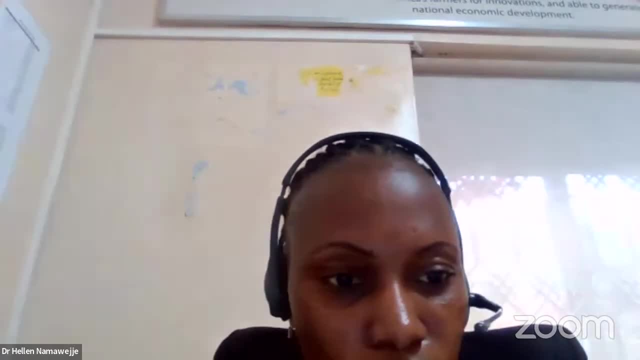 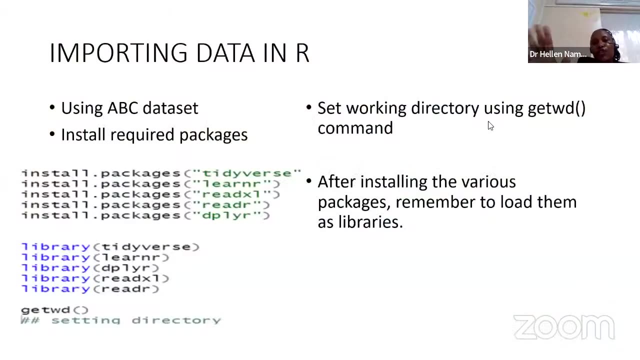 decide otherwise how to move on. Let me share my PowerPoint again. That was the little bit of the introduction of R programming language: how you can import and so on, Importing data into R. we've achieved that today, In case you're importing the file. 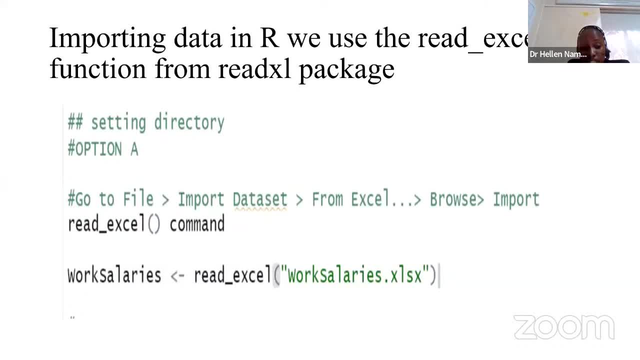 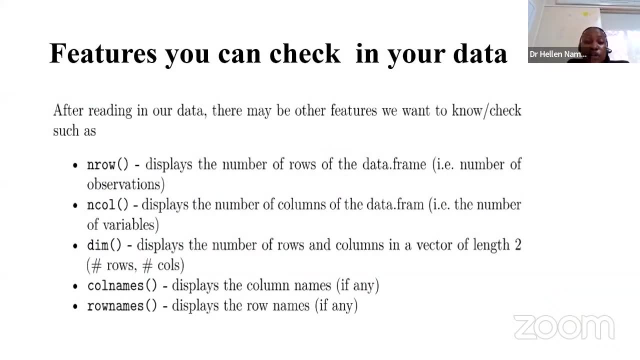 saved as XLS. we've achieved that by using the readXL package. We've imported the one that is saved as CSV. Some of the features that you can check in your data. please check the PowerPoint that we sent or you can check it on a Google link. 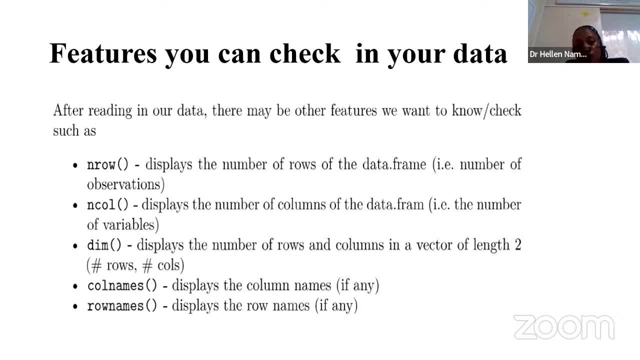 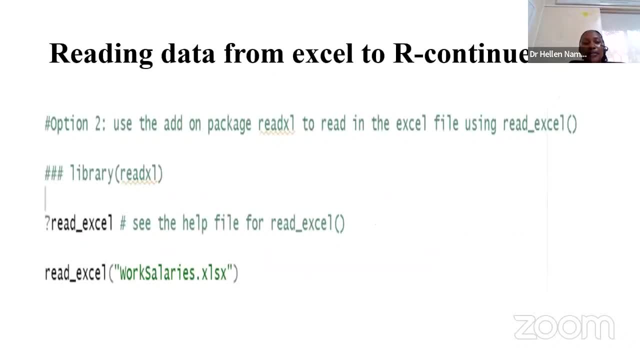 and see how these are inbuilt commands that you can use- and we've also seen them: The use of comments, as you said, the Actors Reminders, then reading data from Excel to R. this is just a continuation. Other important features that are: 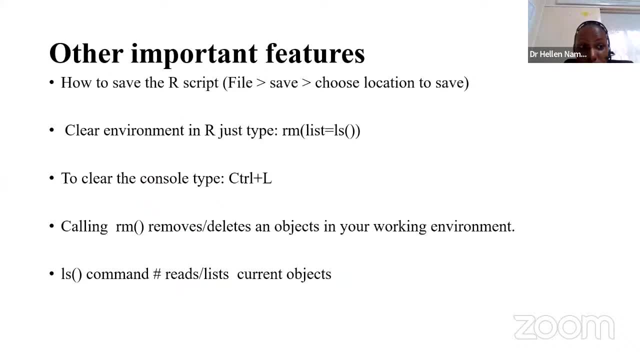 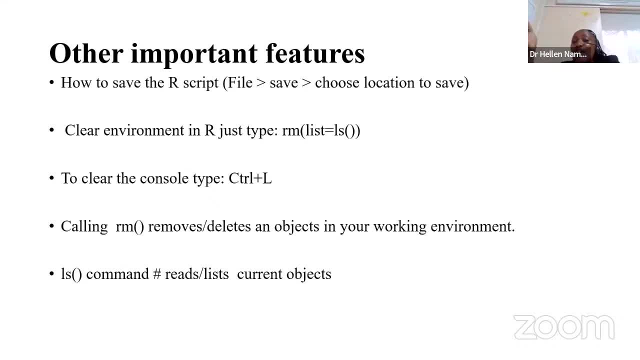 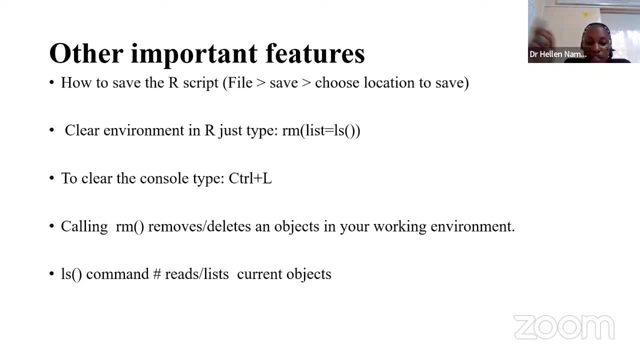 clean your environment. we use the remove. I've already shared about that. Then I mentioned that in this particular command- sorry- I mentioned that R means remove or delete all the objects in the working environment and then list equal to LS. that list removes. 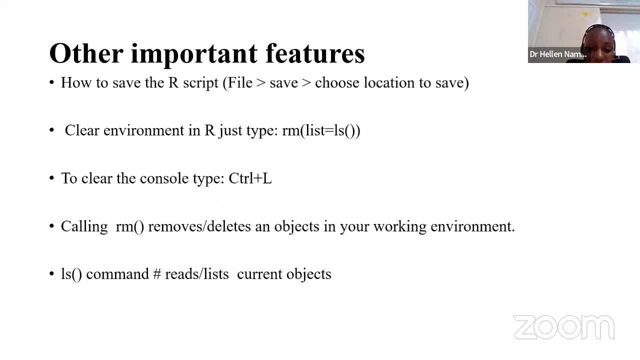 all the current work that you've stored in the environment. So you can, in case you have a lot of things and you're getting perturbed, maybe you get a point and you get confused on the results that you are getting. so you can clear and then resume. 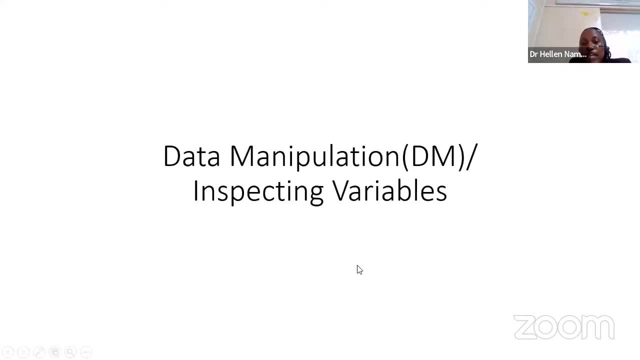 again. Now we are moving on into data manipulation. You know it is always important that as you're importing your data in R, whatever, because sometimes you go to the field and you bring when your data is not clean, you have to do some little bit of inspecting. 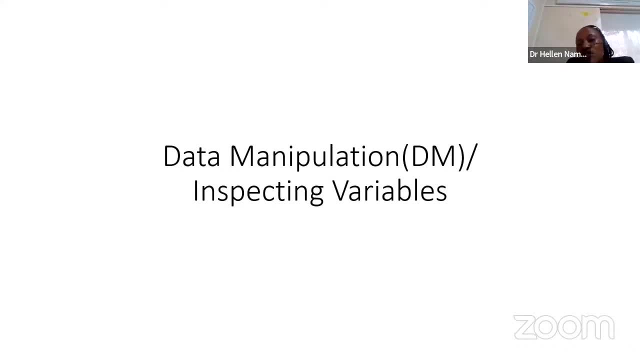 your variables and check to see: okay, when I went to the field, this was captured this way- were my responses complete? or what can I do before I, really before even I do my regressions? Maybe there's a certain variable that I need to create. 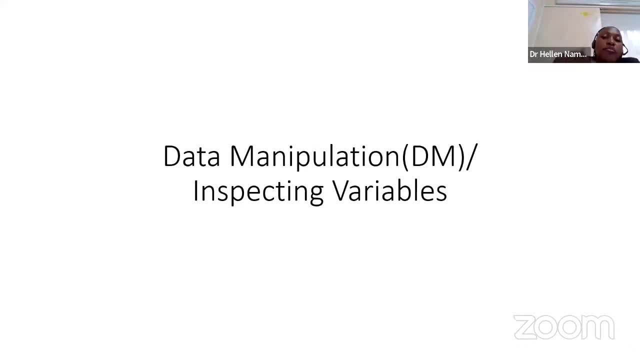 from the existing variables that I want, such that it is able to act as my dependent variable. The way you hear the word manipulation: you're trying to use the variables that you have and either you clean or you record or you delete all that. 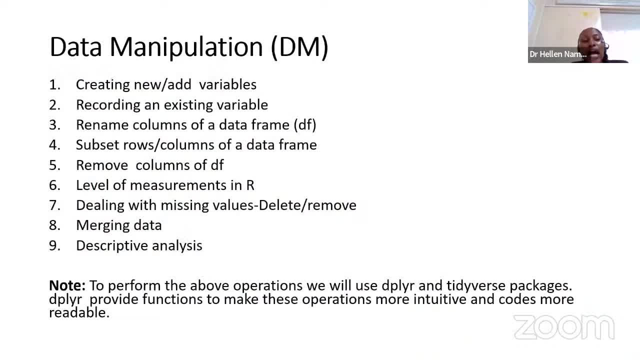 So I mentioned about that particular slide. So under data manipulation, which I'm calling the DM, okay, you can be able to do these nine things. You can be able to create new or add a variable. You can be able to record an existing variable. 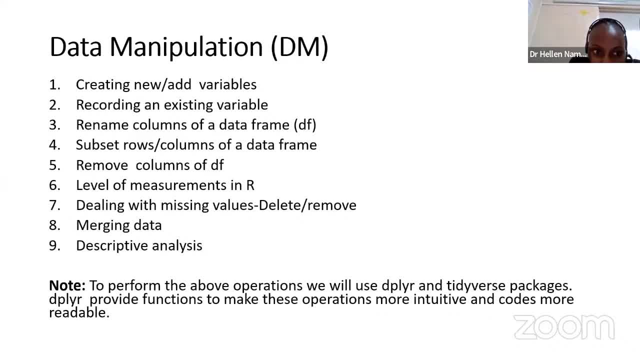 You can be able to rename the columns of the data flame. You can be able to remove a column. You can be able to deal with things that you either remove or use further analysis. You can merge data and you can do descriptive analysis at the same time. So 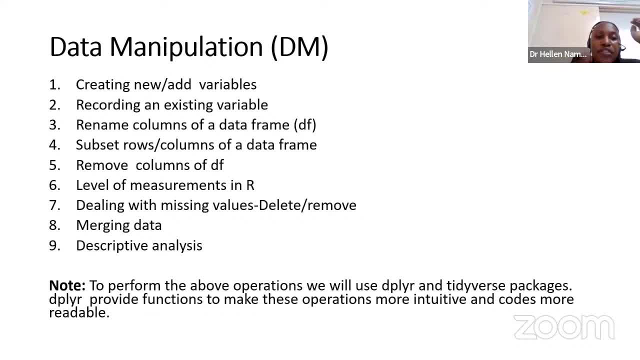 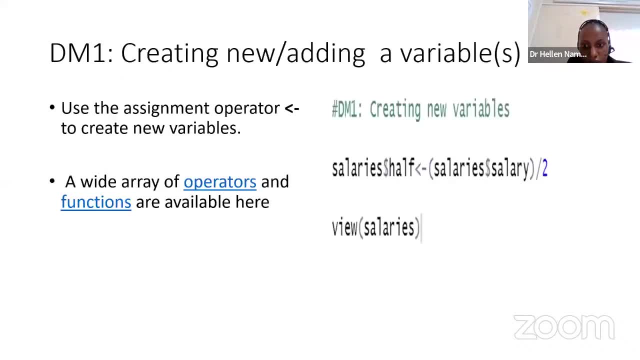 given the remaining time. let's see how far can we go with that. Of course, all these things can be done. Let's first get a theory, bit a little bit, and then we move back to R. Okay, Now, within this data set again, for example, 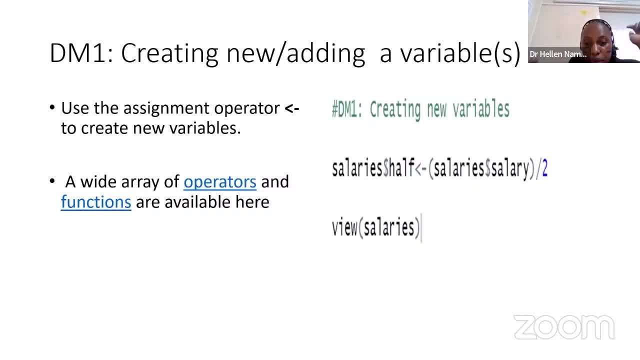 in case you want to create a new or add a variable within my data set I've got. I can create another data set called half. Sorry, another column. I'm creating a new variable called half. Maybe I need to get the half salaries of the. 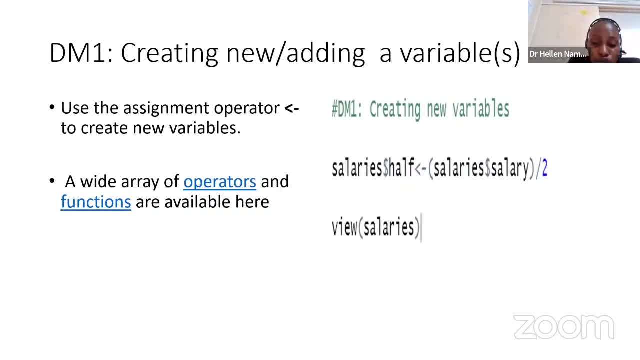 respective, of the respective runs. All I need to do is to create another variable called half, And then after that and after that I from the salaries I say divide by two. Okay, And then I see if that one has worked. 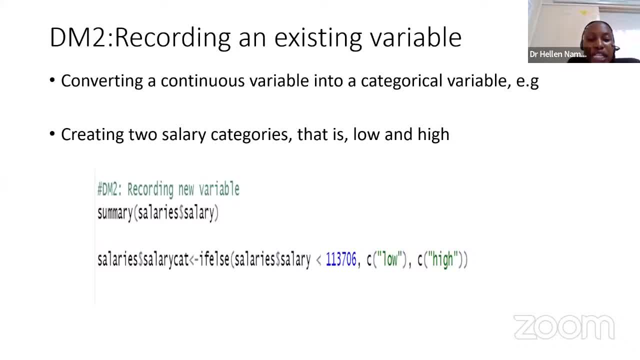 I can be number two, re-recording a new variable. I can have a new variable, for example, in my data set which has good salaries, But then at the back of my mind I want to see those who get low salaries. I can categorize. 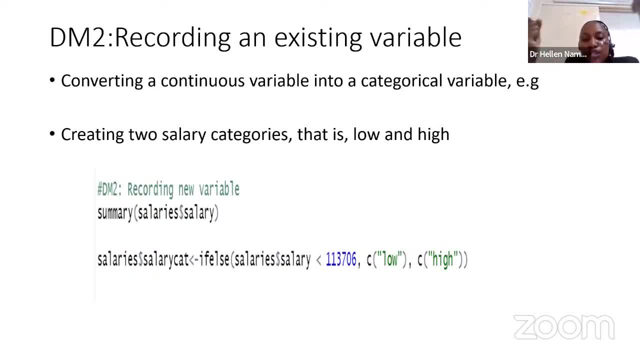 it as low and then high, Depending on the threshold that I want. I can say, maybe, looking at my, looking at my summary statistics, I can consider my mean as the threshold. So those who are below my mean, I'm going to categorize them. 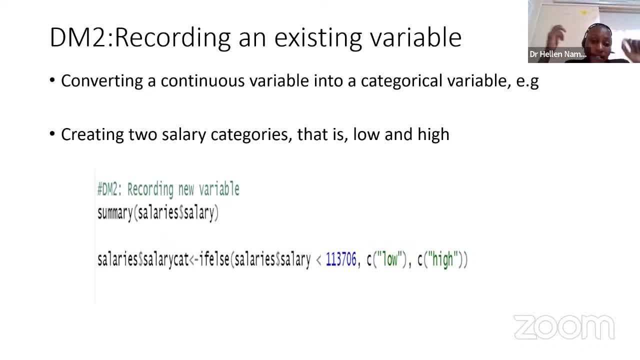 as low. Those who are above the mean. I'm going to categorize them as high. That is all data manipulation From the rate of existing. you're trying to do to record another variable that is important or you need to use to achieve the objective that you. 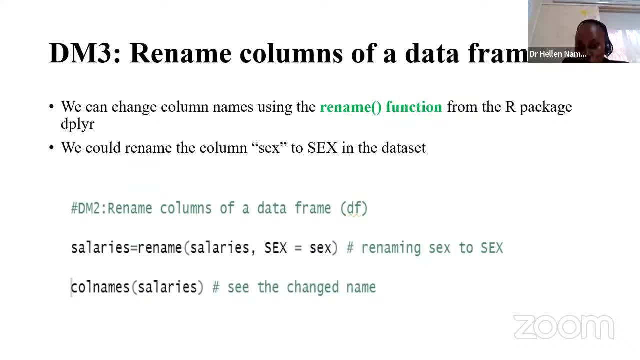 want to get. Okay, You can also rename columns. Sometimes you might be working and maybe you feel the names are confusing you, So we'll use the rename, the rename command or the rename function to see how can you rename a particular column to what you want. 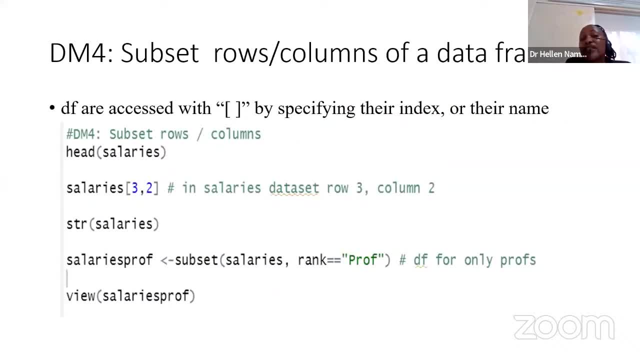 it to and then to check if it has really worked. We can subset rows and columns in the sense that sometimes maybe, for example, we looked at the rank variable, which has three categories: the professor, the associate and then the assistant. Maybe you as a new? 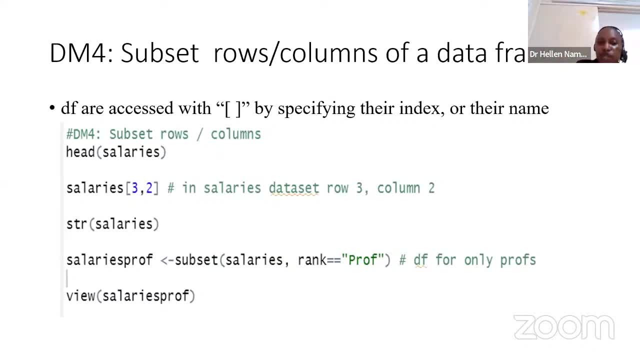 individual. you might be interested in working with only professors and you're not interested in the other levels. So how can you subset that group only from the main data set? That's what we refer to as subsetting, and we use the subset command and we can still. 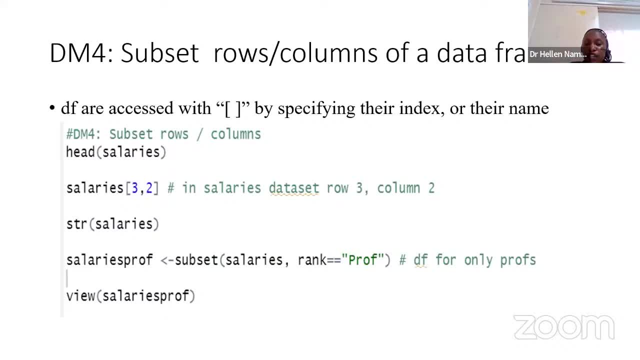 be able to see all how this is being done into R, For example. maybe some of you are in agriculture or you went and collected data from different plots of land and you're like: no, in my analysis. I only want to deal with plot A and 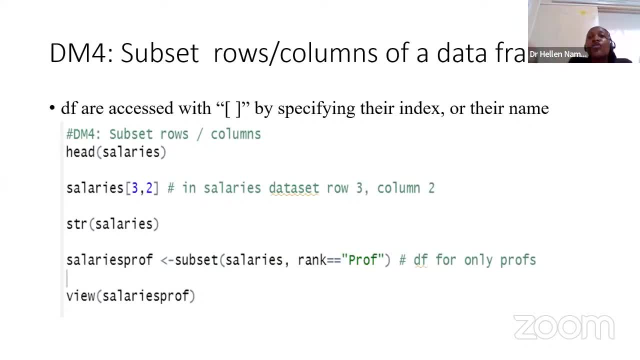 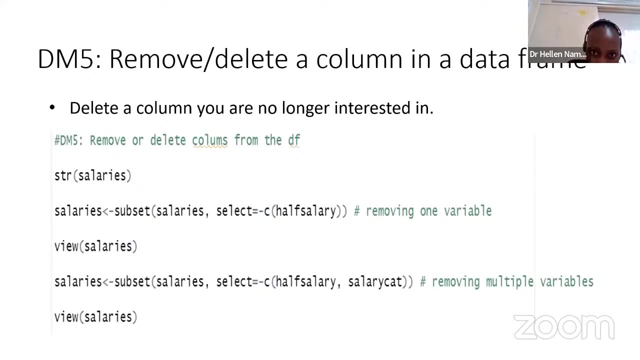 for now and do away with plot B, So you can use the subset command and only concentrate on what you want to work on. Maybe later you can see the interplay of other groups joined in. I'm saying that you can also remove and delete a command. 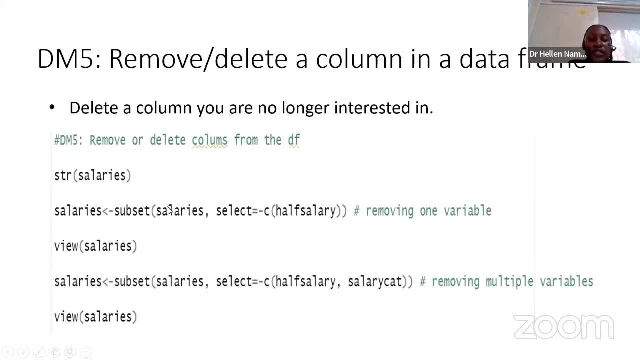 delete a column. How do we do that? We still use the subset command and also within the subset command, inside we put the select argument, The select, and then we put a minus sign. You're going to see this in R. You say that, no, within my data set. 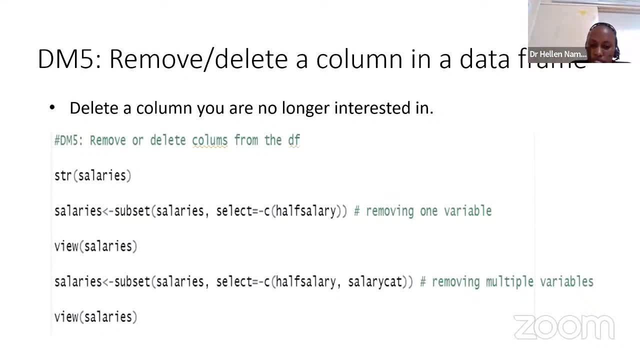 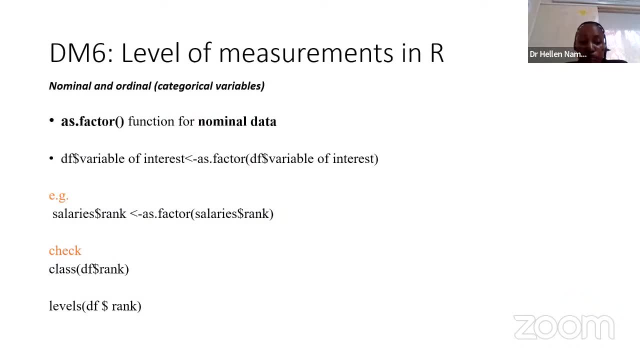 select this and delete it. I don't need it anymore and you can delete. You can delete one column. you can delete multiple columns, depending on what you want. I've already talked about the levels of measurements. that is important to understand whether you're dealing with. 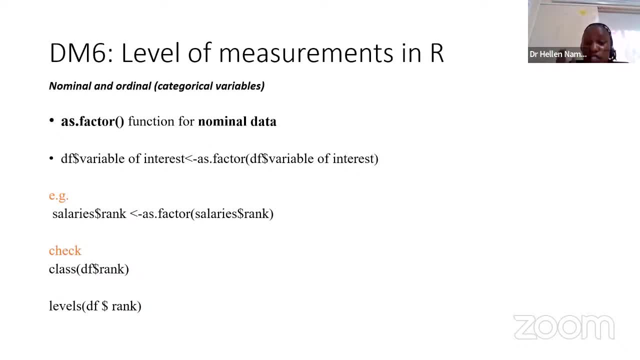 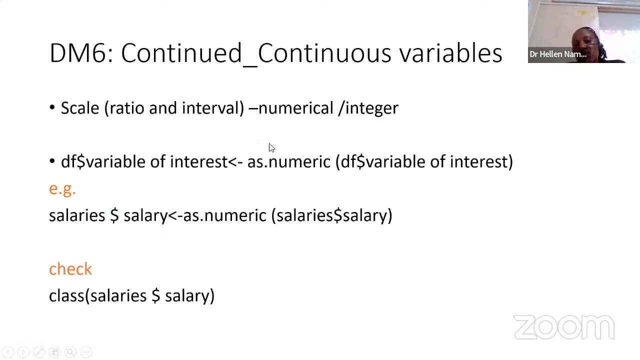 a nominal or a nodinal kind of variable. It is important to support you to do the right interpretation and the right statistic. I've already talked about the as a factor. Yes, there's also. in case there's, we have a command as numeric. 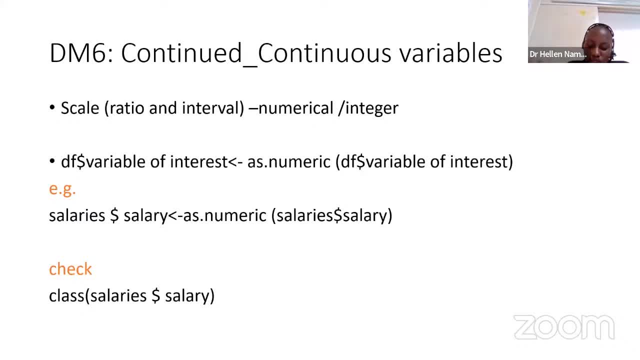 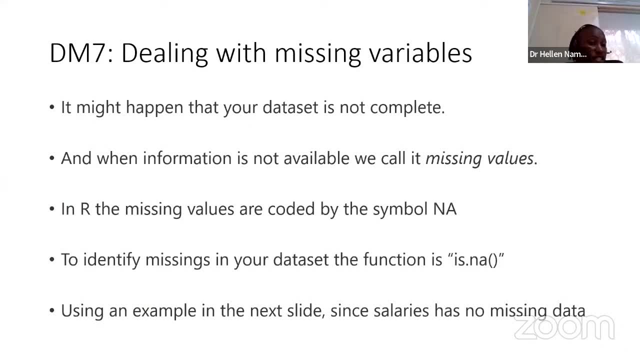 the old integers and numeric in nature numbers, continuous variables. R can still also look at that If time allows. we're going to look at how to deal with missing variables During this training. we are not going to go into details but 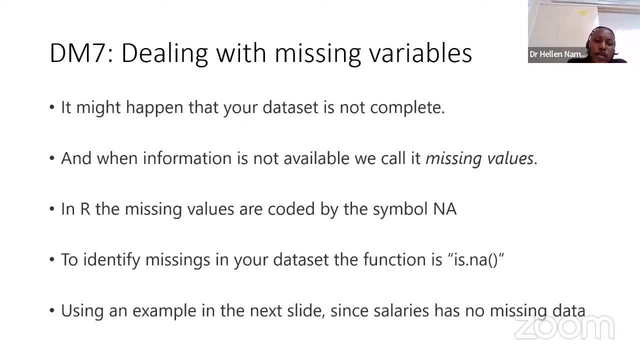 however, the thing that we are going to look at is: how do I tell that my data has got missing variables? Because you go to the field or as you go to work out in a survey, some of the responses are not filled and the time you get back on your desk. 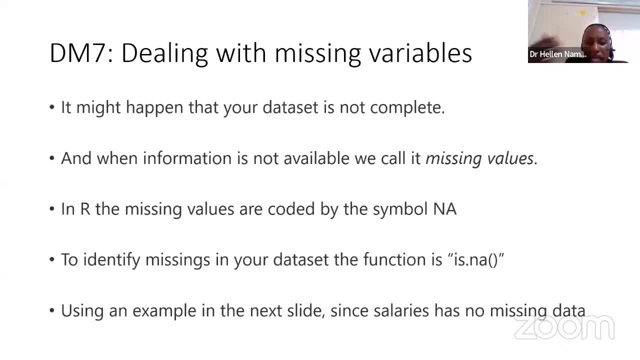 some of the points are missing. We are going to see how do you locate that in case your data is incomplete, and then in R, how does R look at missing data? and then how do you identify the missingness Within the data set that you have? 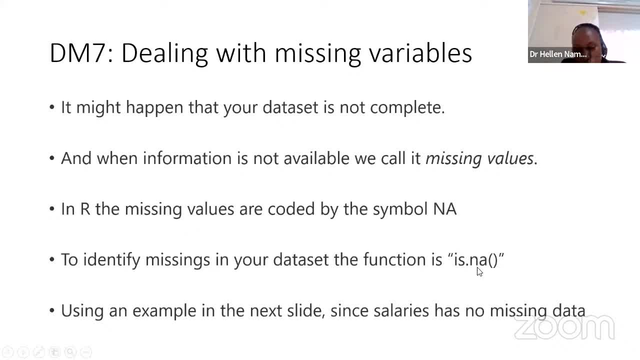 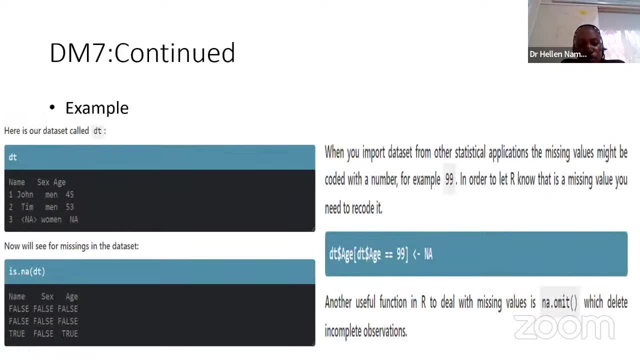 Here. I wrote that you use the isend a command. We are going to see how to use that. I said that when we move on to the next slide, we are seeing that. this was just an example that can support us to understand, in case 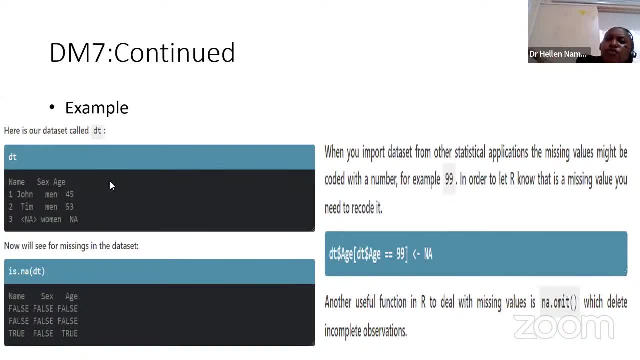 you've got missing data. Assuming I've got a small data set, because the moment with this small data set it is the same theory that applies to the big data set. Assuming I've got this data set, DT with name, sex and then age. These are the variables. 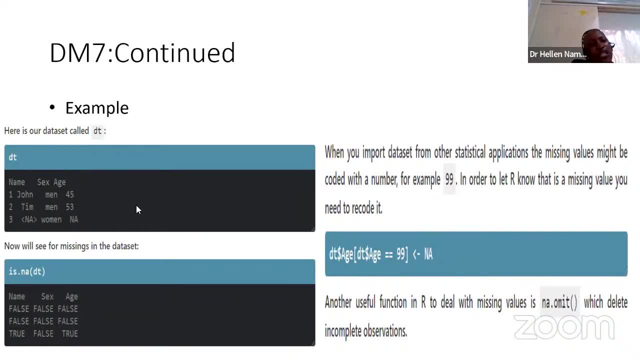 Under the names I've got. the dimension is three by three. I've got three variables and three observations. I'm having John Tim, then NA In R. whenever you see NA, it implies that not applicable. It is telling that I'm not seeing. 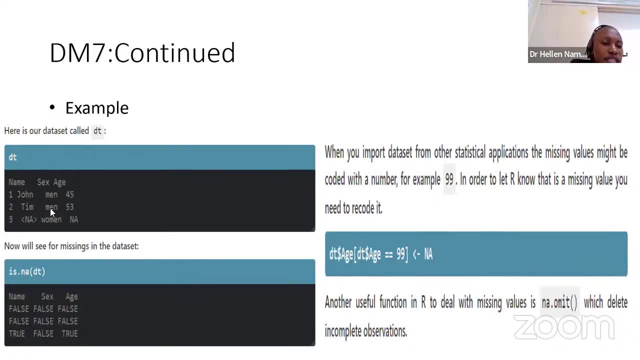 anything. It is empty. Then it is telling you the sex and then it's telling you the age. What we are going to do that now for you to see the missingness in your data, the command that we are going to use when you go back to the 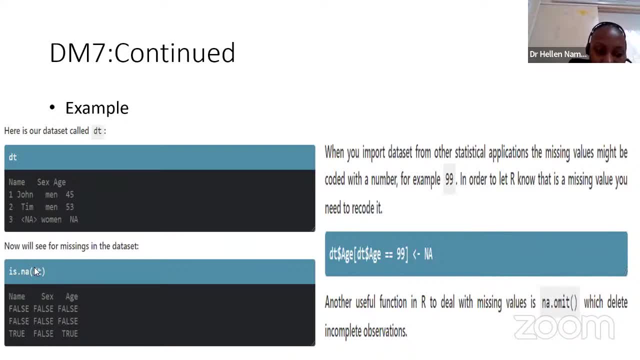 practicals it is isNA. in brackets you put the name of the data set. The moment you run this particular line, whenever it is going to bring to logical output a yes, a true and a false. Where there is false, it implies 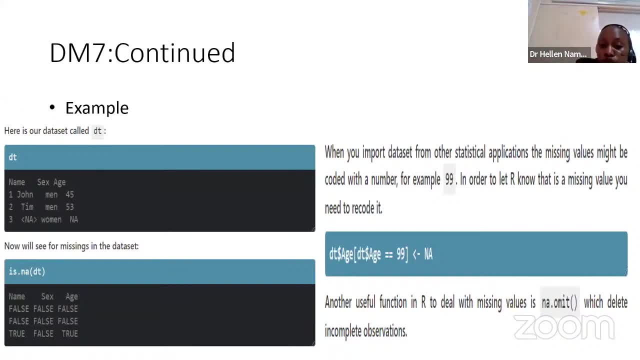 that the data point exists Where it brings true, it implies that there is a missing point. there is a missing data set there, Like on this particular output. we are going to do it in R and you see it automatically Where there are recordings it is showing. 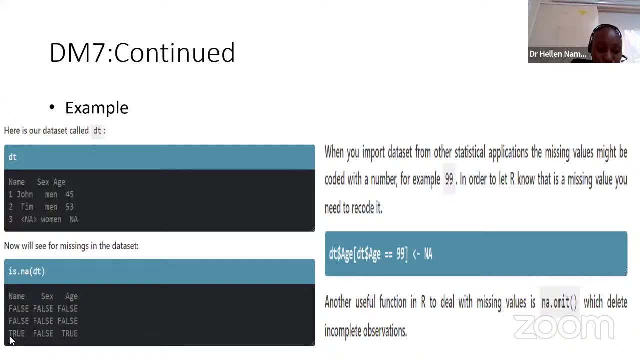 false, Then where we have NA, it is showing you true. These true ones are the ones that enable you to understand that my data is missing certain data points. You can be able to go back again at the start, or you even go back and check. 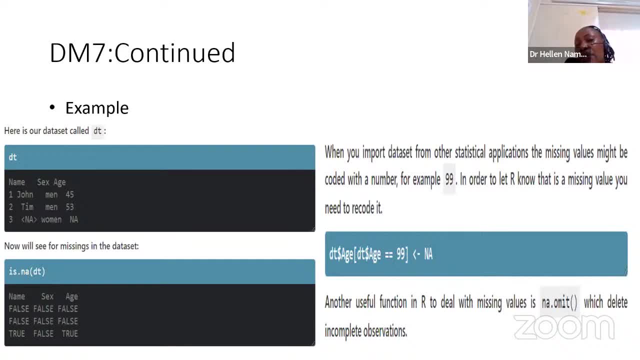 in your data set and you ask yourself: did I really input in my data well, or what happened? How come I've got many missing? Maybe do I need to do some data imputation and so on. We are going to see how to use in case you've got. 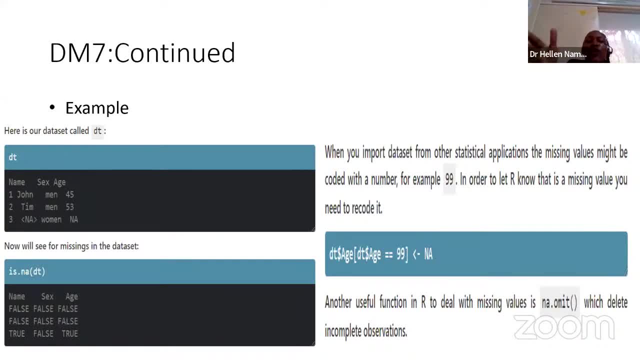 for example, a million observations and you only want to deal with the only complete result. maybe at the back of your mind you're like: I want to do with only a complete data set, I want to do away with incomplete data set. That is also. 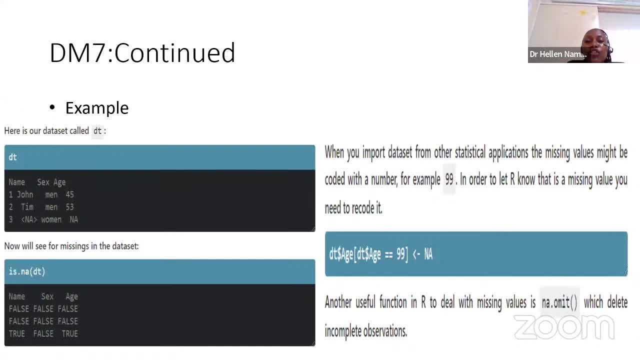 very risky because each time you remove, each time you're deleting out certain rows with certain columns with missing information, it implies that a lot of information is being lost. As you are advancing analysis, you will see that there are various methods on how you can do data imputation. 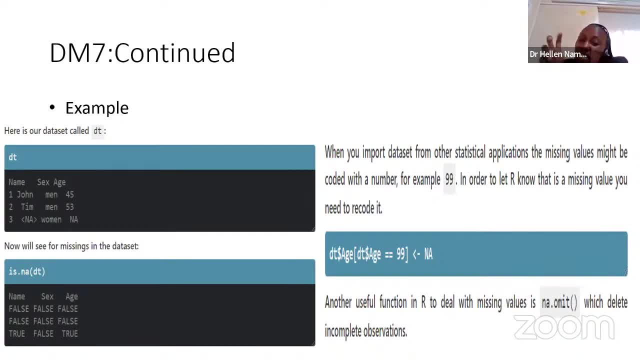 To see that you don't lose a lot of information. In case you want to deal with only complete data, we use the command NAOMIT- NAOMIT. In brackets you put the name of your data set That one will produce for you only. 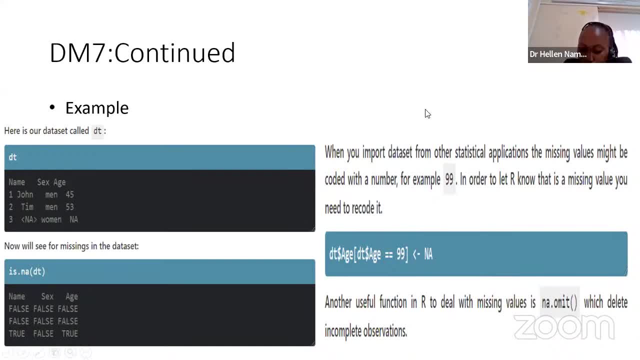 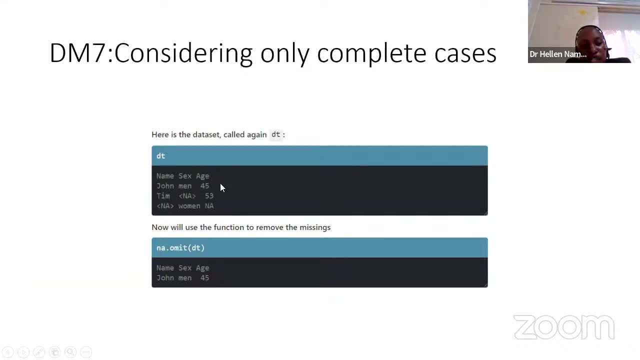 complete data. It will only bring for you only a complete data set. This is an example from what we had earlier. We saw that when you look at this particular data set, I've got NA here implying that this person did not, the sex was not recorded. 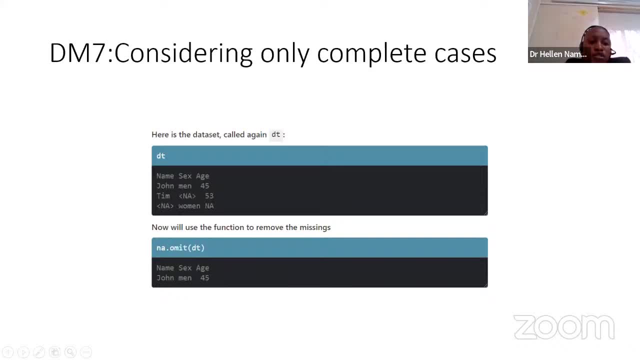 When you come to the third person, the name was not written. In case you want to do away with all missing variables, all you need to type is NAOMIT, NAOMIT, and then, in brackets, you put the name of the data set. 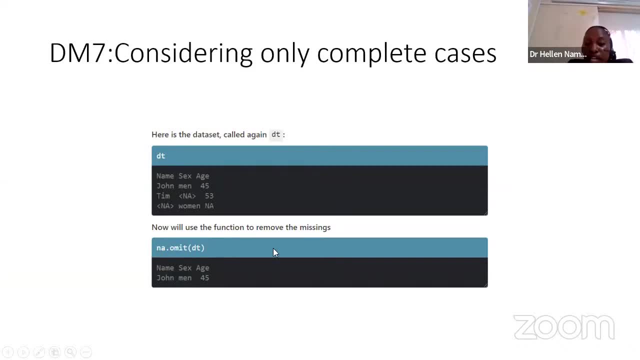 The result that you're going to get. it is going to show you the output that you will get. It will only give you complete cases When it has deleted all the rest that are not complete. Then it's up to you to think and 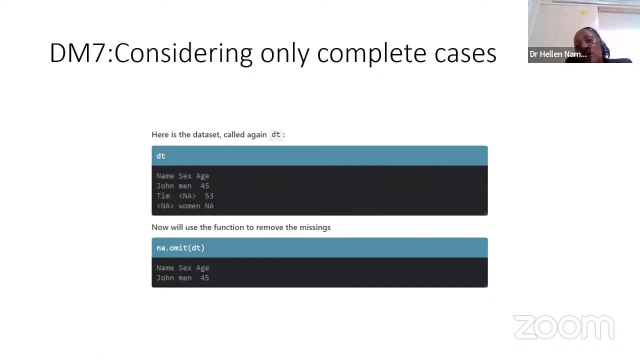 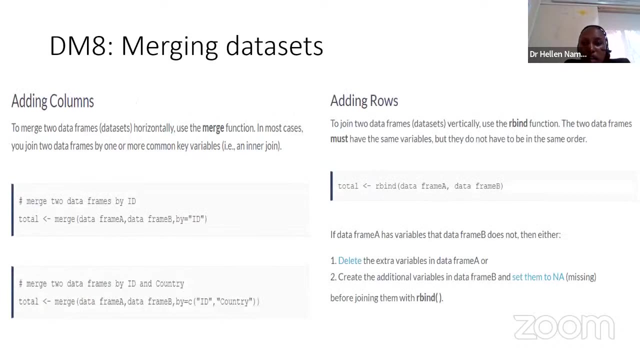 say: can I continue with this data set with complete result or it might give me misleading information and I need also to deal with the missing results. You will read that particular bit and so on. We've got how to emerge data, Emerging data. 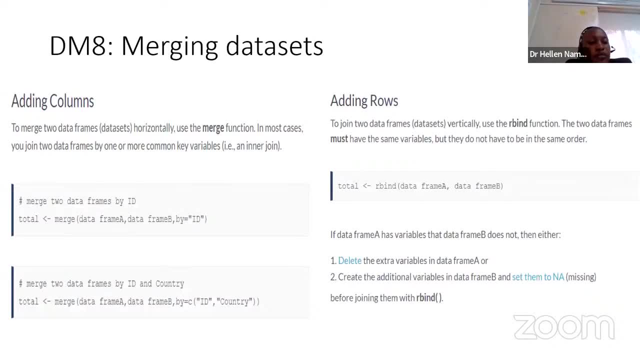 There are various ways. Sometimes, for example, maybe you're collecting data set from various points, But then at the end of the day, they could. you want to emerge these data sets Also. R gives you that option on how you can emerge data. 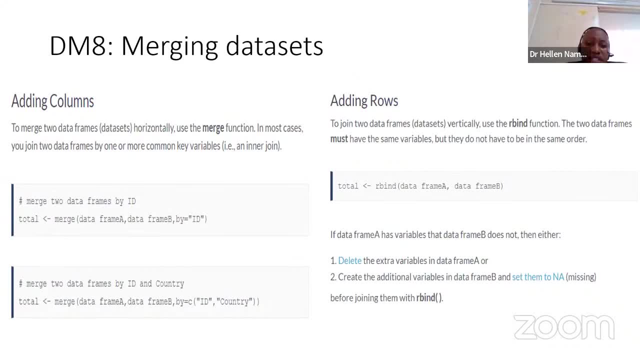 I don't know whether you've. if you've looked at the national data sets that are being collected, They tend to collect data within either Stata or in Excel, And then you need to know how do I, in case I've got two data. 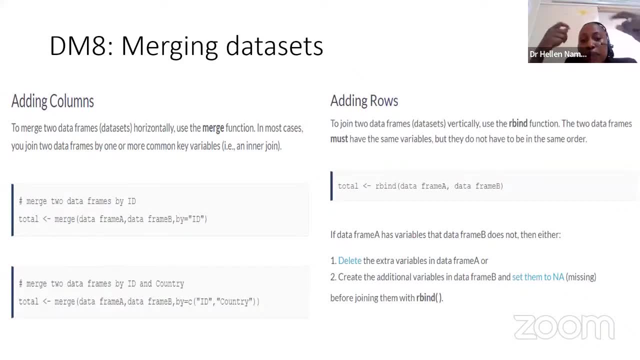 sets of interest which have got, for example, common identity, and I want to merge them together. How do I do it in R? It is also something very important that we can consider The other thing when you're joining data. there are also 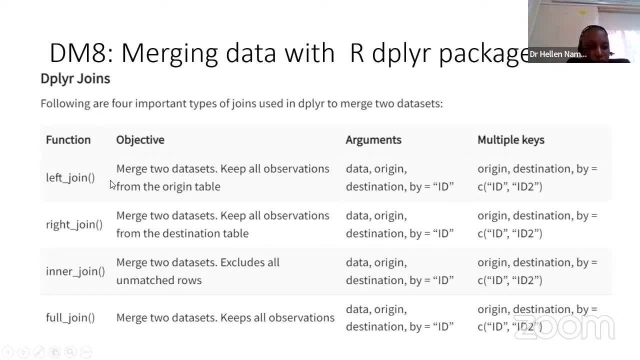 some other interesting functions that you can use, like the left join, the right join, the inner join and then the full join With the left join, as we are going to discuss. in this particular case, you're merging two data sets, but you 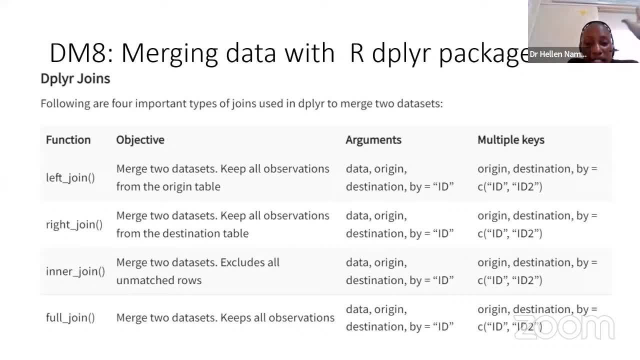 want to keep all the observations in the first data set, That is, the left join In the right join. you're having two data sets, but you want to keep all the observations in the second data set. In this particular case they are referring to as the. 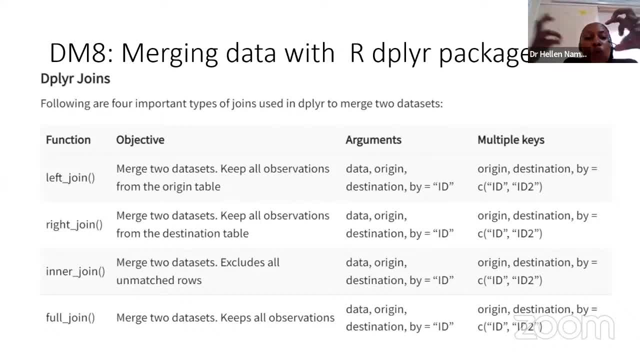 destination table. There are two of them: Inner join. what it does the word inner? it looks at the intersection. It only brings out the common points, that are, the common rows that are within the first data set and the second data set. 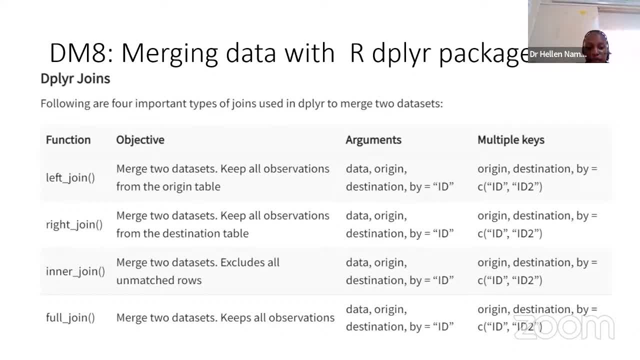 It will exclude all the unmatching rows. Then the full join for it. what it will do? it will merge everything for you. It is up to you to decide which data set you can use. It is also sometimes important to understand. okay, I've got different. 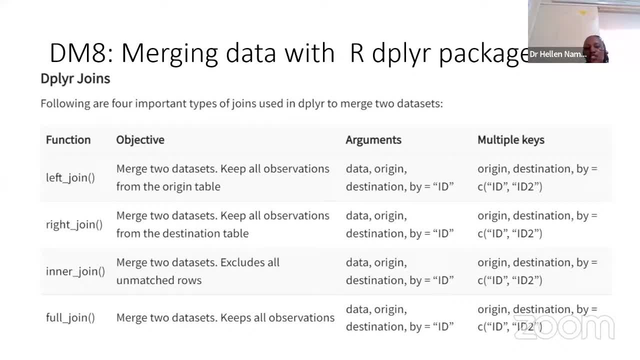 data sets. In case I merge them, do I need to just get those that are common? Do I need to shift up everything or I'm going to only take the ones that are common in the different data set? It's important that these 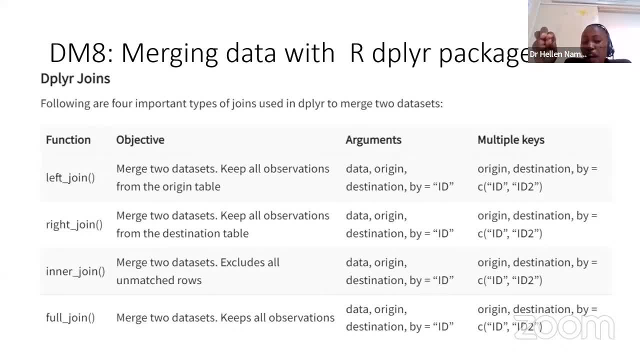 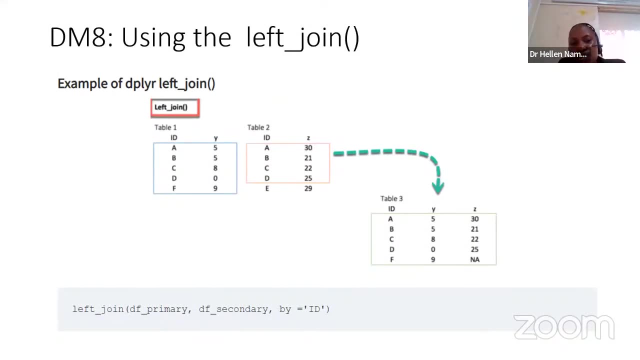 two data sets have got an ID or they have got a common column which is going to help you to merge these two data sets together In R. you can do it very perfectly. Like I said, this is a theory bit. We are going to see. 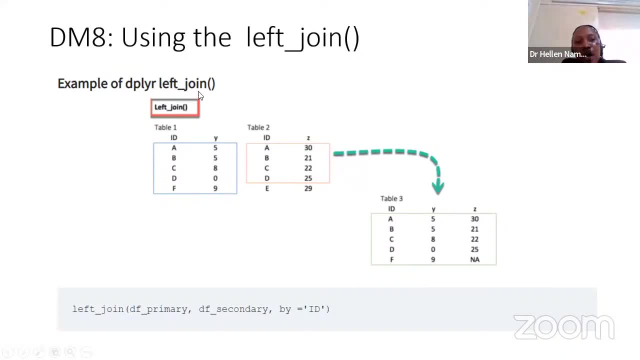 how practically we can move to R. I've already mentioned about this example We are using. if you remember, the deployer command I mentioned supports us in data manipulation. It is a reason why I'm saying: each package you put there is a reason why you're using. 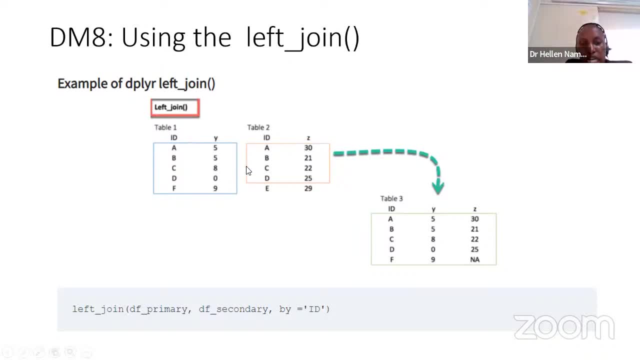 it The left join. I've got two tables. Refer to them as two data sets. I've got table one. That is my data set one. I've got table two. That is my data set two. We are going to do it in practice. 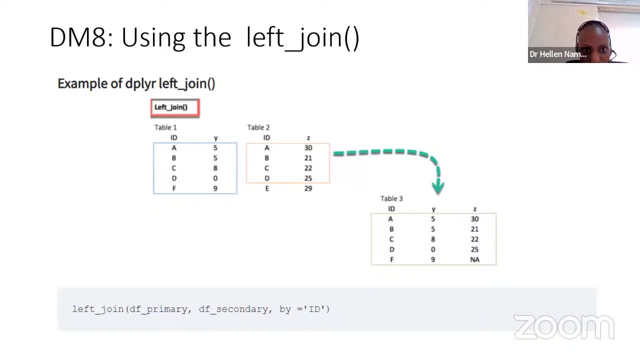 In R using two data sets, Or I can even leave it as homework. Within this first table, which is data set one, it has got ID A, B, C, D and F. Then it has got a Y variable In. 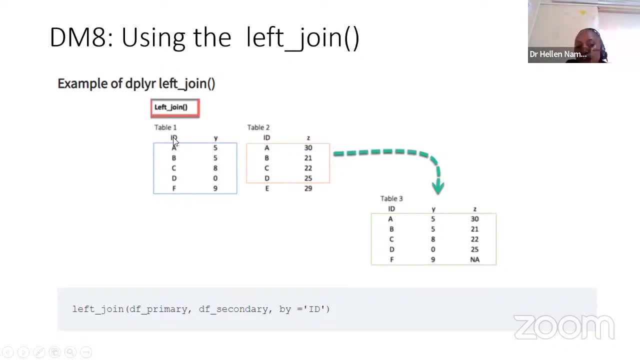 table two. it has got an ID. This ID is common to the first table one. It also has- and this one has- a Z variable, In case you want to merge these two together, assuming that these are your two data sets, the 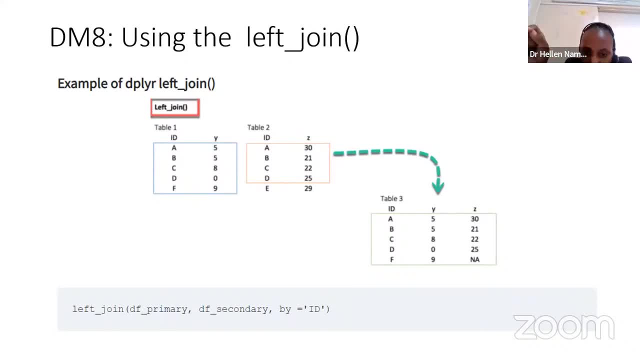 identity that is common in each is the ID, This particular data set. most of the time we merge them with identifiers that are unique in each. I'll use the left join command. Inside the left underscore join. I put in the name of my: 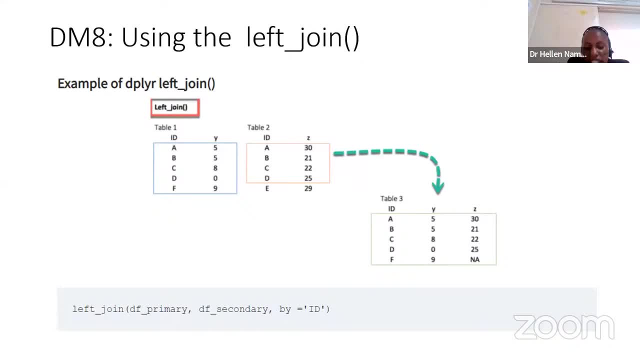 first data set I put in the name of my second data set. Then you want it to be joined by what? What is unique in both? What is common in both data sets? It is the ID, Even if you have many, many 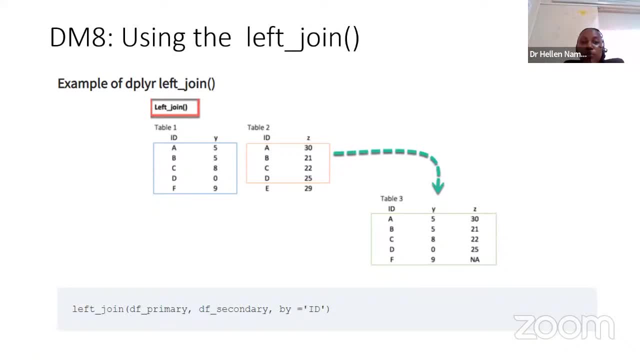 columns that are identical. you just need to put by what and everything will be sorted automatically with R. Okay, Like I said, with the left join, it will keep whatever left. you have got two tables. It will keep everything in the first data set. 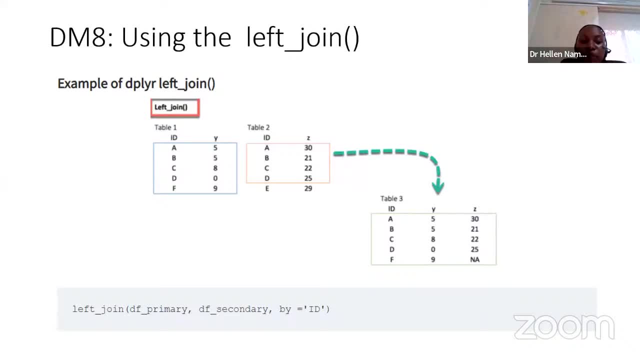 Whatever is in the first data set, it will keep and get information in what is in the second data set and it's a merge together, If you can see the output that you expect to get. at the end of the day, we are having A up to F. 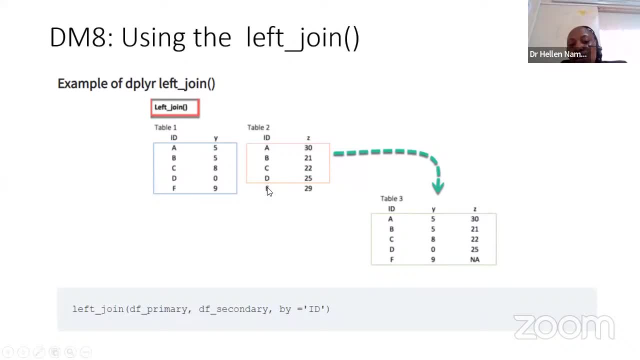 and in B. in table two there is up to D, So it has neglected E. It is not picking it, It is only taking everything in E. That's why, when you come to F, F, we don't have it in table B, So under. 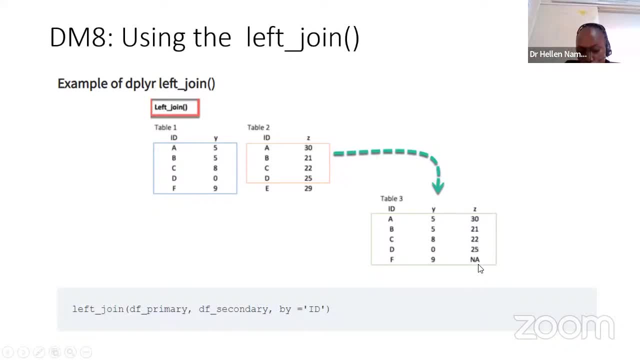 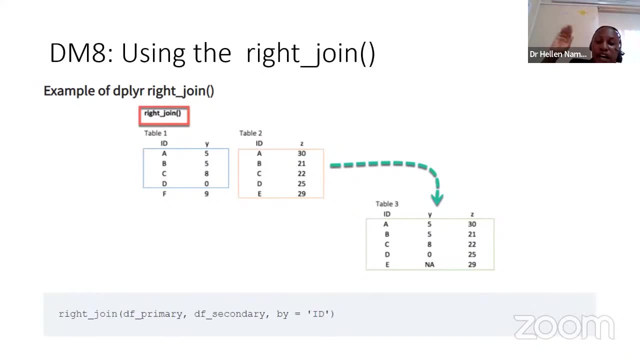 Z, it has put in A missing, not applicable Right. When you do the right join. it is now the opposite. It keeps all the elements in the second data set and matches it with what is in the first data set and 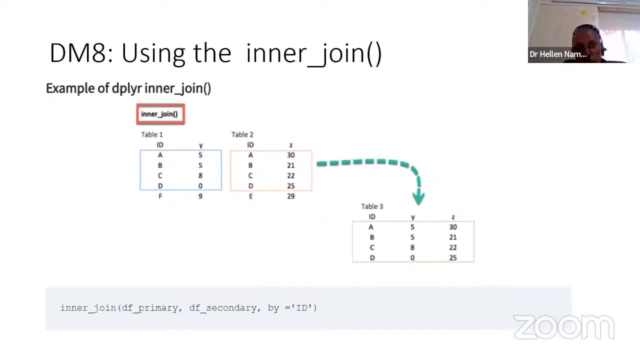 ignores whatever is not there In the inner join. what it will do? it will only bring out the common rows. It will join them together And then that is the output that you are going to see. All right, Do you see the? 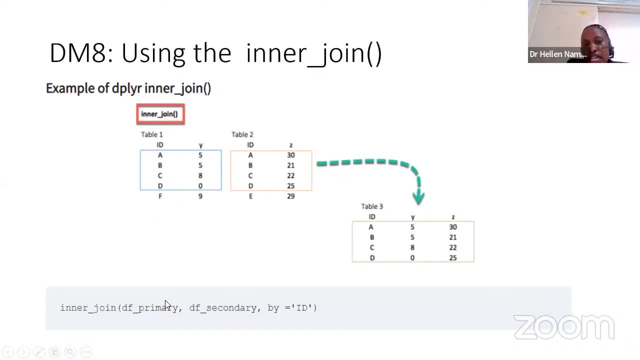 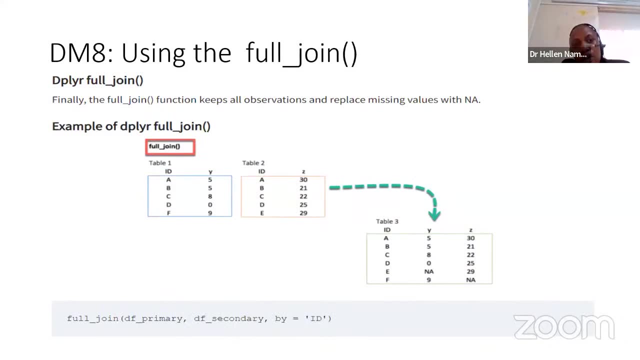 same command, inner join, put in the name of the first data set, the name of the second data set- you are identifying it with what? And then the last one is the full join. In this particular case, it emerges everything Where there is a missing. 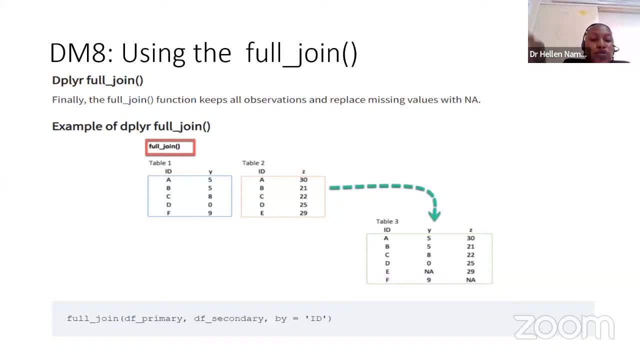 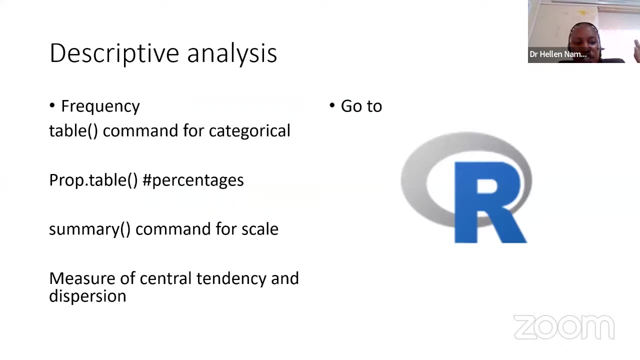 data point, it will put in A. That's when you get to know that, okay, there is no much, there is no variable, There is a missing data point at this particular one. So the rest is descriptive. We can do. I've already talked about.